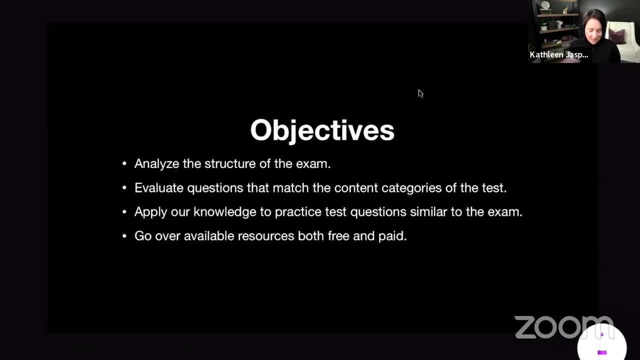 We're going to do purple, because you guys know I always do purple on my presentations. but today's objectives are: we're going to analyze the structure of the exam. That's one of the most important things to do. No matter what exam you're taking, you're going to want to really hone in on what's. 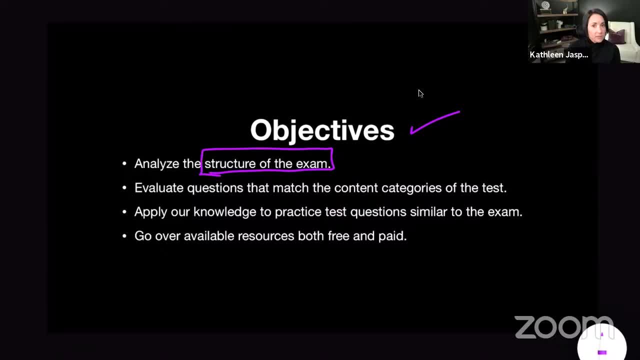 going on with that exam. What is it made up of? What skills are being asked of you? And I'm going to show you how to do that. Then we're going to evaluate questions that match the content categories of the test. So I'm going to show you. this is the type of question you'll see for this. 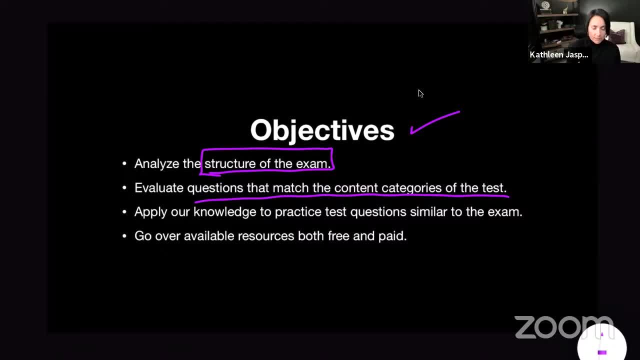 content category. This is the type of question you'll see for that content category. Then we're going to apply that knowledge to practice test questions That are similar to the exam. Are they exact? No, I have no idea what test you're going to take. 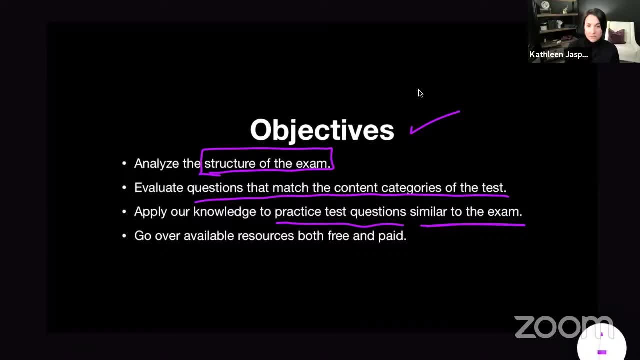 I have no idea what form you're going to get, but I do know the types of questions that you will get, So they will be similar but not exact, obviously, because it's a standardized assessment and we're not supposed to know what the test has on it And then go over available resources, both free and paid. 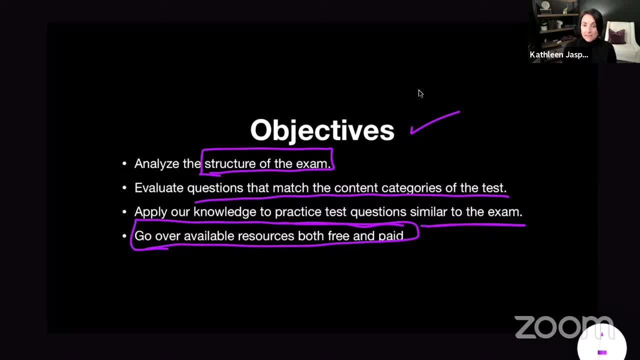 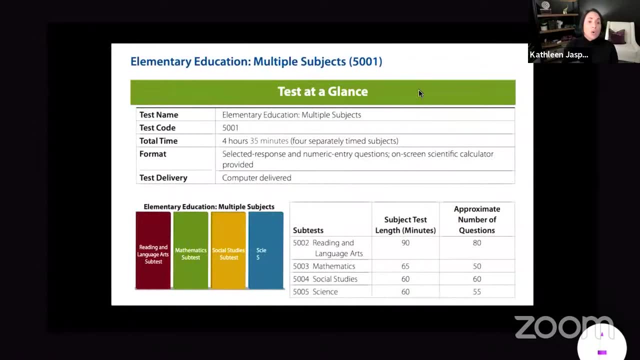 I'm going to show you where you can get more resources beyond this and I'm going to be jumping in and out of that. OK, so those are the objectives of today Presentation. So we are going through again multiple subjects: five zero, zero one. 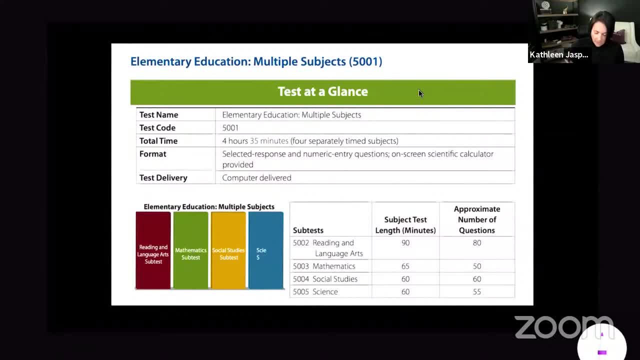 There are four main subject areas of this test, or subtest, I should say It's language arts and reading, mathematics, social science and science. We're actually going to start here today at five or three, Then we're going to go to five or four, Then we're going to go to five or five. 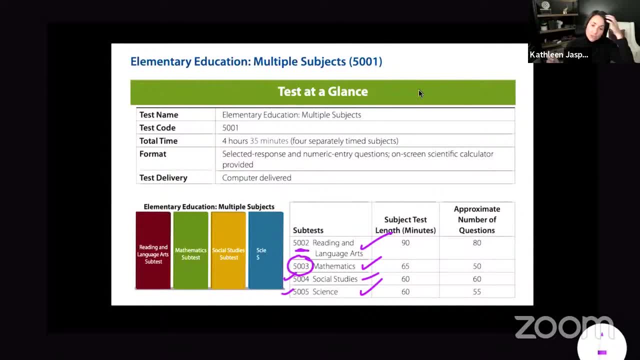 Then we're going to go to language arts. The reason I'm going backwards is usually when I do these webinars, I focus a lot on the language arts Because it is the bulk: It's 90 questions, It's the biggest, biggest part, or 90 minutes, 80 questions. 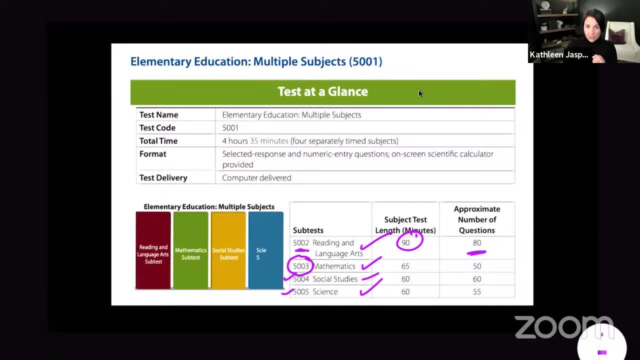 Sorry it's bigger than any others, But I just did a webinar on teaching reading. I've just done a webinar on Pearson foundations of reading. I have a giant playlist for teaching reading and usually the math, social studies and science gets a little pushed to the side. 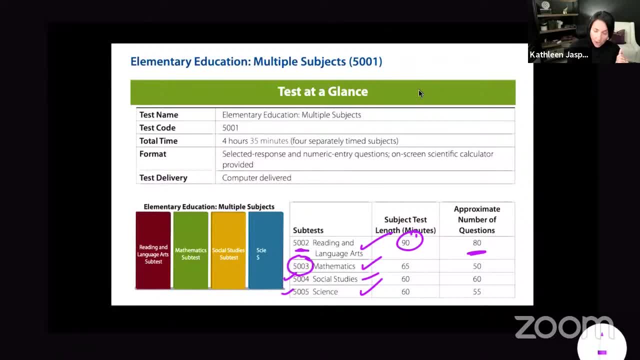 So I wanted to start below and then go back to reading and language arts. We are going to cover it, And I'm also going to show you where to get even more videos on that, because I have hammered Teaching reading for like two months, over the last two months. 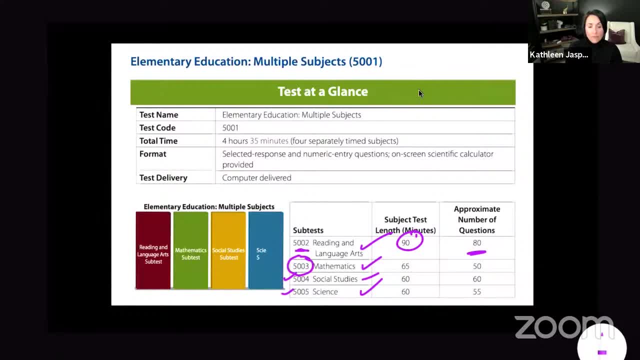 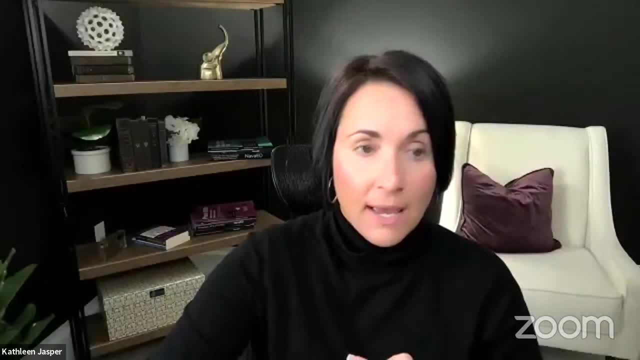 I've done so much on that, So I'm going to show you exactly where to find that We will cover it, but it's not going to be the first thing we cover. All right, Now let's go to. let me stop share here and just go screen here. 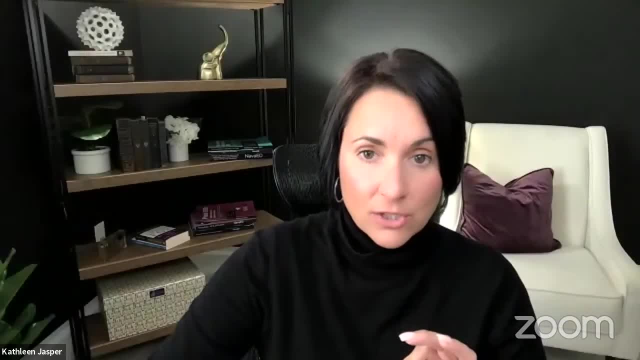 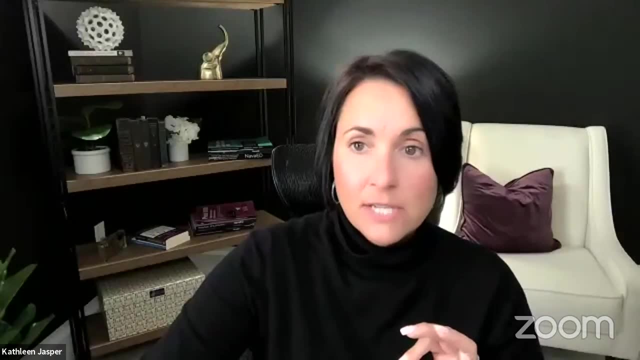 So we are going to now take a look at the structure of the exam, And that's really, really important as we look at, you know, all different types of of test questions and things like that, So let me just go here before we go. 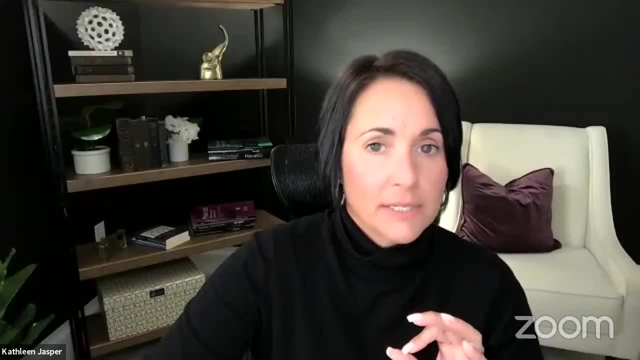 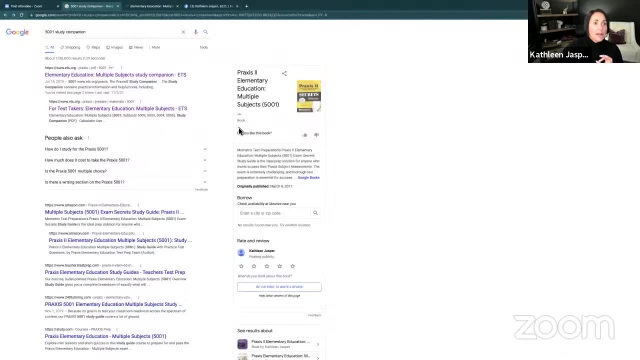 OK, I don't like to share Screen until I have everything ready to roll. OK, so let me go ahead and share screen here. All right, So if you want to find the study companion for this exam, all you have to do is Google five, zero, zero, one study companion. 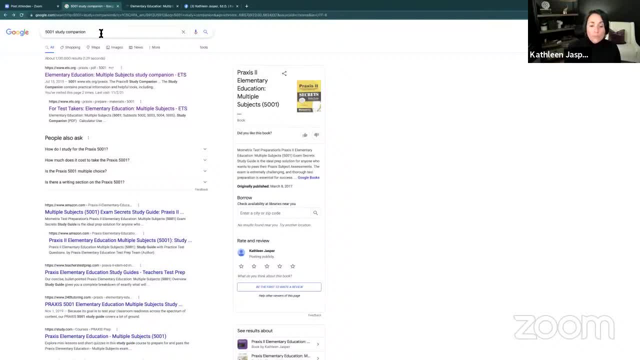 Another good Google term are test specs or blueprint, So those are good terms. So if you're here for another exam and you're, you're getting prepped for whatever you could do. like the Texas EC six blueprint, you could do the Intel Elementary Ed test specifications. 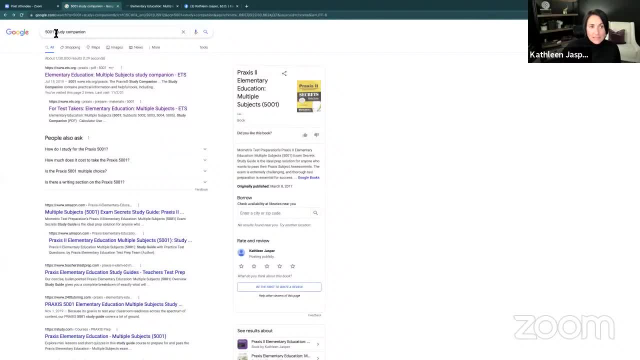 Those are good words to use ETS, which makes- that's the company that makes this exam. They have what they call a study companion. All right, And so you can grab the PDF right away by just going here. I believe this is the PDF. Oh well, it'll take you to the preparation materials. 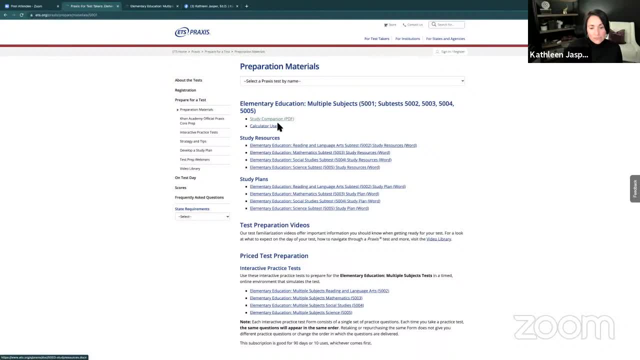 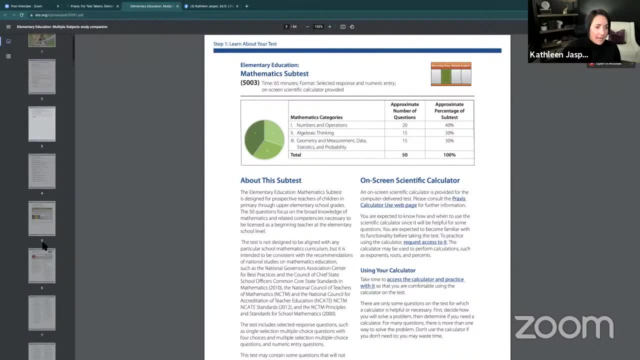 And when you do, you'll see the study companion here. Then they have a bunch of resources. ETS really gives you a lot of free Resources for the exam. I'm going to go straight to the study companion here and you can see- I just showed you this. 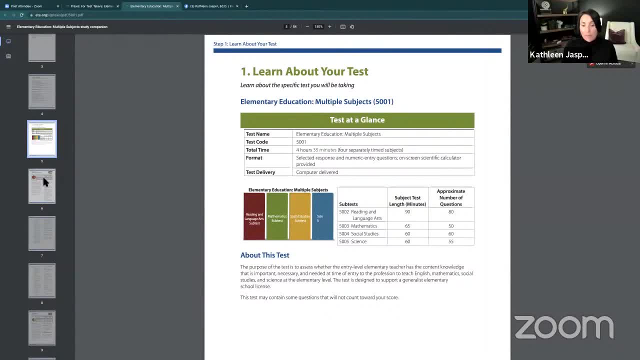 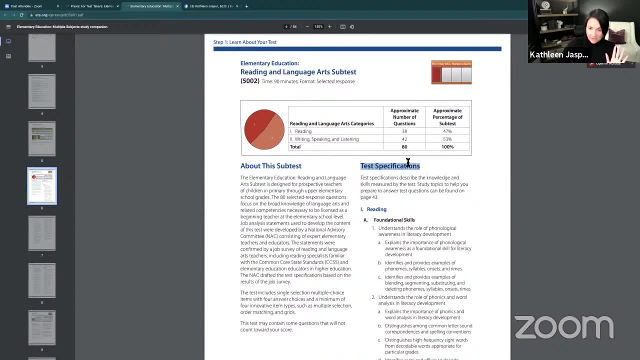 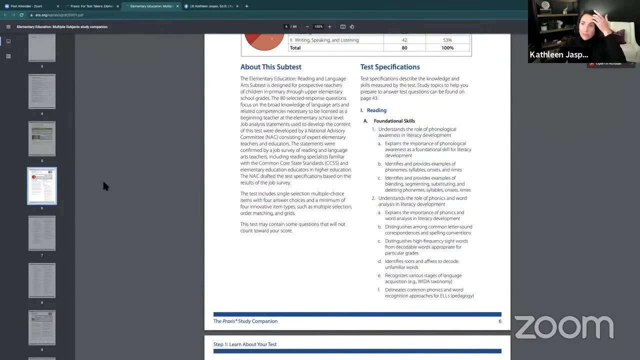 Now what we want to focus on are the skills underneath that, because the specs- or what we call the test specifications or the specifics, Notice how much information there is here. So I am constantly telling people who take my courses in my webinars: you've got to analyze the test specs. 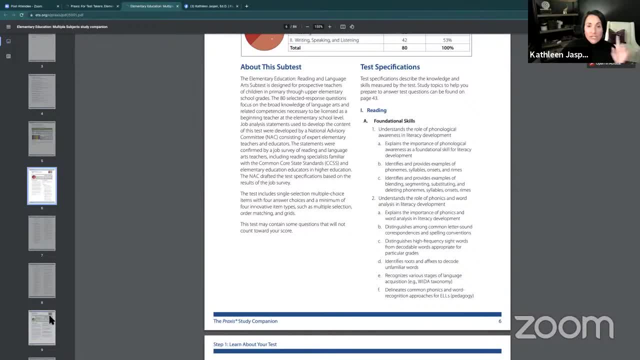 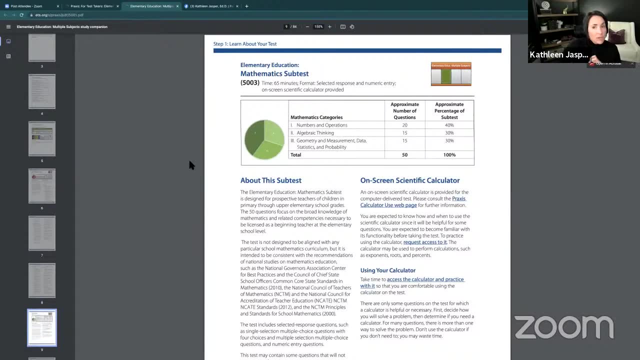 That's where the important information Is. I don't care what study guide you're using, even my own. This is where you should start Now. we always have the test specs outlined in our study guides, but you always want to match your study guides up. 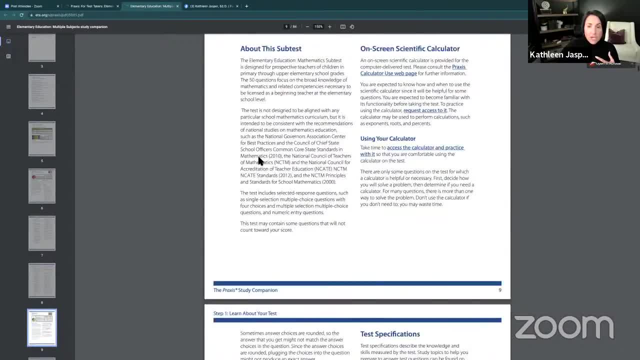 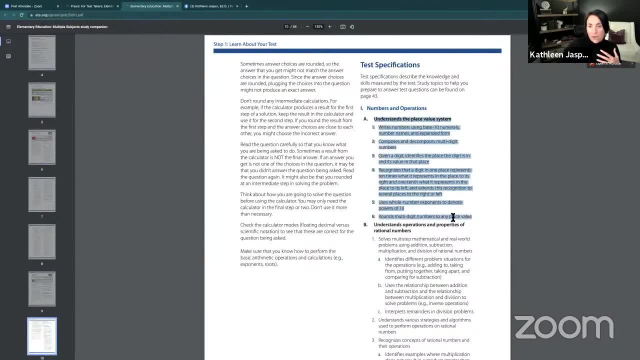 Make sure that they are covering everything in your test specs. So we're going to start with math and you can see that there. this part here is numbers and operations, And this gives you all of the skills for numbers and operations, and then a little bit more rational numbers and all of that. 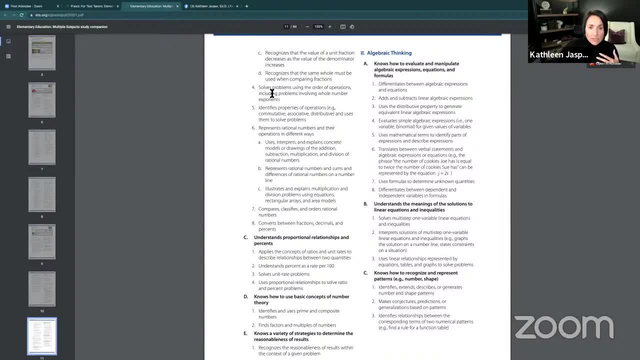 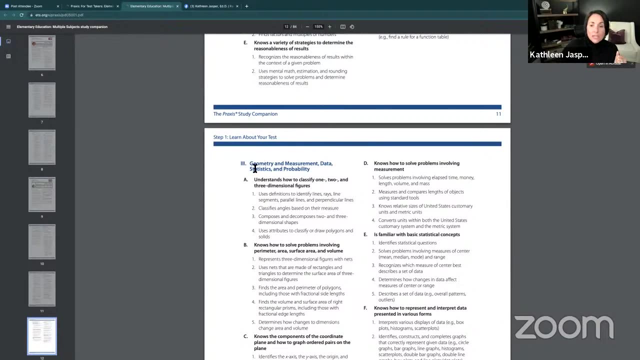 And then we get to look, look how much Of numbers and operations- I mean just a lot of things- going on there. Then we have algebraic thinking and then all of the skills under algebraic thinking, And then the third part is geometry, measurement, data, probability and stats. 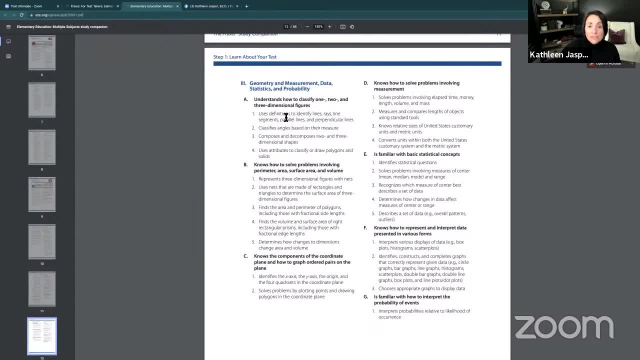 And look at all of that information there. It's very important that you can get go. Yes, I can do this. Yes, I can do this. Yep, Know how to do that. Yes, I know how to do that. If you really want to pass, you want to be able to check off the skills in the test specifications. 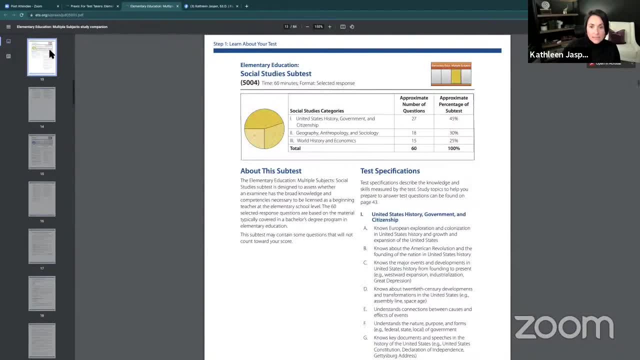 OK, The same thing goes for the social science. We're going to go through that. Notice, there are three categories there. Every social studies exam has US history, government and citizenship. They all have geography and they all have world history and economics. 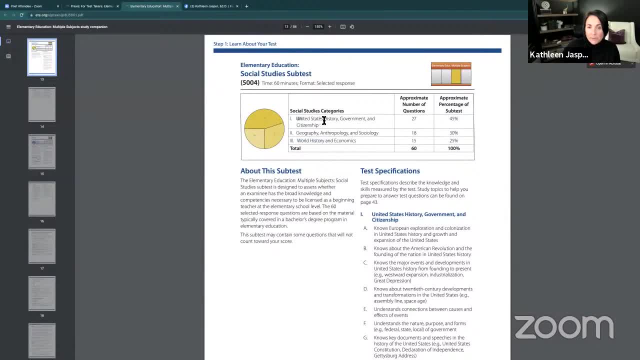 Now, as you get up in the grades, they split these up. So one section will be US history, The next one will be government and citizenship. They might break these up as you go up in the grades, But in elementary they tend to smush them together because you're covering. 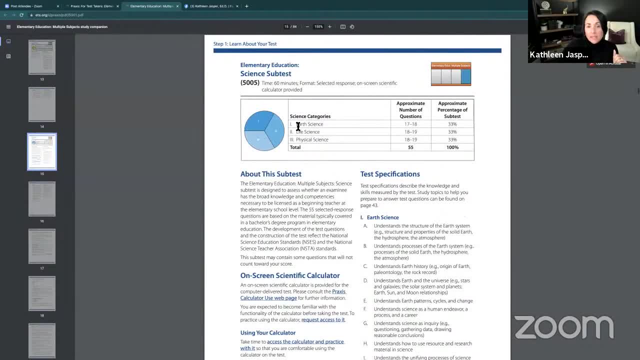 Everything in one grade level. then science. typically, science is made up of these three category: Earth, life, physical. And again I'm going to show you questions that match those. So you know, oh, this is an earth science question, This is a physical science question. 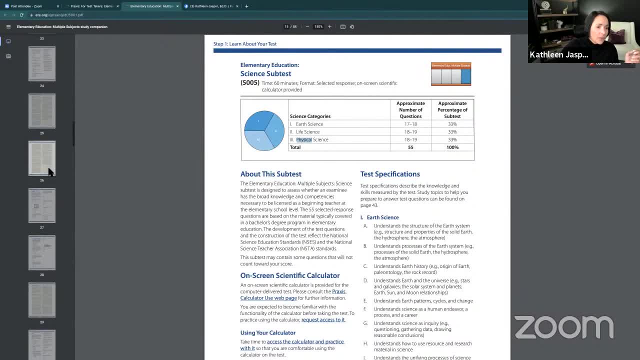 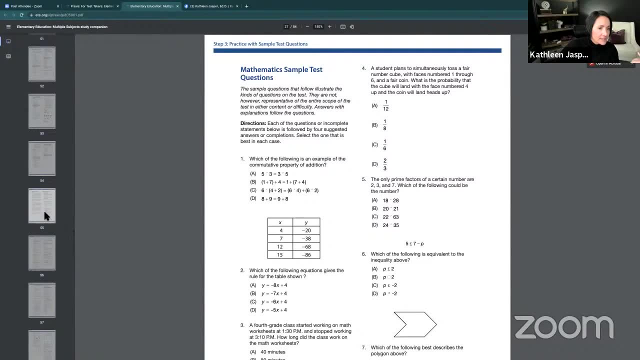 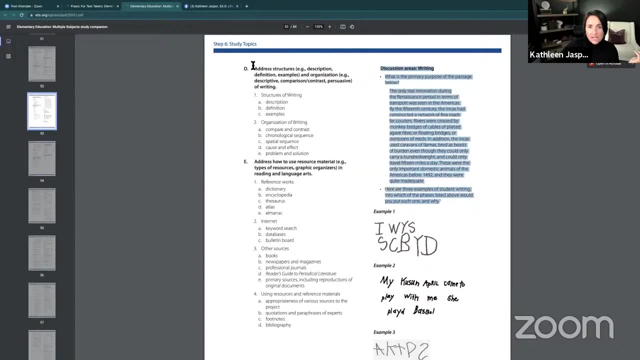 You're going to be able to do that by the end, And then you go all the way through there. Obviously, they have test questions here, But what they also have are what I love, which is they have, You know, different discussion areas here. There's a lot in this study companion. 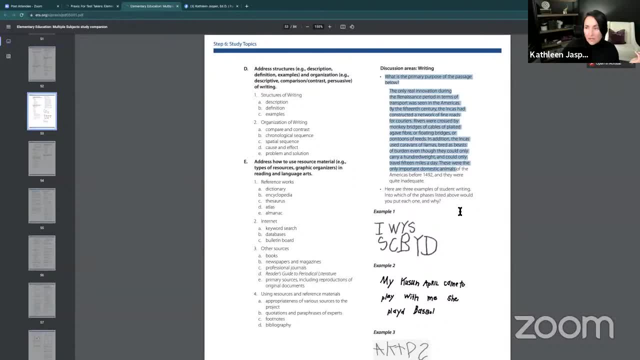 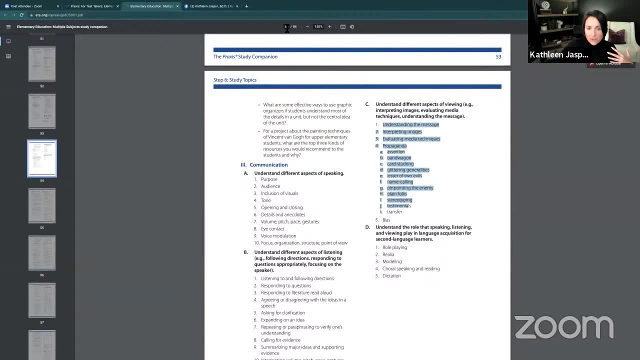 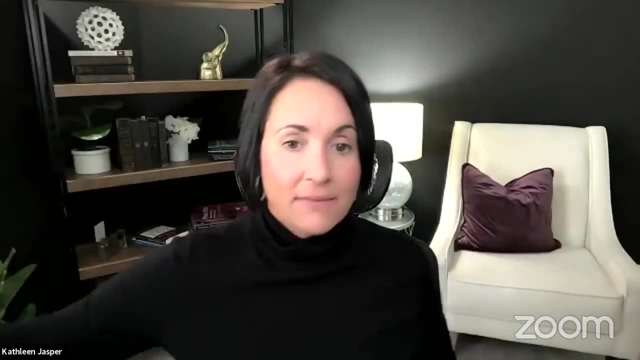 So they have all these discussion questions here and then they have examples and all of these very specific things. Now, this is at the end of the guide, on page 54.. But definitely look through this entire thing. It's really really important. OK, Now, beyond that, obviously I have a big fat study guide: digital courses, all of that. There's YouTube videos for you. I'm going to go through all of that. There's YouTube videos for you. There's YouTube videos for you. I'm going to go through all of that. Obviously, I have a big fat study guide: digital courses, all of that. There's YouTube videos for you. 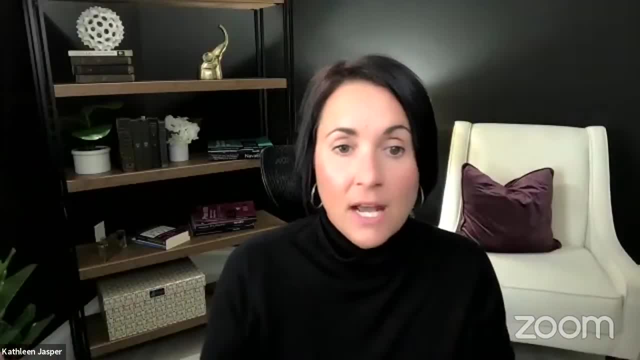 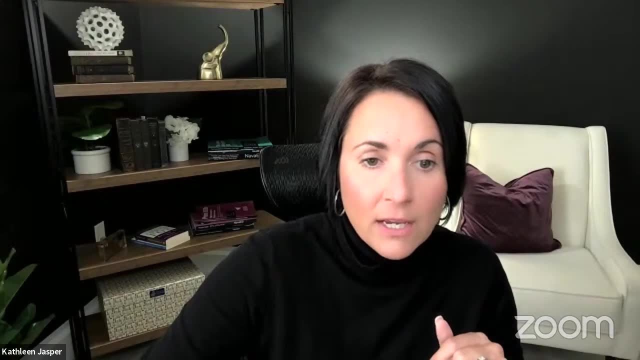 for free all kinds of resources out there from my company and others, but you want to go with the test specs first? Okay, So that was our first objective was to cover the structure. We kind of have an overarching structure now Let me go ahead and let's go to my presentation here. So let's get 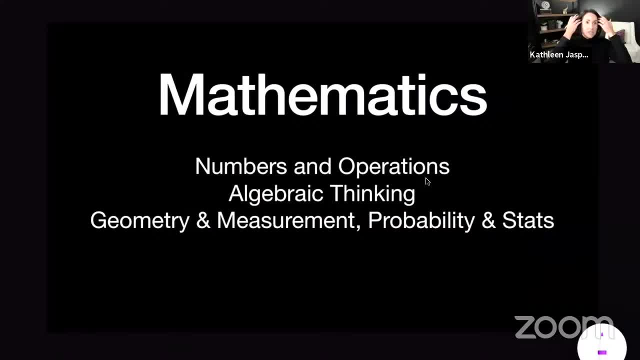 started on some of these test questions. So I said before that we're going to start with math. If you have questions and you're on Zoom, you can throw them in the chat. If you're on Facebook, you can put them on Facebook or YouTube. but I'll try to get to them. but I'm trying to be in three. 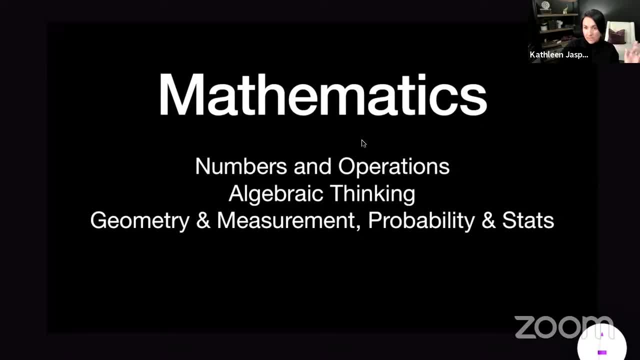 places at once, but I will get to them at some point today. Okay, So we're talking about math and we know that these are the three categories: numbers and operations, algebraic thinking and geometry and stats. All right, So what's really important here is that we kind of figure out what 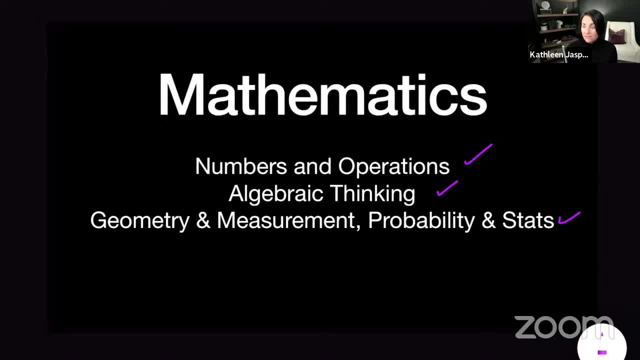 types of questions you're going to see. Now let me tell you, the mathematics on the 5003, which is the subtest on the elementary ed- is not easy. It's really hard. They have slope intercept- We're going to go over today- and they have everything from very basic questions all the way up to very 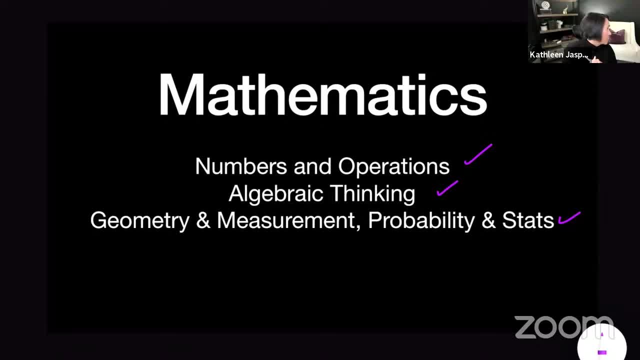 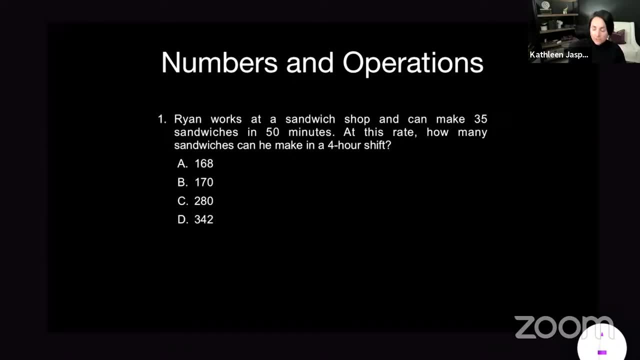 complex questions, because now in elementary school they're doing a lot of complex things. So I'm going to go right here, We're going to get right into it. You can see that this is a numbers and operations question And this also happens to be a proportion question, And I'm 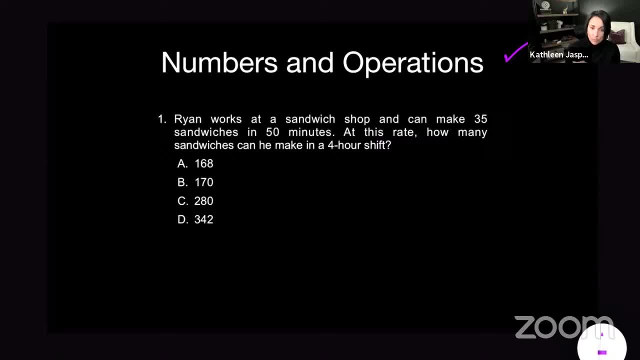 going to show you about that in just a second. So we have a word problem. we want to think like a test maker. We want to look at the answer choices. I always love to start with the answer choices first. It helps me understand what I'm doing here. Here we're. 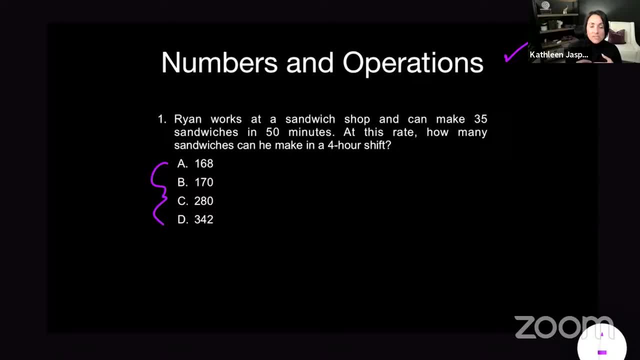 just looking for a number, but if this had like the symbol pie in it or it had like a algebraic equation in it, it would help me understand what's going on. So this is very, very important. Always kind of work backwards, All right. So I have Ryan works at a sandwich shop and can make. 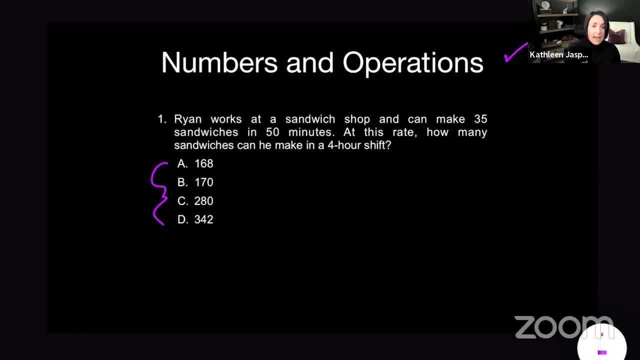 35 sandwiches in 50 minutes. So I have Ryan works at a sandwich shop and can make 35 sandwiches in 50 minutes. So I have Ryan works at a sandwich shop and can make 35 sandwiches in 50 minutes. At this rate, how many sandwiches can he make in a four hour shift? Now a couple of things here. 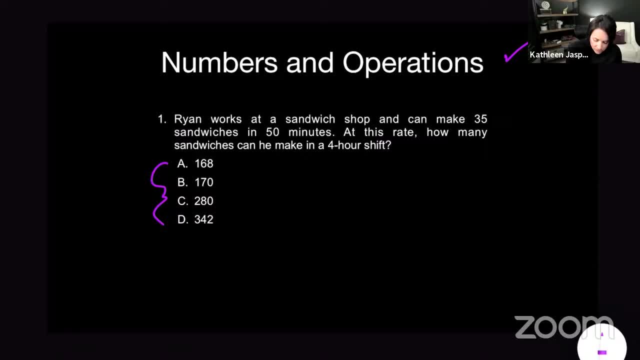 right away it jumps out to me as a proportion, And what we want to do is set two fractions up or two ratios up equally. We're looking for a rate, And the other thing that gives me an idea that this is a proportion is: I have three out of the four things I need. I have 35 sandwiches in. 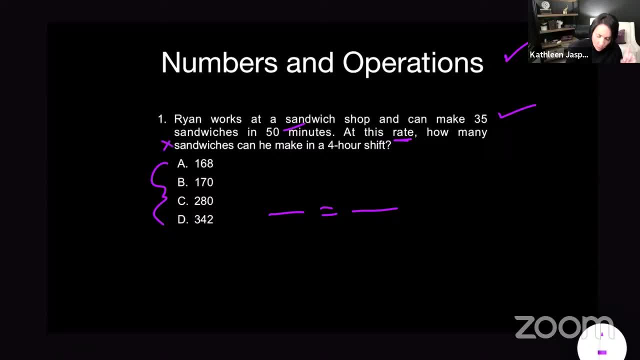 50 minutes. How many sandwiches, which that's a proportion. I have three out of the four things I need. That's the one I don't know Does he make in a four hour shift. So I have sandwiches in time and then I have time, but I need sandwiches because what I really want is sandwiches over. 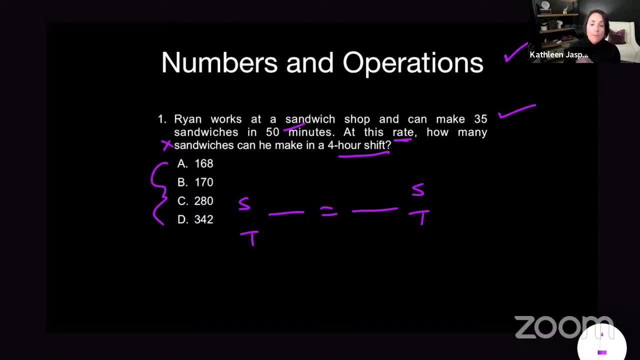 time equals sandwiches over time. Matchy, matchy You could do. time over sandwiches equals time over sandwiches. Either way, whatever you put on the top has to match on both sides. Whenever you put on the bottom has to match on both sides. We like to call this when we do our math section. 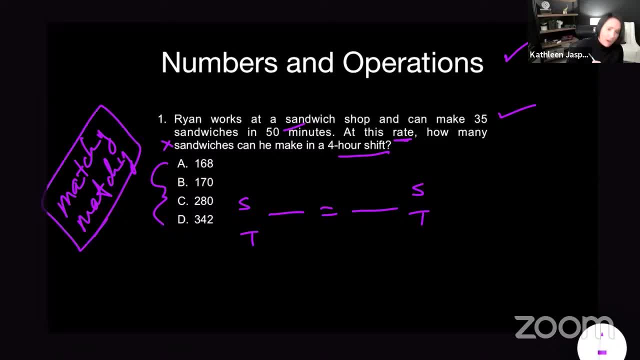 matchy matchy. When you're thinking about proportions, you want to think matchy matchy, All right. So let me just set it up by reading out loud: All right, We have 35 sandwiches in 50 minutes at this rate. How many? when we say how many, that's an X, right. I'm looking for the. 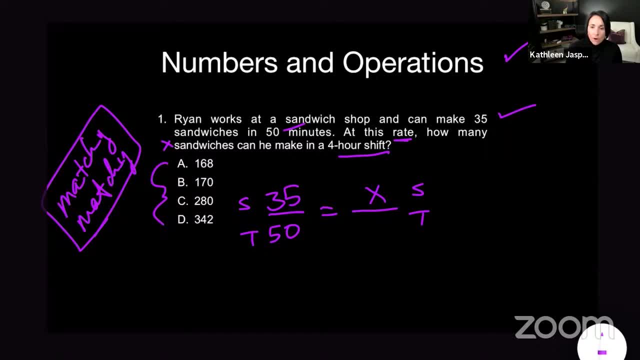 variable: How many sandwiches can he make in four hours? Now they're doing another thing with you with number sense. I have hours And here I have minutes. This is a conversion situation. So you're being tested on a bunch of things: algebra, conversions, proportions. There's a lot going on in this question, All right. So if 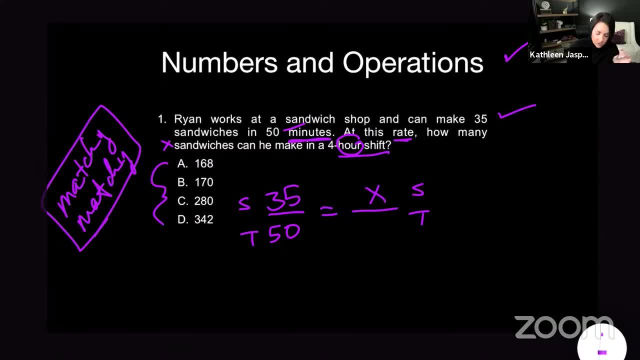 I want to turn four hours into 50 minutes, which is going to be much easier than turning minutes into hours. you could turn the 50 minutes into hours, but that's not a full hour. If that were 60 minutes, we could make that one right, But it's 50 minutes, So it's going to be like point. 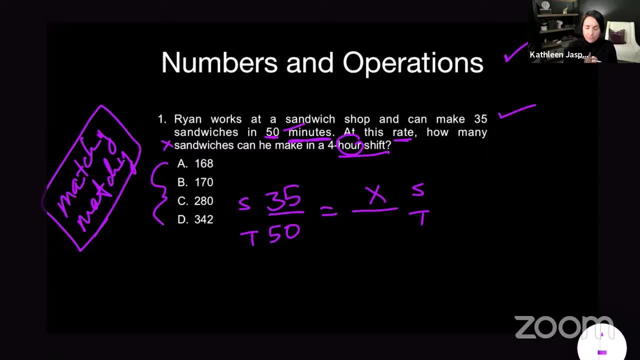 whatever, whatever. So let's take the four hours and turn that into minutes. So what do I do? I take 60 times four. 60 times four, bring down the zero, that's 240.. Now you do get a calculator for this exam. 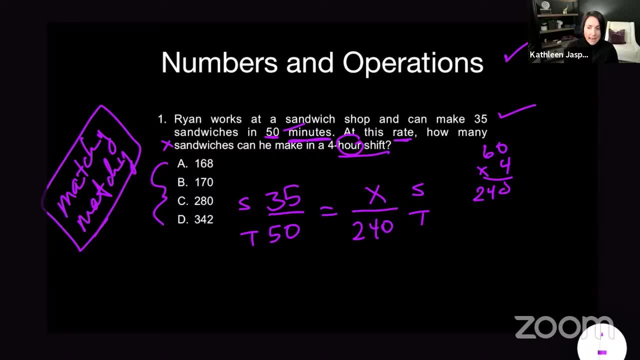 the 5003.. But if you didn't, it's okay. You just got to brush up on your facts. Basically, you want to take six times four, which is 24.. So that's going to get you to zero. You wouldn't have to do that long, long multiplication situation. 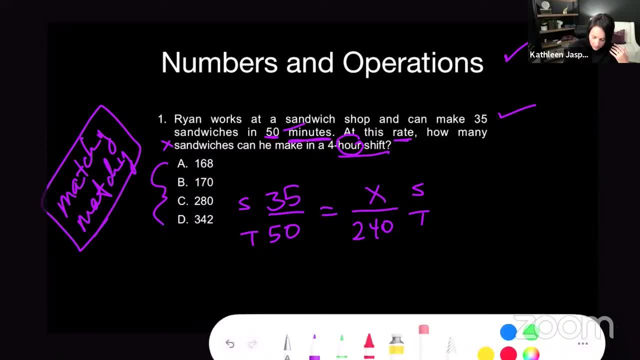 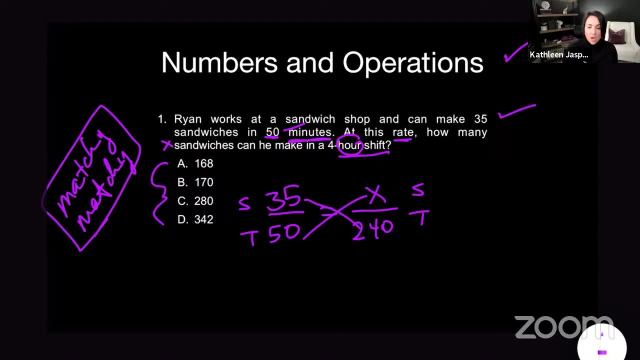 there. I'm just erase that to keep things a little bit cleaner out here. All right, So now what do we do? I've got it matched up: sandwiches over time, equal sandwiches over time. now, because they're equal and it's a, it's a ratio or a proportion- I can cross, multiply and solve. And when I do, 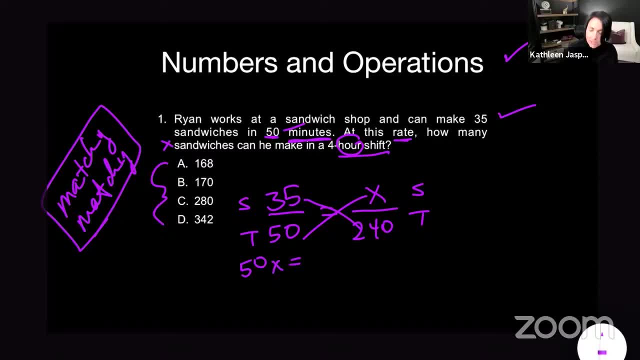 I get 50 X equals and I have my calculator here. I'm allowed to use it If not. but just do 240 over 35 and work it out the long way And I'm not going to do that right this second. 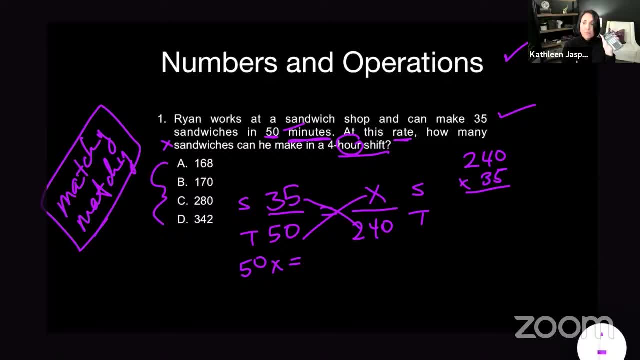 I'm going to just use my calculator for time's sake: 35 and we get 8,, 8,400.. Now, right away, I can see that this is going to divide out evenly, which is what they do on these exams. 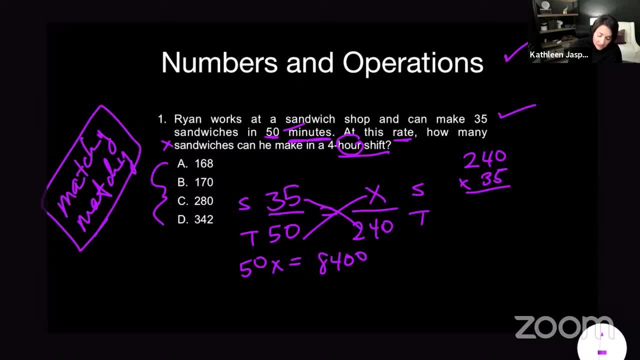 Typically you're not going to have a lot of decimals in the answer choices And you can see my answer choices by looking at my answer choices here. I know this is going to divide evenly, And 50 does divide evenly into 8,, uh, 8,400.. 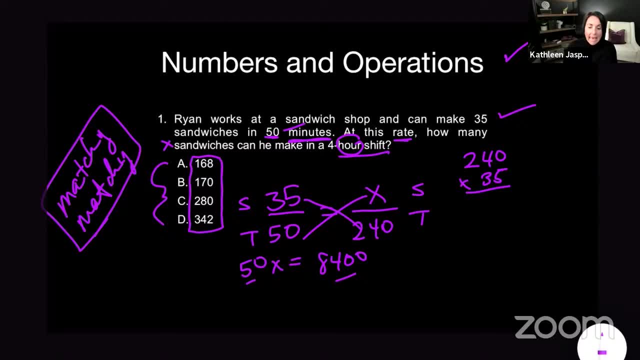 And that kind of leads me in the right direction. If I had like, if it was like 84,, 32, I would know I'm on the wrong track because 50 doesn't go into that And I would, I would need to start over. 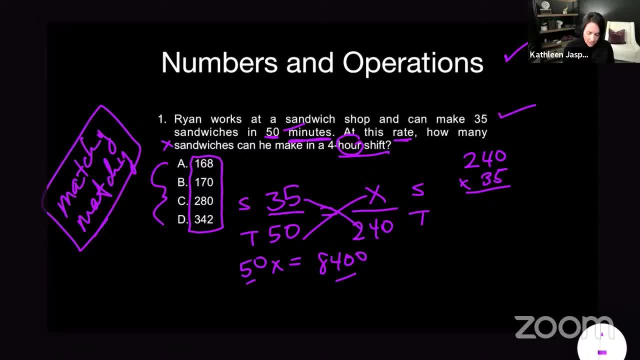 So I always be checking your work, looking at the answer choices for a math exam. So what do I do? I got to isolate the X. I'm looking for X here. So I divide by 50,, divide by 15.. When I do, I get 168. 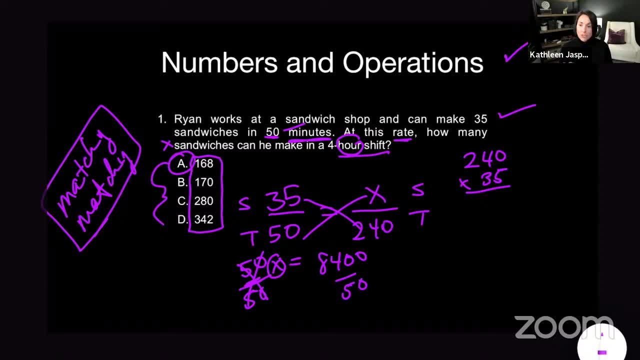 A Is my answer there. All right, So proportion word problems. proportions can help you on many, uh, different parts of the exam. You can use proportions to solve all types of problems. All right, Let's take a look at the next one. 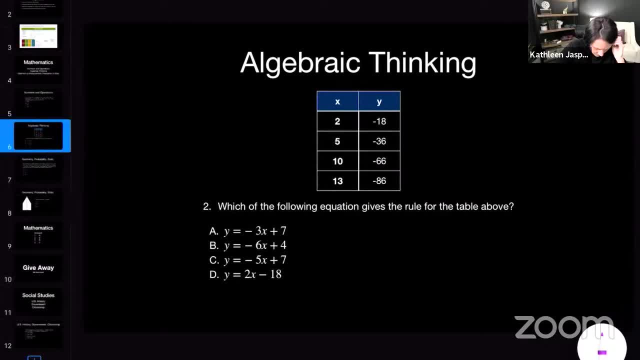 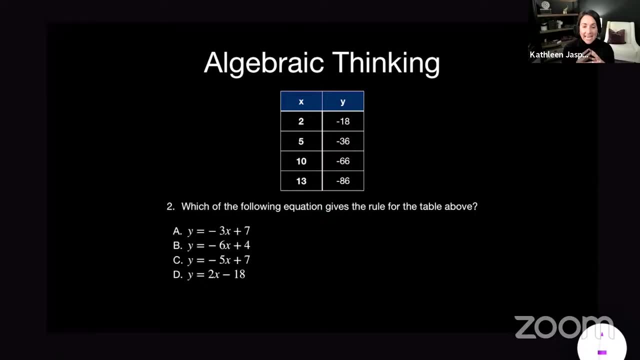 This is what's going on here. How many do I? Okay, good, good, I thought I messed up my PowerPoint again. Okay, So this is algebraic thinking And this is, let me say something here. Okay, I got it. 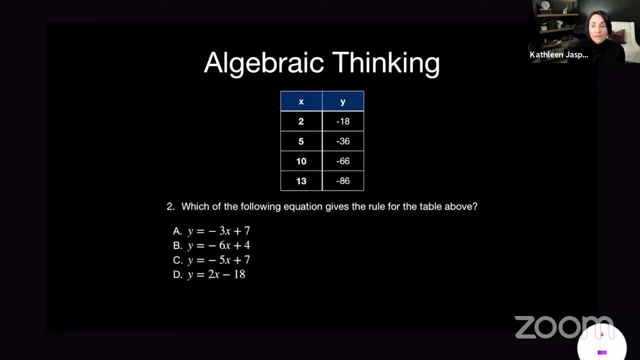 Sorry, Sorry about that. I was wondering what was going on. So we have algebraic thinking here And this. when I work backwards and look at my answer choices here, I can see that I'm working with slope, which is what. 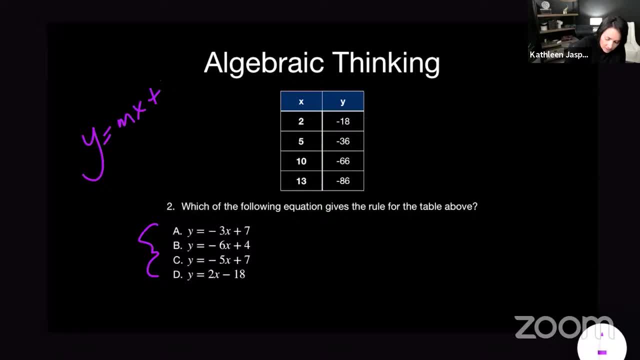 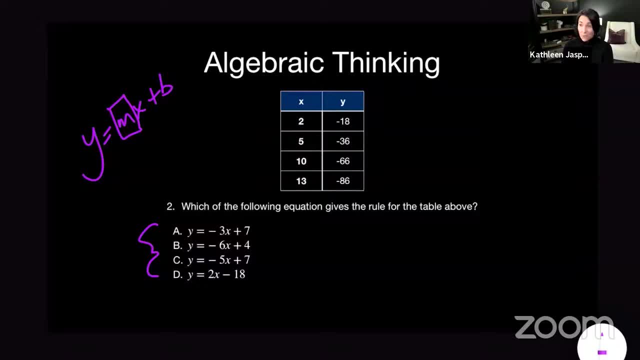 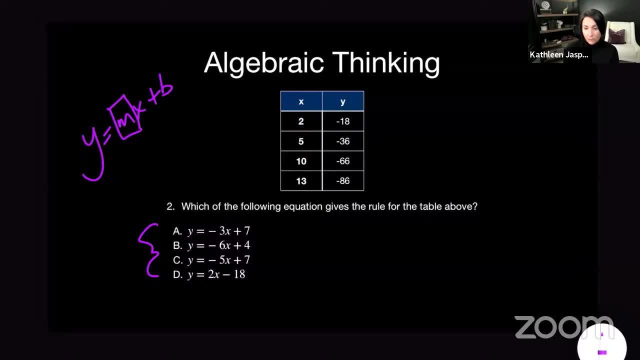 So this is hard. Now you might get a table like this. You might get in different ways, But right away, because I'm looking at the answer choices, I know that I'm looking for the change in Y over the change in X because I can see that I have different slopes in. 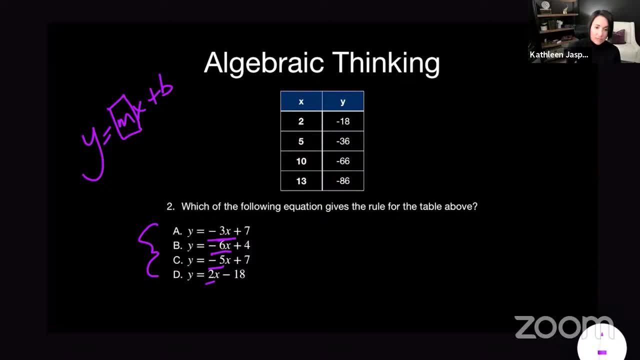 all the answer choices there. Do you see that I have negative three, negative six, negative five and positive, And so all I have to focus on is this: M right here, And I know that M is the change in Y over the change in X. 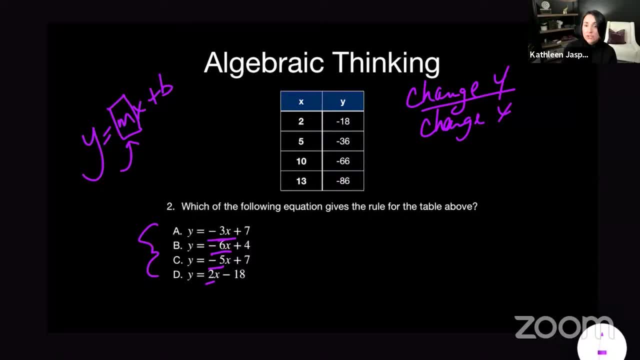 Okay, So there are a couple of ways to do this And the easiest way that my husband, who teaches math for us on Tuesday nights from five to 6 pm. What he would say is to his students is: find two places in this table, stack them and subtract. 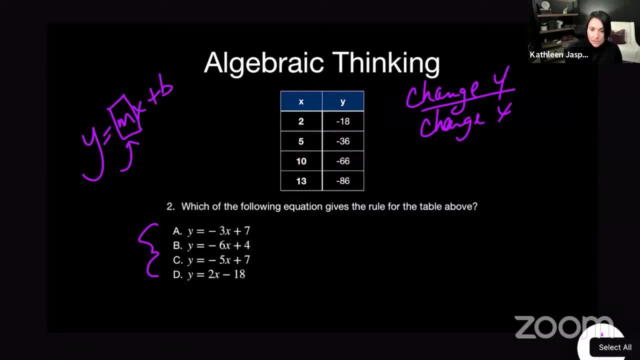 them to find your, your slope, Okay, So I'm going to take these two areas here. You could take any of them, but we're just going to take those two because they're the easiest. They have the kind of the smaller numbers. 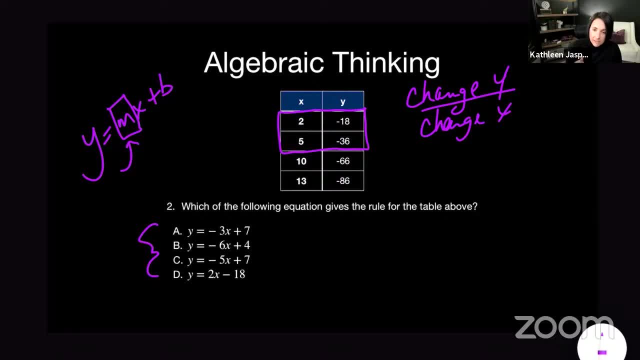 They're going to be easier to do here. All right Now. typically, if we were to do this- we're going to do this Typically. if we were to do this, we're going to do this. If we were going to do this by the book, we would do Y2 minus Y1 over X2 minus X1.. 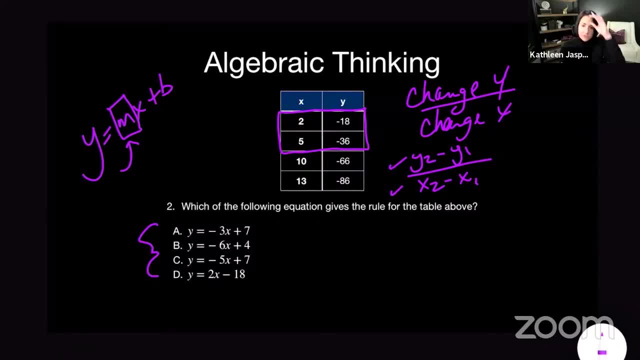 Notice change in Y over change in X. The change is subtraction, right. You could also do Y1 minus Y2 over, sorry, X1.. Sorry, I'm Y1 minus Y2 over X2.. I'm sorry, Gosh. come on, Kathleen. 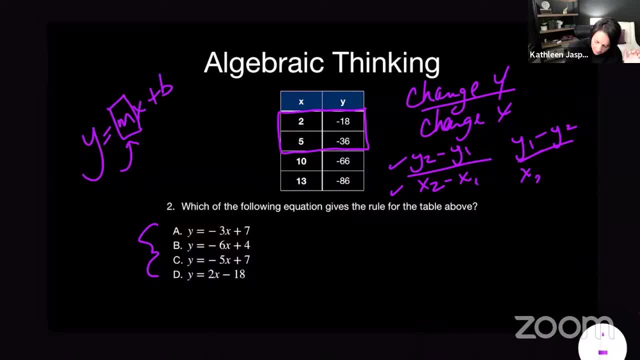 I'm Y1 minus X2.. It doesn't matter, This is like the proper equation, but just like with the proportions, if you, they just have to be the same. So this has to be X1, X2, Y1, Y2, or Y2 minus Y1 over X2 minus X1. 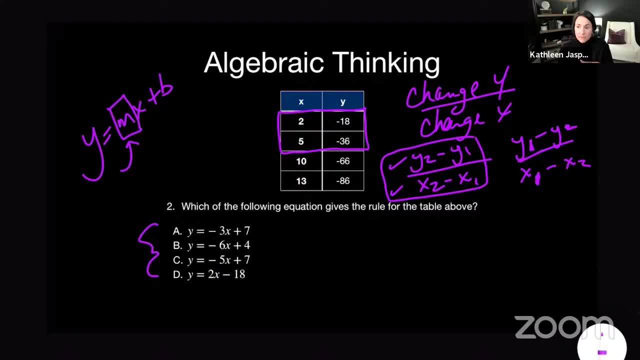 If you were to work these out using both of these formulas, as long as you kept it matchy matchy, you would get the same answer. Okay, So that too is kind of a mess. Sorry, Let me fix that for you. 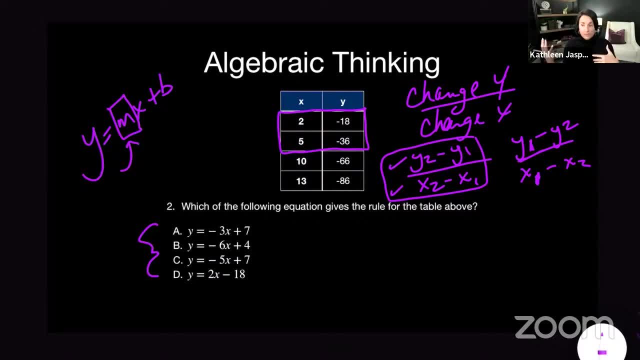 So there's no confusion. Now we could do that, and I'm going to show you both ways so that you can see. All right, So let's go with the traditional way. We have our Y and we have our X, So I'm going to do it with the traditional way first, and then I'm going to show you. 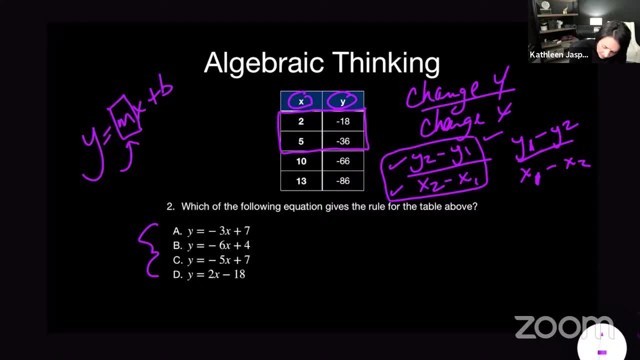 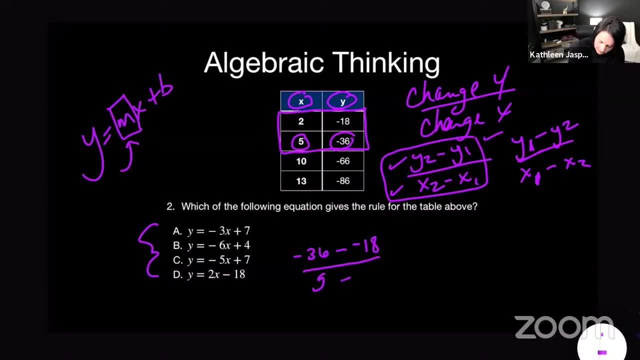 Be careful: five minus two. my fives are looking weird today, I don't know why. Sorry guys, Let me fix that five for you. Okay, Let me just check, because it gets crazy with the Y2, Y1.. So Y2 is negative 36 minus a negative 18 minus Y1 over X2, which is five. 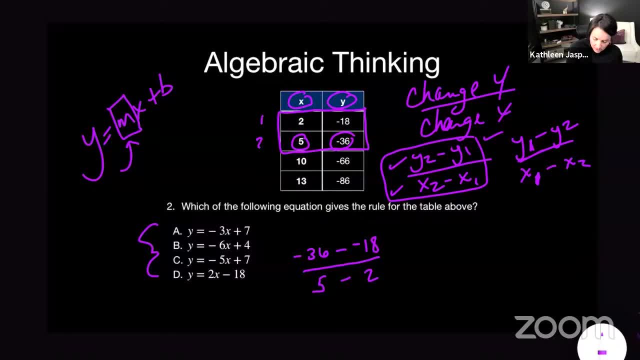 Notice: this is: this is a row one and this is row two. All right, Now you may want to use your calculator when you're doing this, because when you have negatives minus a negative, it can get jumbled up in your head. 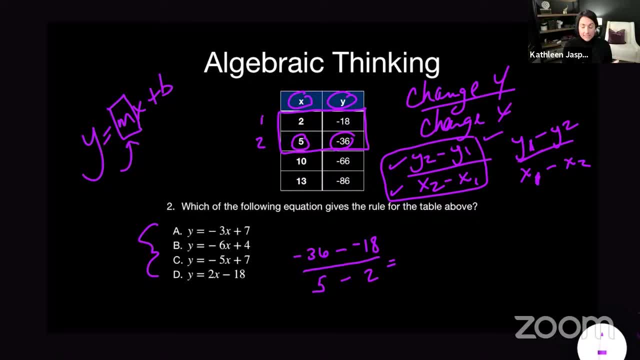 So let's just do that We have now the test is going to be a scientific calculator and you're going to want to put the number first, So we're going to go 36, then hit the negative sign- negative minus 18, then hit the negative. 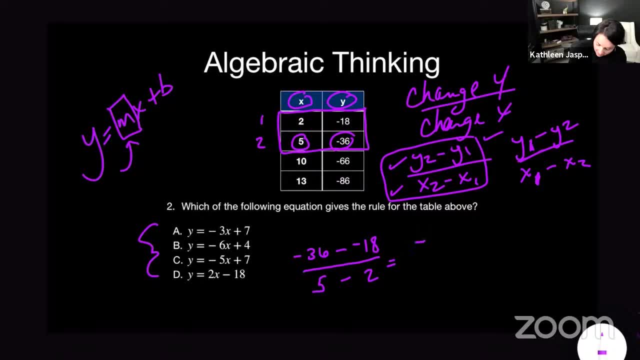 sign And I get negative 18.. You could also do this, which is the shortcut: negative 36 minus a negative 18.. That becomes plus a positive, and 18 plus 18 equals 36.. But we have the negative here, and the negative is with the higher number. 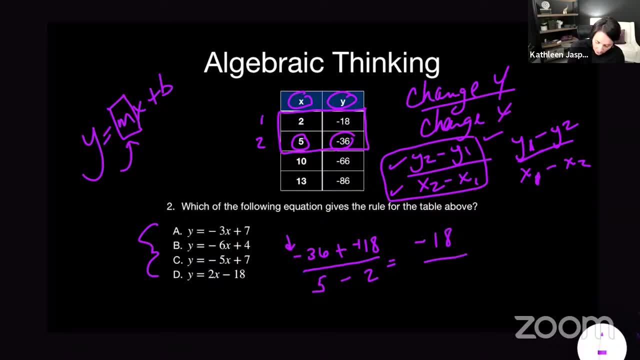 So it's going to be negative 18, but however, you want to do it And then you put that over five minus two, which is three, And then when we do that, we get three goes into negative 18.. That becomes negative. 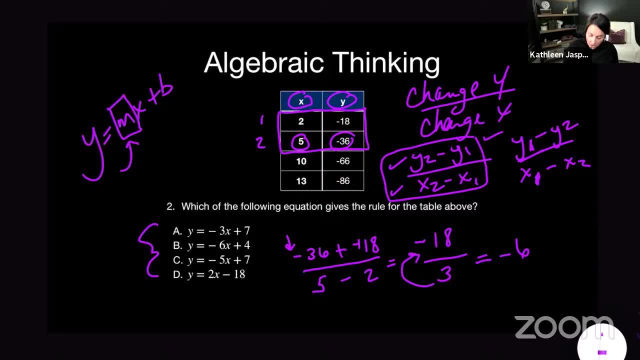 Six. Now let's take a look. This is our slope. When you put the change in Y over the change in X, that equals slope. Well, where is slope in the equation? This is going to help you. Slope in the equation is M right here? 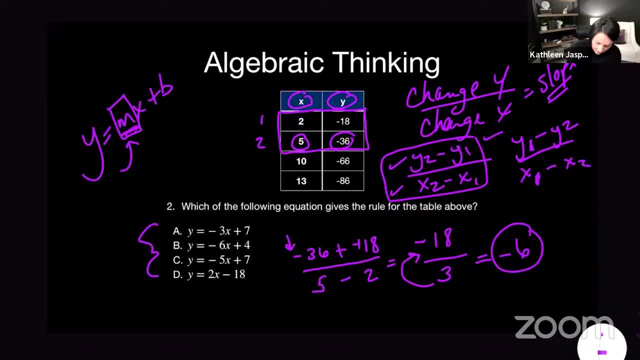 So I just need to figure out where is my negative six here? Well, here it is right here. Now, if we had another answer choice that was like negative six, X plus two, let's just pretend, And they probably will not do this to you. 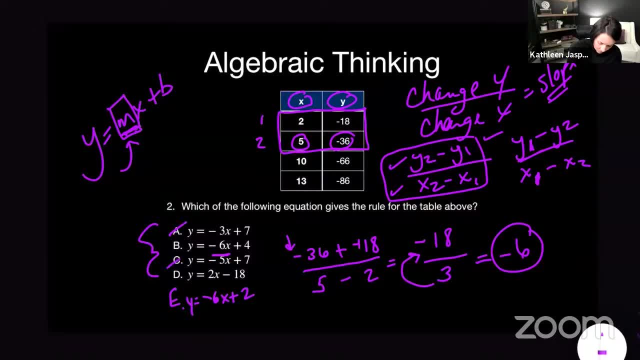 I have two negative sixes here, And so I go: oh, I got to figure out the Y intercept, which is what this is. B is the Y intercept, But on this test they don't. they don't assess that. 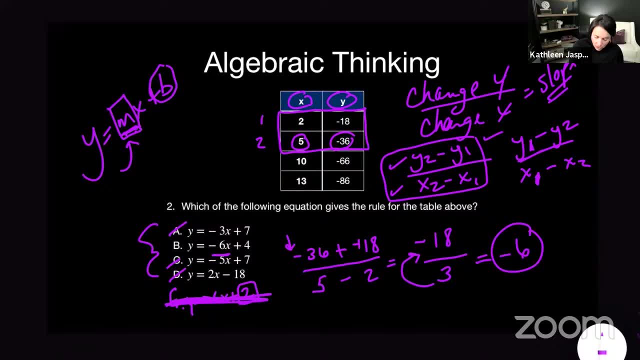 So you won't have that, You won't have that here, And so right away I can grab B and move on. Now let me show you a quick shortcut, because I know Jeremy would be like showing my shortcut, because it's so much easier. 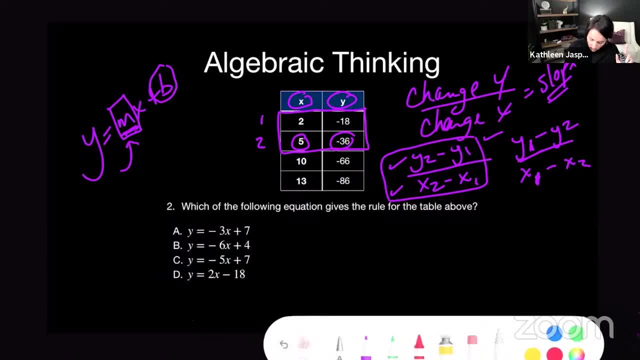 So let's just erase all this to clean it up, All right. So let's say: I don't want to mess with Y2 minus Y1, all of that. Let me erase this too, please. Let me just- And I'm on test day and I need to figure out slope quickly, because I got to keep it moving. 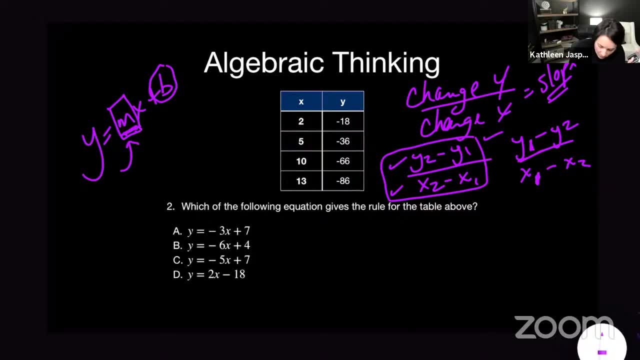 I only have so much time on this test. What you can do is take two points on this table, which is really two points on a line, And you're going to want to stack them and subtract them. So here's what I'm going to do. 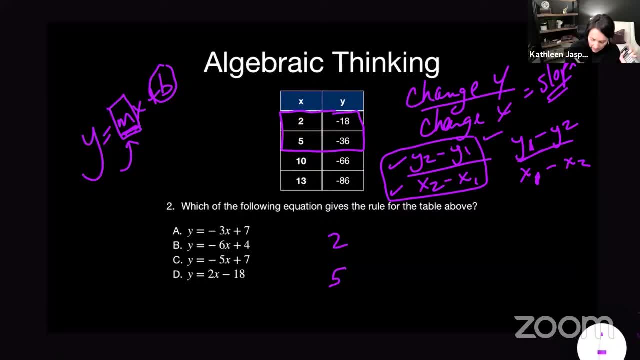 I'm going to go: These are my X's, I'm going to stack my X's And then I'm going to stack my Y's, But I'm going to subtract them. OK, so if I have two minus five, I get negative three. 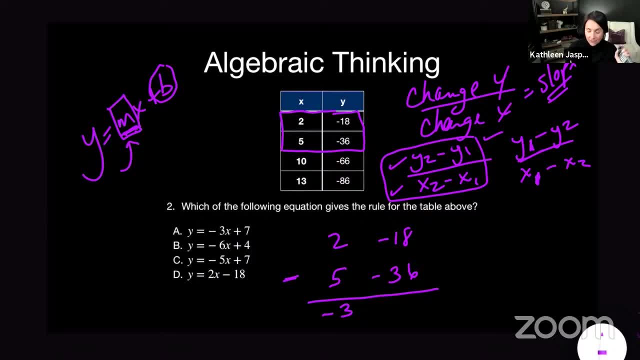 And if I have negative 18 minus a negative 36, let's put it in our calculator: It's actually flipped from the other thing. So we have 18 negative minus 36 negative, I get A positive 18.. Now it's the change in Y. 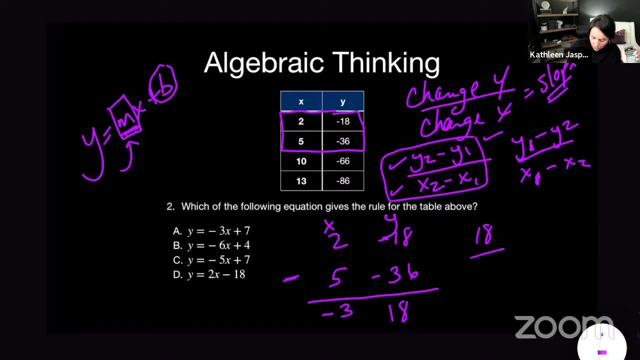 This is Y over X. Put 18 over negative three And we still again get negative six. So B is our answer again. So there are two ways to do it. You can go with the traditional or you can go with stack them and subtract them. 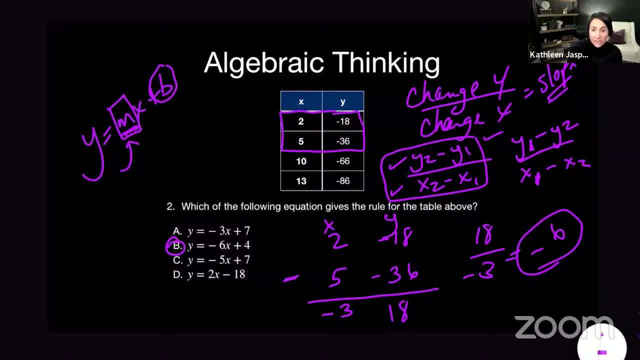 But when you stack them, remember they are going to put these negative numbers in here because they want you to remember it's minus a negative And that will throw you off. It's really difficult But that is sloping Intercept. We do cover that in our book. 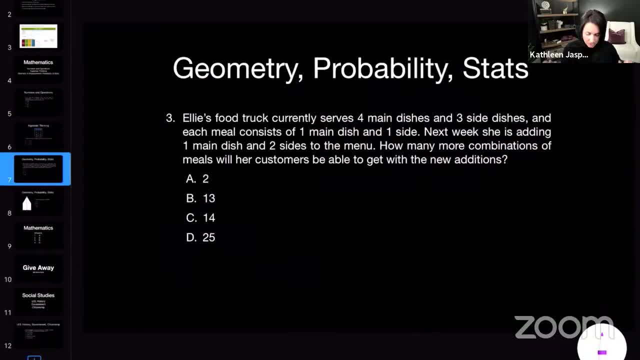 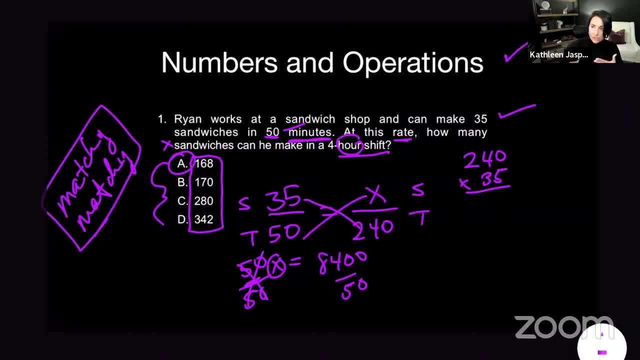 I cannot believe kids are doing slope at this age. It's insanity to me. but it's just the way. it is All right. So we just went through. So this is what a problem would look like in numbers and operations- That first part of the test, right. 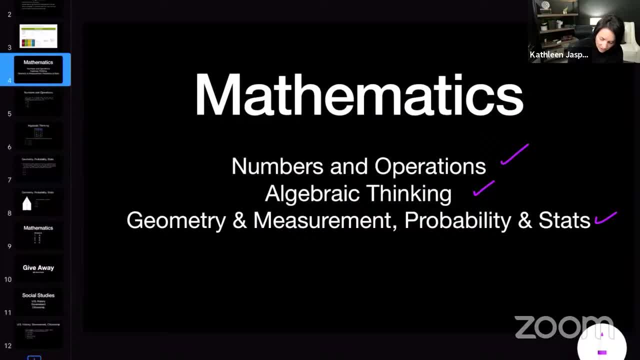 Because we have numbers and operations Check. We did our proportion. Algebraic thinking: We did slope, which is one of the harder skills of algebraic thinking. Now we're going to go to geometry, measurement, probability and stats. This one's kind of a big one. 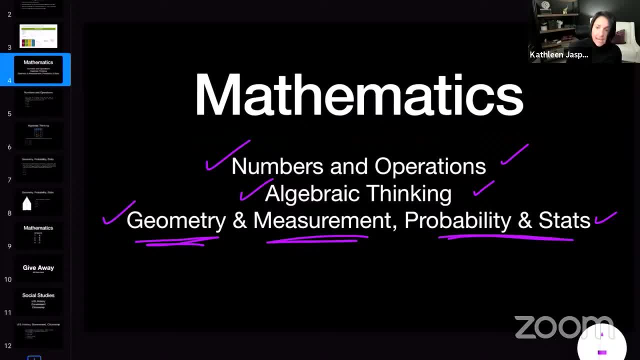 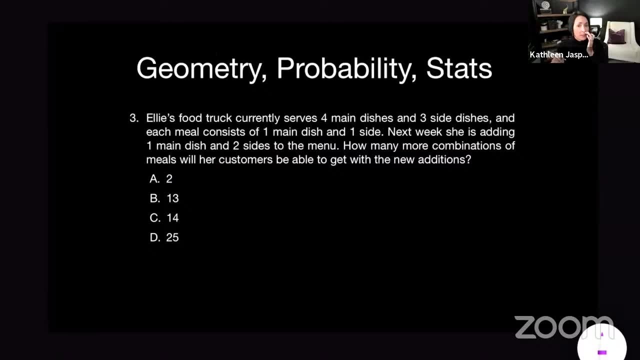 Because you not only have geometry and measurement, but you have probability and stats. So I have two questions for this. OK, So this let's go here. This is more of a probability and stats question. This is when you see something like this: 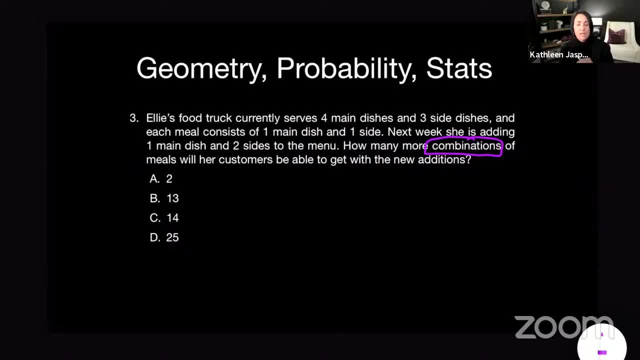 Combinations. When you see combinations, a lot of people get freaked out And they try to do it by hand, And they try to work out the combinations. All you have to do is use multiplication, All right. So let's take a look at this. 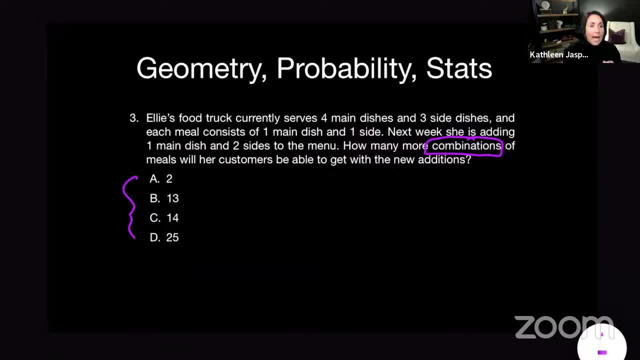 I can see my answer. choices here are just regular old numbers And we're looking at this. We're looking at now. we want to look at the question stem, which I always like to work backwards again, And here's my question: stem, And I can see combinations here. 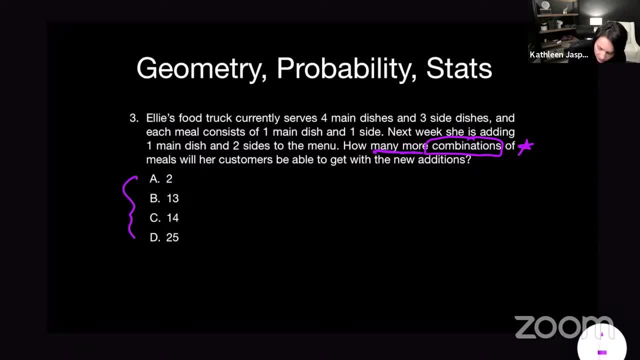 All right. So how many more combinations- looks like a subtraction of meals- will her customers be able to get with the new additions? All right, Let's start now at the top. Ellie's food truck currently serves four main dishes and three side dishes. 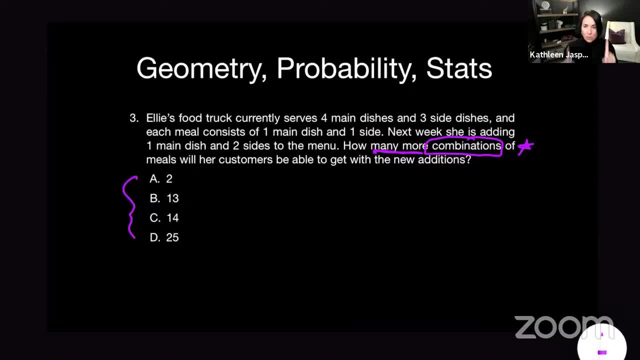 And each meal consists of one main dish and one side, So you get one of each. Next, Next week, she's adding one main dish and two sides to the menu. How many more combinations of meals will her customers be able to get with the new additions? 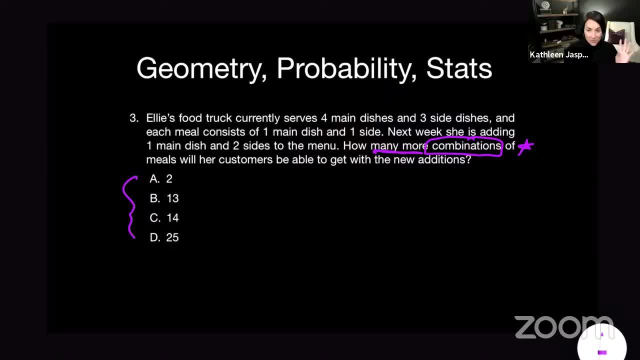 Again, elementary school Crazy word problem, But you will see this on the exam. I went for the hard ones for this webinar. You know, you guys know some of the easy stuff. This is kind of hard. So let's figure out how many current combinations we have. 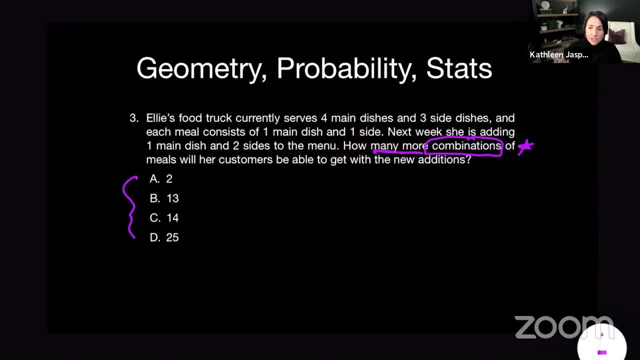 Well, let me wait until the end for that, because I'm going to show you a trap. First, let's figure out: we have Add one main dish, So this is actually going to become four plus one and two sides. This is actually going to become three plus two. 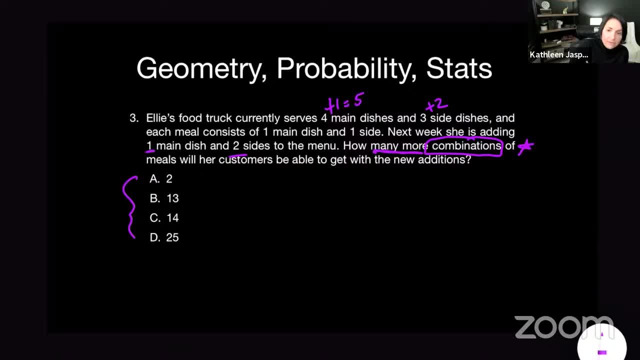 Right. And when I do that, this becomes five and this becomes five, All right. Now how many combinations will they get with the new additions? Well, when you do that, you just multiply the two things, So it's five times five is twenty five. 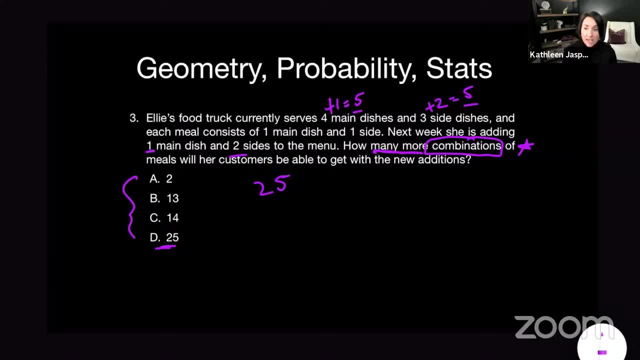 Notice there's D Here. twenty five. A good math exam will anticipate your mistakes. We're not done yet. They'll get twenty five combinations with the new menu. But it's asking: how many more combinations do they get with the new menu from the current or original menu? 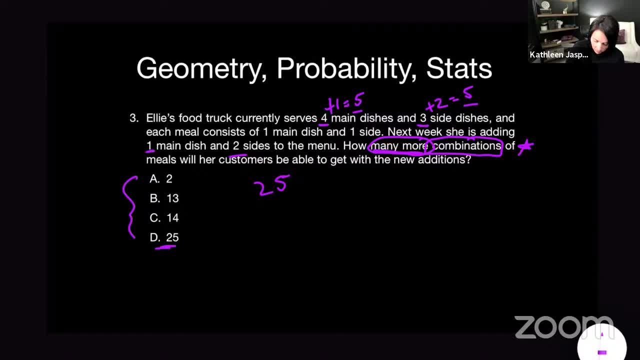 Well, what's the original? The original is four times three, So I have to subtract: four times three is twelve. I have to subtract twelve from twenty five to determine how many more they're going to get Right. So when I do that, I get thirteen. 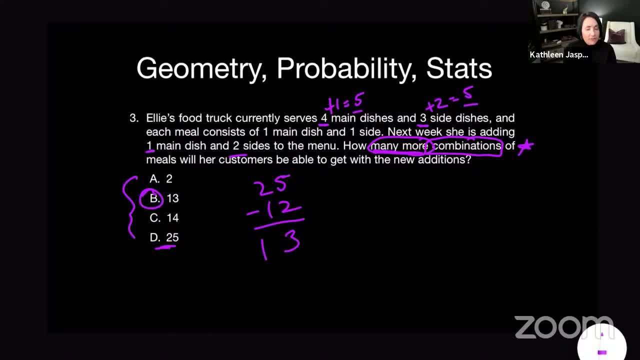 And that is the answer there. So be very careful that you read your question stem. Usually the last sentence in a word problem is telling you what they want you to do, And so you want to make sure you're clear here. If you just went off of oh, she's adding a main dish and a side, or two sides, I'm sorry, you would have said twenty five. 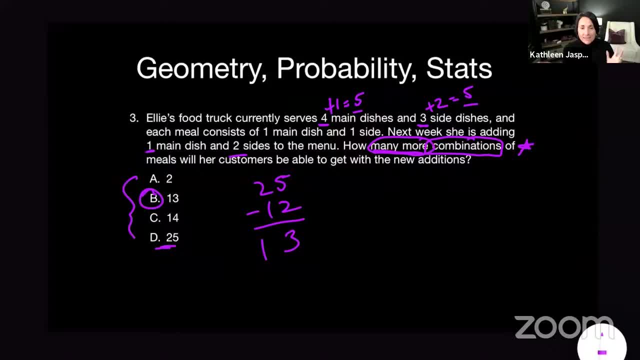 And that would have been incorrect. So be careful. They do that a lot. Now let's say it's another type of problem. Let's say it says Susie has three shirts, two pants, five pairs of socks and two belts. 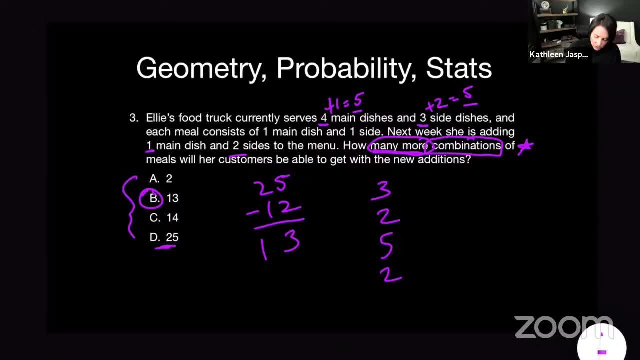 How many different combinations of outfits if she has to choose one of each every day? How many different combinations? All you have to do is multiply three times two times five times two. That's how you do the combinations. This one. there's only two variables. 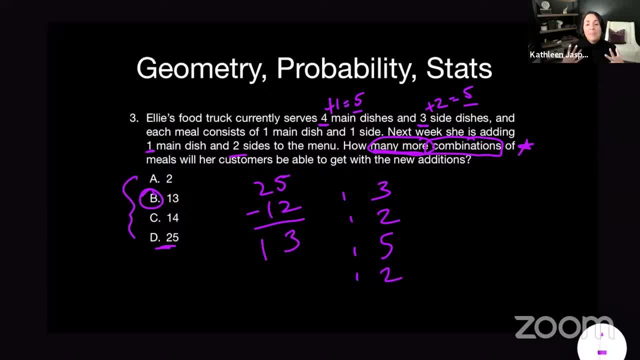 So two things. I guess there's probably a better way of saying that, but there are only two things. We have the four and the three And then, when we add the dishes and the and the sides, we have five and five. But you could get one where it's like outfits or it's like I don't know other things that they combine. 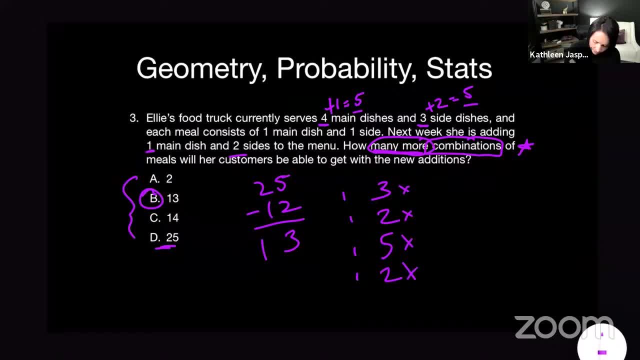 And all you have to do is just multiply all of the numbers and that will get you the total combinations. All right, So let me just erase that, so we're clear. All right, I'm also going to, if you signed up through Zoom. 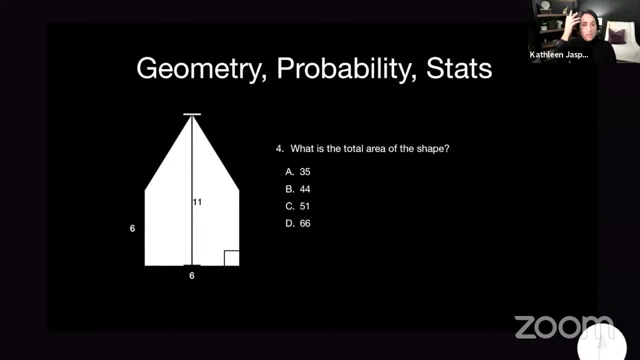 Zoom, I will send you this PowerPoint. if you click the link and all of that, I will send you this PowerPoint. OK, so let's go with geometry, probability and stats here, And so we are talking about this. looks like a geometry problem, right? 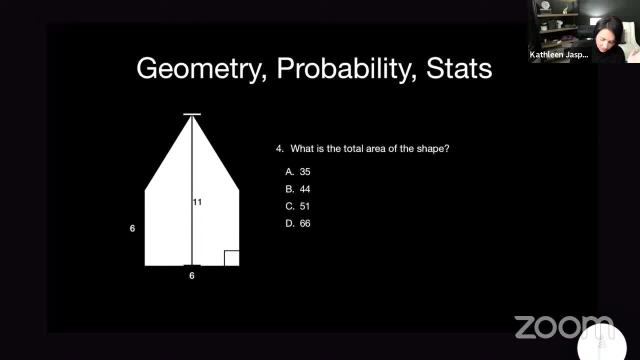 We've got some shape and we have, you know, things going on here and we have a shape, and then we have measures, right, This measurement, geometry, that type of thing. So what is the total Area? area of the shape. 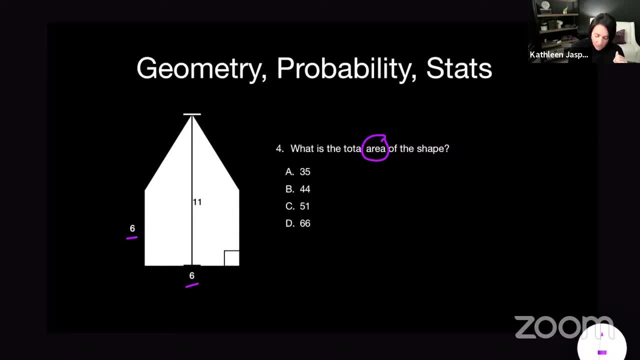 So we essentially have two shapes here and they will ask you to do this. This is adapted from the study companion. There's a similar one on the study companion. So we essentially have two shapes here. So I want to kind of draw a line there. 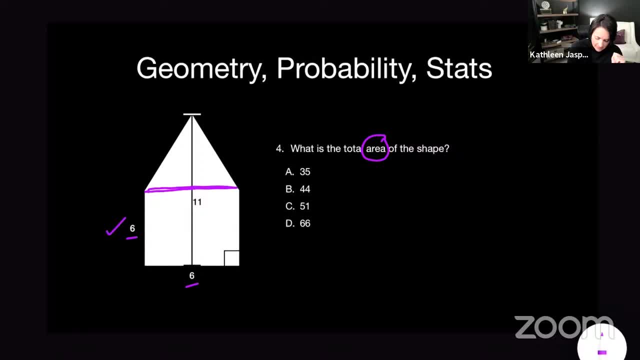 And I know if this is six and this is six, this bottom half is a square, So the bottom half area is thirty six. six times six equals thirty six. What they're really testing you Here is area, of course, but they're also testing you area of a triangle. 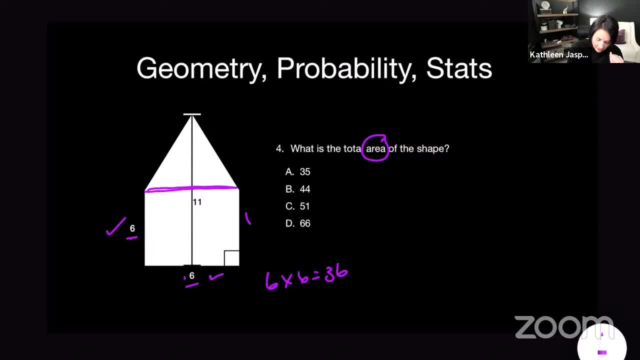 All right. So if these two are six, this is also six, And that means that from here to here is also six, But they gave us eleven, which means that from here to here is five. All right, And so, and of course, we want to pay attention to this right angle. if they have that right angle there, this is definitely a square which helps us fill in some missing. 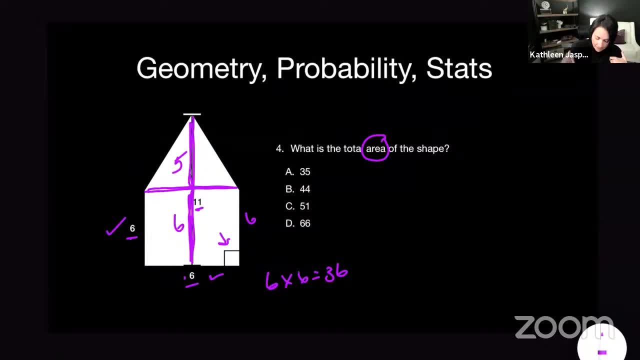 blanks here, And so we have five as our height of this top triangle here. All right, So what is area of a triangle? It's one half base times height, Right, Well, what is base times height? Well, if this is six- and this is a right angle here- then this base is also six. 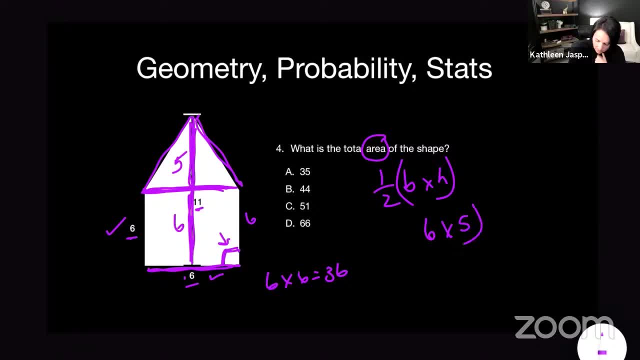 So I have six times What's the height? Five, One half times six times five is one half times thirty, or thirty divided by two, which equals fifteen. I'm not done yet. I need to multiply or not multiply. add fifteen to thirty six. 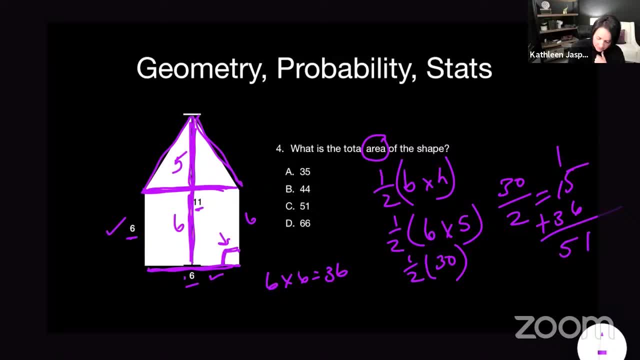 And I get one. one fifty one C is the correct answer there. All right, So a few things going on here. First of all, definitely geometry, working on your area. How do I find area base times height? But then it's the area of a triangle which is one half base times height. 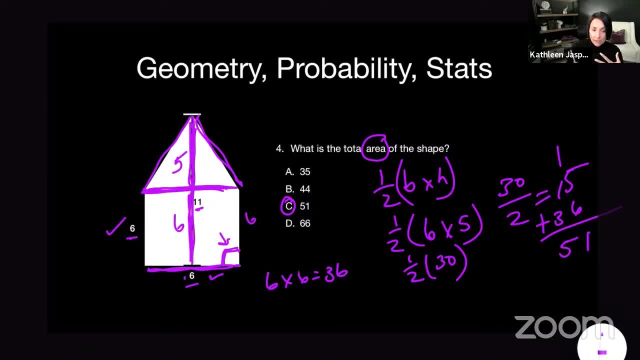 Also, they're kind of working your logic brain here by only giving you a piece of the puzzle and you have to fill it in based on what you know about shapes. So you know a square has all equal sides, And so that's going to help you fill in some of the some of the blanks here. 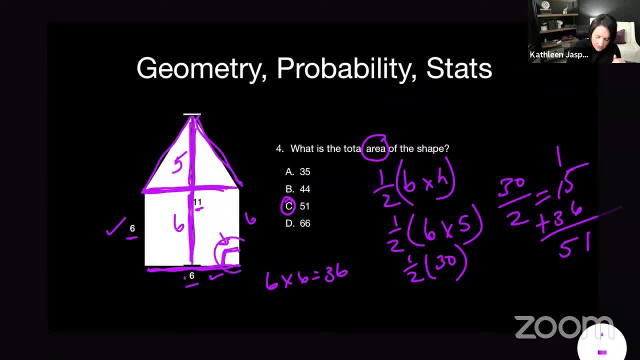 Also a 90 degree angle right here in this area is going to help you figure things out. So it's a lot of different skills kind of going in one area. All right. So I believe that is the end of mathematics. So now we are going to do a giveaway. 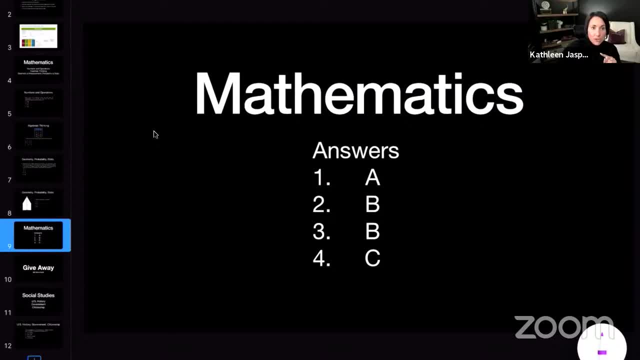 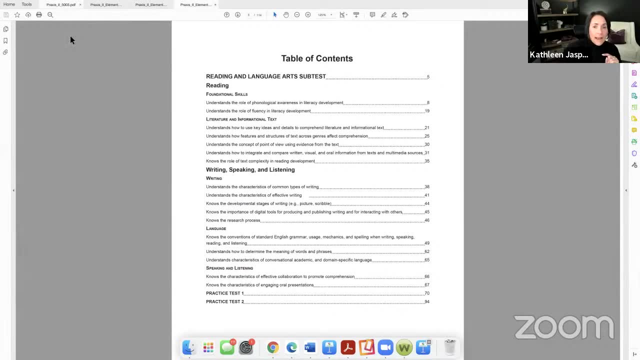 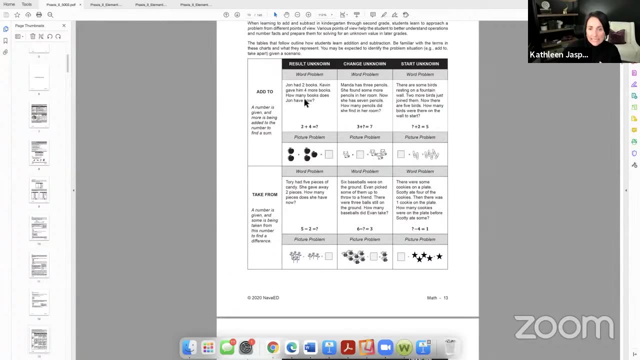 I'm really excited about the giveaway, But before I do that, I just wanted to show you guys something quickly. I just wanted to show you our my thing here, our practice math book. You can see that we have lots of. of course it goes to the easy stuff here. 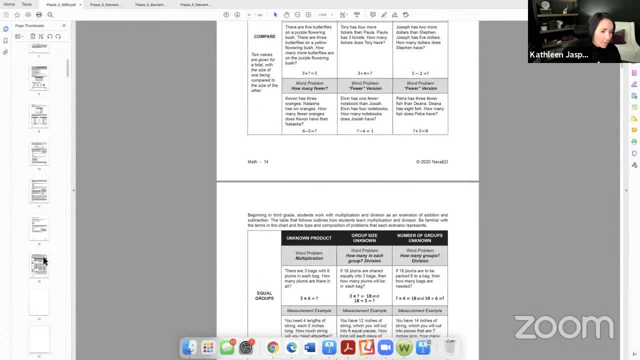 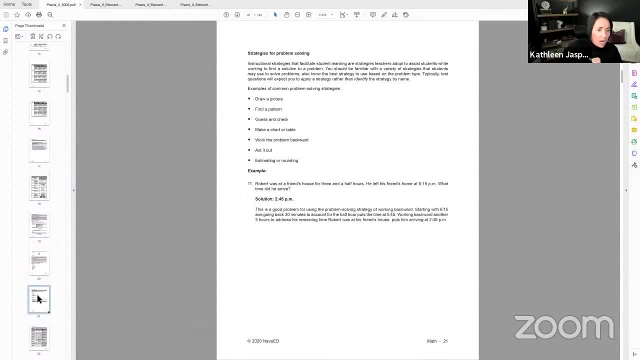 Right, But then we get into the more complicated Good stuff. Hang on, It's going very slow. Give me one second here. Then it goes into the more complicated stuff, where we get into, you know, fractions, part versus whole unit fractions. 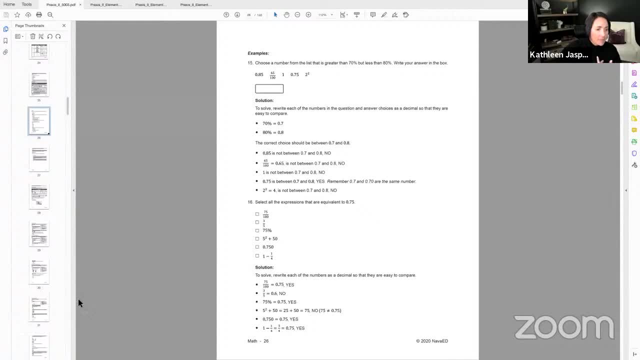 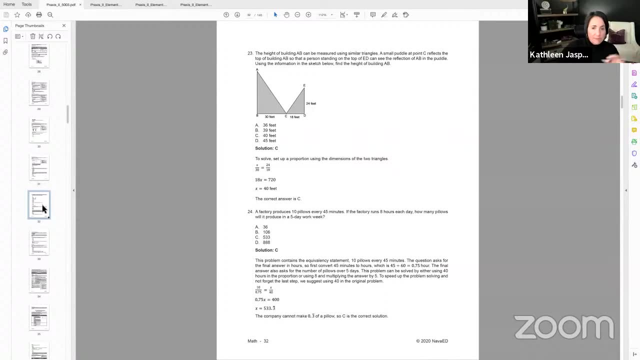 There's tons of practice problems in this book. Then it goes to proportions. We've got, you know, different shapes, proportions in terms of shapes, proportions terms of rates. Then we get into the real number system. We get into 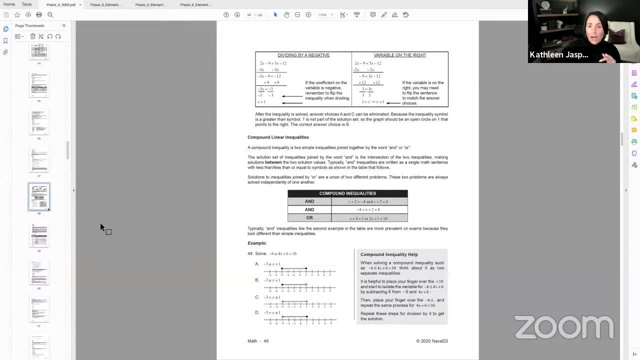 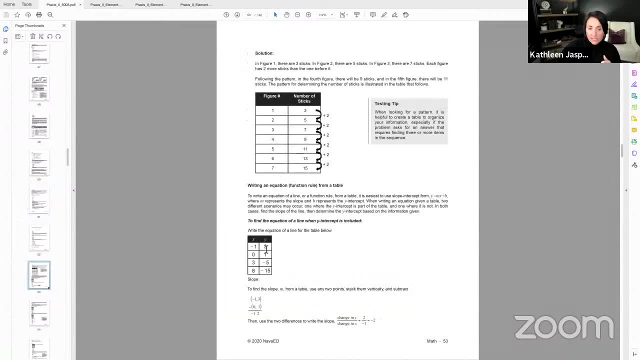 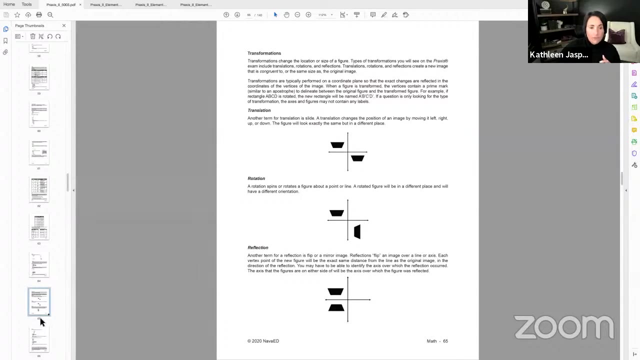 Sorry About that. We get into slope, slope intercept, We get into inequalities. I mean, the math on this is really, really tough. You can see slope- This is the one that I did with you just a minute ago- And then, of course, we have tons of practice problems, tons of different things going on here. 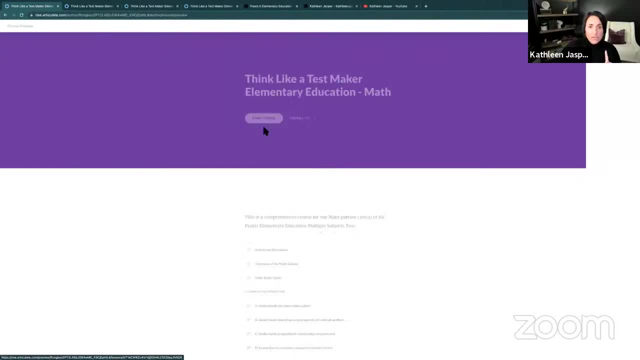 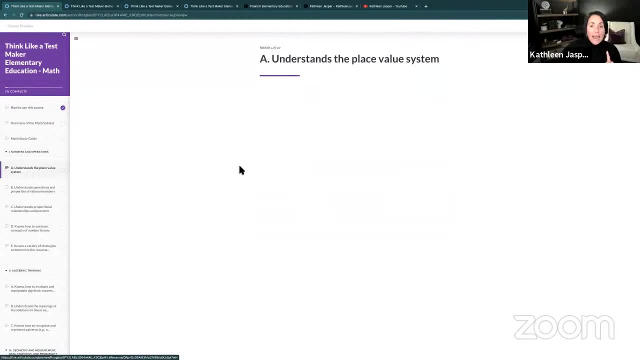 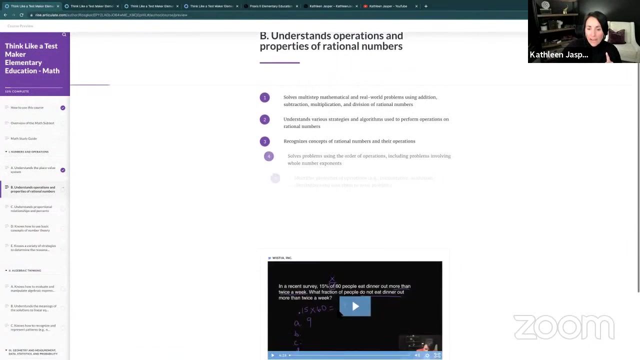 And then another thing I wanted to show you is our math course is very comprehensive here. Look at all of this. So look at over here Numbers and operations. I have tons. I have tons of practice problems. You keep hitting- continue. We have videos for everything. 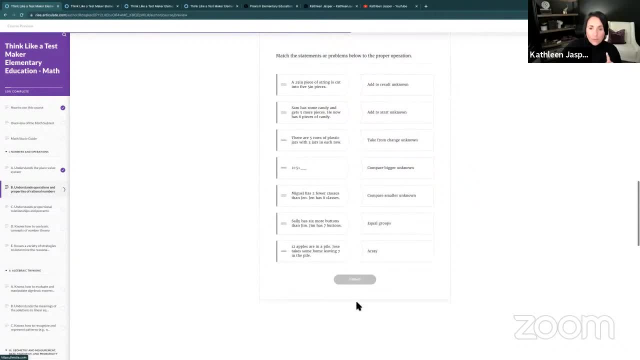 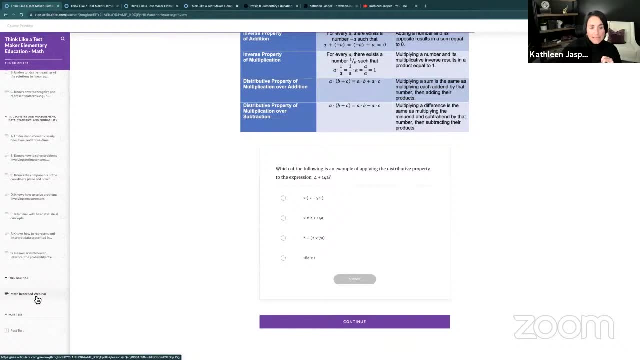 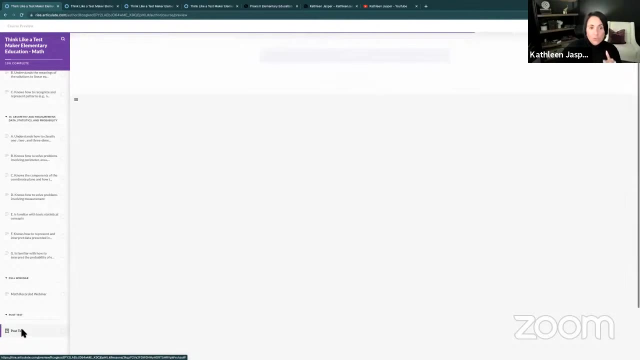 Hit, continue, Continue. Notice so many problems and practice problems here, All of the different things here. And then we have a webinar you can use as an audio course or it's just more practice. And then we have a post-test here that you can do online, which will help you if you're trying to get good at taking the test online. 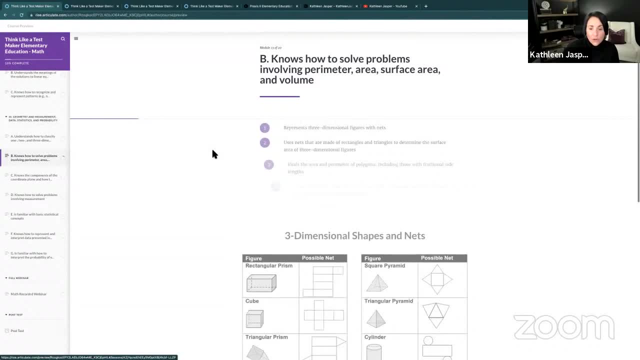 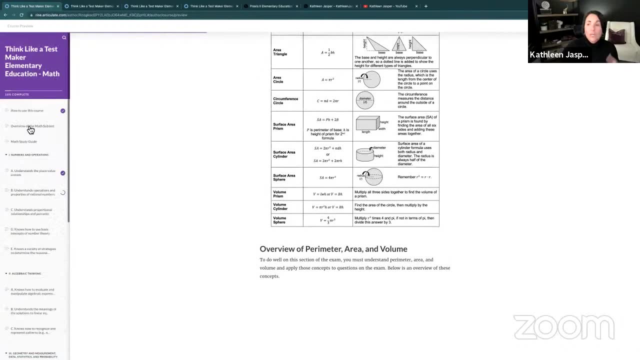 which is what you're going to be, But this course is full of just. it's got so much. So if you're someone who struggles with math, I highly recommend you get yourself a course or you really focus on those skills, And I even go through how to use this course, because it is giant. 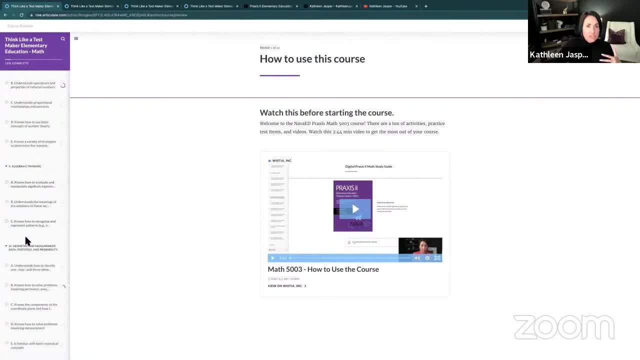 And so you know you could do one section each day. All right, One section each day, And that will really help you. All right, So now we're going to go into our giveaway. I'm giving away some $50 store credits. 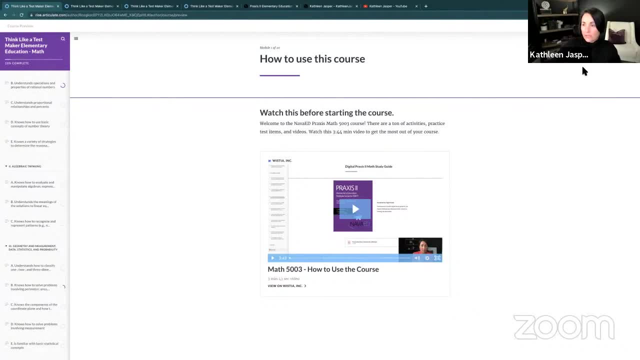 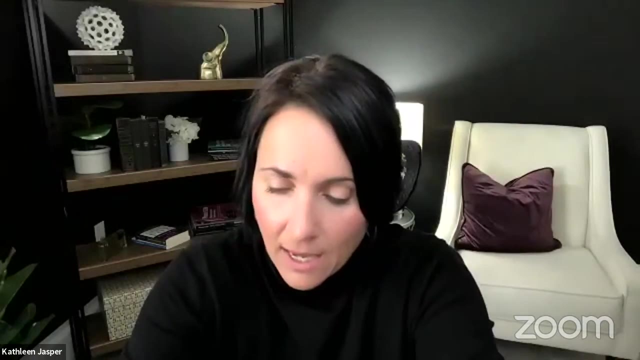 And so I'm just going to do. I have a random generator on my screen and I just want to go through and see who might have me go to. Let me stop share here so I can do my random generator here, All right, So randomly I'm picking John Thompson. 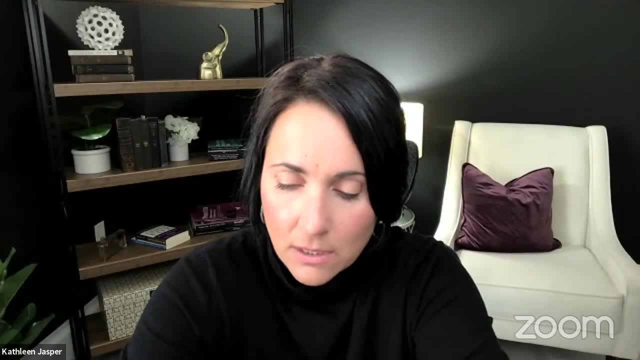 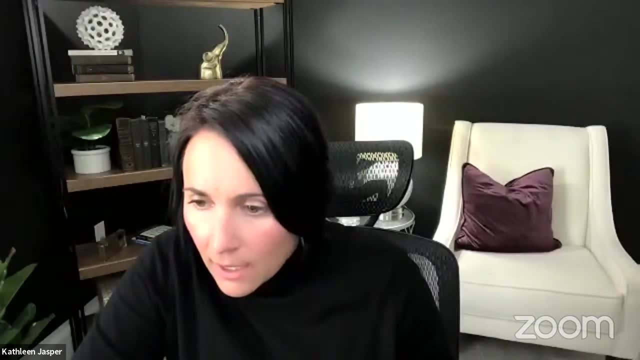 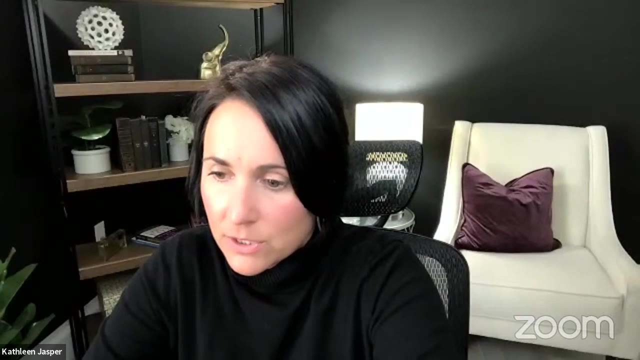 Are you here on line, John Thompson? Are you, if you? if you are, let me know in the chat, John Thompson. Let me go down to my chat, John Thompson, Are you here? If not, I'm going to. maybe it's somebody signed in as John Thompson. 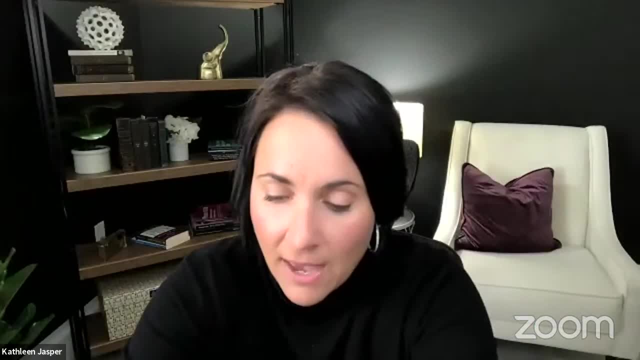 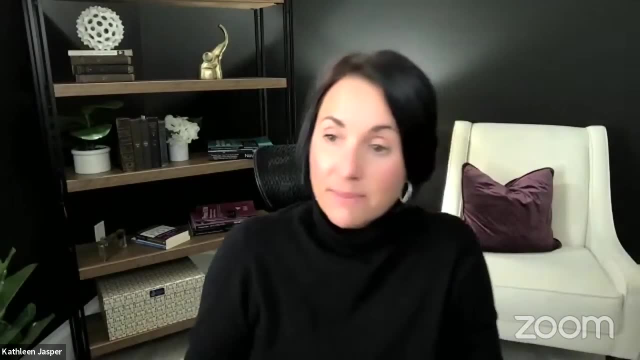 All right, John, Awesome job. Well, you just got yourself $50 store credit. You'll get an email from me later on today with that, So you can use that to buy anything on my website. All right, So really awesome stuff. 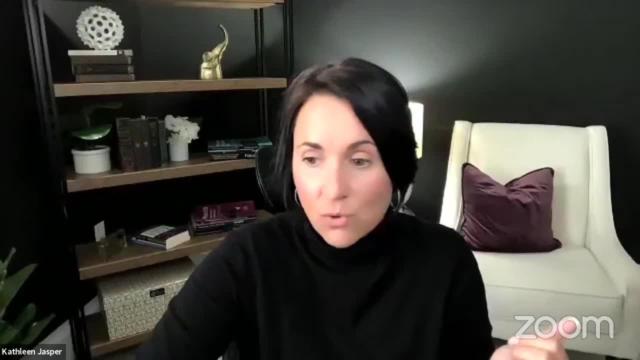 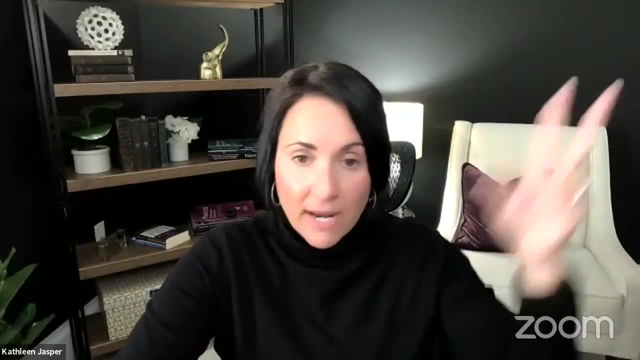 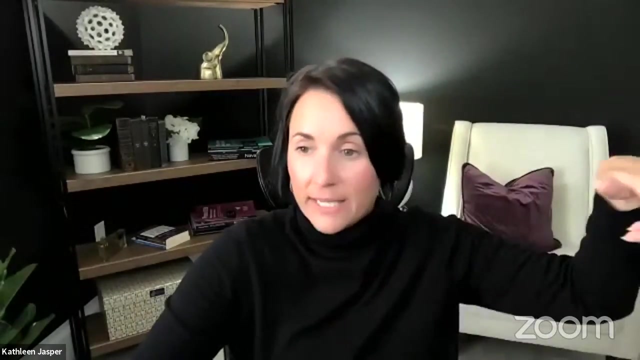 We've got books and all of that, So you can check that out. We have the digital course there. So well done, John. Good job, And I'm going to be giving away more store credit for the other ones, So just stay here and you'll get entered to win. 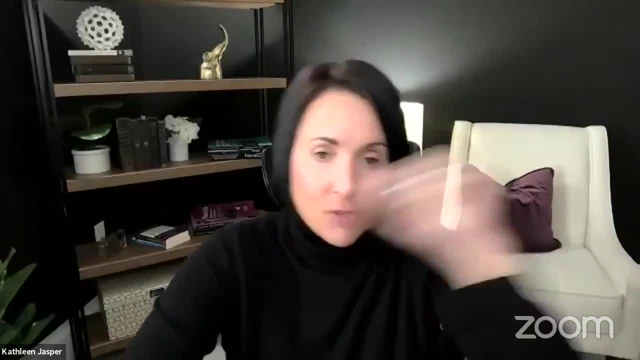 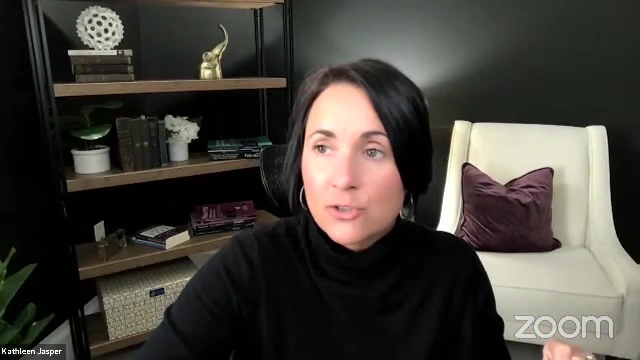 If you're on Zoom, you're going into this hat and I'm just pulling from- you know proverbial hat. It's a fake hat, I'm just randomly generating. All right. So, John, good job. $50 store credit coming your way after this is over. 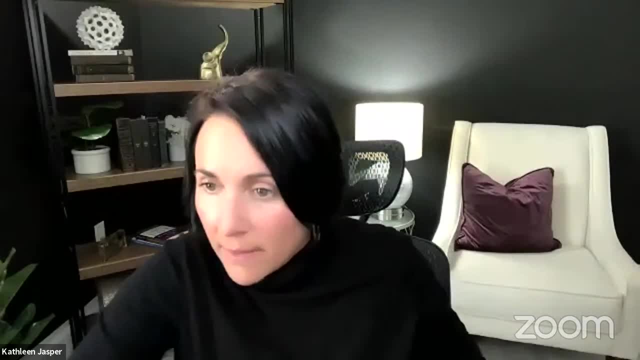 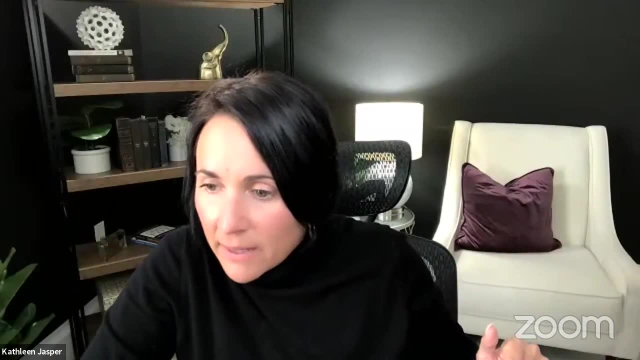 All right, Now anybody. let me just check my chat real quick. Some people are saying how they struggling, how they're struggling with math. Someone asked: is my mic off? Your mic is always off on my webinars. I make sure everybody's muted. 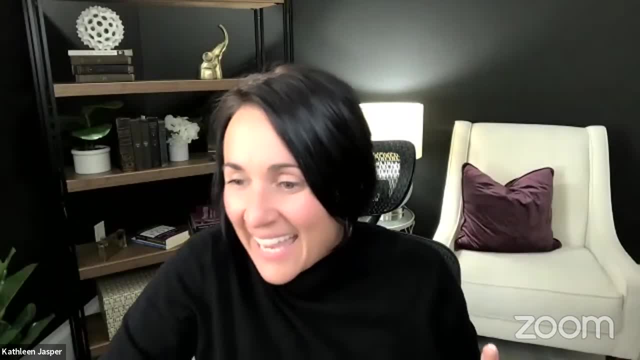 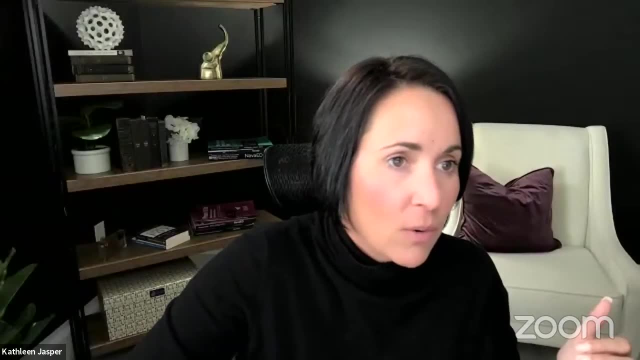 So don't worry if you made a sound, I don't think anybody can hear you And it looks like we're good here. All right, Let me just check Facebook and make sure there isn't anybody with like any burning questions on Facebook. really quickly. 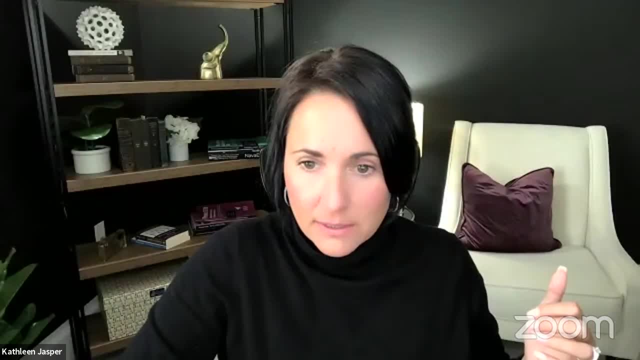 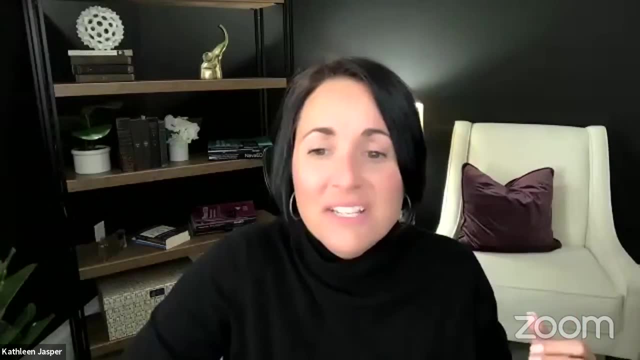 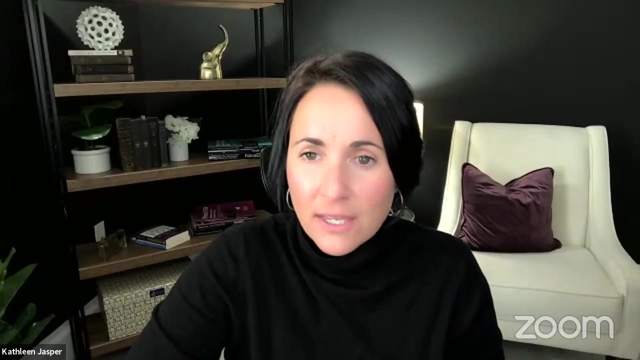 All right, Looks like we have one comment. Christina, if he is not, I am for sure You got Christina. If you're in Zoom, Christina, if you sign up using the oh, you know what I have the wrong thing on. 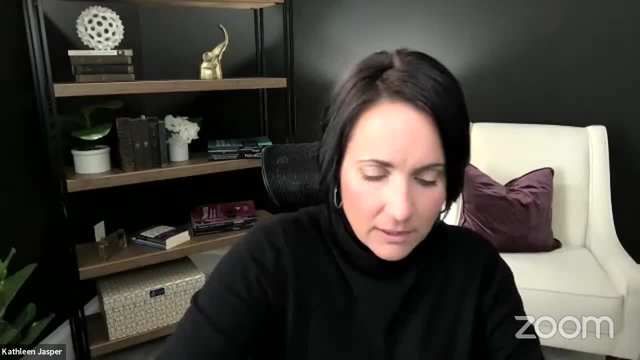 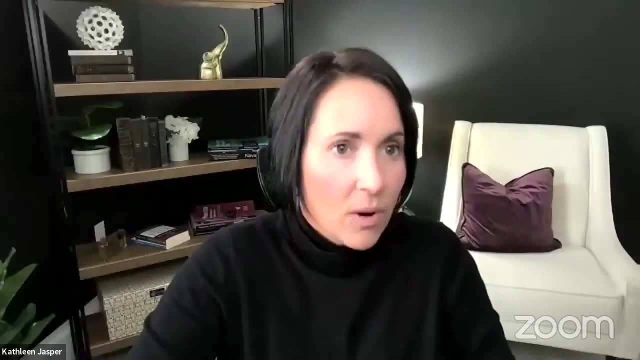 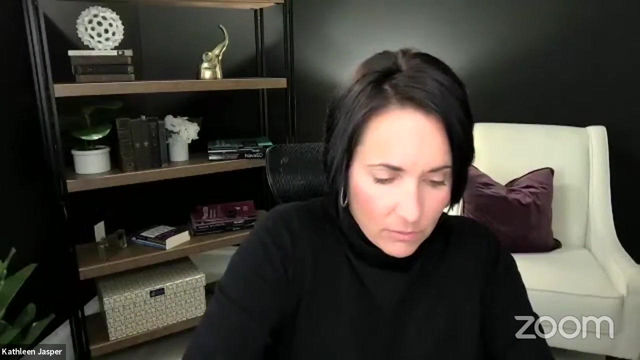 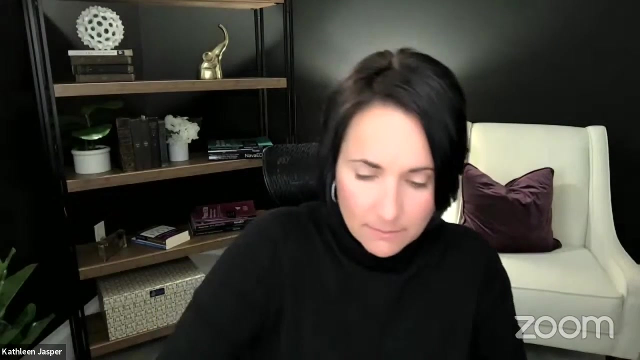 Let me go to really quickly. Let me get my thing here. I have the wrong thing on Facebook. Let me just fix the link really quick. Okay, To get resources, click here. Sorry about that. I have the old math link and sorry. 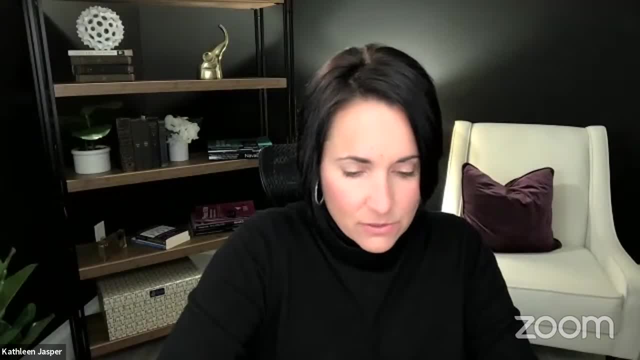 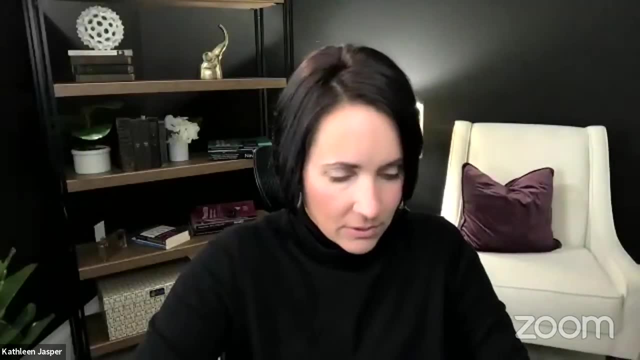 Praxis 5001.. Sorry about that, guys. I'm going to change it in my restream. That was the one thing I forgot to do, And give me one second Talk amongst yourselves really quickly. I need to fix this. 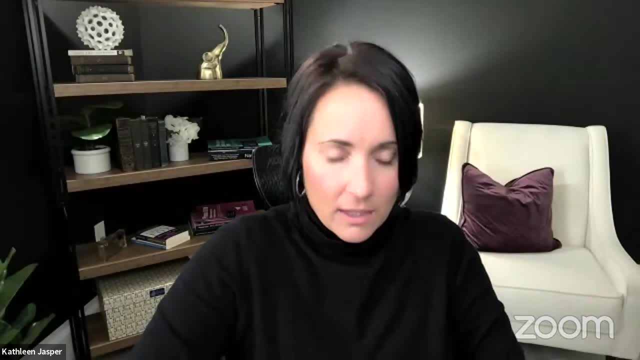 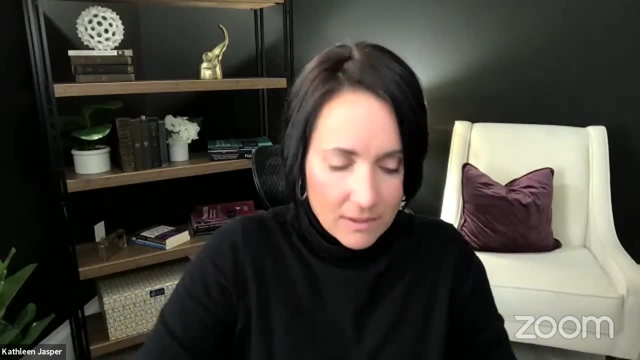 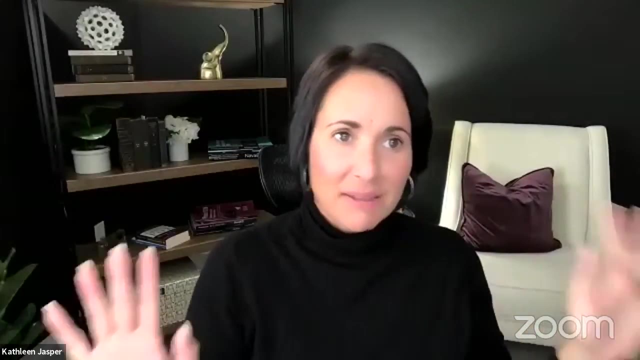 I need to fix this in terms of my title. Okay, because I have the math webinar. There we go. It should be fixed all up. There we go, Okay. so let me go back. Sorry about that little live TV there. 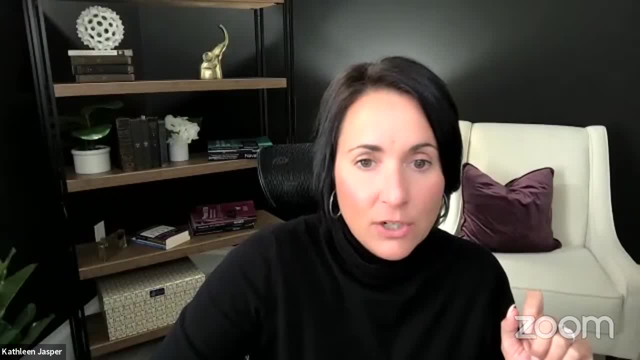 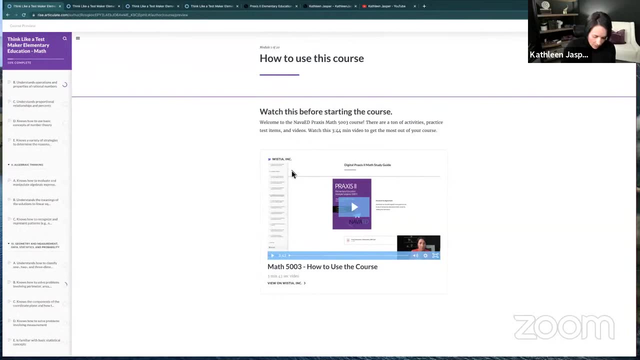 Okay, so let's go. now. We're going to go to social science. Again, you're going to want to stay with me till the end because I'm giving away a bunch of store credit, So you can check that out. So let's go to social studies. 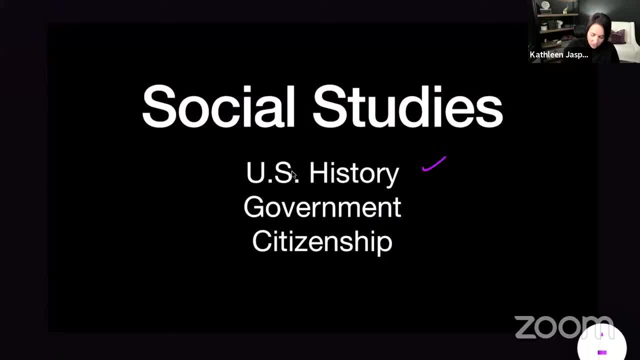 So in social studies we have three main things. We have US history, government and citizenship, All right, and these are the three main categories. US history obviously is going to be everything from: oh this is actually US history, government, citizenship. 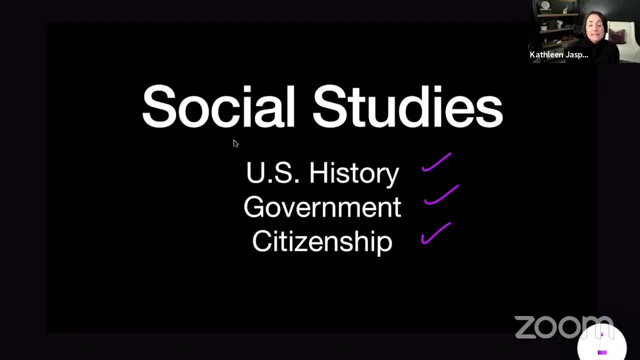 for the first section of social studies And that is going to be things like, obviously, the Civil War, the Declaration of Independence, all of that. The government's going to be like the three branches of government and that kind of thing and how the government runs. 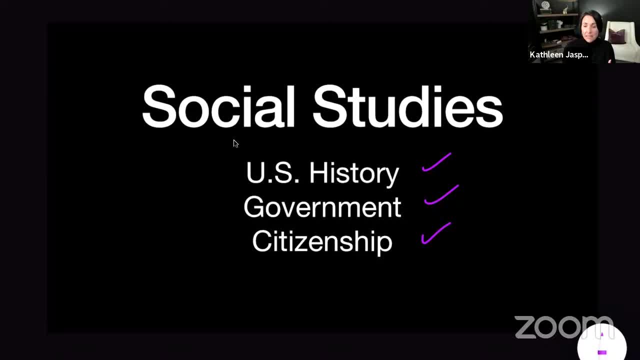 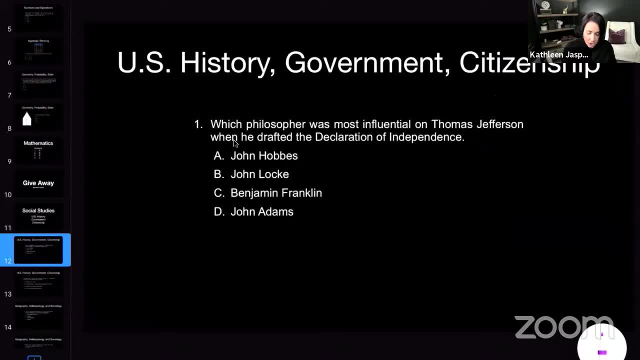 And then citizenship is going to be civics. our responsibility as citizens of the United States that they really hammer that in with students. They want them to understand their civics. So we have US history, government and citizenship. So let's take a look at what you might see on the test for that. 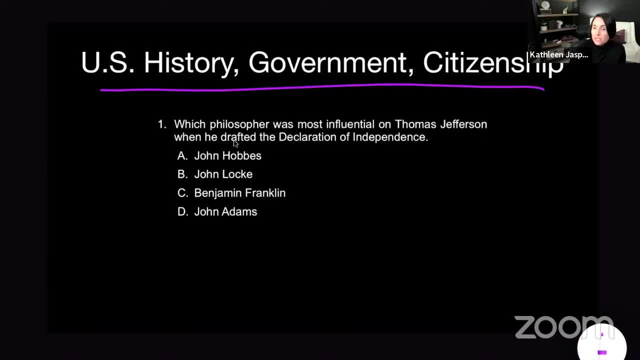 So we have which philosopher was most influential on Thomas Jefferson when he drafted the Declaration of Independence? So a couple of things here. I should have started with my answer choices. I forgot. We have some people in history. We have Hobbes, Locke, Franklin and John Adams. 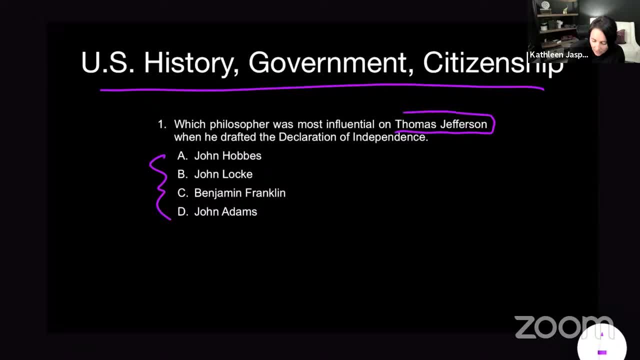 Of course, you're going to get a question on Thomas Jefferson, on the US history And a couple of things to remember about Thomas Jefferson. He was heavily influenced by philosophers, typically John Locke. So the answer is John Locke, And let me tell you why. 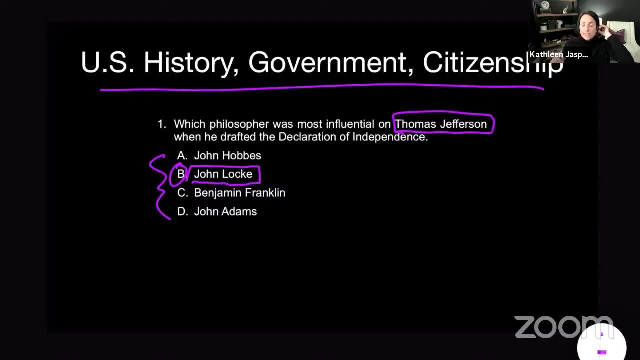 So think about it. Thomas Jefferson wrote the Declaration of Independence. Thomas Jefferson was all about the freedom of a person to decide his or her fate. Now, he also was a slave owner, And so he also didn't free his slaves. He had slaves until the end. 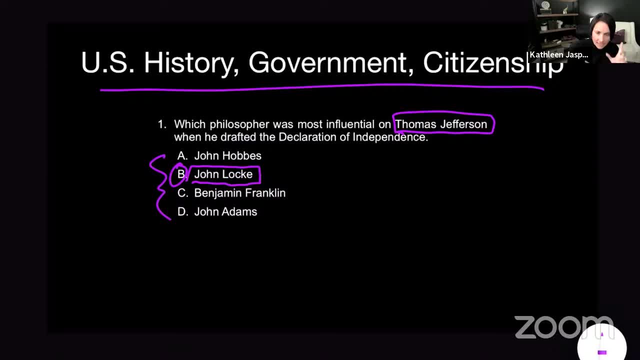 So it's a complicated past. Just want to put that in there. But he did draft the Declaration of Independence, which did lead to our independence from Great Britain. Now He was influenced by Locke. Now let me tell you the difference between Hobbes and Locke. 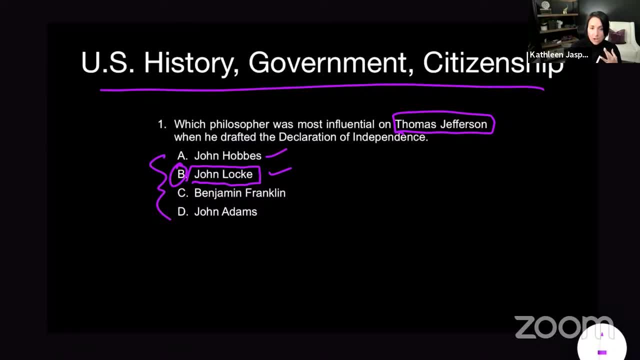 because this might help you on the exam. So two philosophers, John Hobbes and John Locke, talk about a social contract between the individual and society. Basically, like when I go outside and walk around and run my life, I'm engaging in a social contract to not kill anyone, to not steal. 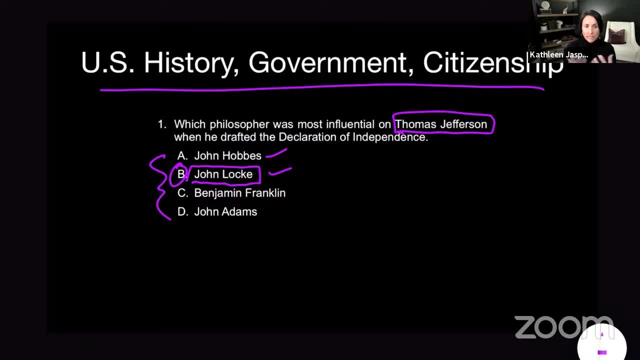 and that we need to have that social contract right. We need to treat people with respect. We need to. We need to be able to do our own thing without hurting other people, so to speak. It's much more complicated than that. 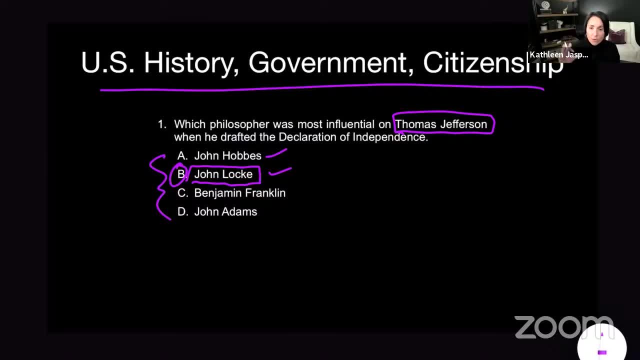 These guys are philosophers, It's. you know. some of you are really into history, You know more about it than I, But those are the two things. Now, the difference between Hobbes and Locke was. John Locke thought, as people, we are able to engage in that social contract without the help of government. 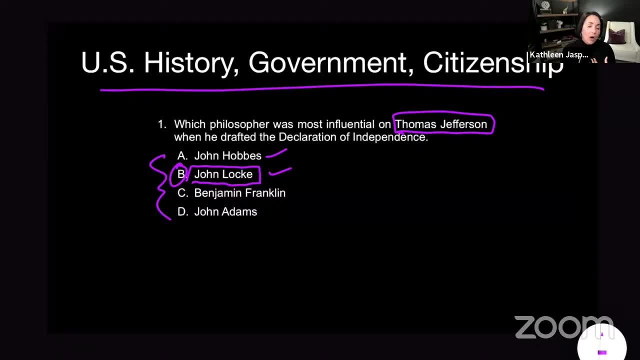 That in innate, in our innate senses, we are good And that we will. We will do the right thing and we don't need government to tell us what to do. right, Notice the Declaration of Independence. right, We can be independent of government. 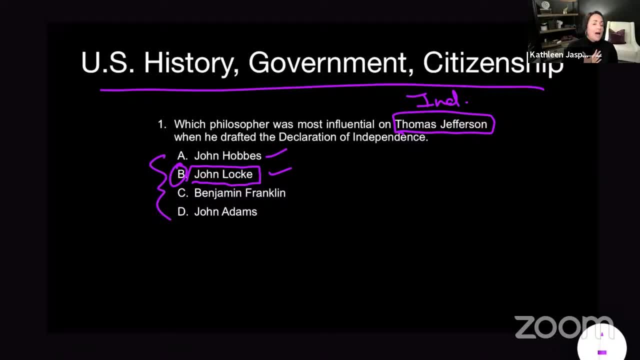 Hobbes was like: no, I don't think so. Hobbes was like: humans are innately evil and they need government to help them not to be so evil. And so to say, two of the same social contract but two very different philosophies. 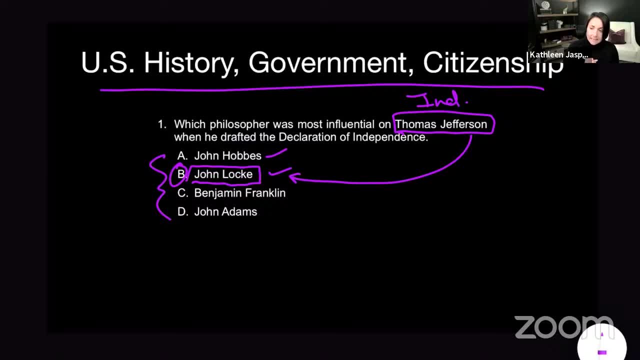 Obviously, Thomas Jefferson is all about the independence and that's going to help them there Now. John Adams and Ben Franklin were a part of Thomas Jefferson's life And I've been reading because I've been working on a social science high school. 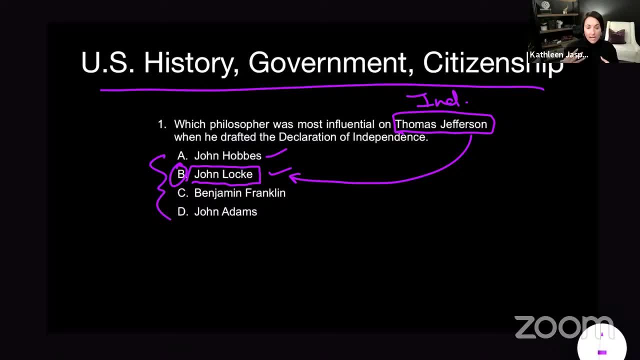 book for the high school exam and I'm really trying to read a lot of history, So I'm consuming a lot, But when we're talking about philosophers, we're talking about John Locke or John Hobbes, that they were way back in the day. 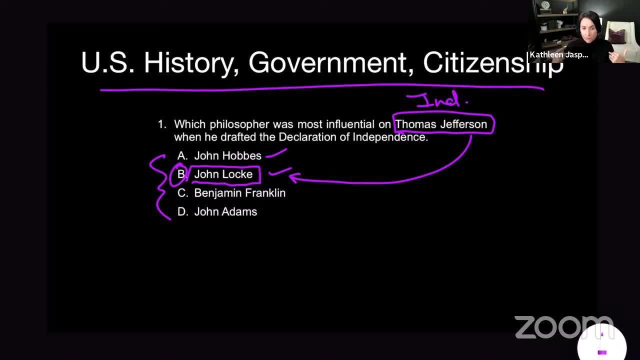 and they helped Thomas Jefferson in turn think of what independence means. So think about that. Locke and Jefferson go together when it comes to the Declaration of Independence and the start of our nation. independence for some- Let's just say that- not independence for all. 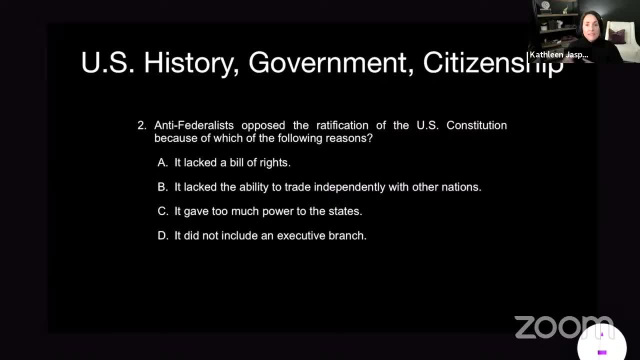 All right, Let's do another one. US history: government and citizenship. This is going to be more of a government and citizenship question Now. this is where you're going to be able to think like a test maker In this kind of situation. here you've got to know your people. 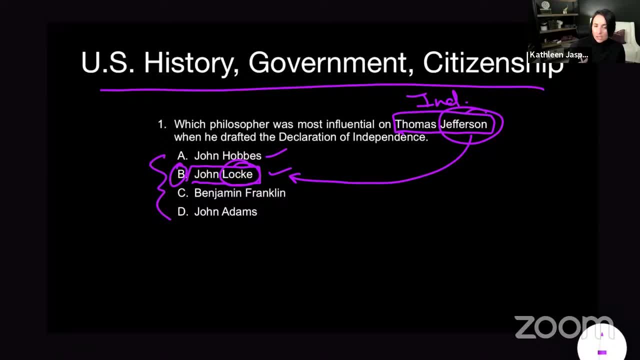 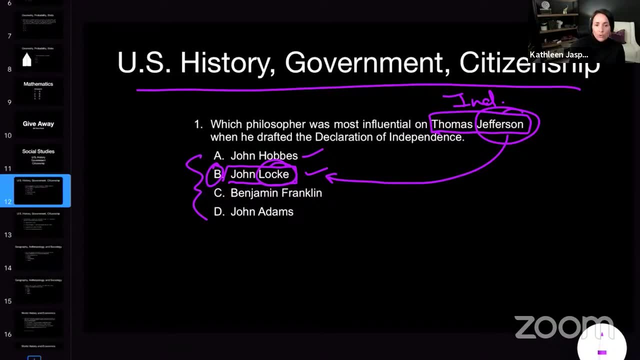 so to speak. but you always want to focus in on John Locke when you're thinking about our history. just a little side note there. But you can't really use the think like a test maker, because you have to know who the person was who influenced Thomas Jefferson. 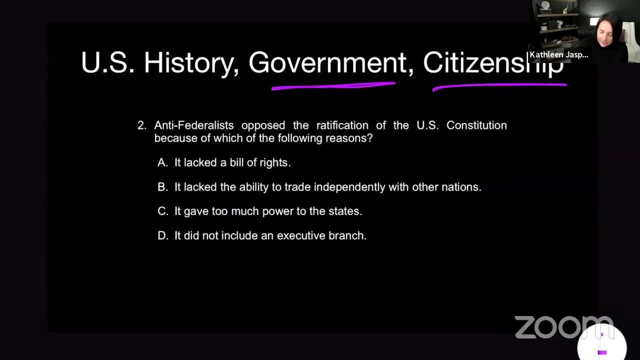 But in this one we can think like a test maker. If we're thinking about this, we know for sure this is a government also a history and citizenship question kind of encompasses most. Let's take a look at the answer choices and see if we can find the best answer without even reading the question. 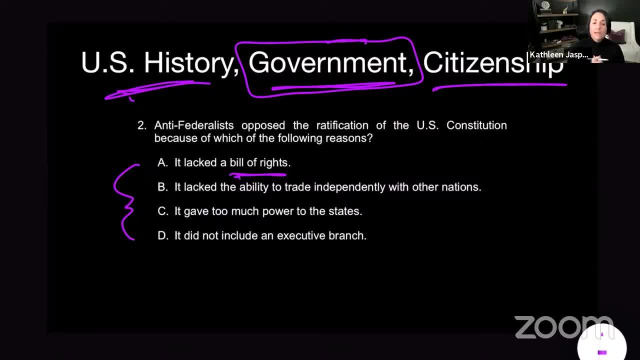 So we have. It lacked a bill of rights. keyword: their bill of rights. It lacked the ability to trade independently with other nations. OK, it gave too much power to the states and it did not include an executive branch. All right, Right away. 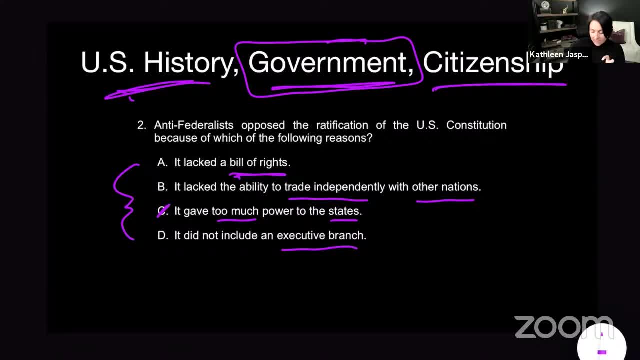 I can cross off C because- or in my mind, think about that- that's not going to be a good answer, because the biggest thing about our government is that the states are sovereign, and then we don't have this central. well, we do have a centralized government. 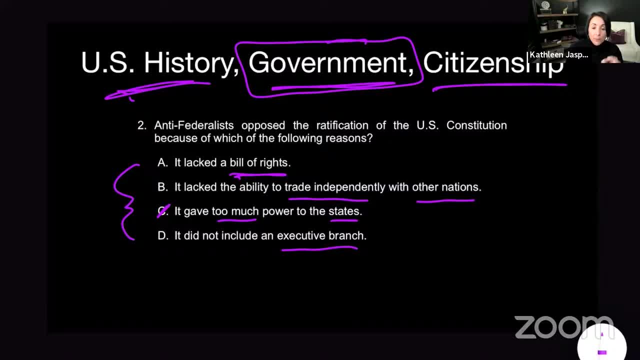 But that the states have their own power And the point is to give power to the states because we don't want the federal government. Well, some people don't want, some people do. It just depends on kind of where you are on which issue. 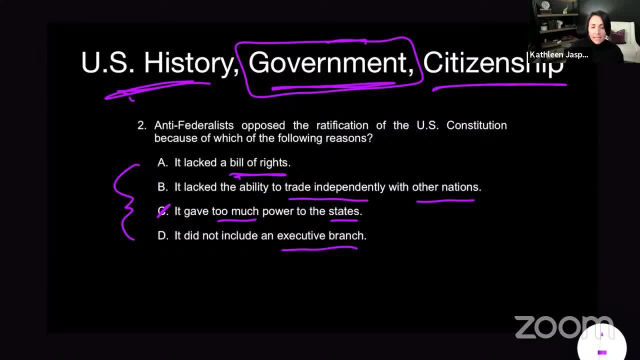 It's very complicated, But basically the philosophy is: states should be sovereign and they should be able to. well, not necessarily sovereign, They should have the power to run their own states. So it gets complicated with things like COVID and education and all these things, because states have their own power. 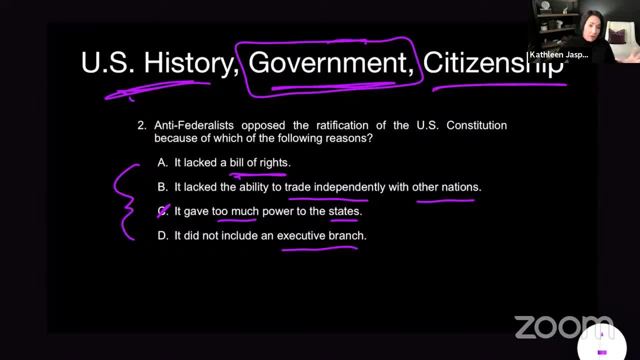 And notice what's going on in Texas right now. They're doing their thing and the federal government is trying to intervene and Texas is like: no, we can do what we want. We're Texas. Florida does the same thing. Notice that in in New York and California they had very strict covid. 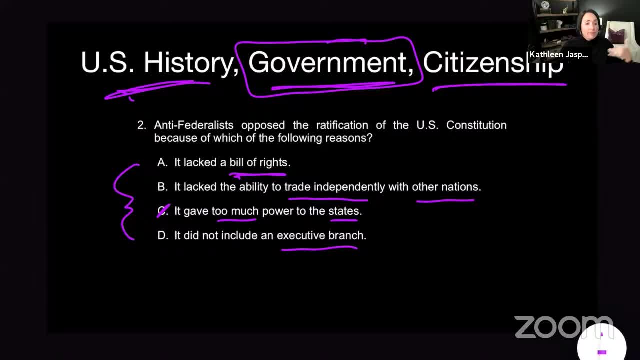 restrictions- and I'm not getting political here, I'm just saying the difference- is Florida, where I'm from, And Texas had very, I would say, not as strict covid restrictions, And so that's really because the states have their own power. So I'm going to cross off C because we 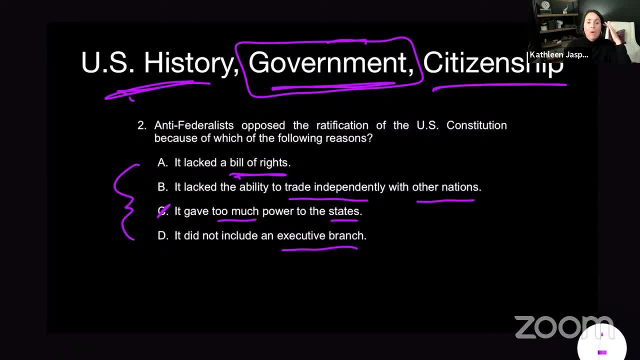 want the states, according to the philosophy of the government, to have power. But I'm going to hone in on this bill of rights because we're talking about government and the Bill of Rights is really important when it comes to our government. So let's go with the question. 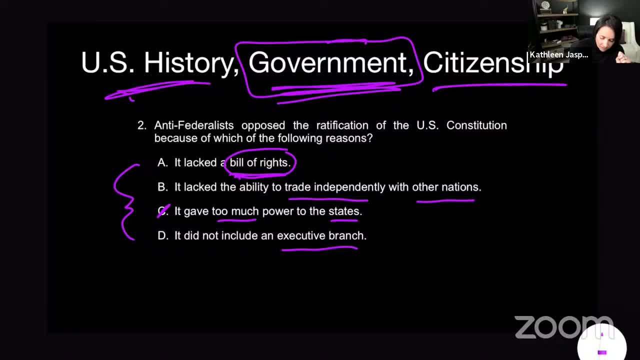 Anti federalists. So anti federalists meaning kind of anti federal governments, meaning anti centralized governments, oppose the ratification of the US Constitution because of which of the following reasons. Now, what does the Bill of Rights give us? It gives the citizen a set of rights. 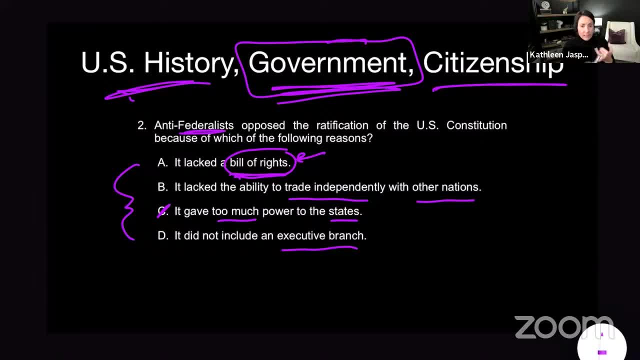 Right, So that the government can't, you know, illegally search our home. They can't, They're not supposed to They, you know. the Second Amendment: our right to bear arms. The First Amendment right Free speech and the press and religion and the right to assemble. 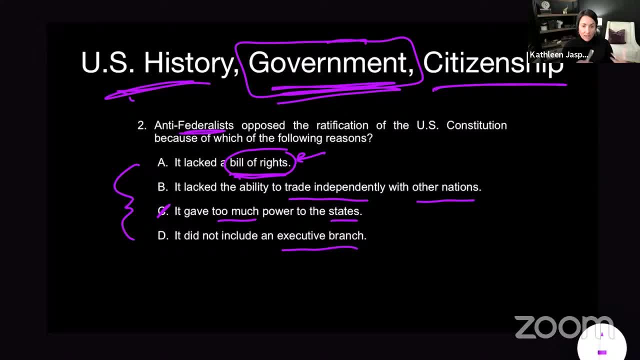 And so that really gives us as human beings in the United States, freedoms, Right Or rights, So anti federalist or anti centralized government people. That's making it very simplified. But we're on the case six. We're not on the high school exam. 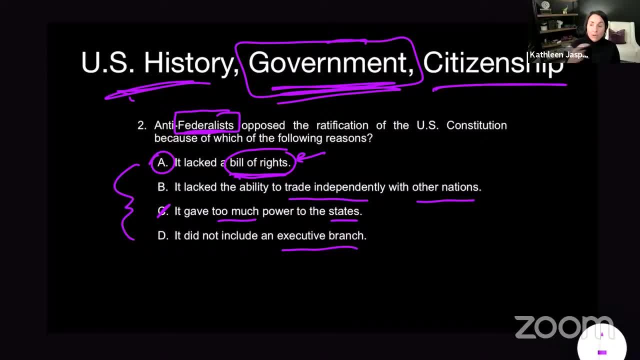 It's going to go with lack. It lacked a Bill of Rights. They wanted a Bill of Rights for the human being in order to ratify the Constitution. This: it lacked the ability to trade independently. We're not, we're talking about the US. 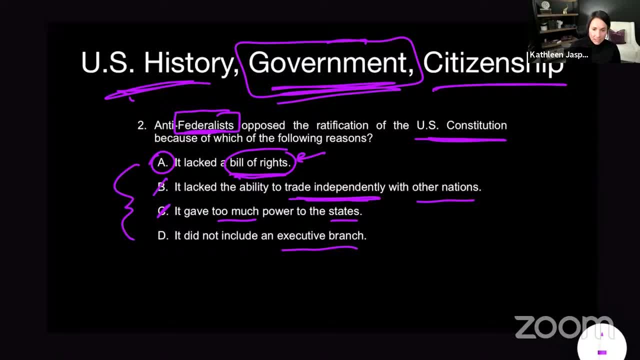 Constitution here. that doesn't really go with B And it did not include an executive branch Right. That is going to be Article two Of the Constitution, which is not what's going on here. It's the Bill of Rights. That's going to be the best thing there. 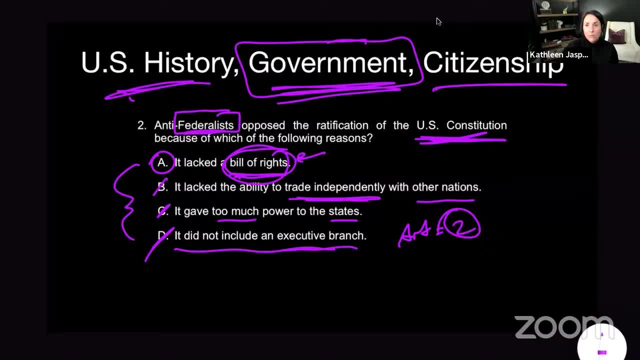 OK, that's anti federalist. All right. I have some people raising their hand which I can't see when I'm sharing screen. So if you have a question and you're in the Zoom, go ahead and throw it in the chat. 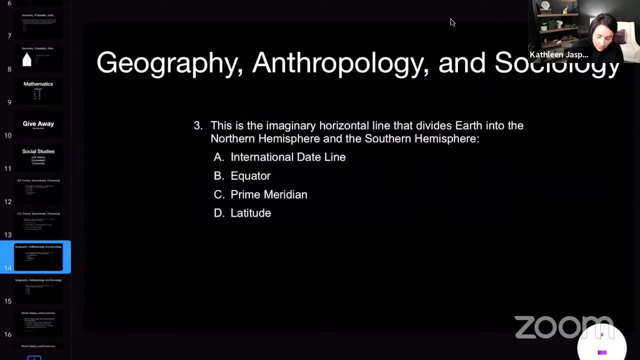 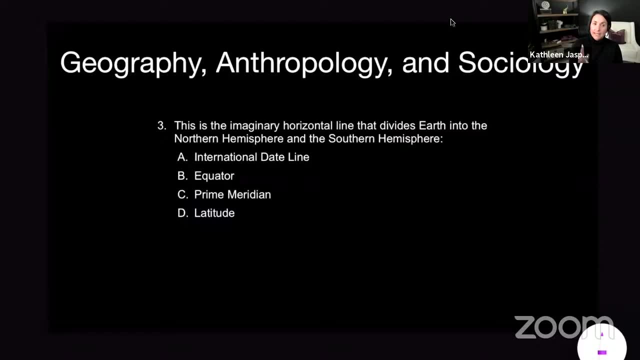 I'll take a look at it as soon as I'm done with this. All right, Now another portion of the test is going to be geography, anthropology and sociology. Now you might say, oh, geography, that's easy. Well, some of these things you might not have thought about in 30 years. 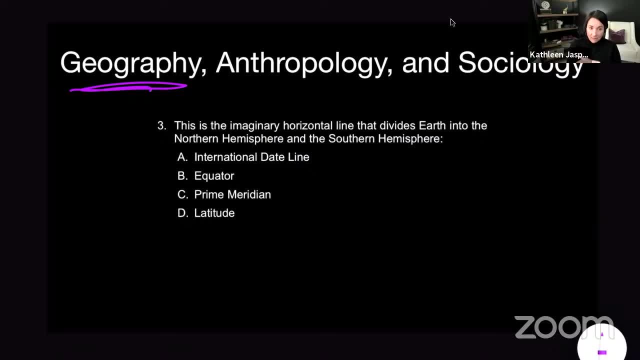 If you're an older person or a career changer, you may not have thought about these things. So let's take a look. This is an imaginary horizontal line that divides Earth into the northern hemisphere and the southern hemisphere. So let's say we've got the map here. 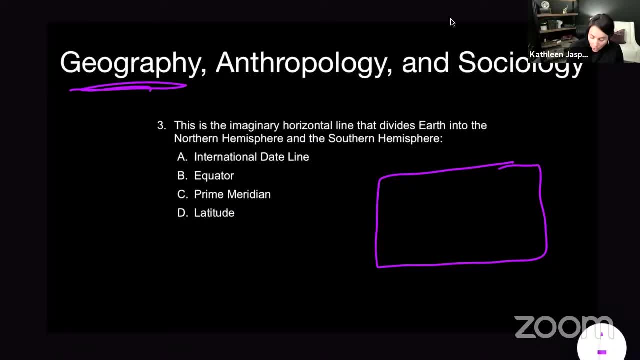 Oh, I'm not going to draw it because it's just going to be terrible, but we're looking at a horizontal line. What is the horizontal line that divides the Earth? Well, that's going to be the equator that puts us in the north- northern hemisphere and the southern hemisphere. 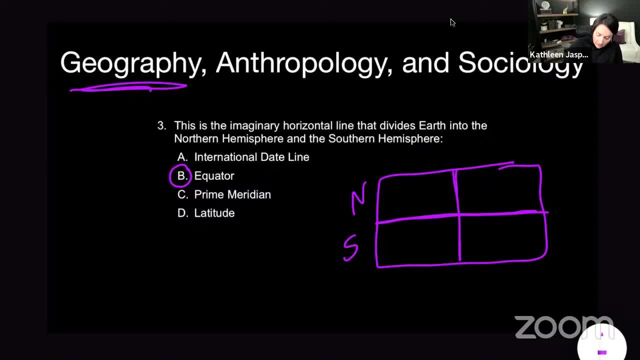 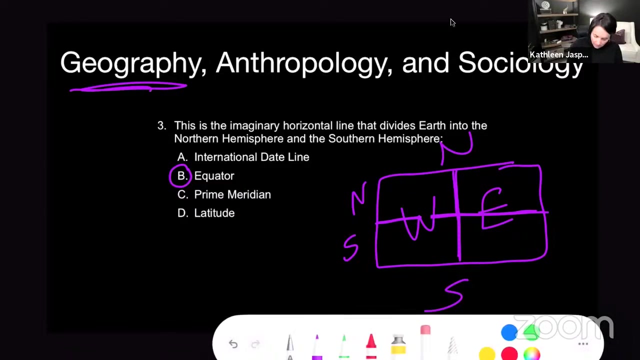 The prime meridian Cuts us for the east and west, so we've got east. Sorry, that's west. Come on, Jasper. We've got west and east Here, So north and south. I should have done it this way. 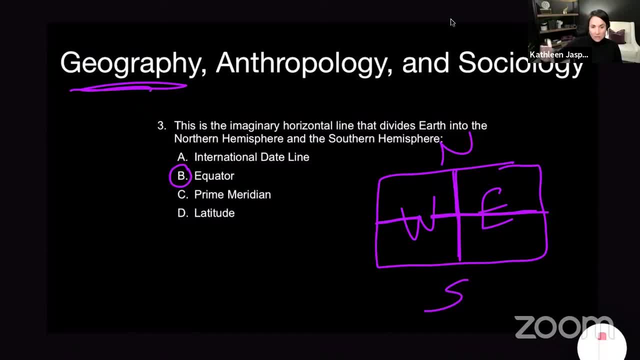 East and west, But the equator is horizontal. That's the one that's going to do it. Latitude are lines of latitude, but they don't necessarily cut. that divides the Earth into the northern hemisphere and the southern hemisphere. Lines of latitude go up. 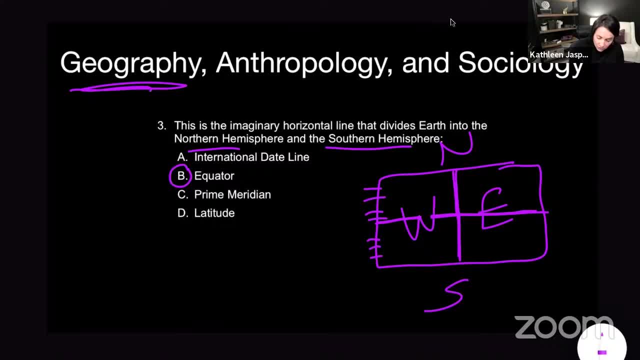 That's like all the way here. Now the international date line goes in between Alaska and Russia and kind of goes down there where the start of the new day happens. It doesn't cut us into the western hemisphere and the eastern hemisphere. OK, now another one which I think is harder, but it's a basic question. 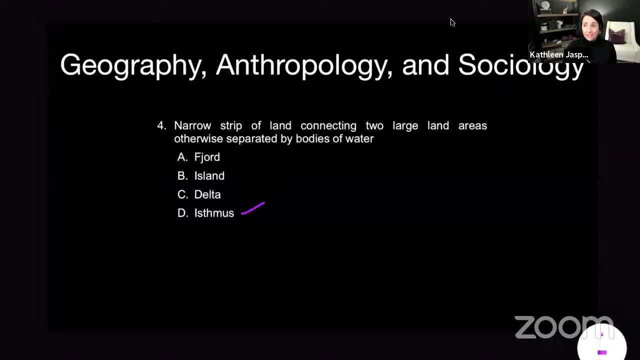 How many of you have thought about a fjord or an isthmus in 30 years? I know I hadn't until I saw them in the study companion. So I'm looking at this going: oh geez, I don't know these land, these land features. 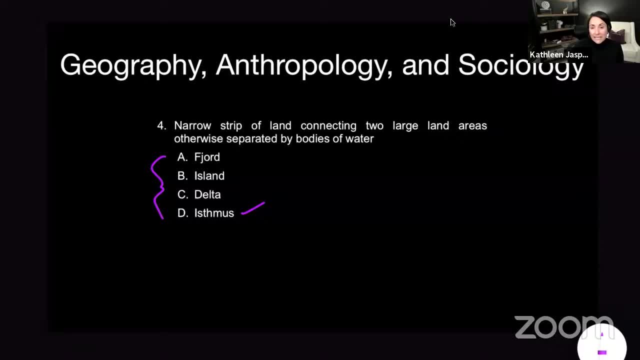 Right, So make sure you get that, And they are in the book. So a narrow strip of land connecting to large land areas otherwise separated by bodies of water. That is an isthmus. OK, an island is obviously here and there's water on all sides. a delta: 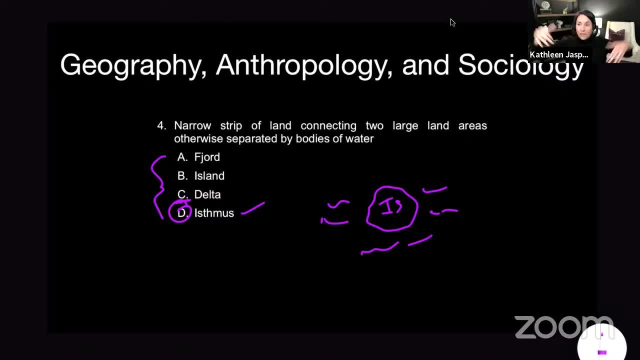 Think about the Mississippi Delta, which is where the river dumps And it's kind of a hodgepodge of fresh and saltwater And it's like kind of a marshy area where the where the delta is, and then a fjord. 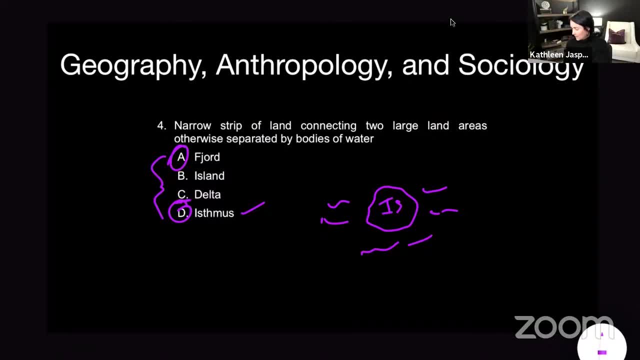 I am here. I didn't look up fjord Anybody in the chat. give me a fjord, fjord, fjord, And I've got it here. It's in the book. Give me a second. Where are we? 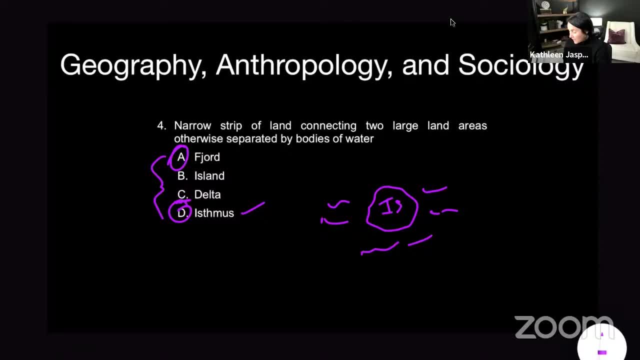 Fjord. There we go, A deep inlet of sea between high cliffs. Oh, yes, yes, yes. So we have high cliffs here and then there's water, But it's, it's the sea. So, on the book in the book, just so you know, like I have this, stop share for a. 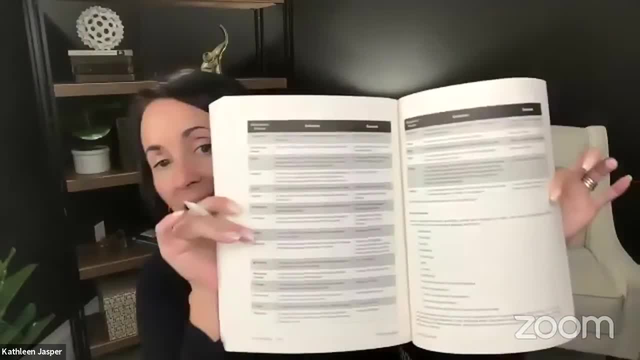 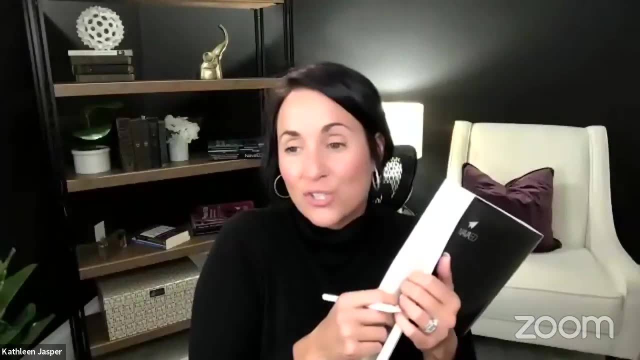 second, there I have this giant table here with all of the different types of land structures. you might be asked on the test. You could make note cards out of these or you could just familiarize yourself with them. That's going to help you. 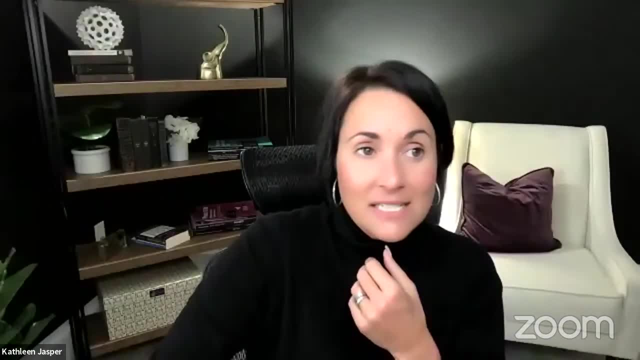 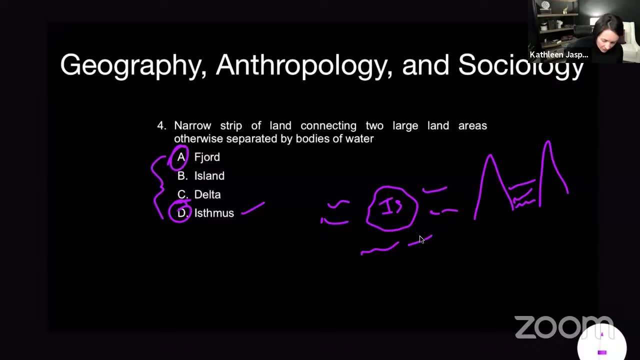 But that's the type of geography question that you would consider kind of easy. But we haven't seen a fjord in a while. We haven't seen a fjord in a while. You're going to have a hard time there, Right? All right. 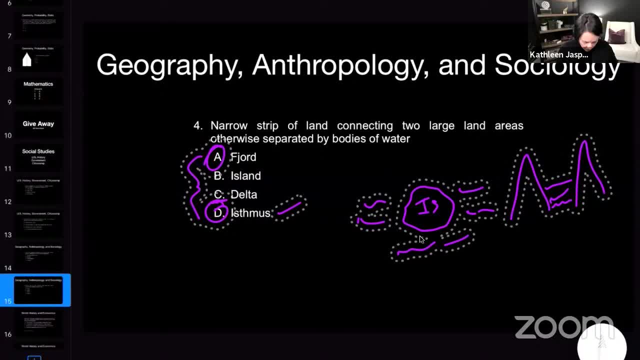 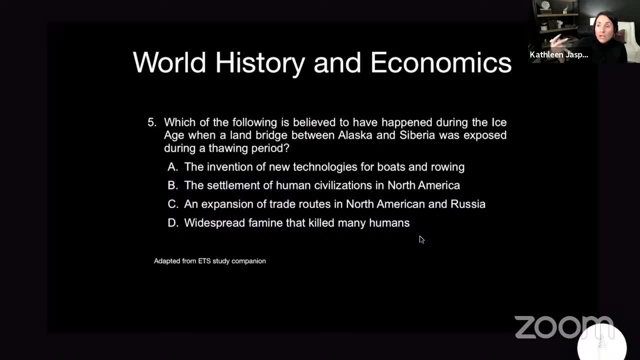 Let's go to the last question here. I got two more questions now. This is world history and economics. So another section. Remember there's three sections: US history, government and citizenship. Then we have geography, which we just did. 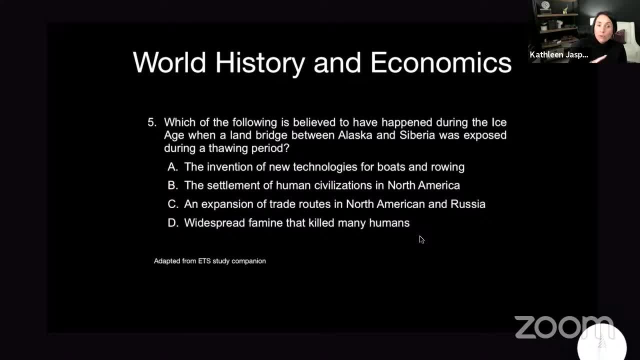 And then you might have a sociology question in there as well. Now we're into world history and economics. All right, This one's actually a world history question And I adapted it from the ETS study companion. All right, So I'm going to go with the answer choices first, like I always do. 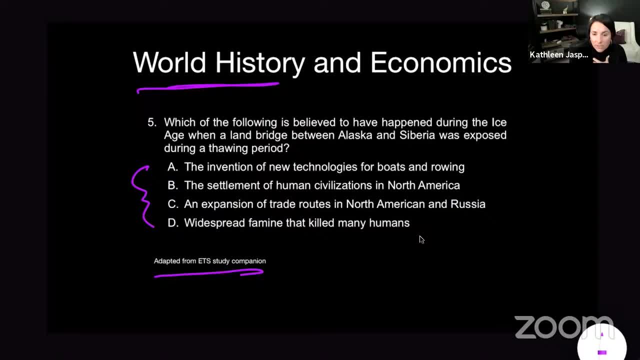 The invention of new technology for boats and rowing. the settlement of human civilizations in North America. the expansion of trade routes in Northern American, Northern America and Russia. widespread famine that killed many humans. All right, I have no idea. I can't do anything yet. 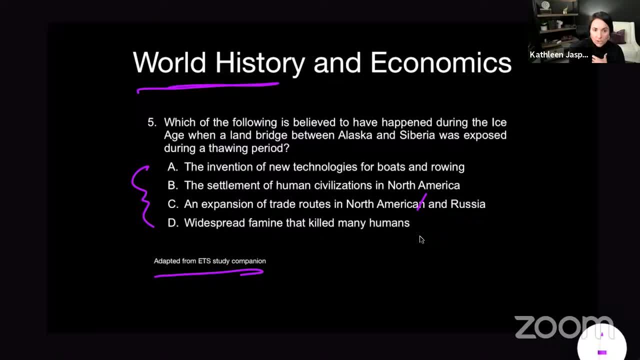 Nothing is standing out to me. Let me look at the question, which the following is believed to have happened during the keywords here: Ice Age, when a land bridge between Alaska and Siberia was exposed during the thawing period. OK, so we're talking Ice Age here. 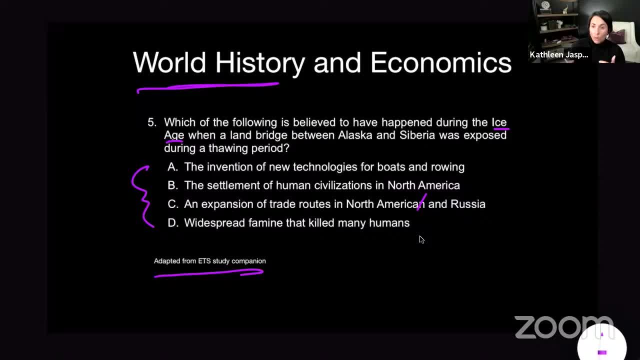 Are we? do we have trade routes going when we're talking about the Ice Age? Probably not. We're not talking about trade routes. All right, Widespread famine here. I guess I don't know enough about the Ice Age. I know that there. 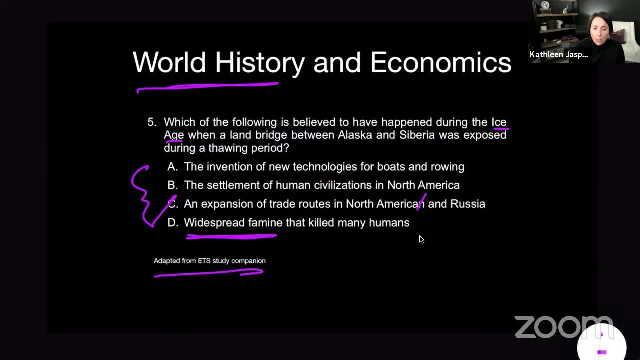 There were problems with with getting food, But when we talk about widespread famine, we're usually talking about the Dust Bowl, things like that. And when we say a land bridge, what can happen with a land bridge? Siberia is over in Asia and Alaska is over here on the northern North America. 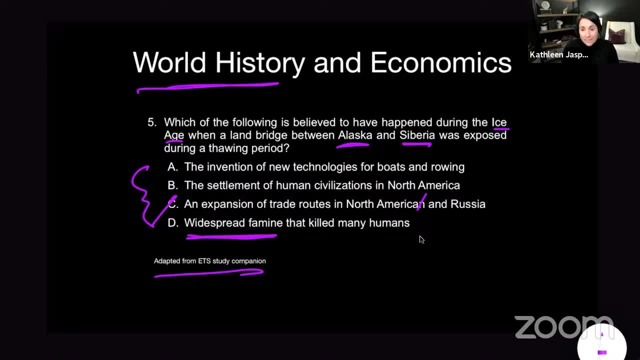 So what happened? People walked across the land bridge. Now, it wasn't that simple. Obviously, it was probably very treacherous and awful, But they got across that land bridge and then started to come down through- Can't Well, Alaska, what is now Canada- and come down into North America now. 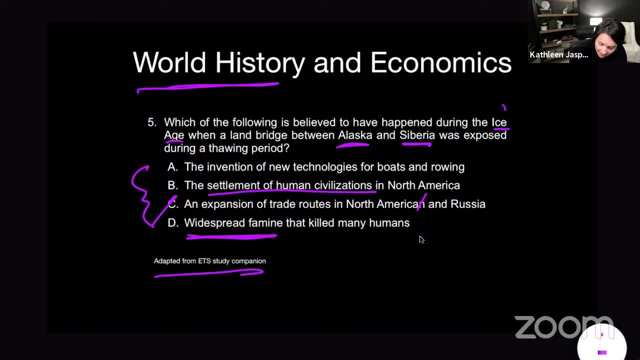 Also the settlement of human civilizations that kind of matches this Ice Age. We're early human civilizations, So I like be the invention of new technologies for boats and rowing. We're talking about a land bridge, So no boats, no rowing. 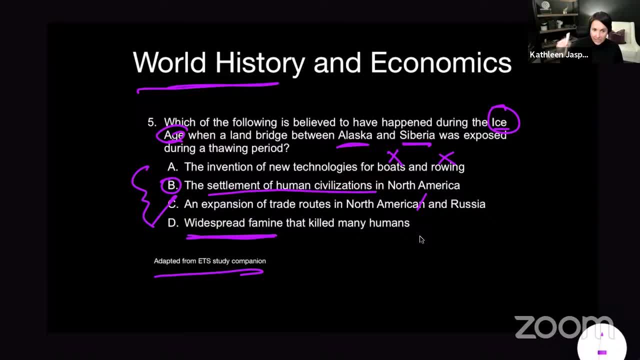 We didn't need that. It's a land bridge. Go with the key words in the question here. Remember: think like a test maker. OK, They're going to throw these in here because you're Like: oh, boats and rowing. 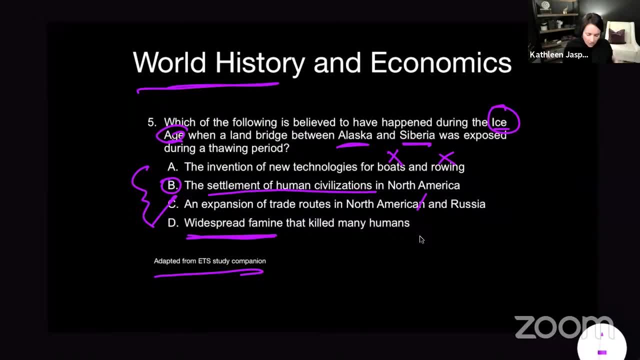 Yeah, early people. they did boats and rowing. I'm talking about land coming across land. A is out and then D is not as good as B. It is true, The settlement of human civilizations in North America was the result. But even if I didn't know that, I could use my think like a test maker: brain. 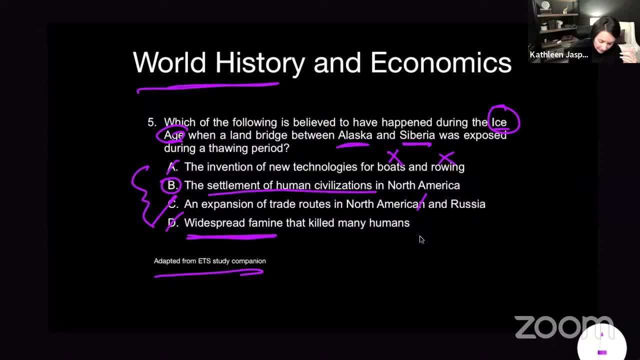 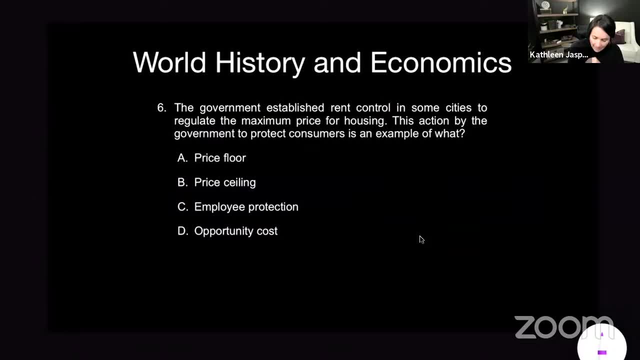 and get rid of almost all of these, where I would be in between B and D, and B would be the best answer there. All right, All right. Final one for social science. Now we're getting into economics. Now they've got some tough economics. 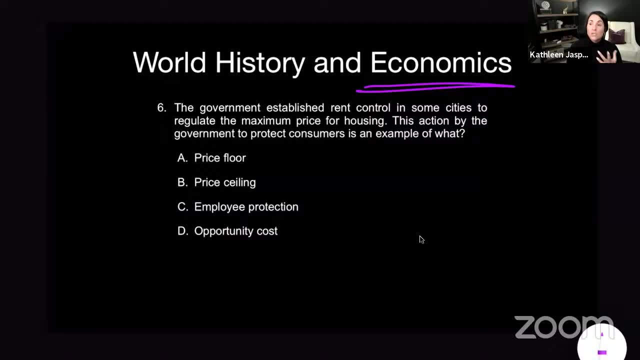 questions on this exam. so you definitely want to brush up on some of your basics. you know supply and demand, that type of thing. But I chose this because you can think like a test maker here. So I've got price floor, price ceiling. 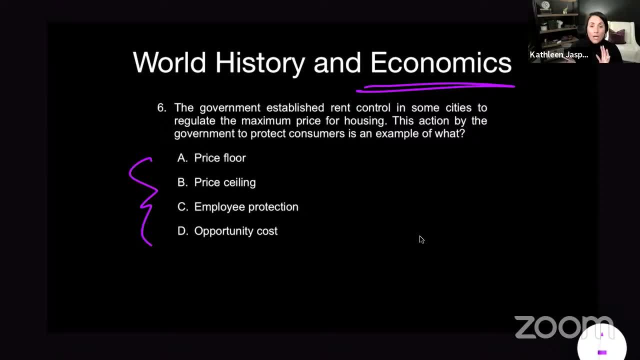 employee protection and opportunity cost. All right, Let's take a look. The question stem here says: this action by the government to protect consumers is an example of. So I have consumers. This says employee protection. This is opportunity cost Right away. notice: working backwards I could kind of cross them off. 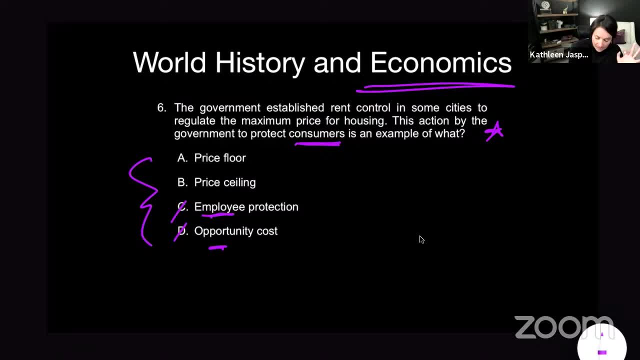 So I'm talking about consumers, not employees, and opportunity cost typically goes for biz owners. So I'll talk about it in a minute. let's go to the top. I've already eliminated two answer choices. The government established rent control in some cities to regulate the maximum price for housing. 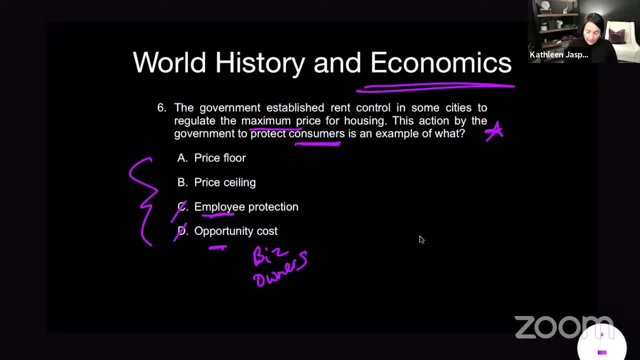 This action by the government is to protect consumers. Now, if I have a place where Rent can only go this high, What do I have? I have a price ceiling that's going to protect the consumer, right? In fact, they had rent control in New York City. 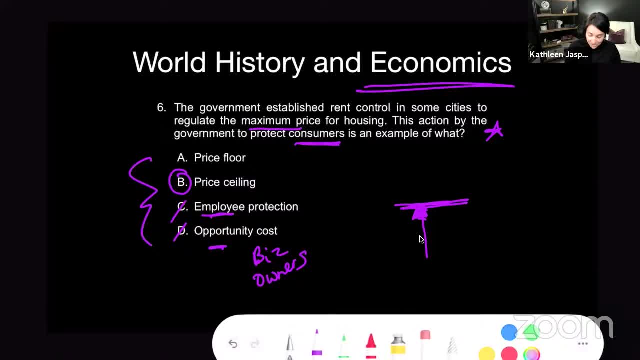 If you got a rent control apartment back in the day. I mean you're living in New York City for very, very cheap, right? So they don't have those same protections now, but are the same type of protections. So this is the max number. 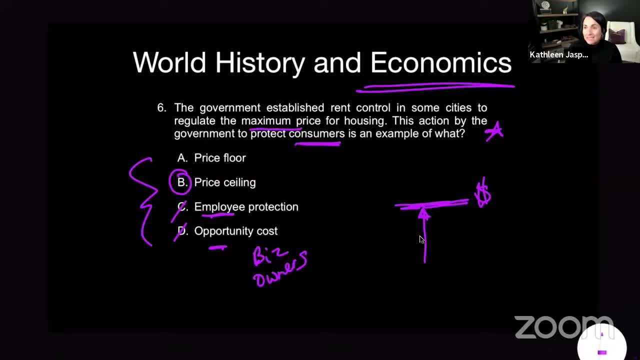 Let's just say. let's say, back in nineteen six, they did a price ceiling in New York City and you didn't have to pay. You could not raise your rent to any more than six hundred seven hundred and sixty dollars a month And you got it. you got in at rent control and you stayed there for 40 years, while. 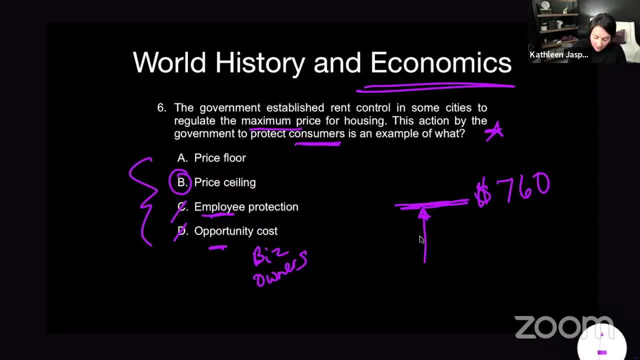 you're living. you're living the good life in New York City for cheap, And so you've got a price ceiling there. right now, A price floor protects the manufacturers, meaning that let's say there's some sort of economic situation, the price of something cannot drop. 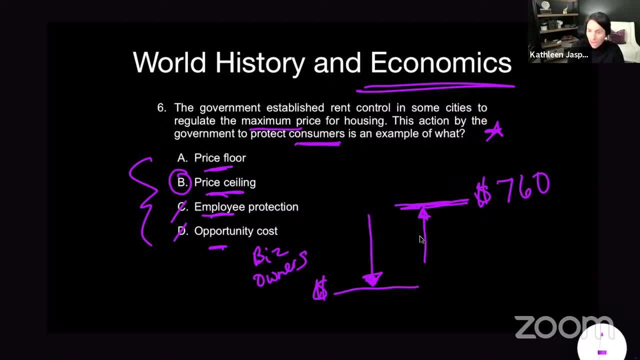 Any lower, then let's just say: I don't know the price of grain, but let's just say: a dollar, a bushel or something like that can never go below that. that protects farmers, that protects manufacturers. that's not what we're talking about here. 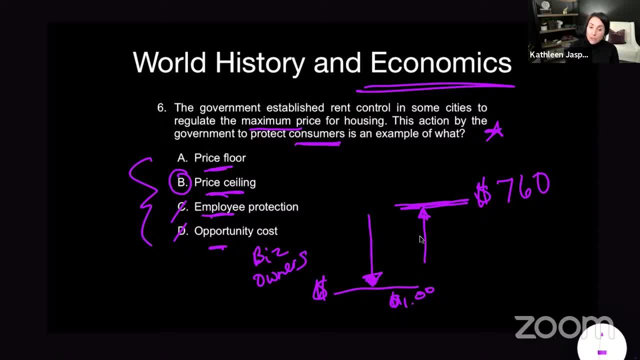 Now employee protection goes with unions and things like that, And then opportunity cost is about business owners. So let's say that I'll give you an example, my own example, for my own company. I decided that I was going to build my own learning management system where my, where my courses were, because I was 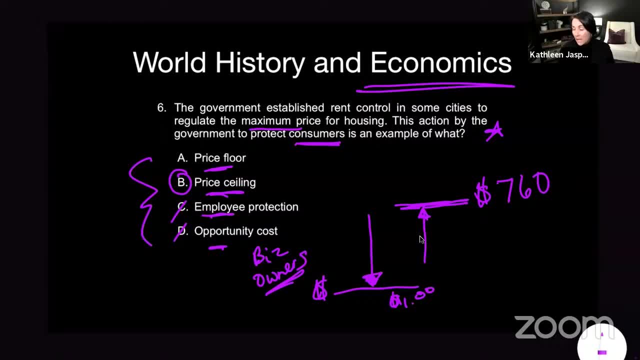 tired of paying this exorbitant fee for someone to house my courses. So I went looking for someone who could build me the elements that you guys use now when you're on my courses. Well, that was going to cost me a lot of money, but it was going to. it was going to. 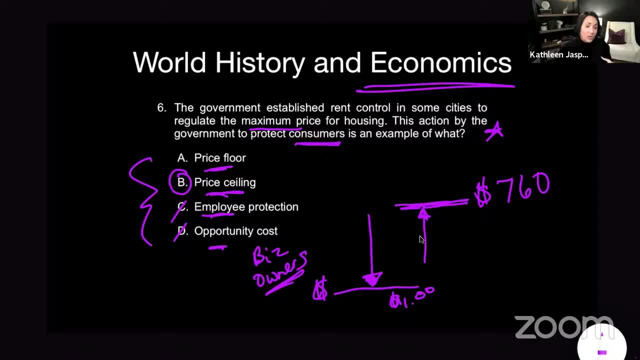 get me out from underneath a monthly bill. that was too much And I knew I would have more control over it. I could add things and make things. so the cost that it was going to Put on my business was actually called opportunity cost, because I was spending that money up front in order to make some. 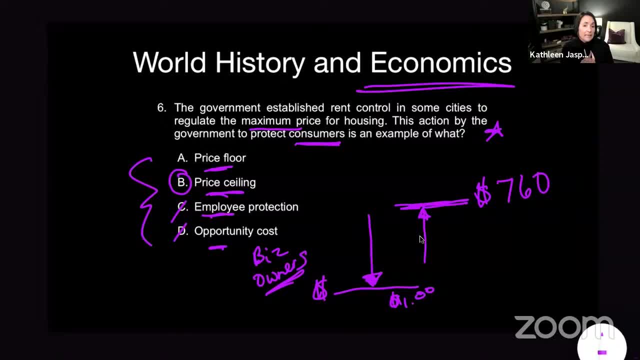 money later or save some money later. another example would be like: OK, if you own a restaurant and you want to build a bigger parking lot, But in order to do that you have to shut down your restaurant for a week or a month. 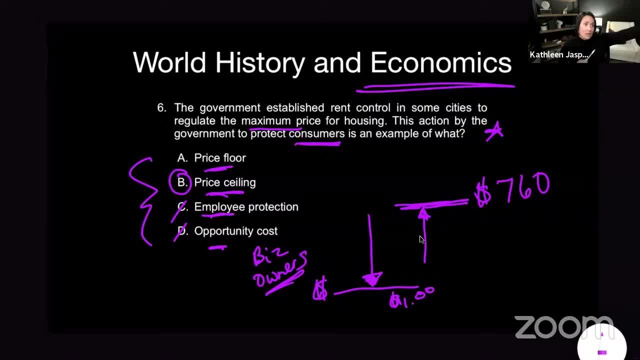 And you know that if you do that or you have to shut down half of your restaurant because they're going to be over there working or whatever. But in order. but when you do that, there's more parking, more people can come. whatever, you're going to make more money. 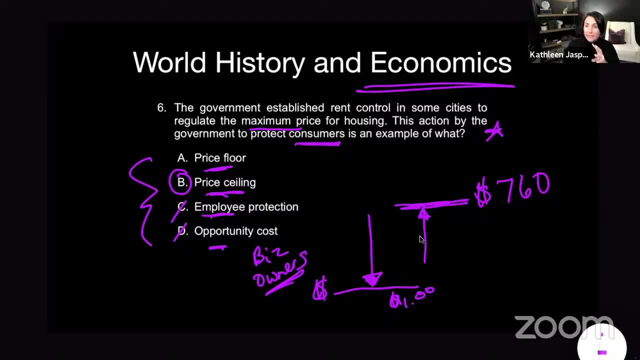 So there's a cost in the beginning, but it gives you an opportunity to make more money in the end. And then, finally, another example would be this. Let's say I said to you: OK, Sally, you can either get the video game or the bicycle, but you can't have both. 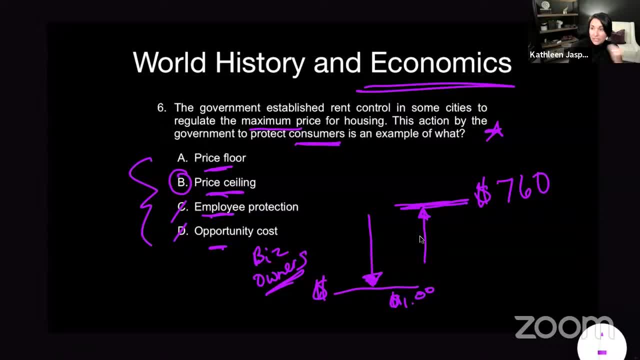 The opportunity cost would be: if you got the video game, the opportunity is the video game, the cost would be the bicycle, and vice versa. So there's a couple of different ways it might be presented on the test. Just know that there's a cost, but there's. 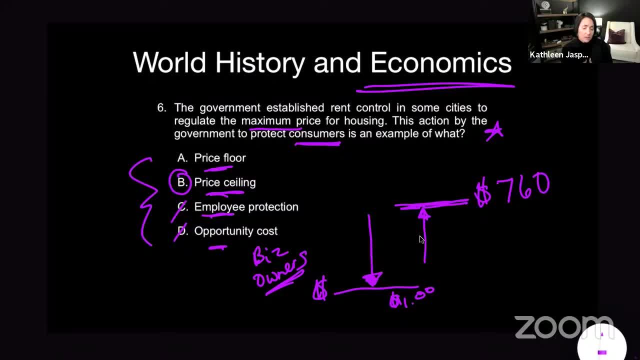 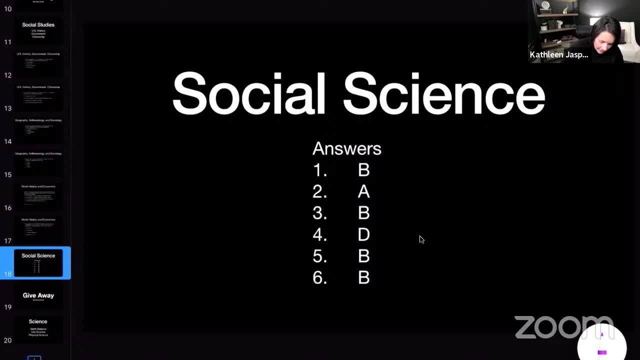 also an opportunity that you get from from taking that cost on. All right, All right, So that should be good. there There's the answer: choices. Now let me go to. I'm going to do a giveaway. Give me a second on that. 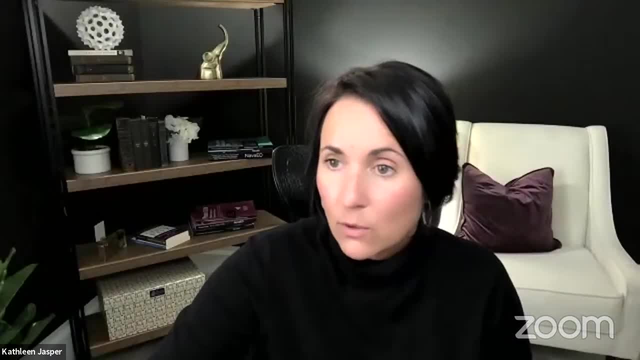 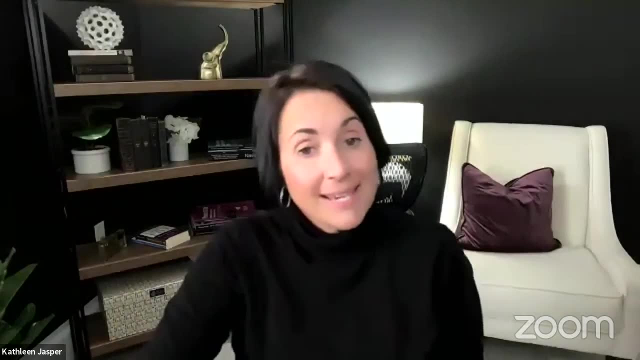 But I just wanted to show you guys first. I want to go into the chat really quickly and see if anybody Has any questions. I thought the math portion had scenario type questions. It does, If you're taking the 7813,. that's all math scenario teaching questions. 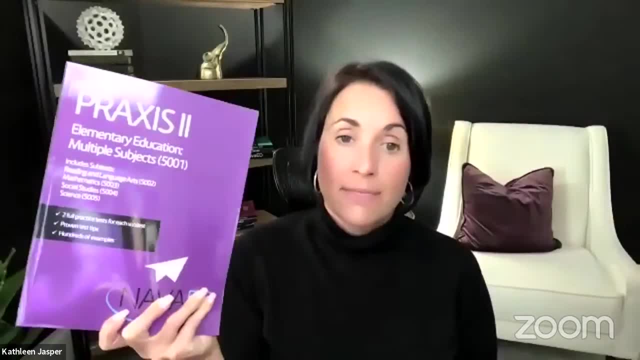 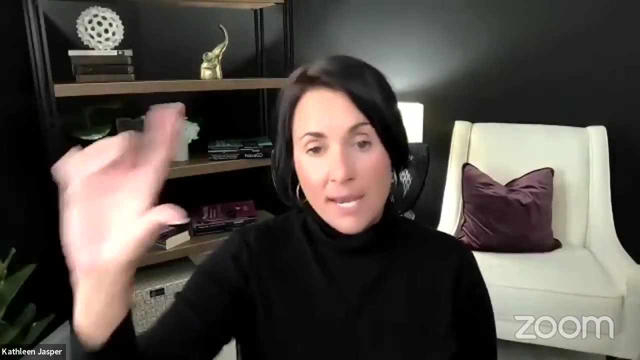 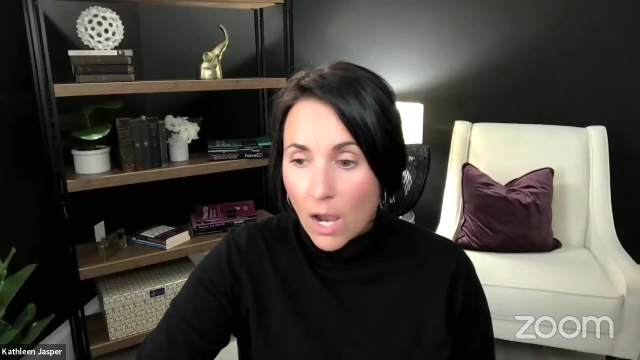 But this math 5003 is straight up math, So that's why I did that today. But you may have teaching math questions. Typically it's a combination of your understanding of the math but also the teaching of the math. So no, 5001 is not only math scenarios. 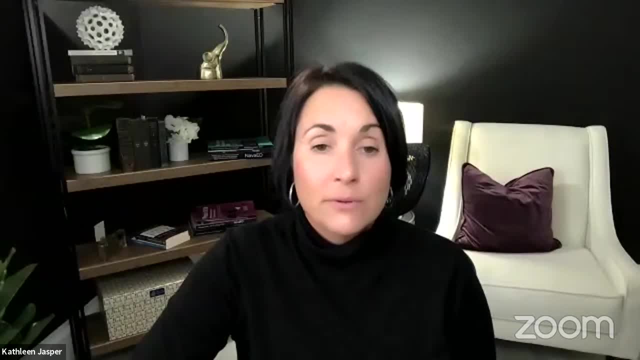 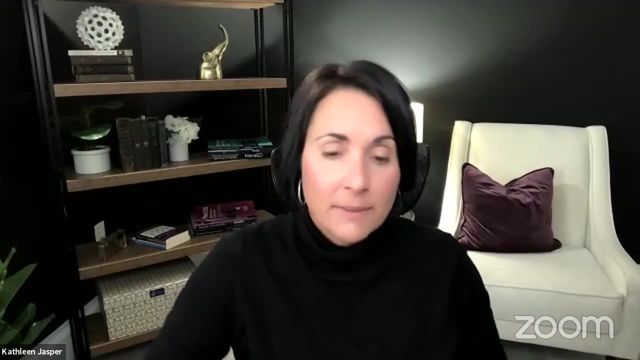 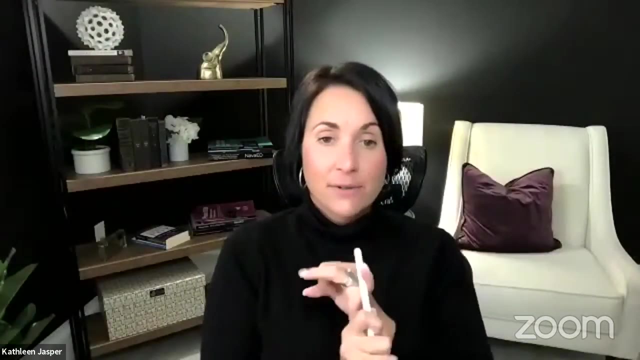 7813 is, and 500, I believe it's eight- is the new math test- is a new test. But 5001- let me explain this to you guys- 5001 is the whole entire elementary education test. Then we have 5002,, which is a subtest. 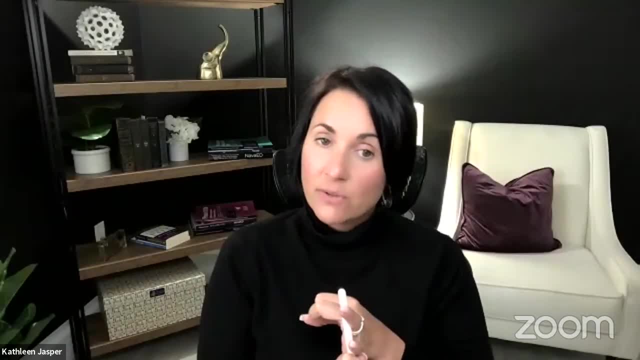 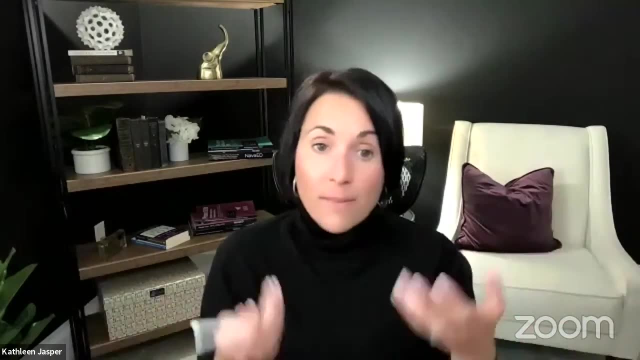 That is the English language, arts and reading. Then we have 5003, which is the math only 5004,, which is the social science, and 5005, which is the science. Now you take all of them at once, but let's say you pass one or two. 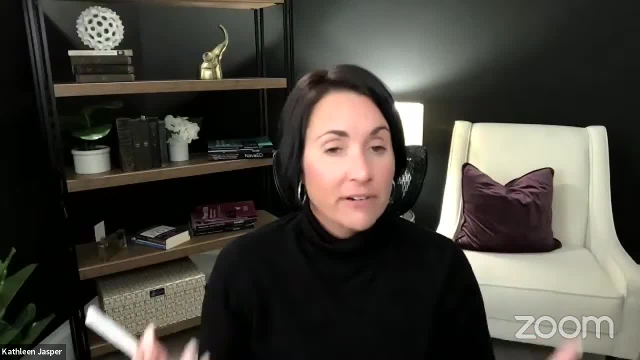 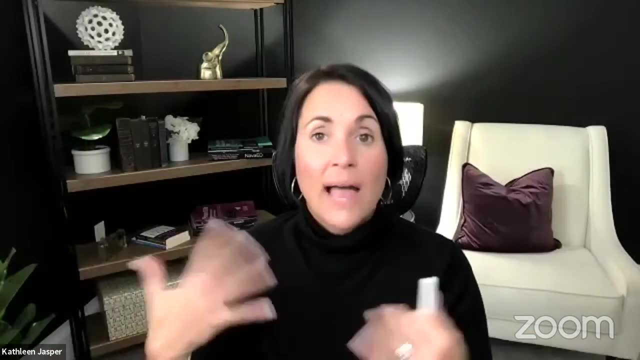 Then you go back and only take the sections that you didn't pass. That's very similar to a lot of elementary ed tests out there. Some elementary ed exams for math will have teaching math scenarios, But the 5003, according to the test specs. 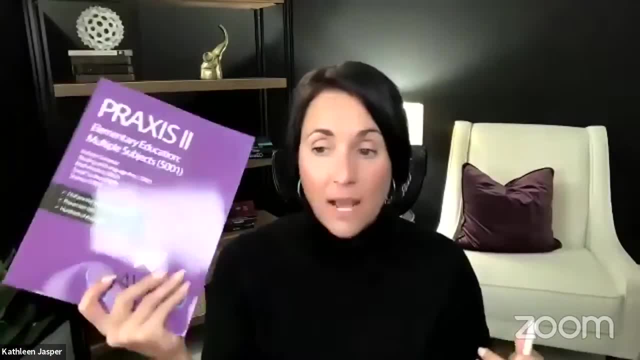 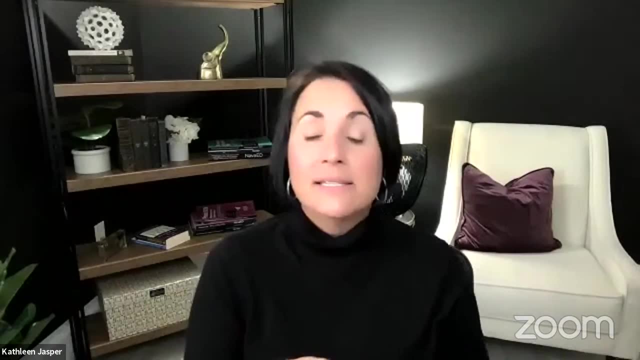 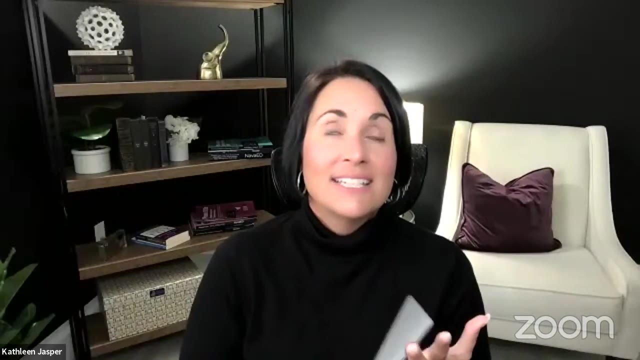 and the sample questions I have seen on the exam. it's straight up math, So you have to know all of this. OK, 5903 is very similar to 5003.. So you're talking about the 5901 or the 5901, which is it does not have. 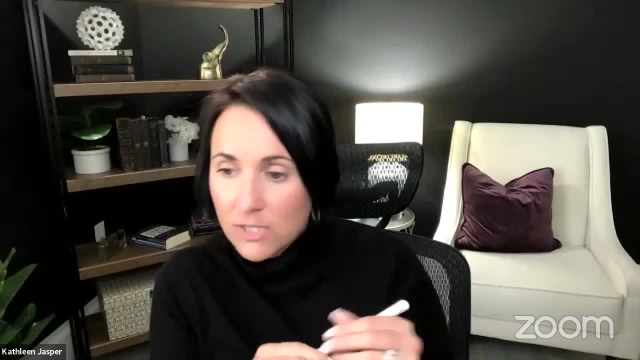 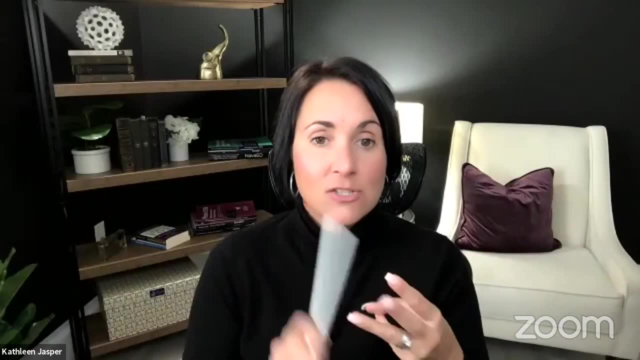 the English and language arts you are probably taking. So this is. Ms Morris, You asked about the 5903.. That is for people who it's math, science and social science, But then they make you take the teaching reading, which I do have a program for that. 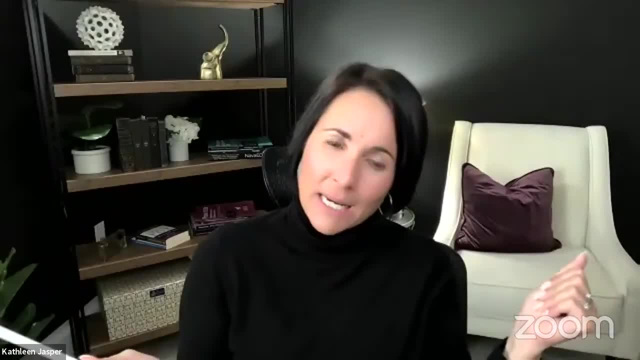 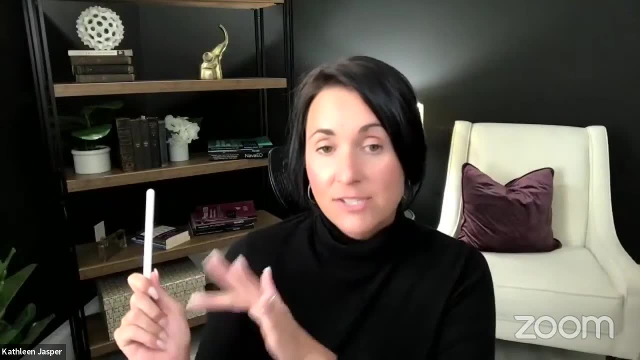 So you have to still do the reading. It's just on a separate test so they can make more money, and it becomes more complicated. So, yeah, so we have that as well, But it's going to mirror. if you look at the specs, it mirrors the 5003,, 4 and 5.. 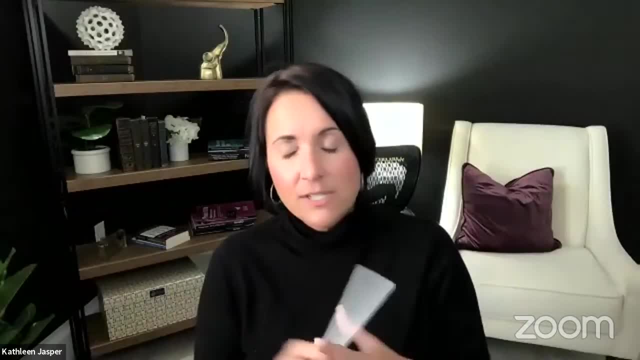 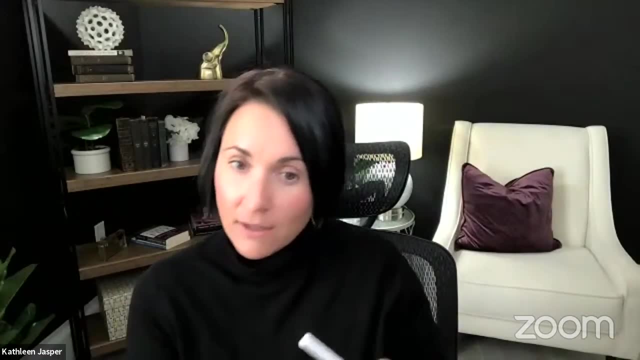 So you're good here with us today. OK, you may have some differences, but for the most part it's 503, 4 and 5.. Yours is 5903, 0405.. OK, I know it's complicated. 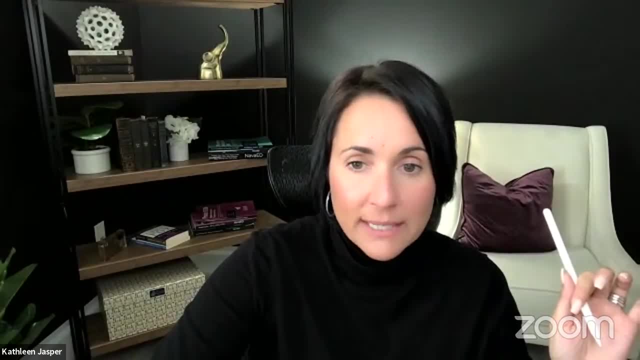 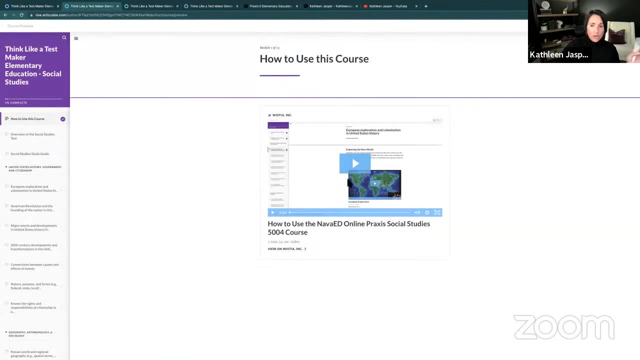 They, they name their tests, all those things. Now, really quickly, I want to show you a couple of things about our social science resources, So let me just take you into here again. If you're somebody who struggles, this has got tons of information videos. 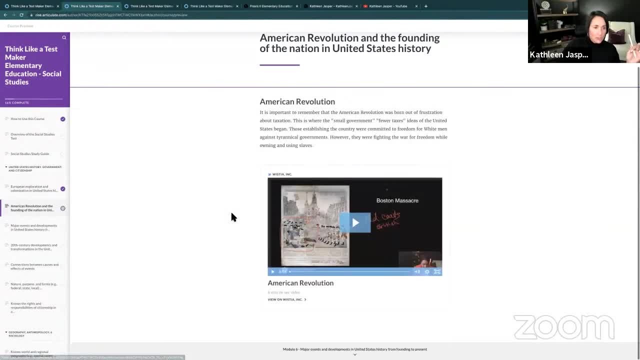 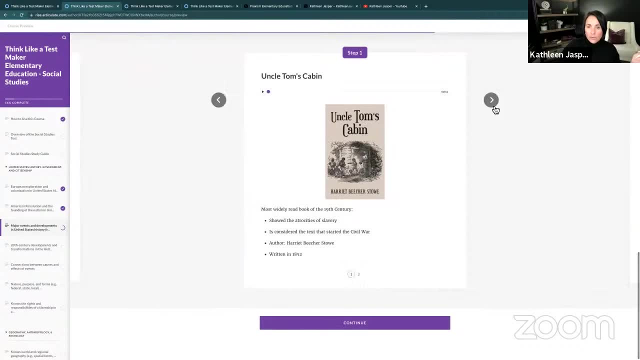 We've got ancient civilizations, We've got the American Revolution, We've got, you know, all the timelines and all these different things going on. I've got audio stuff here. I've got so much. This course is huge and you can see we go through everything. 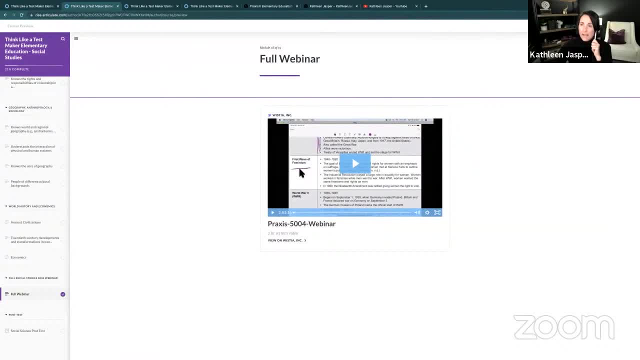 There's also a full webinar. This is a good one to use as a as a audio course. If you're one of those who likes to listen to your courses, then of course we have a post test. It also comes with the online book. 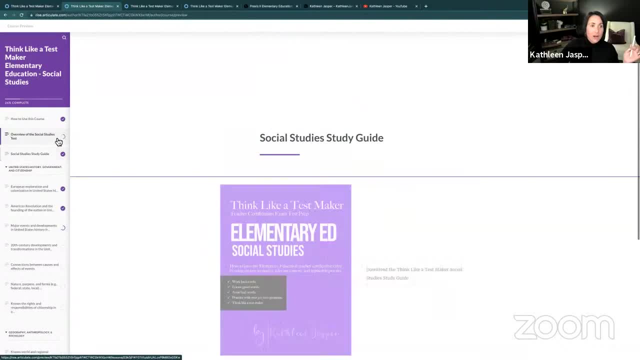 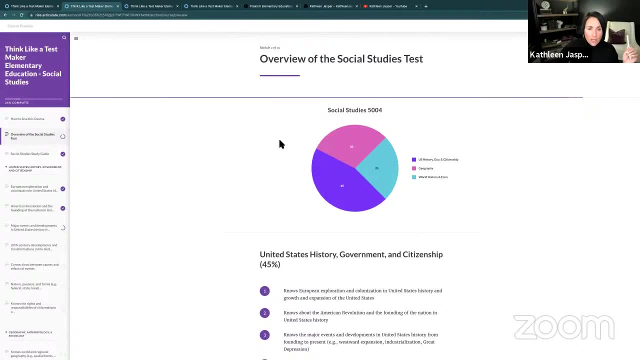 You can see here the study guide. You get to have the study guide there, So really important there Also, let me just show you, let me new share. Let's go to the book. really quickly, OK, really quickly, wanted to show you the book. 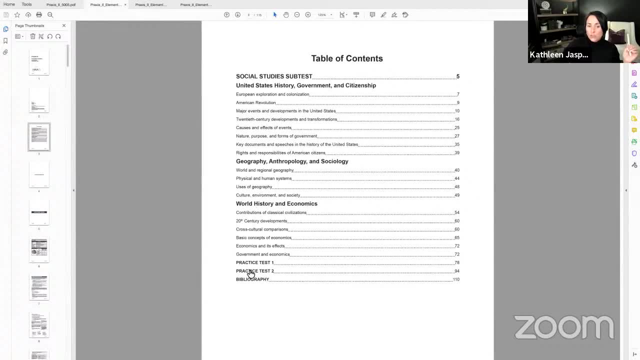 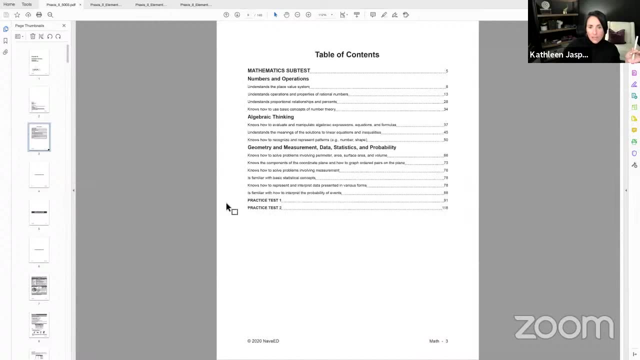 Notice it's broken up into All of the categories. here two full practice tests. Same with math. Math had the practice test as well. Let me go here. Math had two full practice tests. The social studies has two full practice tests. 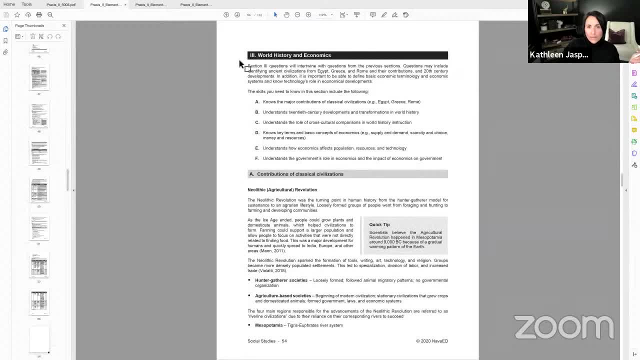 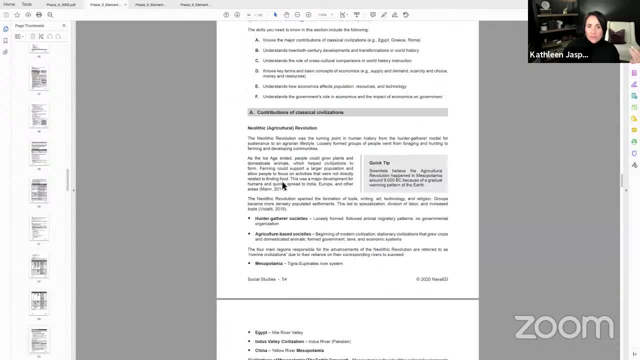 And you know, there's so much information here and we have the specs, We always have the specs you can see, And then each heading is the spec, so that we go right to the Neolithic era, all the way up to modern day, you know. 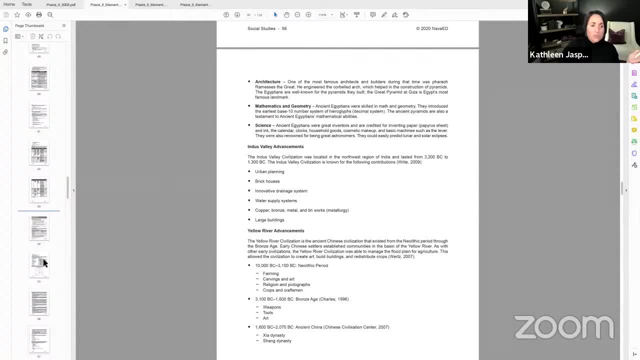 Afghanistan. I think it goes up to Desert Storm, which is what the test does. So you can see it here. We're in Mesopotamia. I'm reading a lot about Mesopotamia and stuff. It's very interesting. 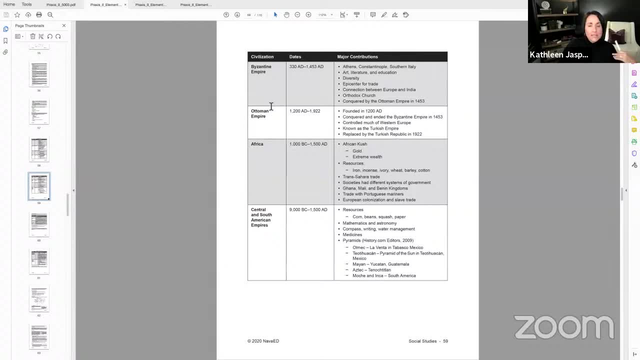 And, of course, I've got tables and things for you to to understand this portion of the test. So really good, It's in the physical guide, but you can also buy the digital on its own And remember that the online courses come with that digital study guide here. 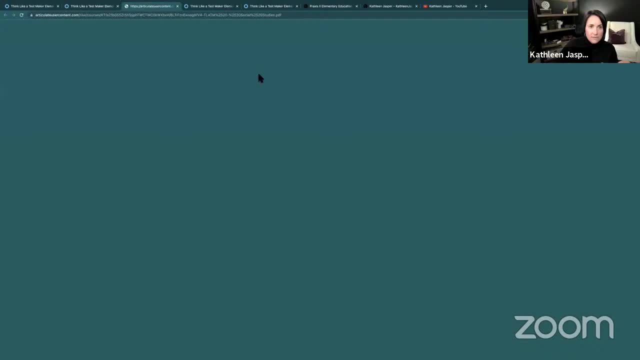 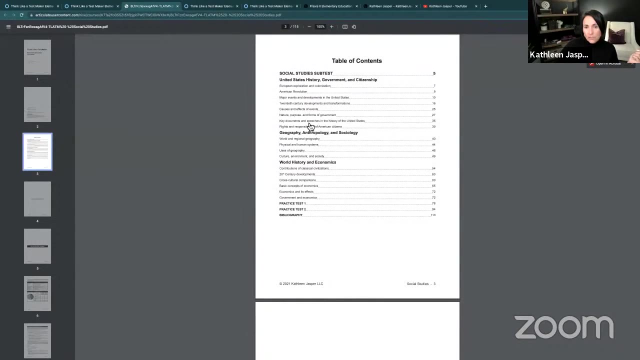 Right here. You just download it and it pops up and you can save it to your. you can save it to your computer and go through it And it's hot linked so you don't have to scroll. You can just click where you want to go. 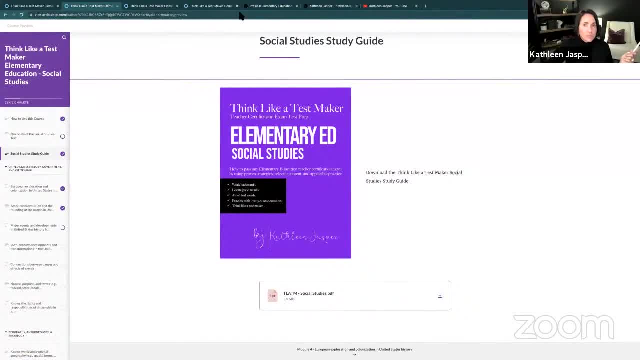 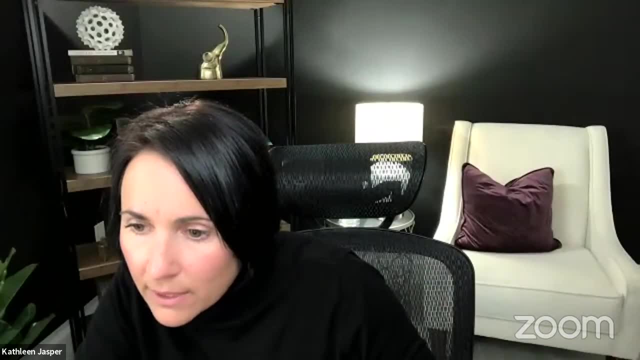 All right, Very important there. OK, I'm going to check the chat one more time. Let me stop sharing here. OK, looks like let's see. OK, still OK to use Perfect Right. right, right, OK. 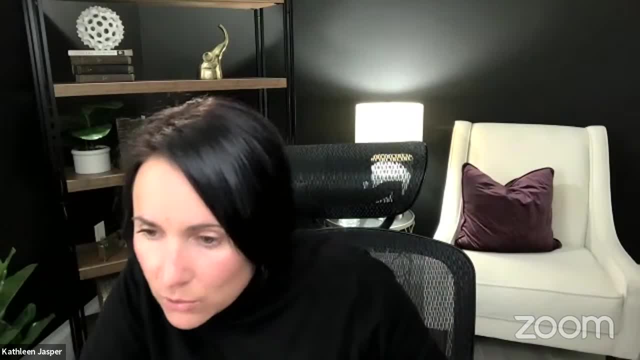 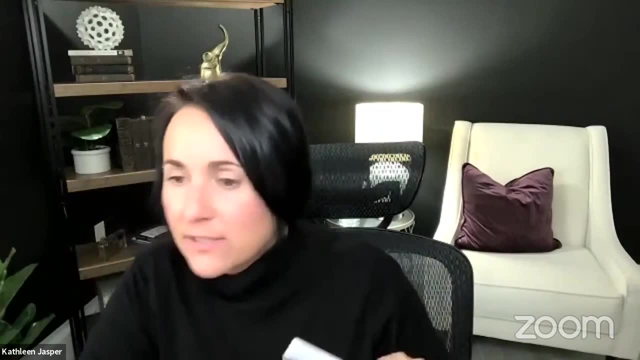 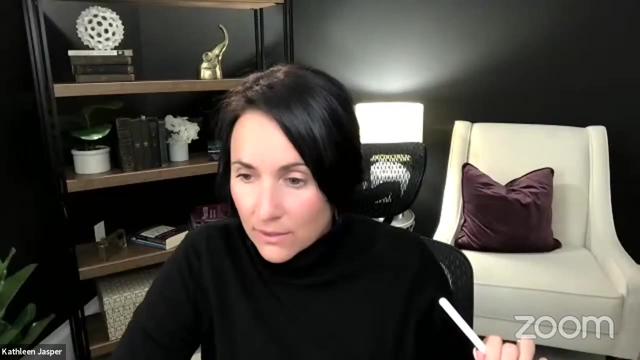 All right, All right. So now I'm going to go to my random generator here. OK, somebody's asking about the practice core in the chat. This is not the practice core. This is the elementary at the practice core is the basic skills test. 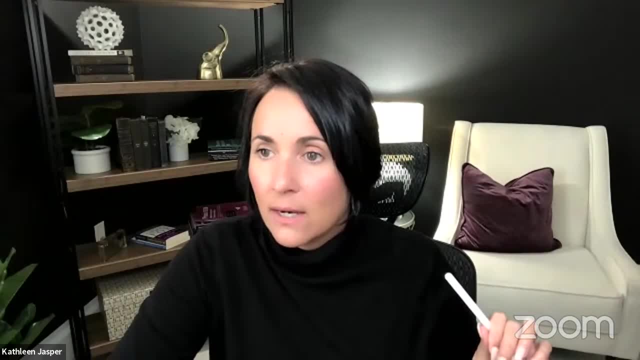 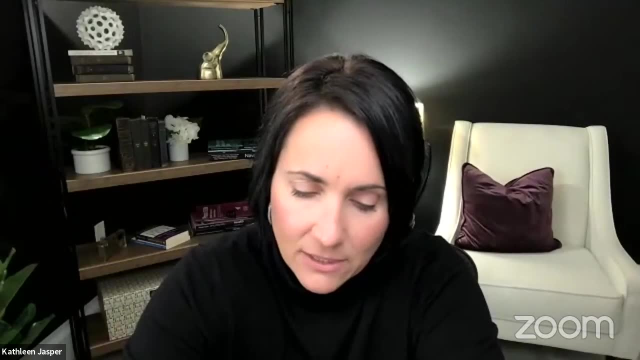 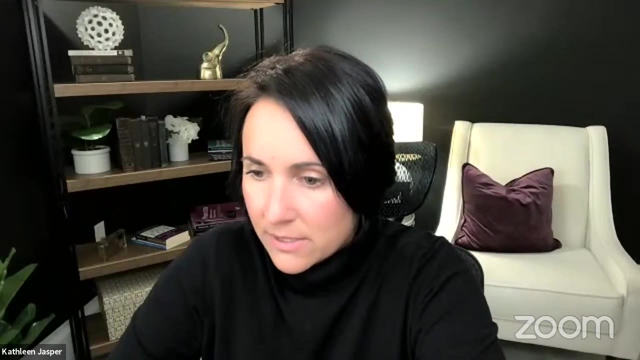 OK, All right. So let's go in here and I'm doing my random generator. Let me just write down the name. All right, I've got Destiny Jackson. Destiny Jackson, are you here? Let me know in the chat if you're still here with us. Destiny Jackson. 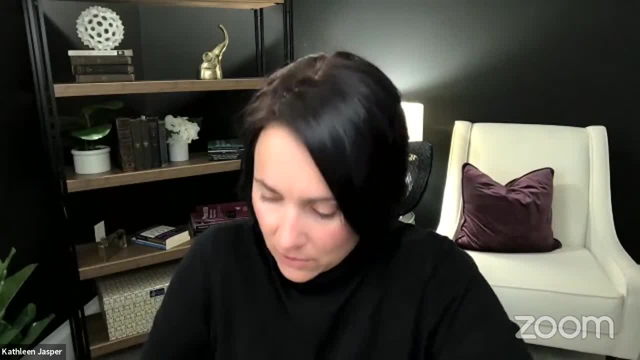 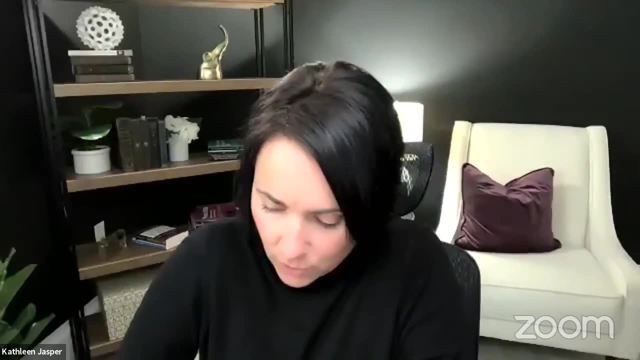 All right, Destiny, you have fifty dollars coming your way. Let me make sure, Destiny Jackson, nice job, Fifty dollars store credit coming your way. Be on the lookout for an email from me later on today, before the end of the day today. 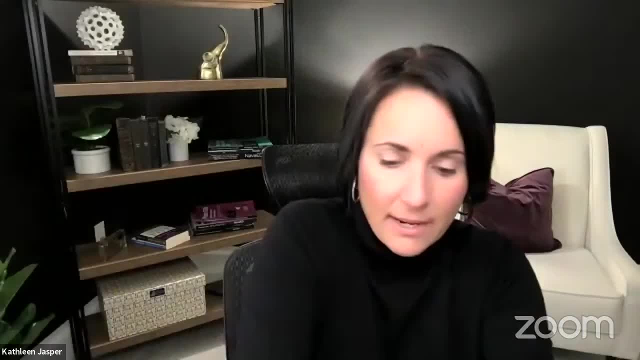 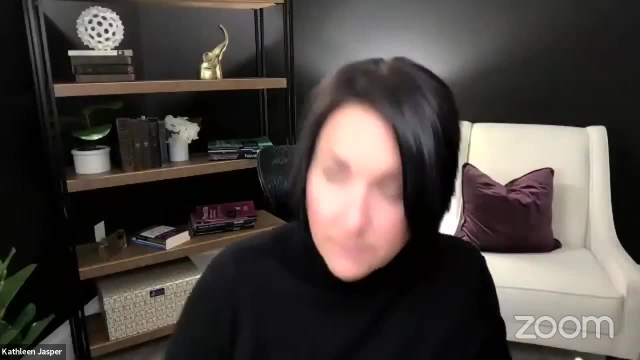 Congrats guys. Good job, All right. OK, good job, OK, so that's it. Now let's go to science. What time is it? OK, I'm kind of on time. I figure it's going to be about an. 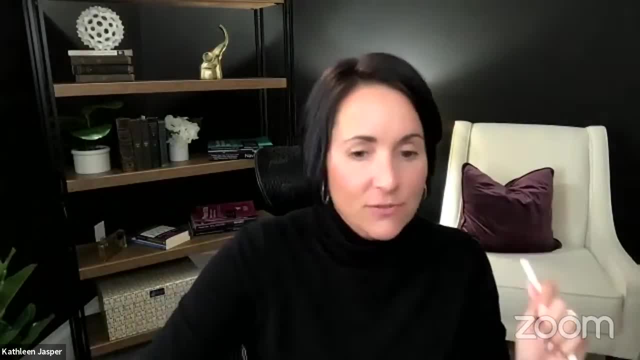 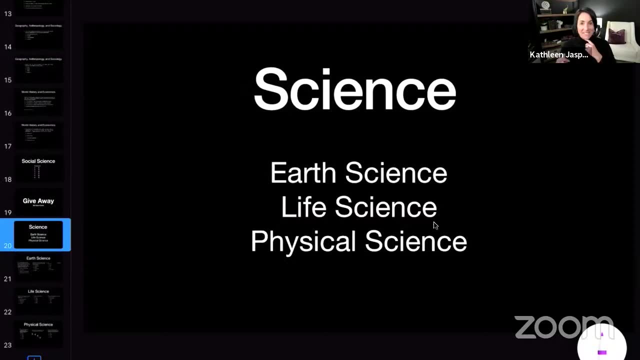 hour and a half to two hours. It's a big test. Good Thanks for sticking with me. guys, I'm actually moving quite quickly. I'm usually longer winded If you've been on my courses, I usually talk a lot more, but I'm trying to keep it. keep it, you know succinct. 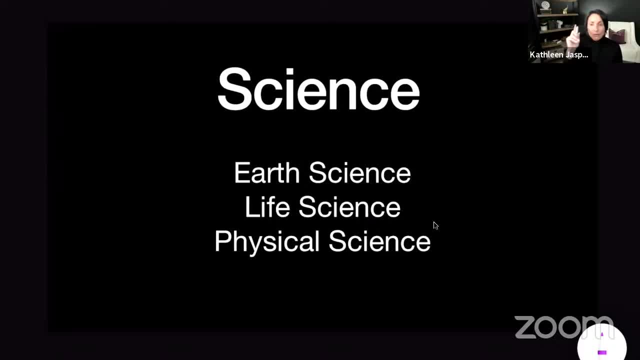 Less is more Right. All right, So we're now. we're in science And remember every science exam- and this goes for the high school, and the middle school is going to be broken up: Earth, life, physical as you get up in the grades. just a little side note here. 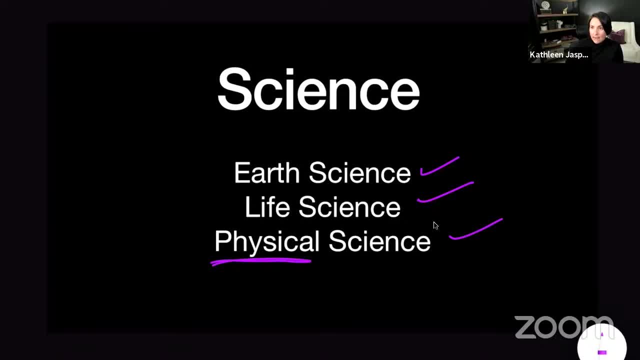 Physical science might be broken up into chemistry and physics, but on the elementary ed they're combined Right. So Earth science is going to be that, that kind of question about the Earth rotation tilt on the axis, the stars, the moon, the sun, all of that kind of stuff. 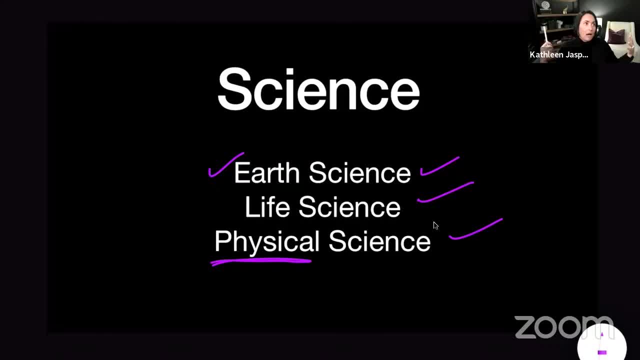 Gravity, also systems like the water cycle and the atmosphere, anything that has to do there, and the crust, Canyons, rivers, all of the stuff on Earth, the lithosphere, the core, all of that type of stuff. OK, then, life science is bio. 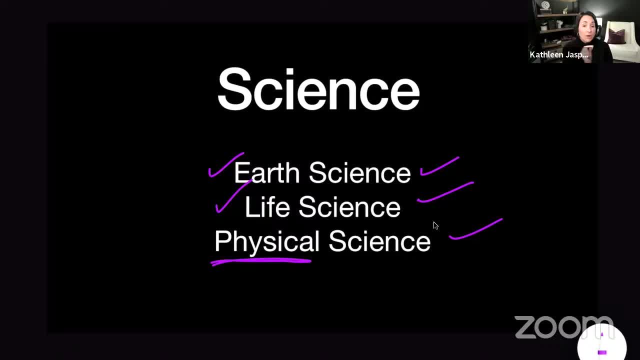 So it's going to be everything from the cell and even the organelles, So DNA getting even smaller, Right DNA nucleus, ribosomes, RNA things. I don't know if they'll ask you about RNA. That's a little bit more advanced than moving out into. 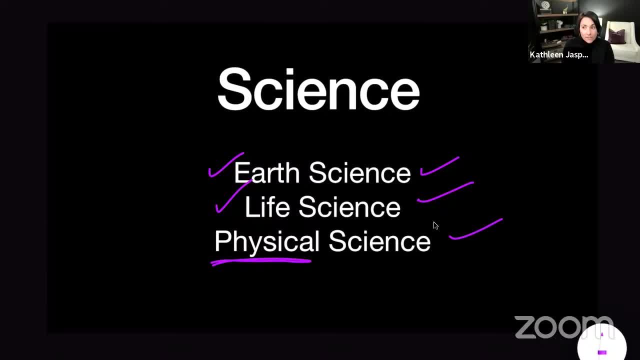 tissues and organs and organ systems and then the organism. So we're going to go with cells and then tissues, What those cells make up. then organs: They'll ask you about the heart, the kidneys, the simple stuff, the liver. They won't ask you about, like you know. 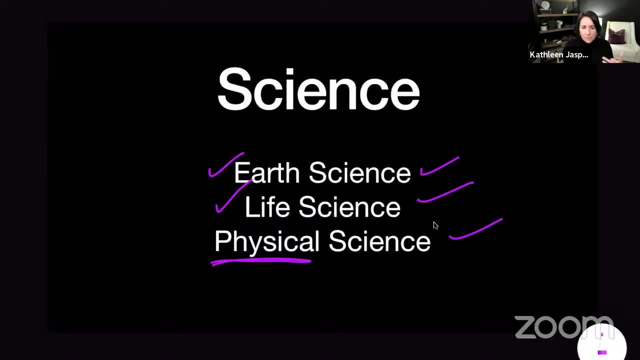 you don't have to have an MD in order to to to pass this, But they will ask you some stuff there. Then they'll ask you about the organism as a whole, which might be a human organism, or it could be a grasshopper or a. 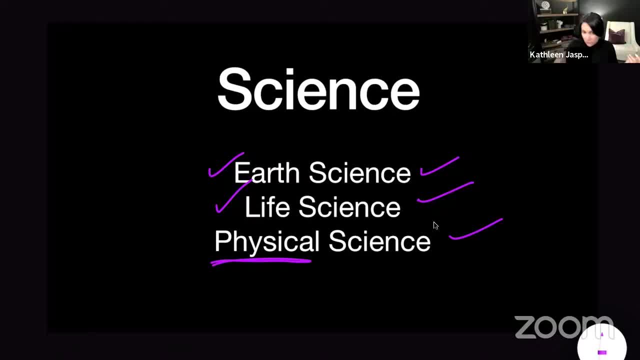 lamb or a cow, or vertebrae versus invertebrates, those types of questions, And again, if you haven't seen a science test in 30 years- invertebrate versus vertebrae, versus open circulatory, closed circulatory- you might want to brush up on those for sure. 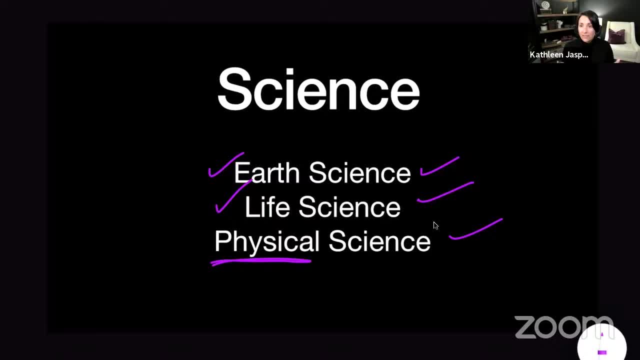 And then it also includes ecosystems, So all the living things within an ecosystem, So plants, nutrients, predator prey, that type of thing. Then physical science is going to be physics and chemistry, So we're going to be talking about atoms and electrons and protons. 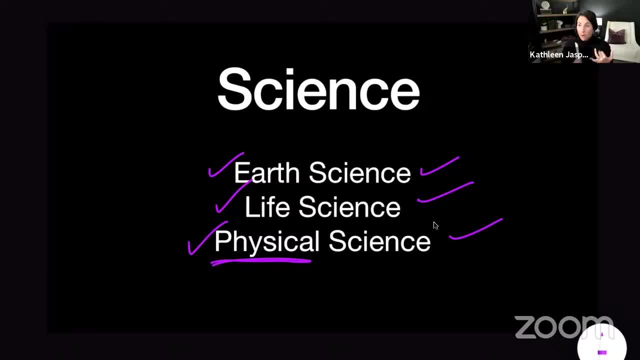 We'll be talking about matter. We're going to be talking about density. We're going to talk about energy, kinetic versus potential and all that: physical machines, different physical sciences, all of the physical world, chemistry. you might have a little bit of the. 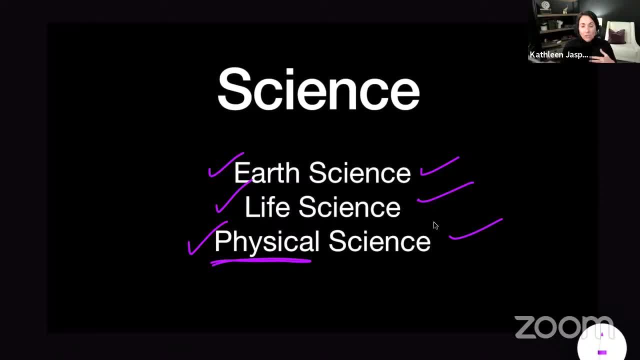 which one is more acidic and which one is more basic. So you'll have that, that chart acid versus bases, And there will be something on there about molecules and compounds in the periodic table. You might have a little bit of that, So just keep all that in mind. 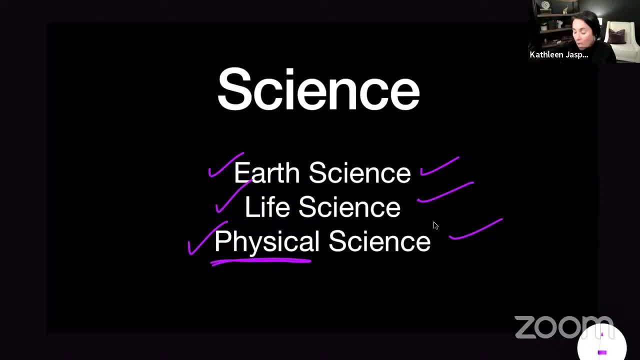 Of course, it's all covered in our book and on our online course, But every science test is broken up this way. Again, I see some people raising their hand. I can't see hands being raised when I'm sharing screen, So go ahead and throw your questions in the chat. 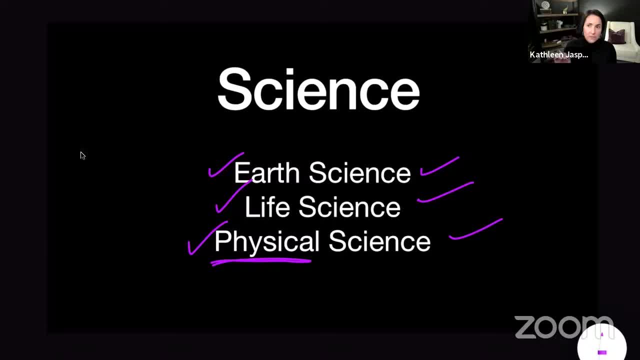 I'll check that really quickly. If you do have questions about this, please throw it in the chat. I cannot see it If you're raising your hand as I'm sharing screen. All right, So let's talk about Earth science really quick. 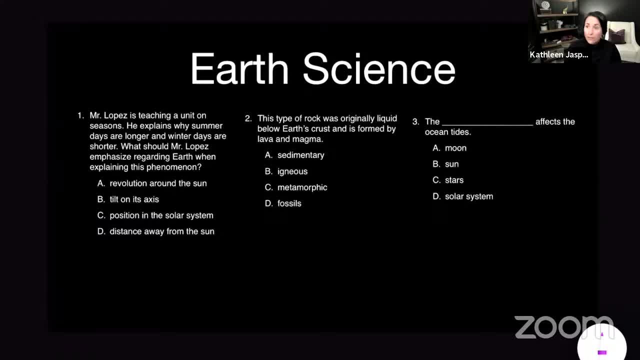 I've got three questions that have to do with Earth science. Remember, this is all about the Earth and the sun, and the moon and the stars and all the galaxies. All right, So again, starting with the answer, choices here: revolution around the sun. 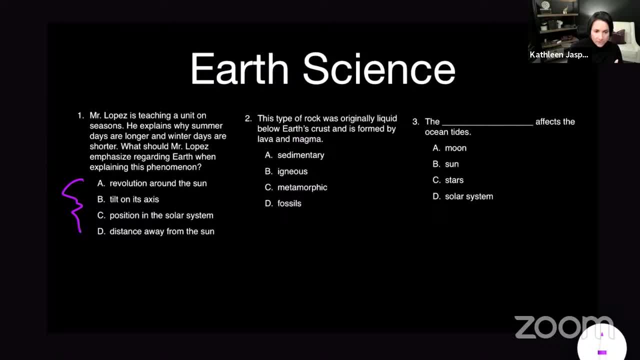 All right. Tilt on its axis, All right. Position in the solar system, distance away from the sun, All right. Well, C and D are kind of the same, And remember it's multiple choice tests, So some things are too similar. 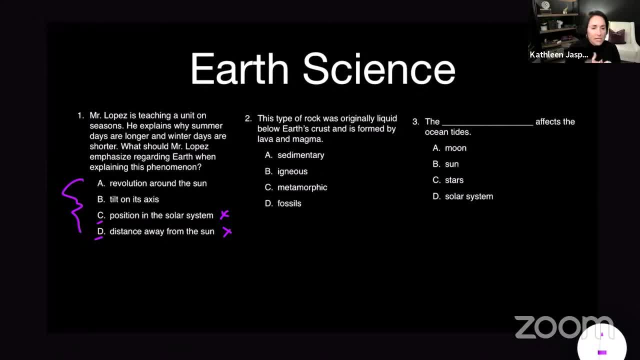 They're probably not the answer, But let's just take a look at the question. Let's go with the question stem, which is right here. What should Mr Lopez emphasize regarding Earth when explaining this phenomenon? Still don't know. Got to read the whole thing. 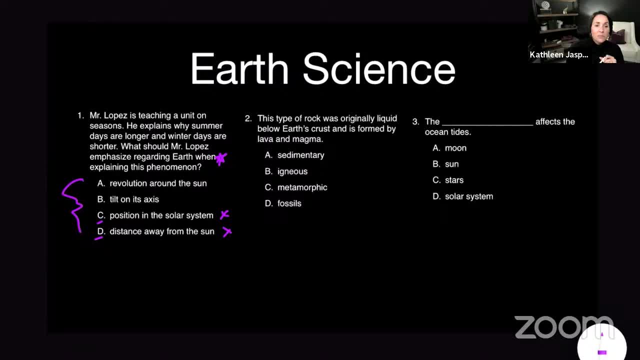 Mr Lopez is teaching a unit on seasons. He explained why summer days are longer and winter days are shorter. I should have put in the northern hemisphere, That would have made it a better question, but Mr Lopez is probably In the United States. 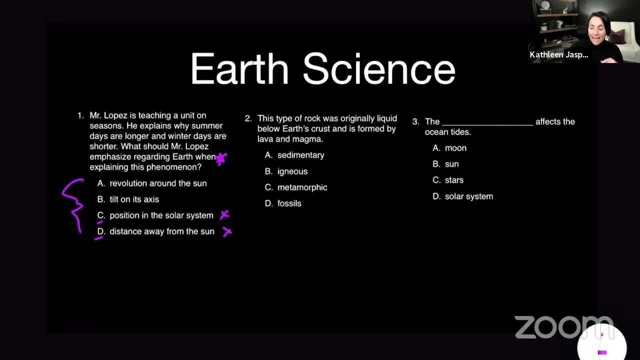 And so, talking about that, what is that? That is going to be the Earth's tilt on its axis. The reason why let's just do a quick little. Very, here's the sun, All right, And here's the Earth, and it's tilted on its axis. 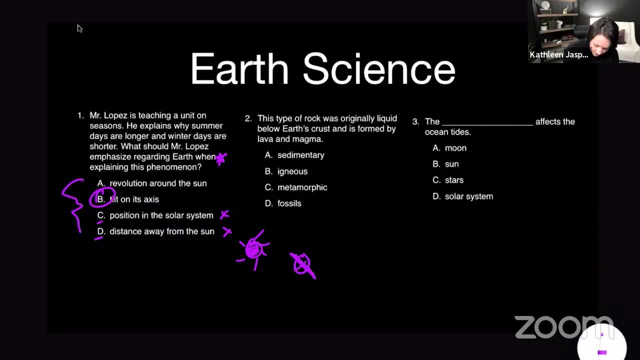 And so during the summer in the northern hemisphere, let's just divide this Earth by our equator: this is north and this is south. in the northern hemisphere During the summer- It just happens to be during the summer months- The northern hemisphere is tilted towards the sun as it's going around the sun. 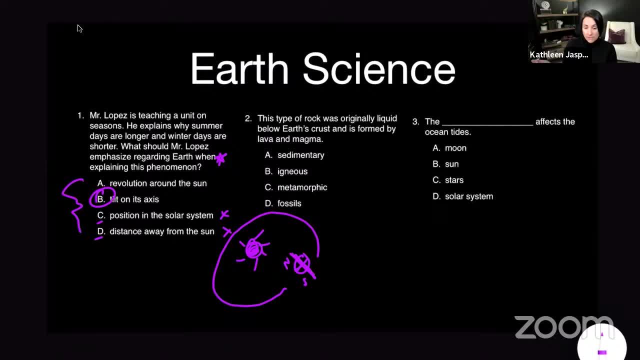 Right. And so in the northern hemisphere in the summer we have longer days. in Alaska Sometimes it's 24 hours of sunlight, which is really crazy. Anybody in Alaska from here do you experience that? And then, as this moves over back over here, we actually have it where. 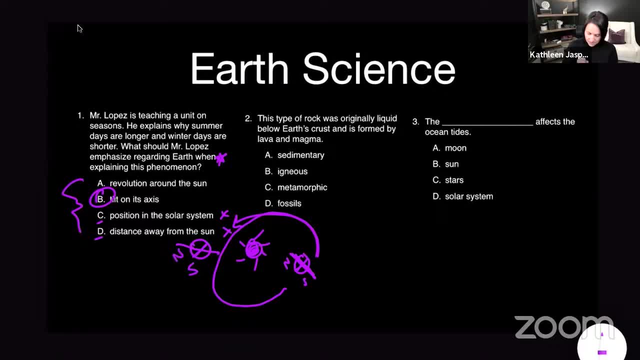 The southern hemisphere is tilted towards the sun Right, So during the winter in South America and Antarctica it's going to be longer days. so that is all about the tilt on its axis. If you see seasons, we're talking about the tilt. 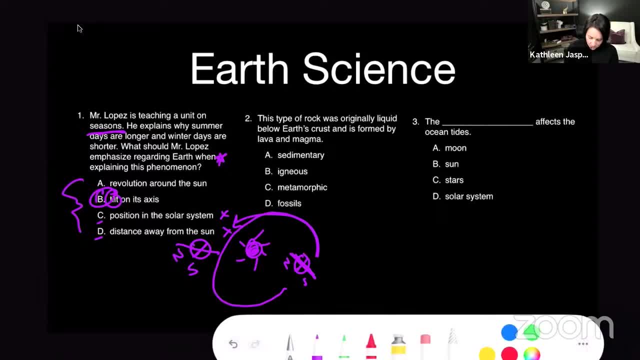 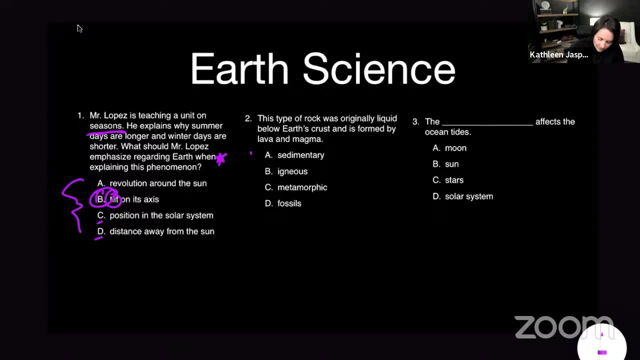 We're talking about the tilt there. All right, I'm going to erase this terrible picture of the phenomenon for you guys. All right, Let's go to the next question. I've got types of rocks here right away. I know I'm going to be looking at four rocks. 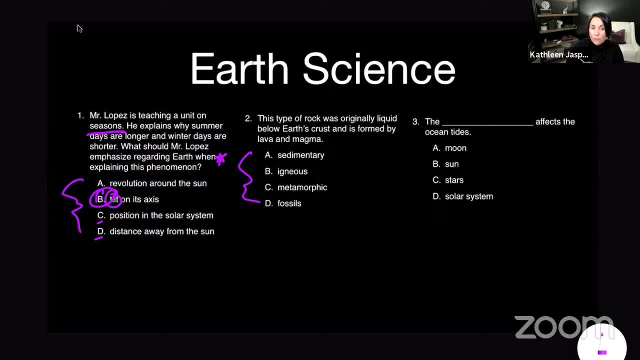 This type of rock was originally liquid below the Earth's crust and is formed by lava and magma. Lava and magma is igneous, Think granite countertops. You can kind of see in these rocks where the lava flowed and all of that Sedimentary rocks are made up of sediment. 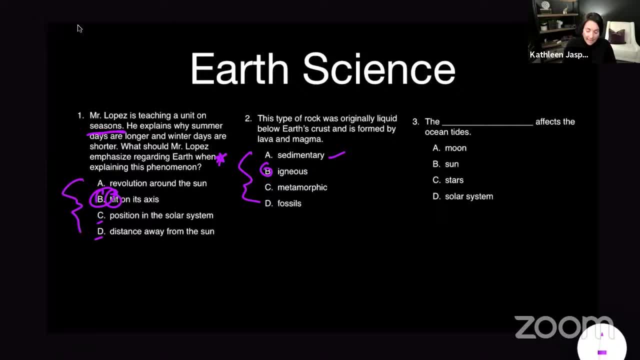 coming together over and over again over time, forming a rock, And metamorphic rocks look like crystals. They're from heat and pressure, And so crystals are metamorphic rock. But in this case we're looking for- and fossils are preserved, preserved organisms and living and nonliving things in rocks that tell us. 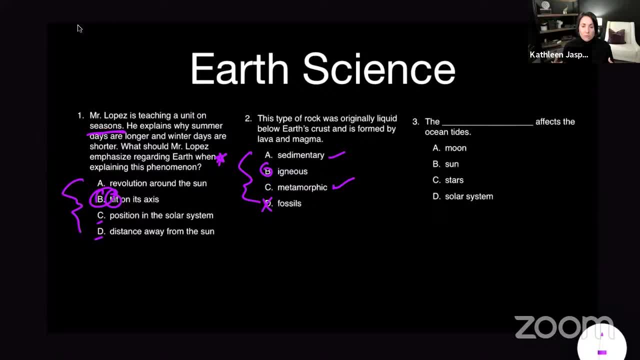 a story about the history of the rock or the history of the time in which the rock was found or which was made. but igneous is lava and magma, So always know that there's a chart in the book that'll help you with that. 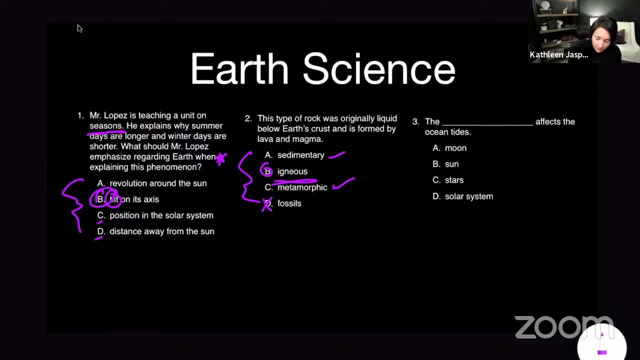 That's an easy one And you will definitely get something about rocks And notice we're talking about the Earth's crust. So this is earth science. Want to be able to think about that when you're getting these questions. Number three: the blank affects ocean tides. 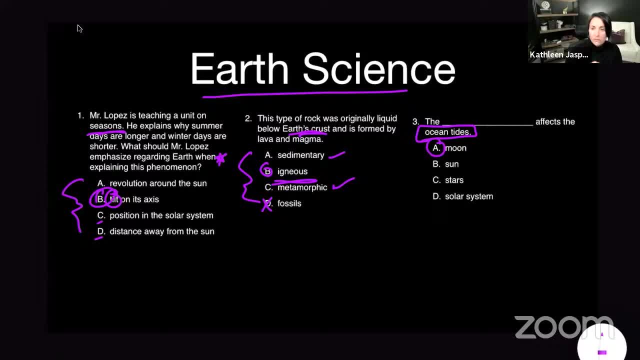 Ocean tides are affected by the moon. All right, You may need to know phases of the moon for this exam, but you will probably be asked one or more questions about the moon and we get into the moon and lunar eclipses and things like that in the book. 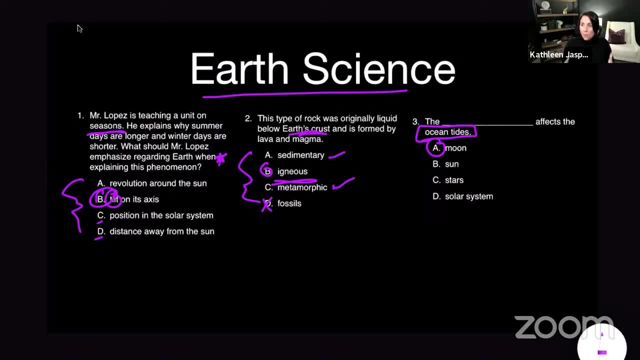 So these three questions are typical earth science questions. All right, We had a little bit of the Earth's crust, We had a little bit of the tilt on this axis with seasons, and we had a little bit of the moon. There are all kinds of other things. 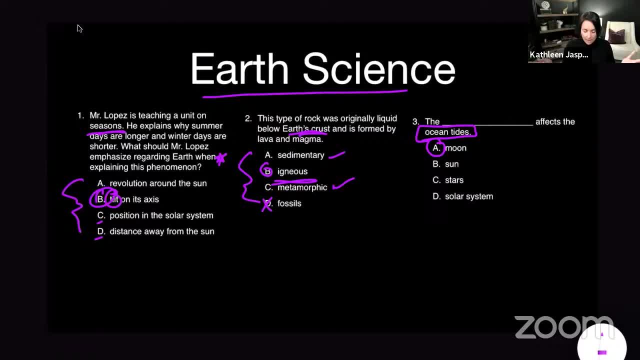 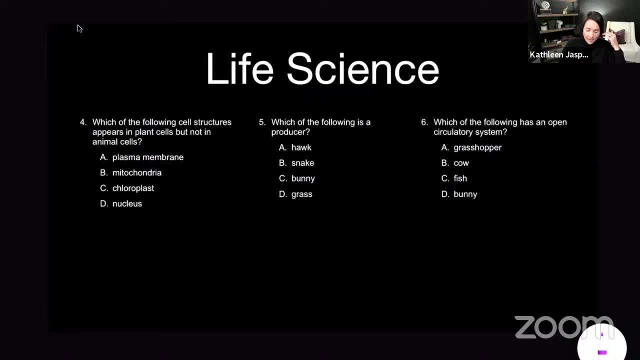 Earthquakes would be in here, all kinds of stuff like that. OK, it's fair game Again, knowing the specs are going to help you with that. Now, life science is all bio. Life science is bio, So let's take a look here. 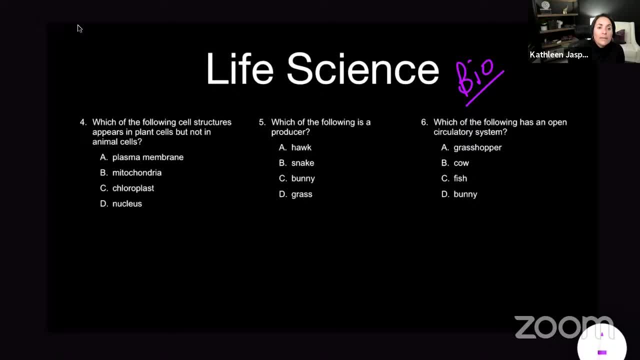 Number four, which of the following cell structures appear in plant cells but not animal cells. So you're definitely going to need to know the The difference between plant cells versus animal cells. that's definitely going to be a theme in the life science and in plant cells. plant cells have chloroplasts. 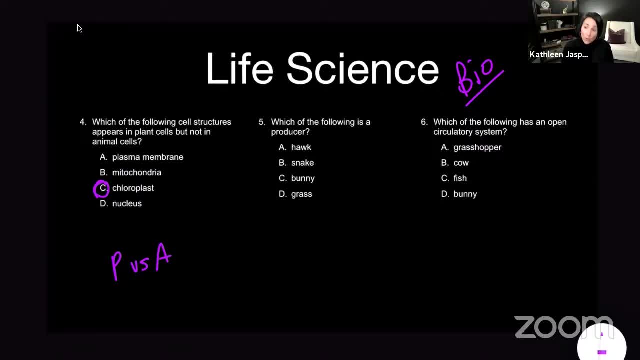 which help to process the chlorophyll and the energy in plants. Both have plasma membranes, both have mitochondria and both have nuclei. The only thing that's different is a chloroplast. Animal cells do not have it. Another difference is a cell walls. 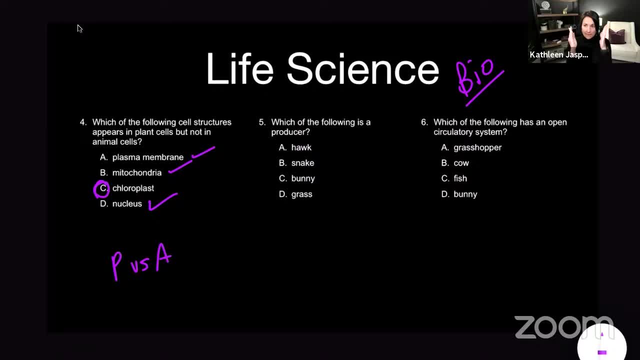 Plant cells have a cell wall. Animal cells do not, because plants have to be rigid Right And the cell wall helps to make them rigid. When you bite into celery, you're biting into the cell wall, or many cell walls, I should say. 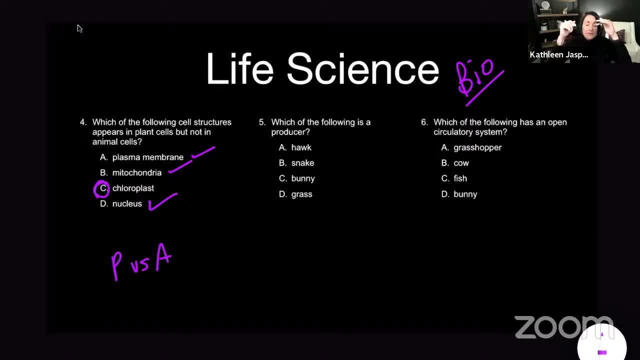 They all have a plasma membrane around, But then the the, the plant cell has another layer of cell wall there. And then the nucleus. all, All cells have a nucleus. Except single cellular organisms, No eukaryotic cells- all have a nucleus. 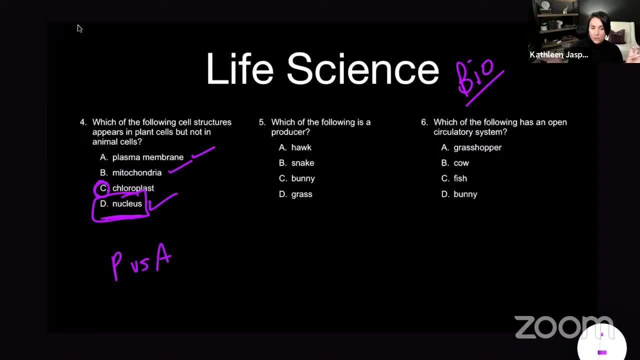 Prokaryotic cells do not. The DNA just floats around. So you're also going to need to know the difference between prokaryotic versus eukaryotic, and that's also in the book. Prokaryotic are single cellular organisms. 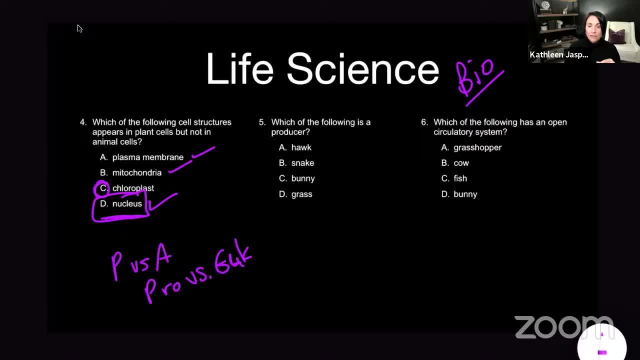 Single cell organisms have prokaryotic cells. Eukaryotic cells are for multicellular organisms And the nucleus is one of the biggest differences between the two. All right, Now we're going to move away from cells and we're going to go into actual organisms. 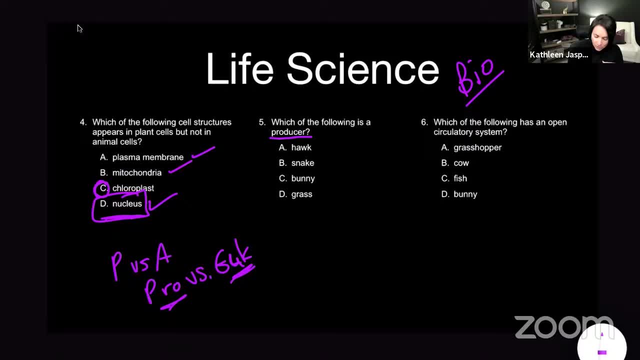 and living things. which of the following is a producer? Now, if we're talking about the energy pyramid, the producers are down at the bottom here. This is typically grasses, right? The grass comes from the plant cells, and plants generate carbohydrates through photosynthesis. 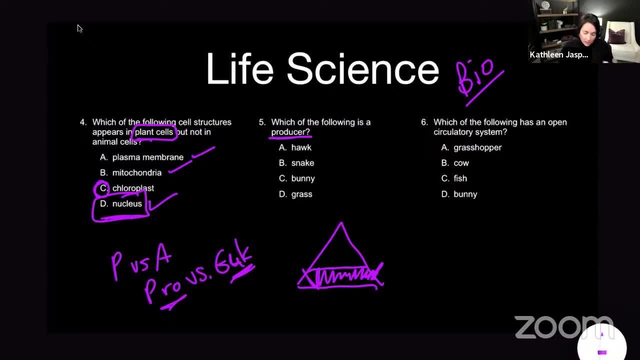 And we eat the carbohydrates And we get energy. So basically, what happens here is: the bunny eats the grass, the snake eats the bunny and the hawk eats the snake. So the hawk is at the top, But the producer is here. The grass produces carbohydrates because the sun is shining. 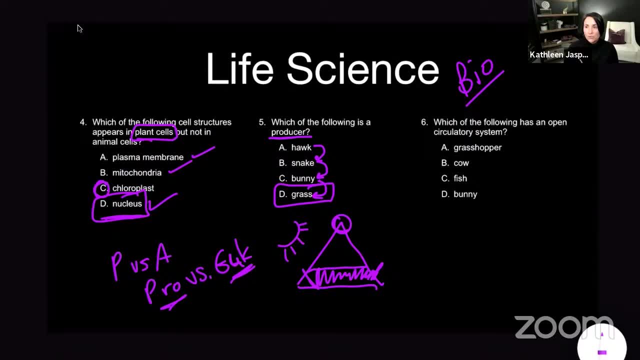 onto the grass and the grass is going through photosynthesis, producing carbohydrates, which is again a very simplified portion of that. But bunny then hops up, eats the grass. The poor bunny gets eaten by the snake and the snake gets eaten by the hawk. 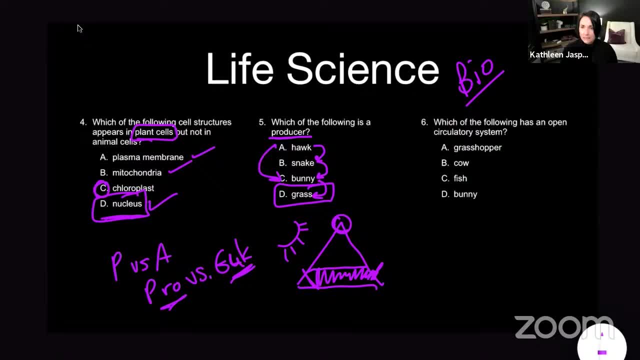 The hawk will also eat the bunny. The bunnies pray for a lot of things, Poor bunny, But the grass is the producer in that situation. And then number six, which of the following has an open circulatory system. So typically, vertebrae have closed circulatory systems and invertebrates have open. What's the difference between closed and open circulatory systems? All right, So closed circulatory systems means that when I take an air, when I breathe in, it goes into my lungs and then it does a bunch of stuff in there. OK, it's closed. 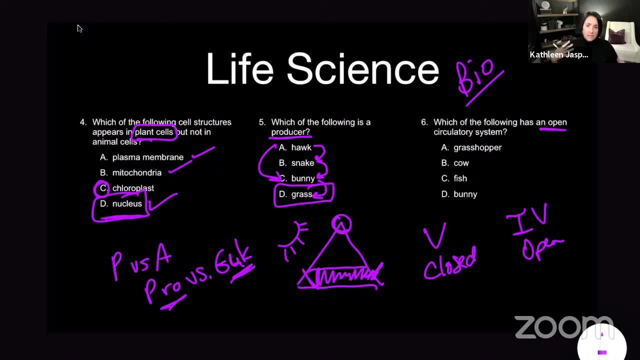 It has to come in through a certain area and then it does its thing once it's in there, and then it actually comes out, as, in terms of humans, It comes out as carbon dioxide and a few other things. So breathing in the oxygen and other gases in the air and breathing out carbon dioxide. 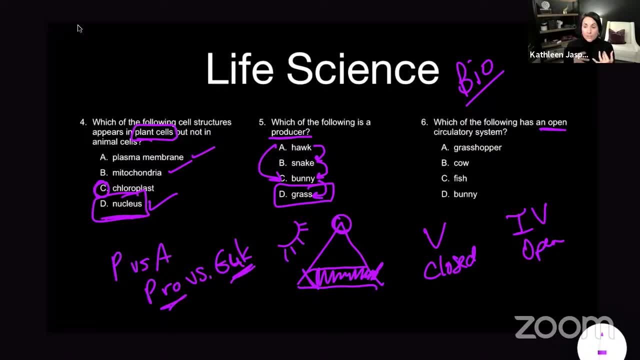 Right, So that's close. Also, gills: gills are considered like the lungs of the fish, So and vertebrae is they have a backbone. So typically anything with a vertebrae has- and I'm saying typically, because there's always something that I miss- somebody puts a comment. 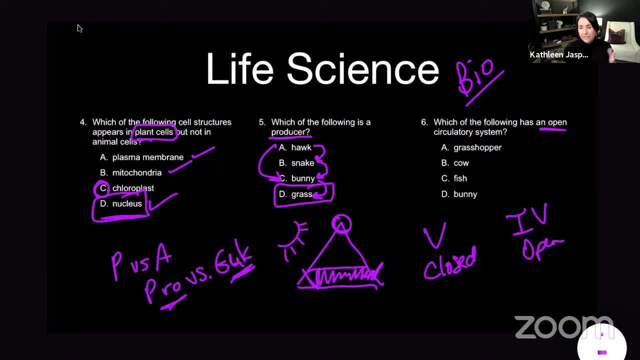 There is such thing as a vertebrae with an open circulatory system. If there is- I haven't heard of it, but there might be- But typically vertebrae have closed circulatory systems. They either have lungs or gills. 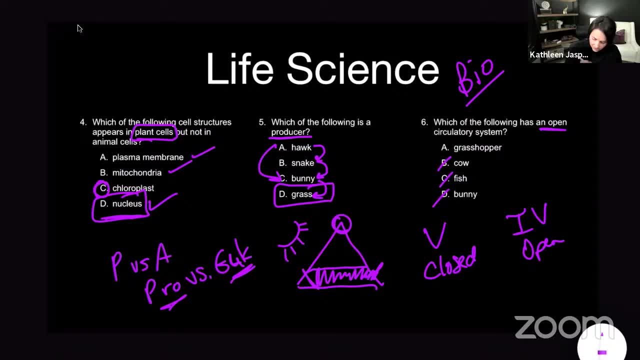 So let's notice here: Lungs, lungs, gills, Those are all closed in an open circulatory system. Let's take the grasshopper, which is the correct answer here. The air just comes in the body, just comes in the body through holes. 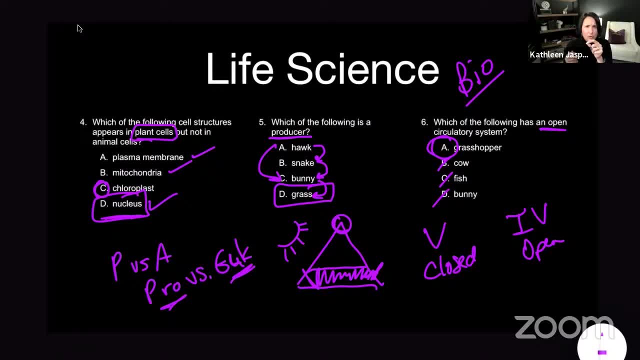 So, like a grasshopper has these little holes called spiracles- spiracles, I think they're called anyways- they come in the body and the air just enters the body. that way, in order for the for the grasshopper to use the oxygen. 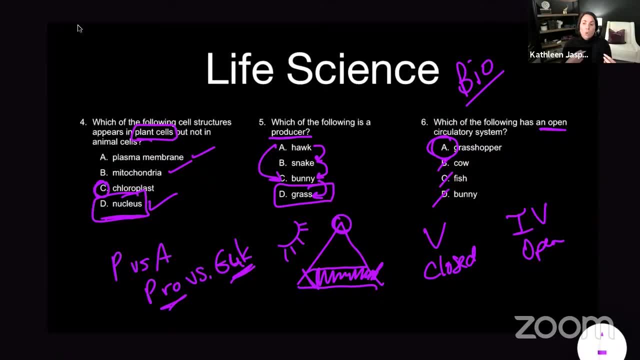 in in cellular respiration. So that's how that works. A very simplified portion. So again we're looking for open. Now a clam has an open circulatory system to bugs anything without a backbone, So that's going to be open here. 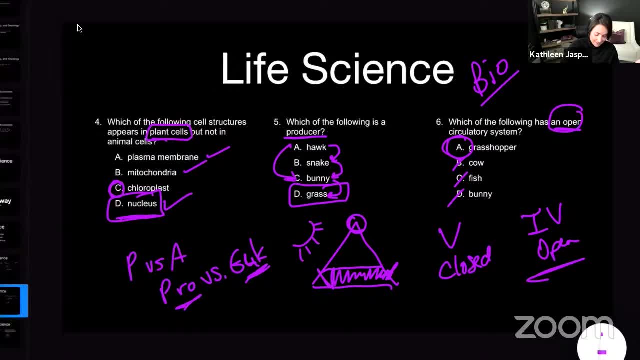 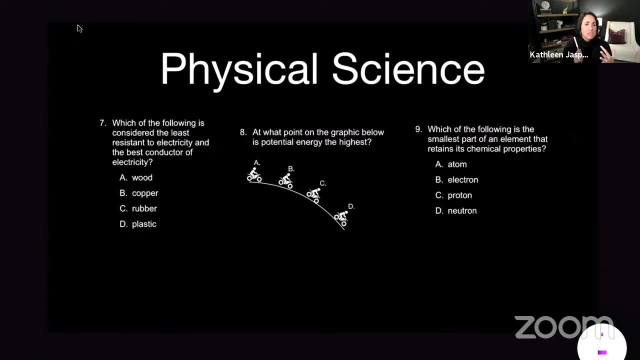 So again, you may not have heard anything about that for 20,, 30 years, Right? So that's OK. Now let's go to physical, physical science. Now we're talking about energy, machines, atoms, elements, all kinds of things. 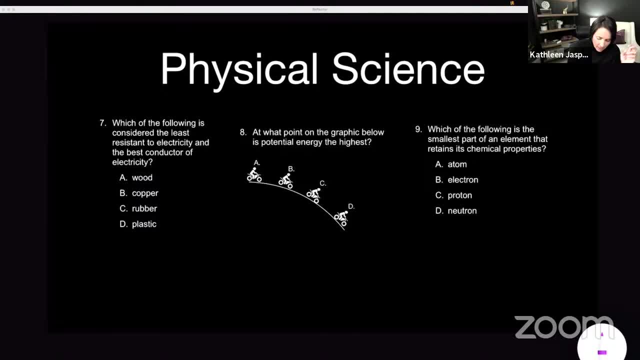 Here are three questions that kind of go with that physical science. All right, Let's take a look at number seven. The answer choice is wood, copper, rubber, plastic. Well, because I take and write so many of these exams, I know we're probably talking about electricity here. 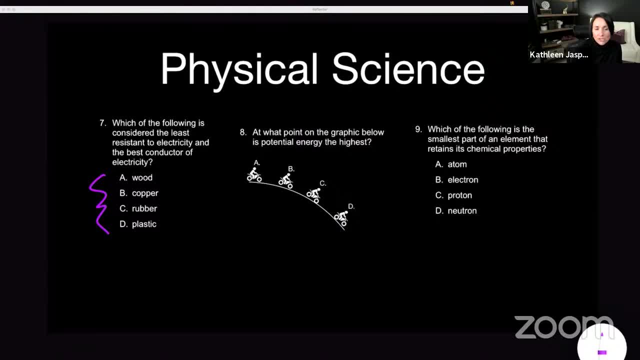 That's. those are usually conductor type questions. So let's take a look at the question which the following is considered the least resistant to electricity, least resistant and the best conductor of the electricity. So if it's the least resistant, it conducts electricity very well. 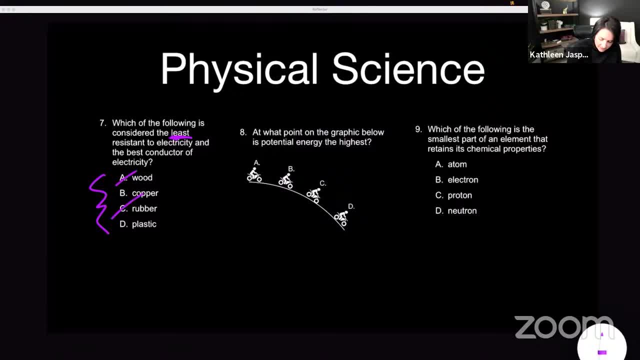 Well, wood resists rubber, resists plastic resists copper- Metal wire that is a good conductor of electricity. Notice that you will have copper wires that will be surrounded by rubber, sometimes styrofoam, sometimes plastic, so that you can pick them up and work with them. 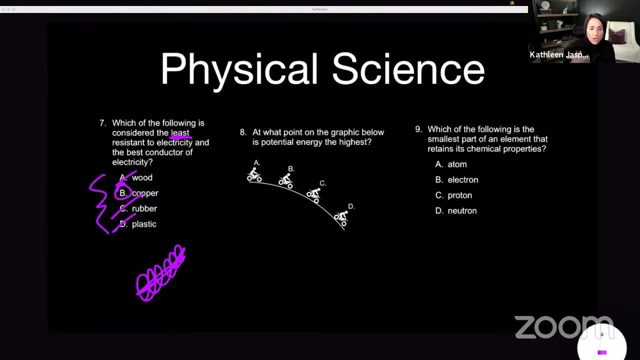 And so they don't set fire to your house or whatever. Wood, rubber and plastic resist electricity and are bad conductors. Copper, metal- other types of metal- are good conductors of electricity, So B would be the right answer there Now, right away. I can see from my answer choices here. 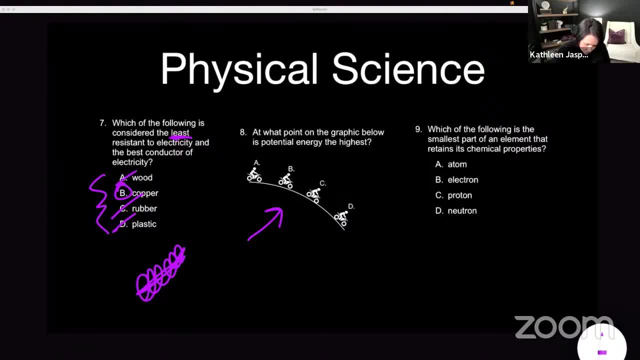 I'm probably talking about energy. I should have put little church There we go. He's going down the hill on his motorcycle, All right. At which point On the graph, on the graphic below, is the potential energy the highest? All right, So a couple of things about potential versus kinetic energy. 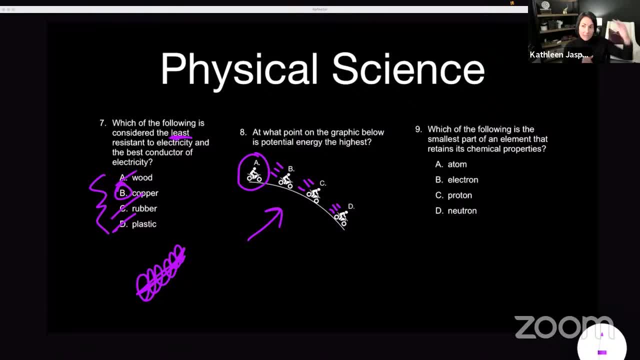 The answer is A, because the potential energy is the highest when it's at the highest point and it's going down. So if I were to take this pen and I were to drop it, this is the highest potential energy when I drop it. That's kinetic energy, as it's moving when it lands here and it's done. 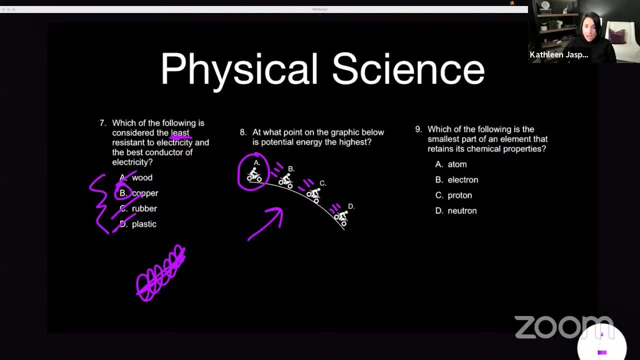 It has the lowest potential and the lowest kinetic. But right before the end, right before the end, this is the highest kinetic. OK, but once it you know, let's say this flattened out here in the motorcycle. I'm just going to do this. 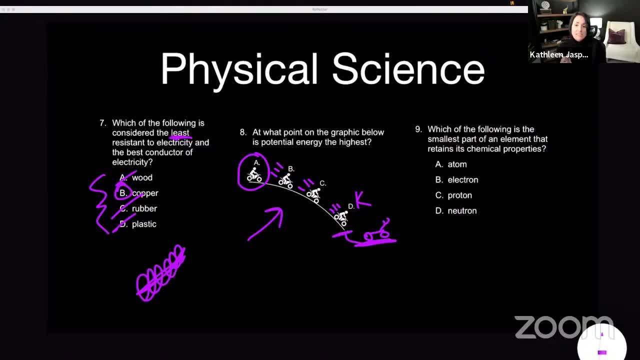 The motorcycle. that's terrible motorcycle, was there stopped. It has low potential and low kinetic. So highest potential, highest kinetic is going to be the best answer choice there. But you could get it the opposite way, which has the highest kinetic, and that would be D All right. 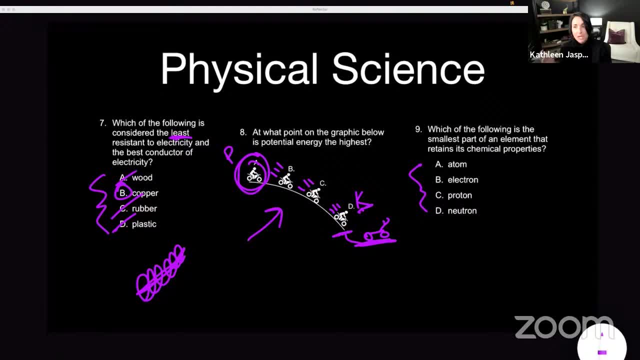 And number nine. take a look at the answer choices. Atom, electron, proton, neutron. I know I'm talking about atoms here and their subatomic units. Which of the following is the smallest part of an element that retains its chemical properties? 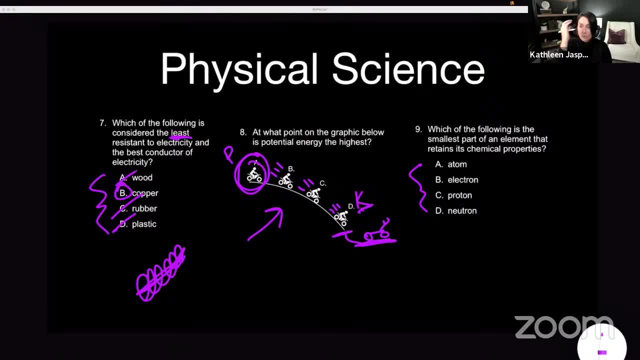 OK. so we're talking about elements on the periodic table. We're talking about atoms here. An electron is a part of an atom. A proton is a part of an atom. A neutron is part of an atom. Let's just quickly go through. 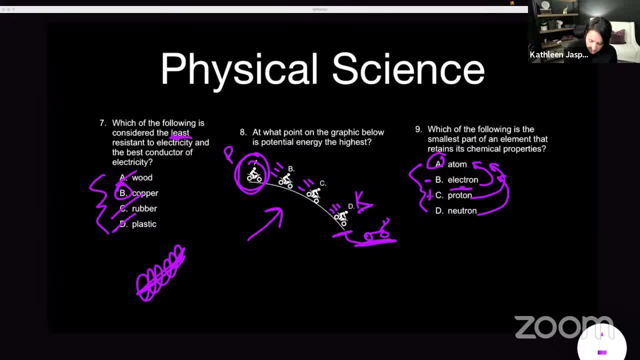 Electrons are negative, We charge, protons are positively charged and neutrons are neutrally charged. When we're talking about the atom, the protons, and make these little bigger: protons, protons and neutrons, and neutrons and neutrons are there. 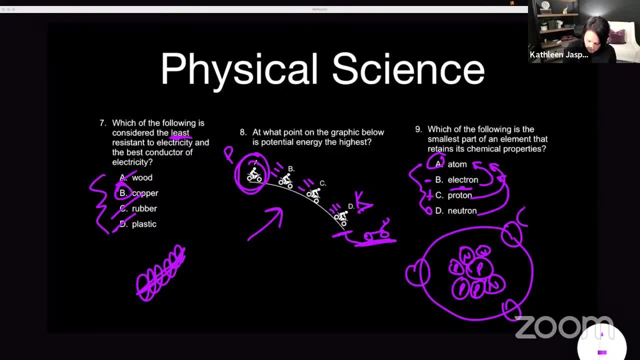 And then around here we have the electrons. They are negatively charged, So that is an atom. That is the definition of an atom. It is the smallest part of an element that retains its chemical properties. A is the correct answer. All right. 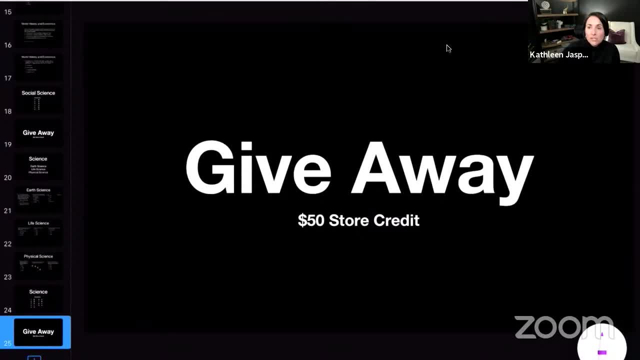 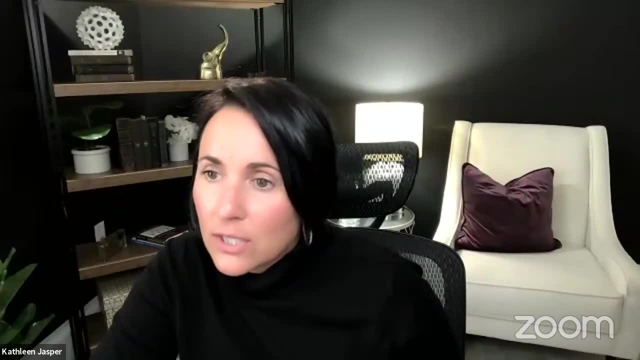 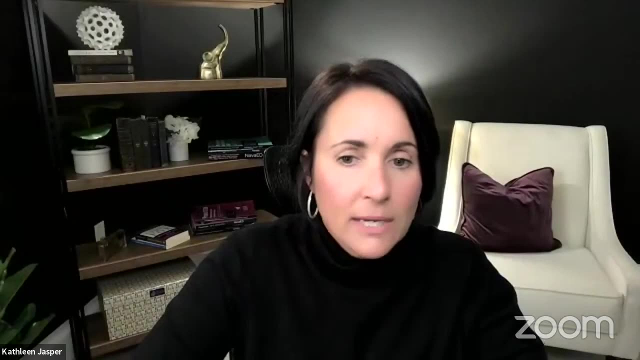 So we've got our answer here. We're going to a new giveaway, but let me just check the chat. Let me stop share here really quickly. A couple of you are interjecting there. Good, good, good. All right, let's take a look at really quickly. 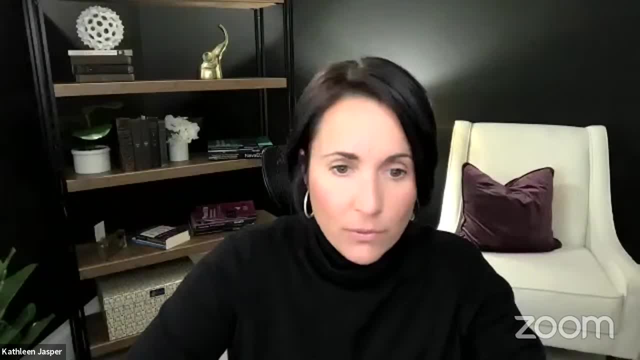 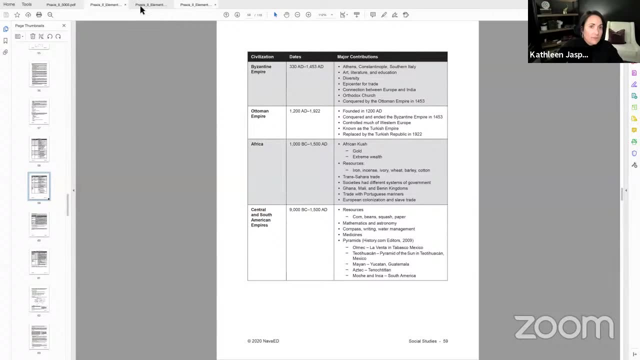 I want to show you the science portion of what we have for you, both free and paid, And I'm going to show you a bunch of free resources on my YouTube channel. So here is the book, for just the science. Again, if you get the full book, you'll see everything. 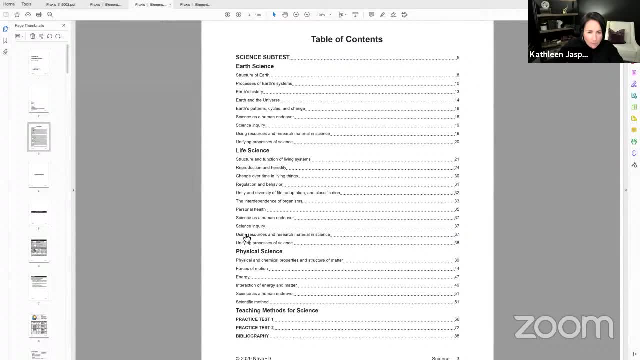 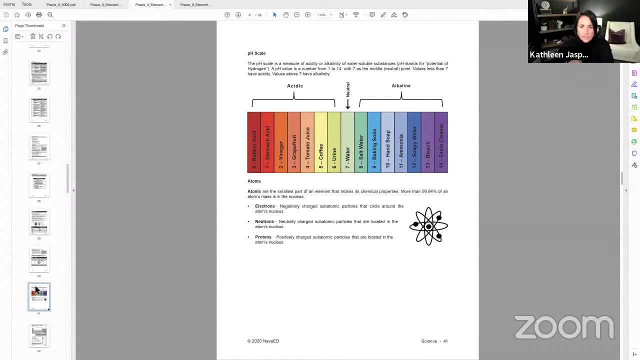 But I wanted to show you like with physical science you're going to get all of this information Notice. I even have the acidic or alkaline versus acidic here. Call it base basic versus acidic. We have the periodic table. This is. they had some tough questions. 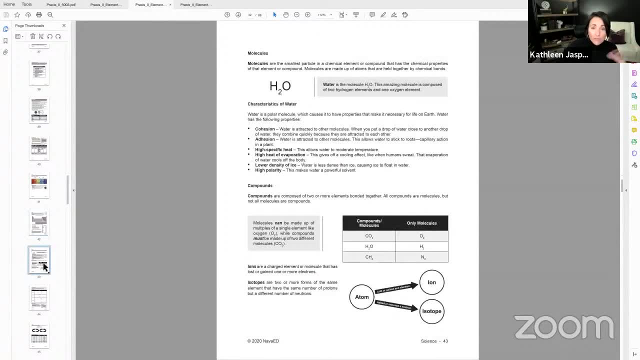 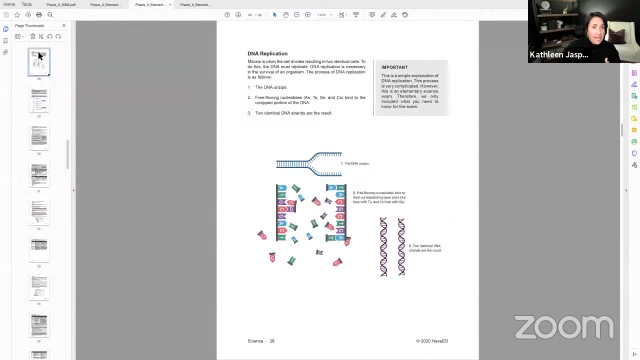 about the periodic table on the study companion and things like that. We've got all of the physical science here. We've got the life science, genetics- You might get a question On genetics. we've got DNA replication- You could get something like that. 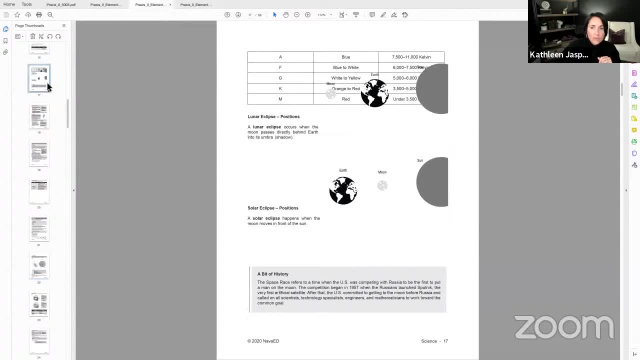 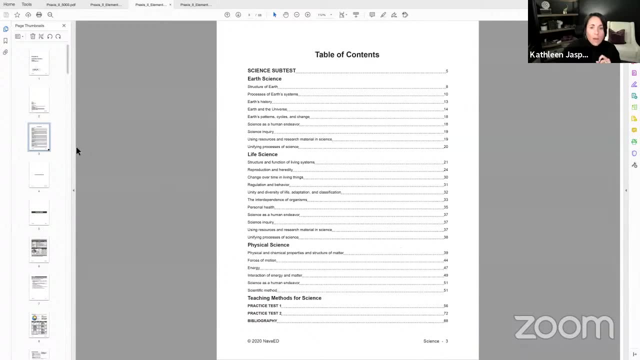 Difference between prokaryotic and eukaryotic cells. I do love this book. It's like a really good book. I'm very happy with with this book Every time I go in and I'm glad I did this book. But so you can see here: physical science, life, earth, structures of the earth. 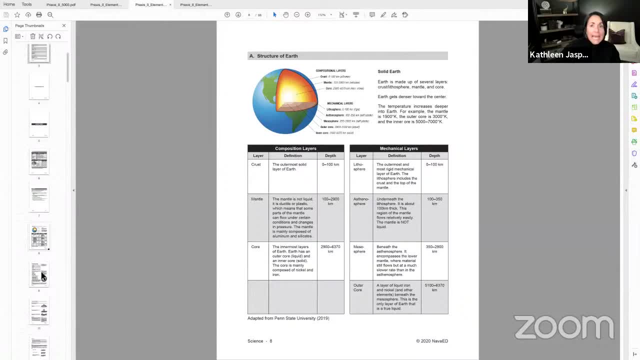 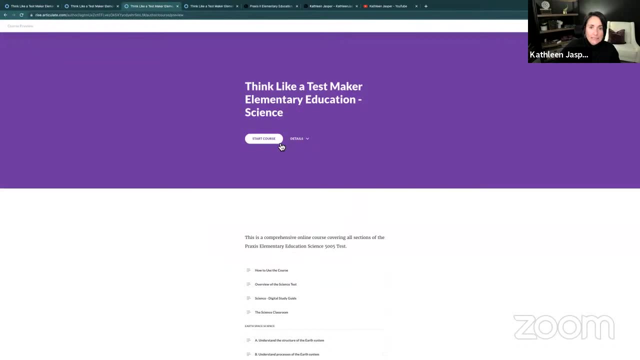 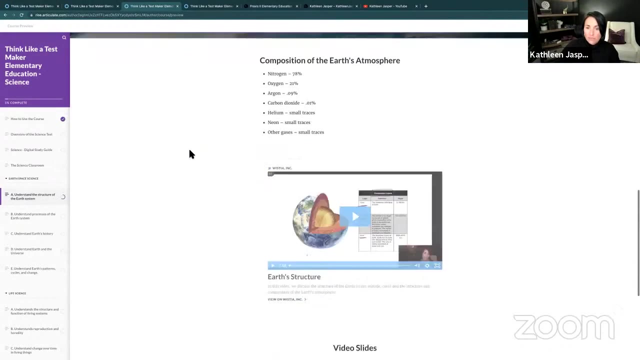 Remember, I've got some, some good stuff there for you. And then, of course, let me go to here. Let's go to Science. The science has got a lot of really good videos, If you want, like an online course. this online course is very, very comprehensive. 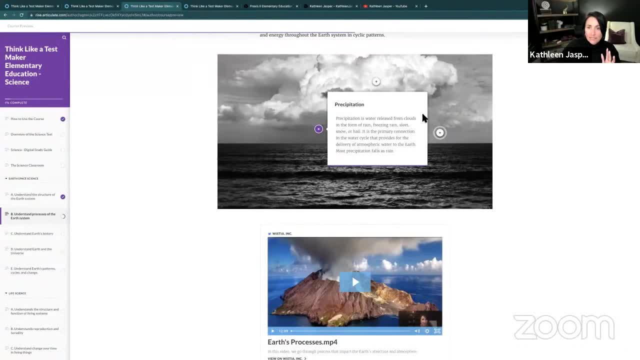 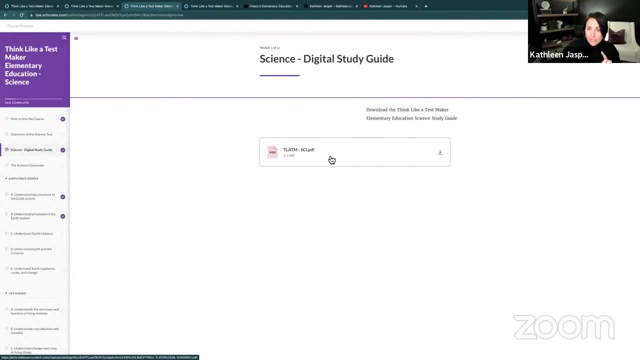 It's got videos for every single thing and different activities and things for you to do. If you're a visual learner, this is going to help you out a lot. And remember, it always comes with the digital study guide, So you're going to always get this and be able to download that digital study guide. 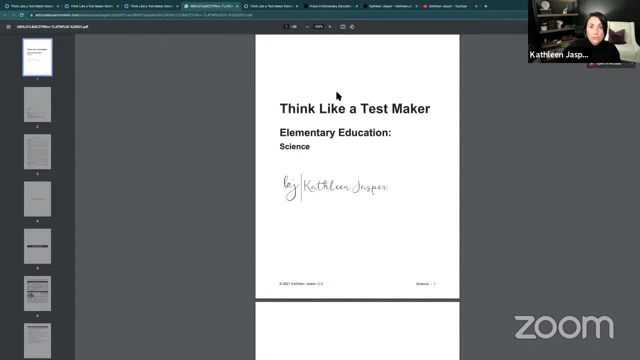 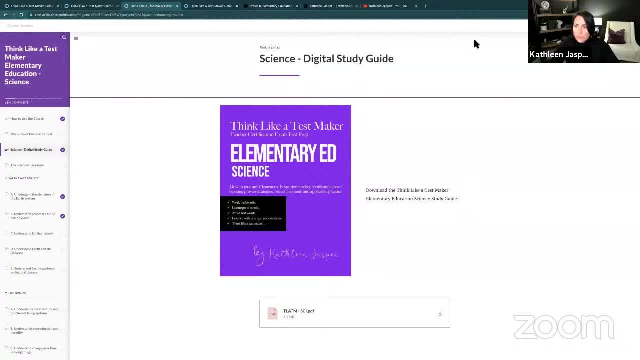 So I recommend, if you get the course work through the course we got, to read the book too, because there's a lot of really good stuff there. Okay, All right, Let me go to my giveaway here. Let me stop share. 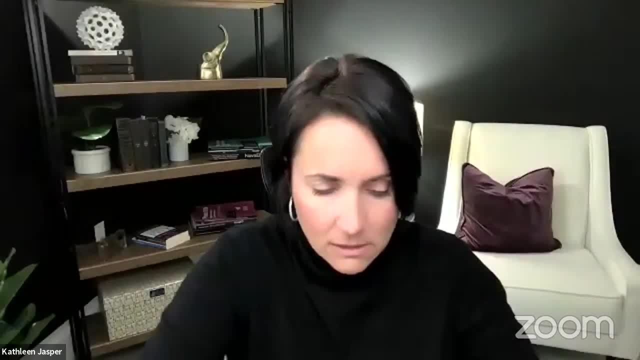 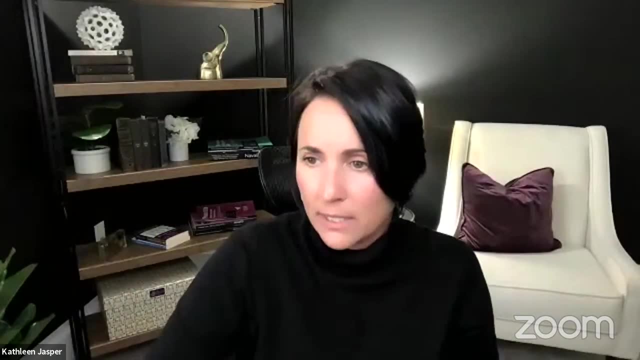 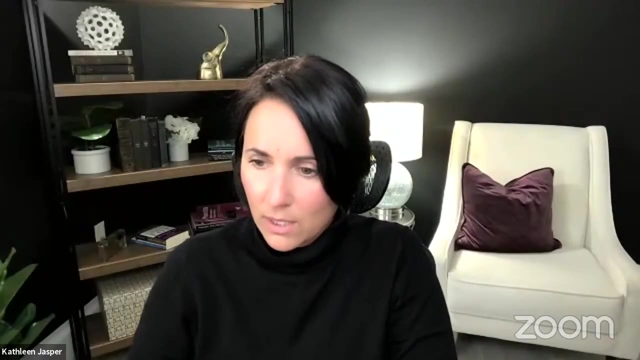 Sorry about that And let me just do the generate generator here And I have Cody Harmon Harmon. is Cody Harmon here? Cody Harmon, Are you here, Cody? Just checking really quickly. All right, Cody, you got fifty dollars Store credit. 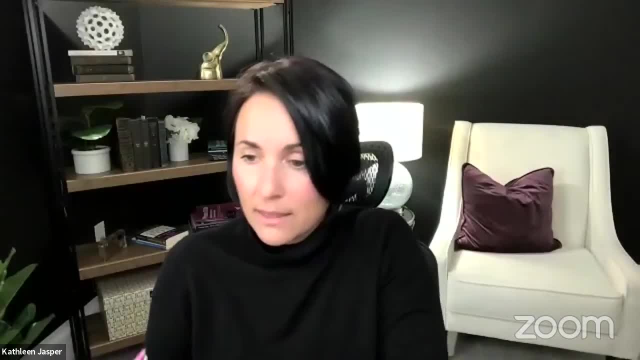 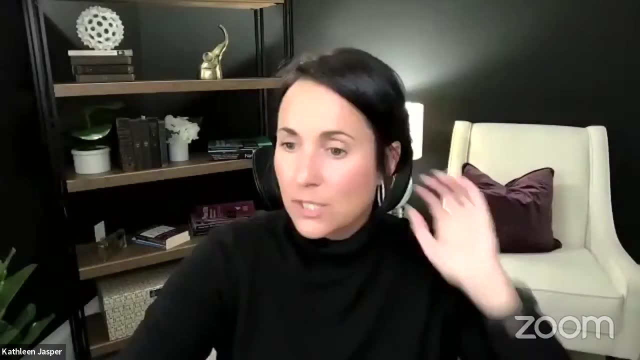 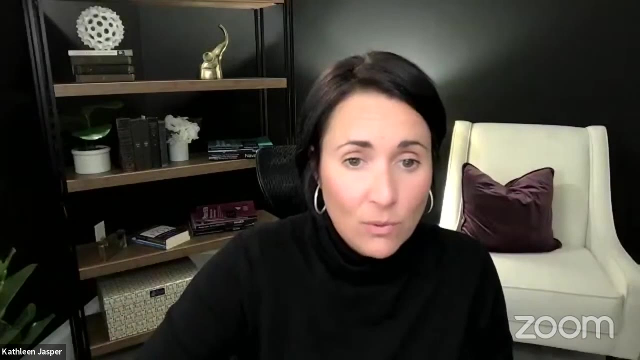 And I will send you that in an email later today. Good job, Cody. All right, Everybody. congratulate Cody Cody. OK, so we're moving on. Let me just go to share screen. This is the last section. We're almost done, guys. 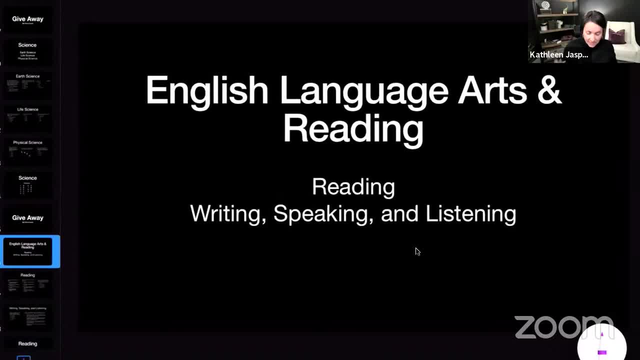 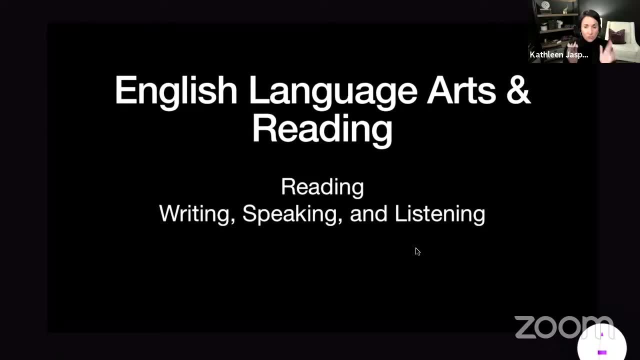 I know it's Saturday and you're like: are we done yet? OK, this is the English language arts portion. I'm going to show you several places where you can get even more free stuff for this. This I hit so much on my YouTube. 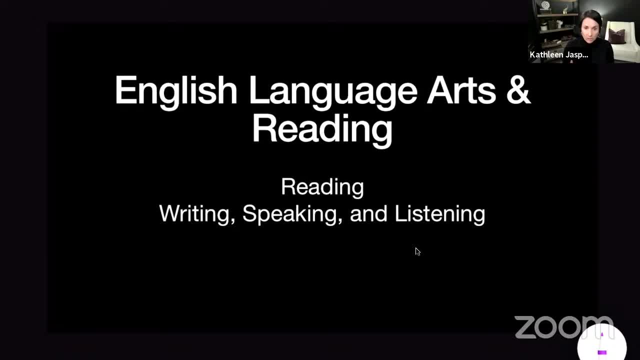 On my YouTube channel and on Facebook, like I'm always in the English language arts and reading, because it is on so many tests. It's not just on the English language arts for this, but it's the five oh three, nine. five oh three, eight for practice, it's the easy six for Texas teaching. 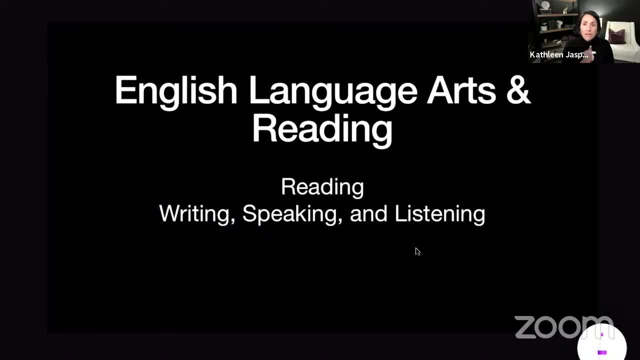 reading: Pearson Foundations of Reading. The philosophy is: everybody is a reading teacher, All right, And so it doesn't matter if you teach social science, science whatever- Everybody's a reading teacher, And a lot of you have to take the teaching reading test or 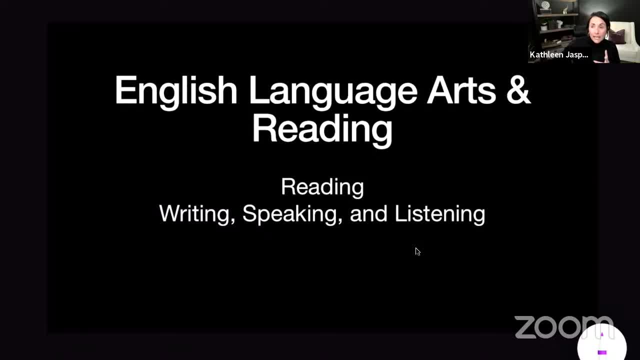 in Florida they make the teachers take a separate reading K-12 exam, So they're really hammering the reading for most teachers in content areas, even for content areas like social science and science. So it's a good idea to get to know this. 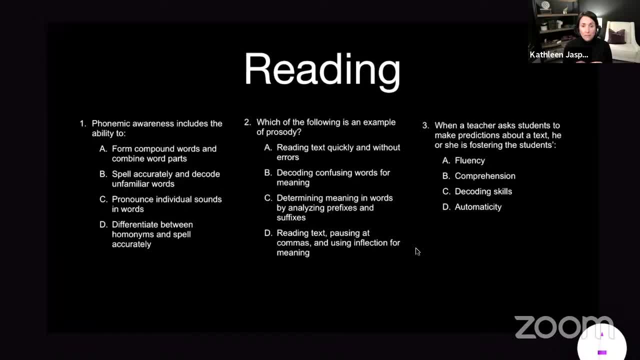 So when we talk about reading, we want to talk about the emergent skills, intermediate skills and, of course, advanced skills. So number one is going to be about your foundational skills. So I'm going to take a look at my answer choices first, and on the reading. 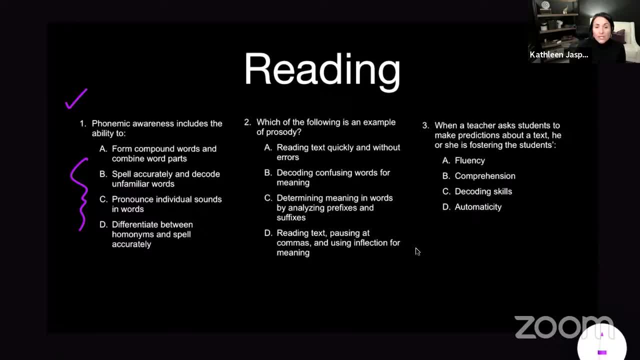 This is where the scenarios really get amped up. You got to know how to teach reading, And there are some good things I want to show you in this, in these examples that will help you think like a test maker for the reading section. So you're going to have a lot of long scenarios for reading. 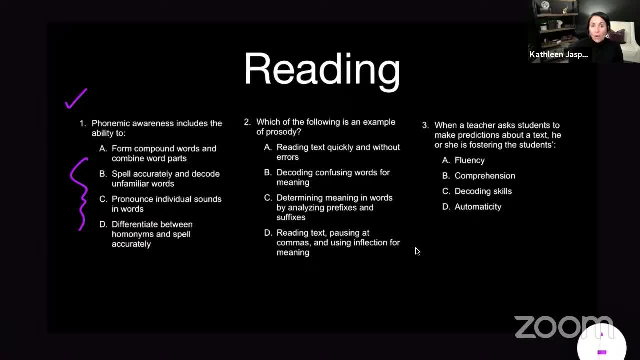 This one's going to be difficult, But again, my YouTube channel, our teaching reading book and the book the practice too, are going to help you with this. So let's take a look at the answer choices first. We have form, compound words and combine word parts. 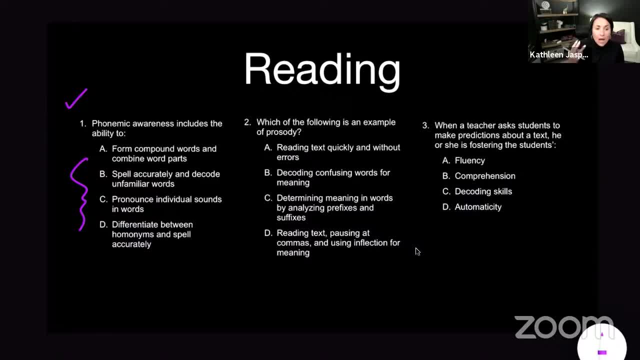 B- spell accurately and decode familiar words. C- pronounce individual sounds in words. D- differentiate between homonyms and spell accurately. All right, So we have spell and spell. I'm probably going to just, in my mind, cross them off because, remember, if it's kind of similar and you're only looking for one right answer, then it's not. 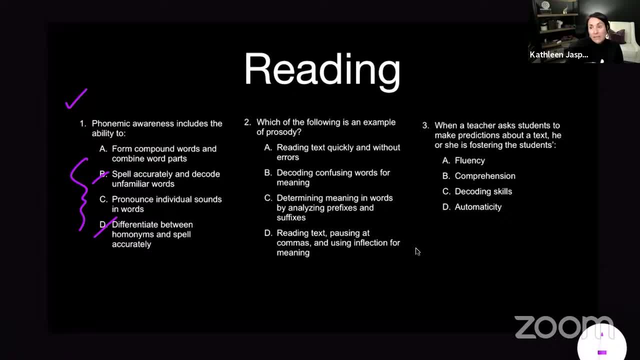 Now, if it says choose two, then I would look at those as being possibly right or correct answers, but it's saying we only choose one here, So then I'm going to look here. Phonemic awareness. All right Now. phonemic awareness. 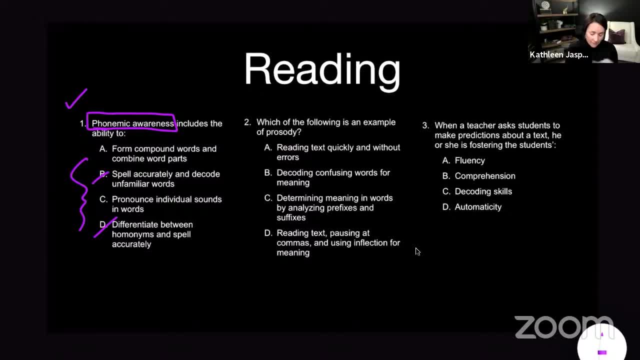 And I go more into this in my other videos and stuff. I talk about the umbrella and it's in the book. But phonemic awareness- I can't do it without doing the umbrella. OK, let's just do a quick little umbrella here. 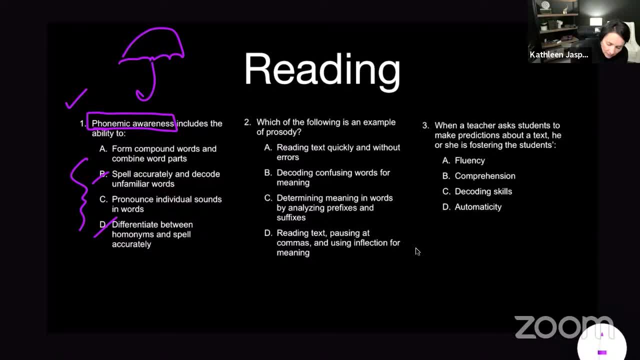 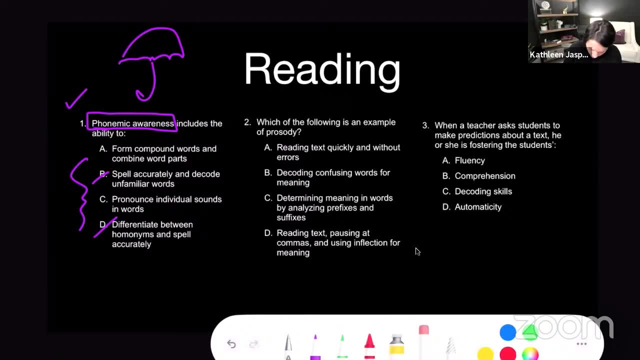 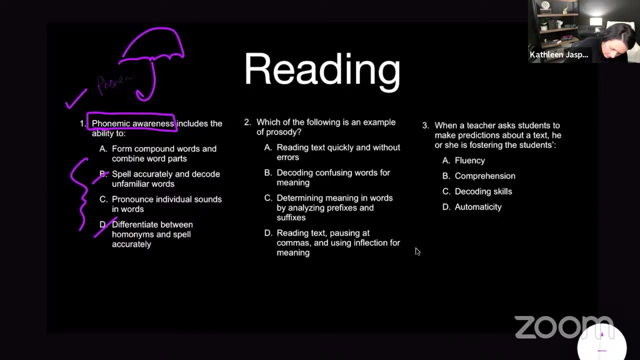 OK, So up underneath the umbrella we have phonemic. My thing is too, too fat. Let me go with a skinnier, Skinnier pen. All right. Phonemic Phonics And then Phonological awareness. Sorry about the. 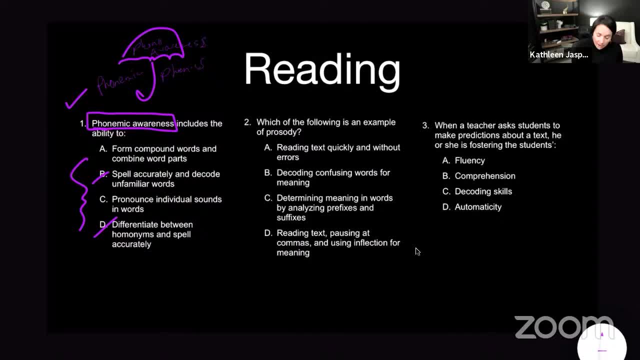 It's just a small thing but I go into this more in depth. But phonological awareness is the umbrella that has to do with all the skills together: spelling, syllabication, all of that, But underneath it we have phonemic. 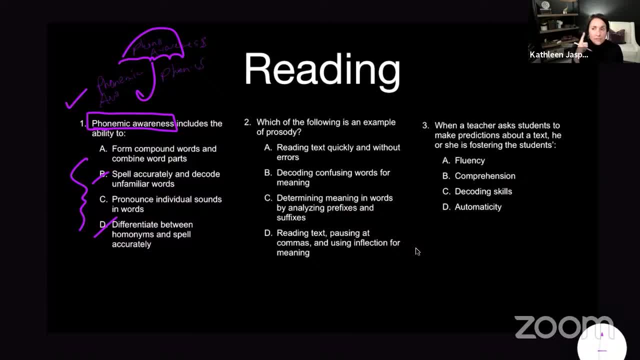 awareness and phonics. Phonemic awareness is about sounds only in words. OK, sounds only So. phonemic awareness includes the ability to pronounce individual- Let me get my pen back up to where it was: Pronounce individual sounds in words. And that's where I say: OK, guys, pronounce all the sounds in the word bat. 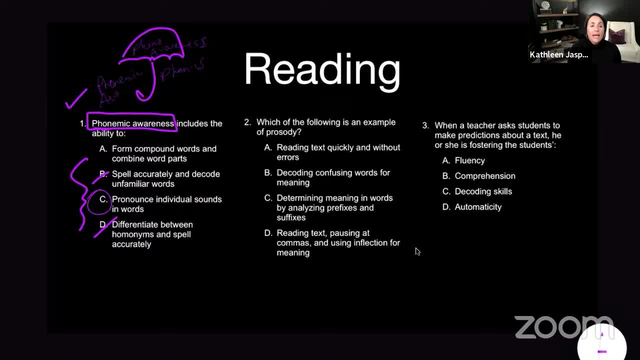 And the kids would go, but at bat. And this is the foundational skill. Phonemic awareness is the beginning of students to understand that there are sounds in words. You can do it in the dark, You do not have to see the word, You do not have to spell the word. 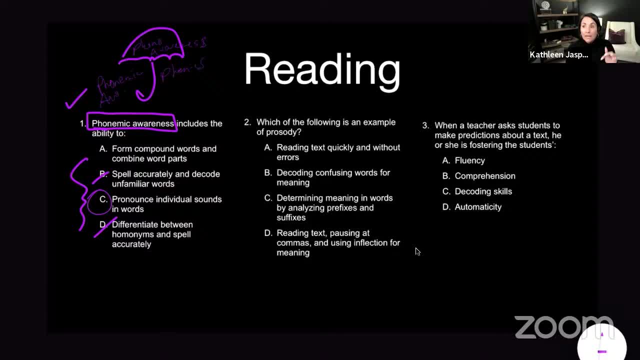 You do not have to even know that that's a B, It's just a sound in a sound, a sound. Phonemic awareness activities include deletion. OK, say the word bat without the sound and all the kids would go at All. right, That's deletion substitution. 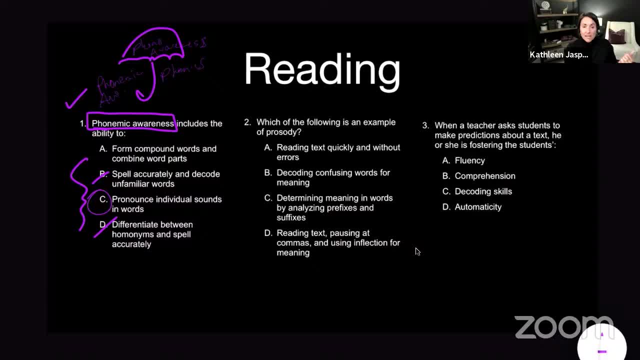 Say the, the word bat with the sound instead of the Sound and the kids say sad, Notice. I didn't say change out the B for an S. I said change out the book sound for a sound. We're talking sounds only with phonemic awareness. 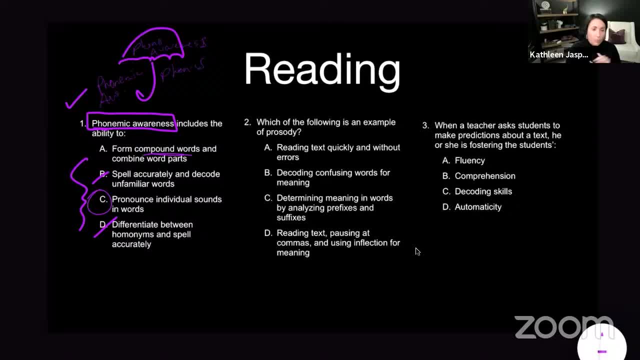 And let's just go through compound words. that has to do with morphology. Spelling accurately is phonics. Phonics has to do with seeing the letter and knowing like. if I see the P and the H together in English, I know that makes it sound OK. 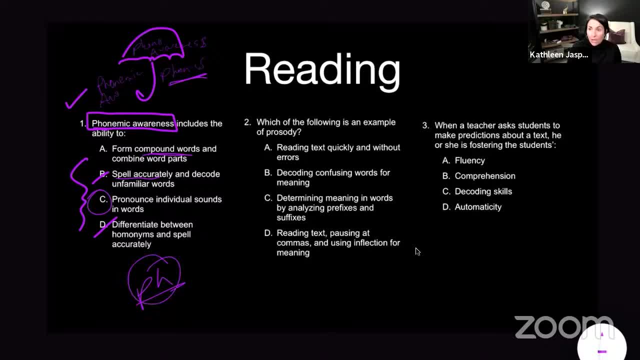 So that's phonics, because I had to see the P and the H. As far as I'm concerned with phonemic awareness, it's a sound, not a P and an H. OK, and then differentiate between homonyms, homonyms and spelling accurately. 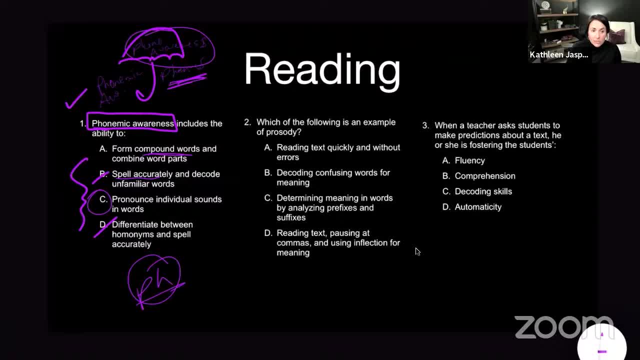 That is also phonics and a little bit of phonological awareness there. So C is the best answer. All right, Let's take a look at number two. Let's look at the answer choices. reading text quickly and without errors. I'm going to cross that off, because do we ever read without errors? 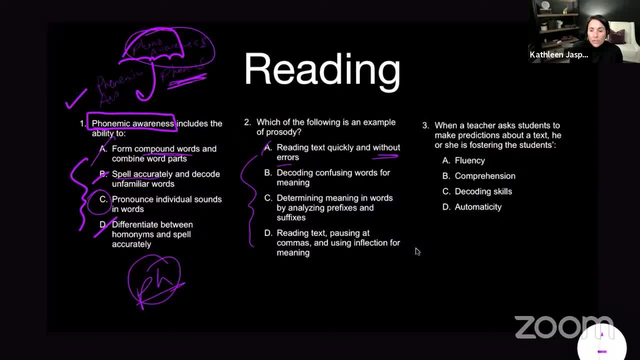 I don't know. It just doesn't seem like a really good answer choice. Be decoding confusing words for meaning? All right, Decoding typically has to do with sounding them out. It doesn't really have to do with meaning, So I'm going to cross that off. 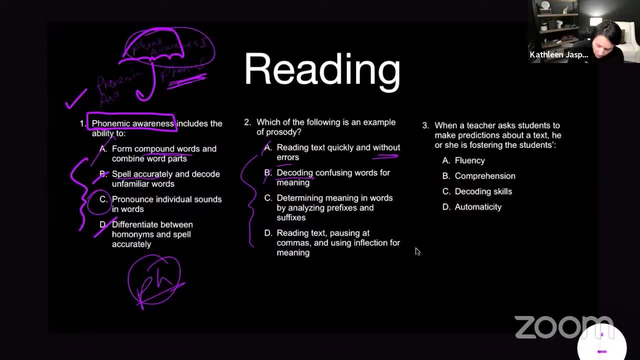 If you're decoding a word, you're going like: OK, if I'm going to decode this word, decoding, I would go deep. Oh, yes, because that's a long. oh, because it's followed by this: I decoding. I wasn't really trying to figure out its meaning. 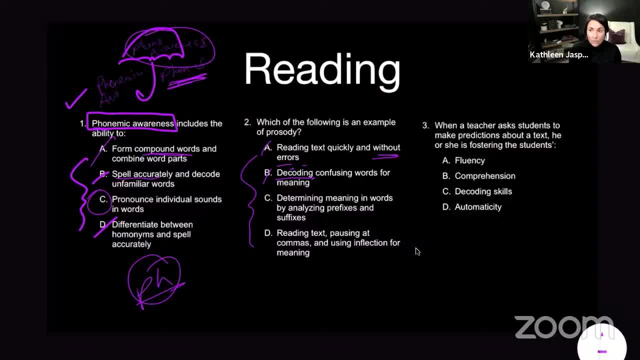 I was trying to figure out how to say it, So I'm across off B. It's not about meaning. When kids are decoding, they're not getting the meaning, They're just figuring out what the word is. See determining meaning in words by analyzing prefixes and suffixes. 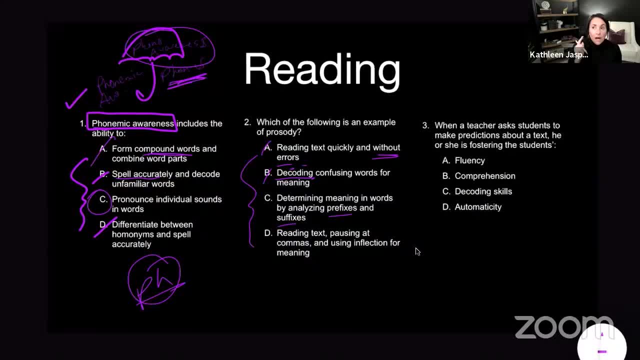 OK, we do determine meaning by prefixes and suffixes Right on, as a prefix means not suffixes. like Edie make it past tense, So I'll leave C D reading text, pausing at commas and using inflection for meaning. All right, Let's read the question. 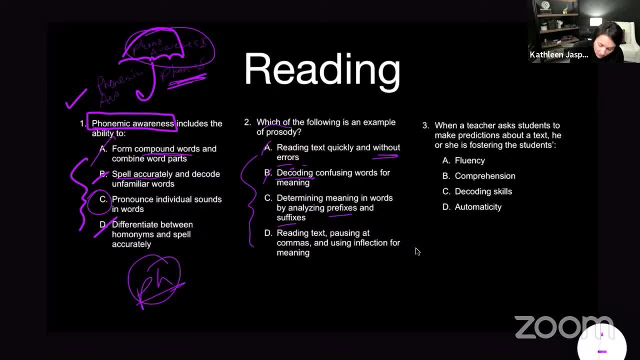 Which of the following Is an example of prosody? Well, prosody has to do with fluency, And the answer is D. reading the text, pausing at commas When there's a question, asking a question with inflection in your voice. 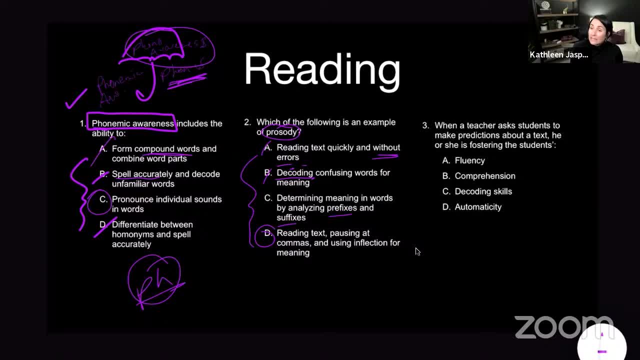 when it's excitement being excited. that is all prosody And it does aid in comprehension. So C is out, D is the answer. But notice that I crossed off A and B before even starting, which makes my job as the test taker easier, because I was thinking like a test maker, not a test. 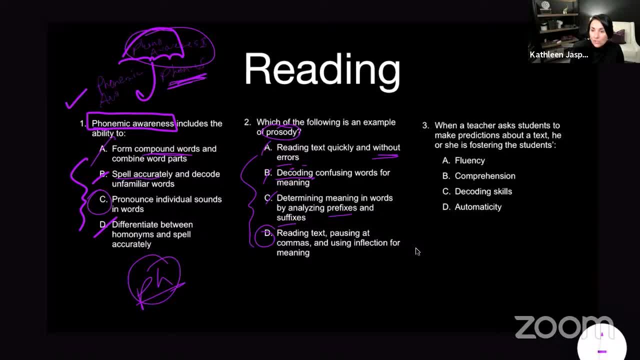 taker All right. Number three: When a teacher asks students to make predictions about text, he or she is fostering the students and the answer choices are fluency, comprehension, decoding skills and automaticity. If I started with the answer choices first, I wouldn't really be able. 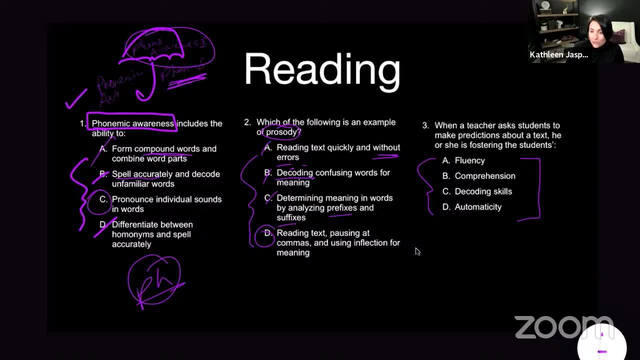 to do anything until I read the question, because those are just like terms- reading terms. So predictions- predictions actually have to do with comprehension. When you use comprehension, you're using your critical thinking skills, You're putting pictures in your mind. You're predicting what's going to happen next. 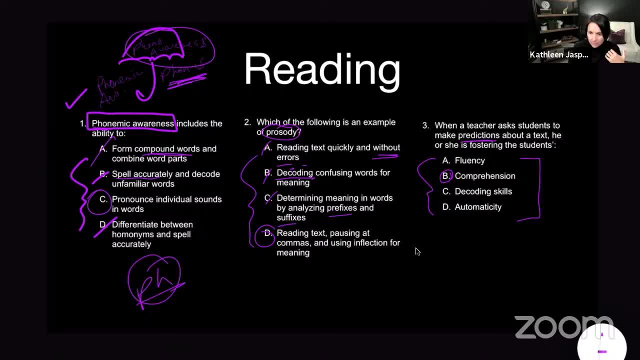 You're asking yourself questions. All of that is comprehension. OK, automaticity is about fluency. Fluency A and D are too much of the same, We would cross those off. and decoding skills also kind of goes with fluency, because if you have quick decoding skills, your fluency is going to be faster. 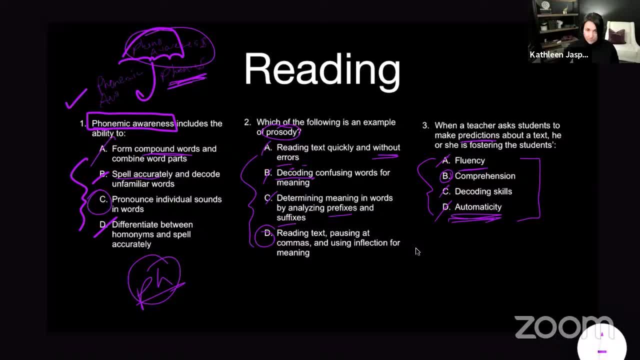 If you have automatic skills, your fluency is even more, even more effective. I almost said more better. I would need to go back to grammar school, But your fluency is even more effective because you are automatic. Automatic word recognition is where we want the kids to be. 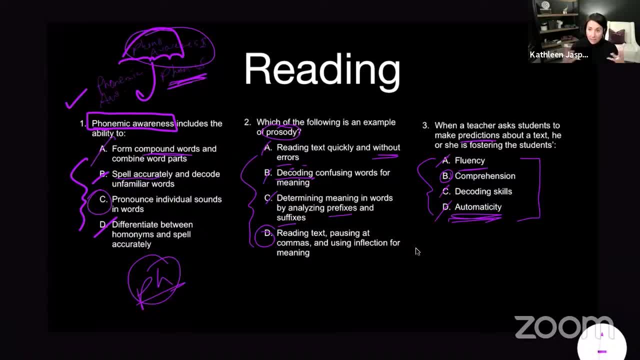 But sometimes they got to decode. There are times I have to decode words when I'm reading big science text and things like that, So, but this has to do with comprehension, because we're talking about that: critical thinking skills. Now, I'm not sure if we said this before. 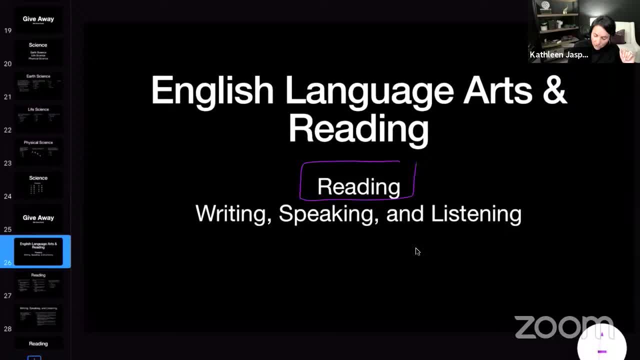 but the English language arts and reading portion has a reading section, which is the biggest portion, which are those foundational skills for reading, And then it has writing, speaking and listening together. Now, while writing, speaking and listening is a bigger section of the test, 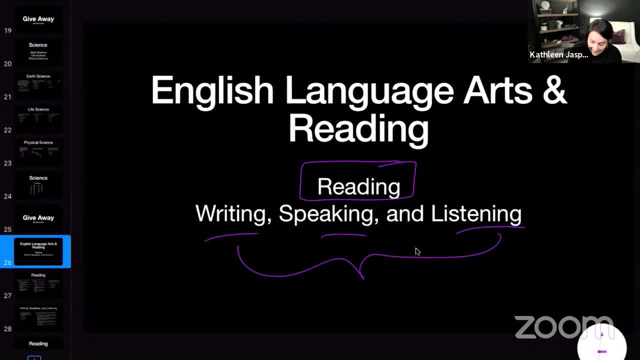 it's split among three, whereas reading has its own Right. So let's just go back here. Oh, I don't have it there, But reading is a little bit less in terms of the bulk of this part of the test. But then writing, speaking and listening are divided up. 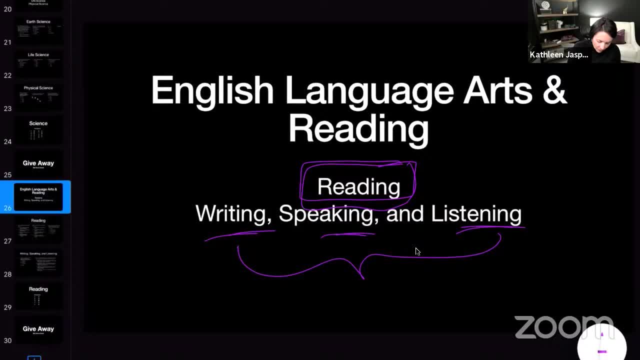 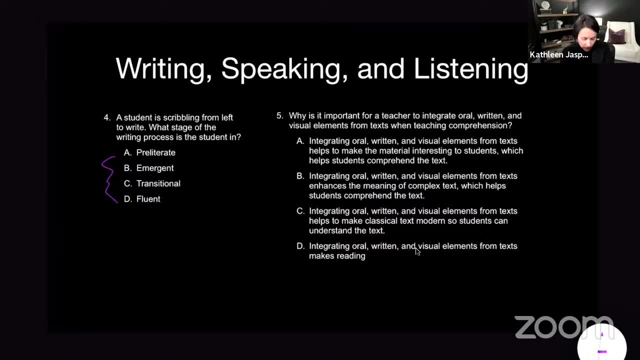 So really reading is a huge portion of it. We want to make sure you have that right now. Let's go to speaking, writing and listening here. So let's go. Let's go to number four: preliterate, emergent, transitional and fluent. 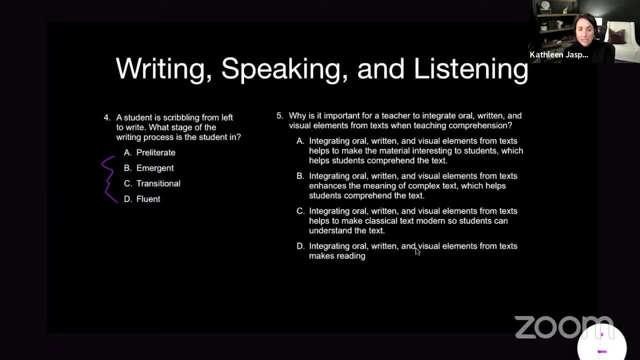 So I just have to figure out. these are, if I know, my stages of writing or reading. This is, these are stages, So I'm probably going to have to figure out what stage. So we have a student is scribbling from left to right. 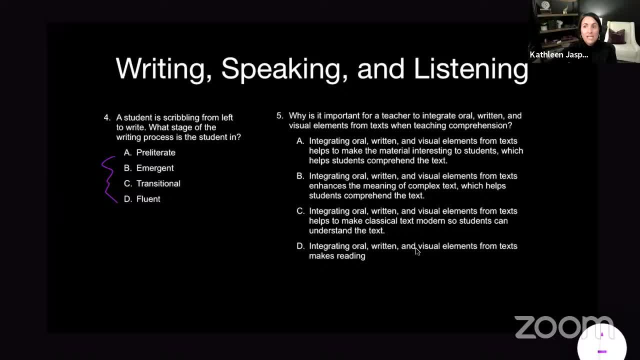 What stage of the writing process is the student in? Now in the book I have a table full of the writing process, So this is going to make more sense to you. But often students are kids when they start. You might see your children doing this, or 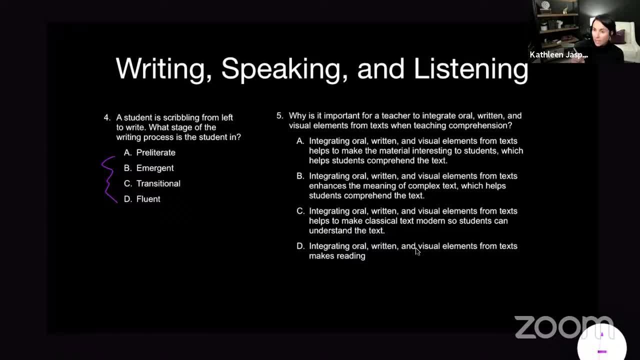 your nieces and nephews Or your students. they start to realize that when mom writes, or when dad writes, or when the teacher writes, they are writing like this, from from left to right. And what kids will do is they'll pretend they're writing and they'll scribble from left to right. 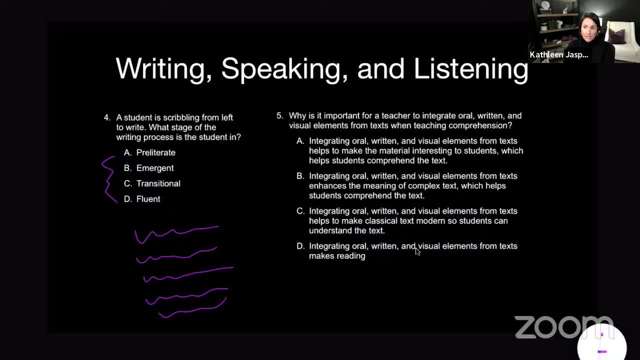 And this is a very important part of the writing process. Typically kids start by just like doing crazy scribbles on a page, you know. But then they move to this kind of left to right scribble there, All right, And then both of these are actually part of the preliterate, because there's no, there are no letters here. 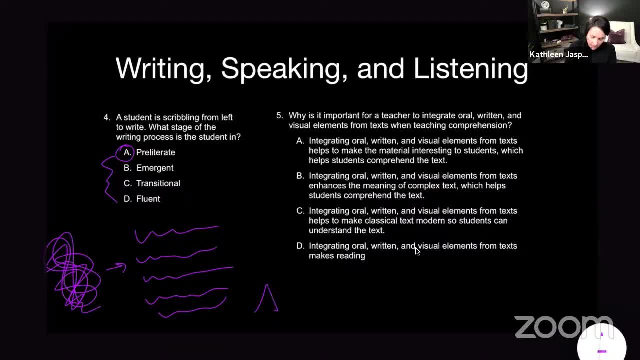 Emergent starts to happen when they start to kind of write their letters. They're a little bit like messed up, you know, but they write their letters. Sometimes they'll write their name like all in caps but a little bit all over the place, like that. 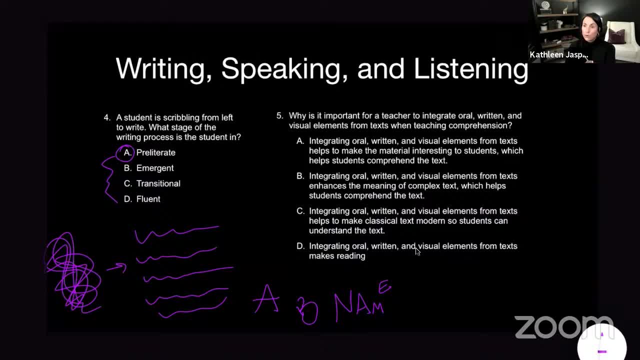 That's more of the emergent transitional. They start to write words like clearly, like they would write the word, write their name clearly, maybe with capital letters, stuff like that, And then fluent is like where we are, where we can fluently write things in English. 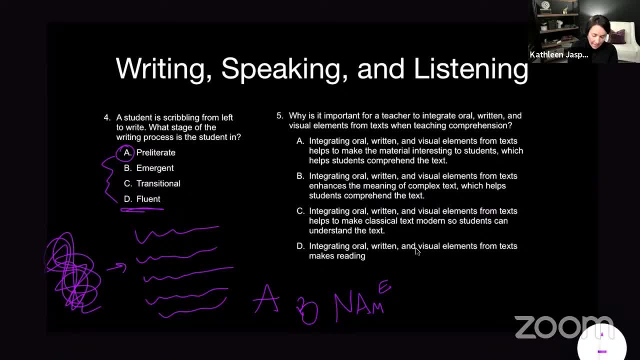 So this is actually a preliterate stage. We're going to go with a there. The word scribble kind of gives you a little bit of an understanding there. All right, Let's go with number five. So this is a big scenario question here. 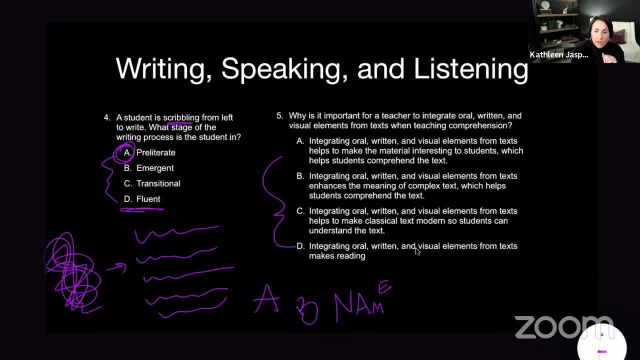 So I'm definitely starting with the answer choices A. integrating oral, written and visual elements from text helps make the material interesting to students, which helps students comprehend text. All right, Interesting is good. Integrating oral, written and visual elements- That's not really the reason why I would do interesting, but I like interesting. 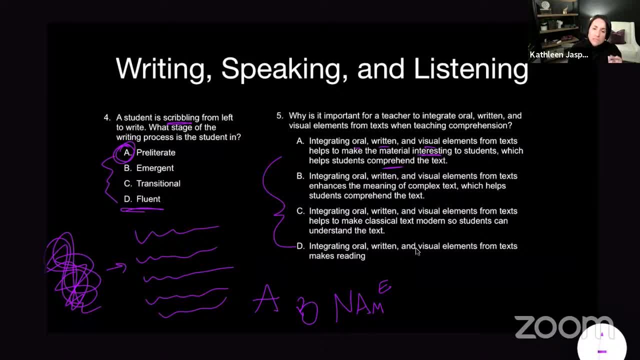 and I like helping students comprehend text, I'll leave it. Let's keep going. B: integrating oral, written and visual elements from text enhances the meaning of good word here. complex text and meaning, Which helps students comprehend text. Meaning and comprehension are related. 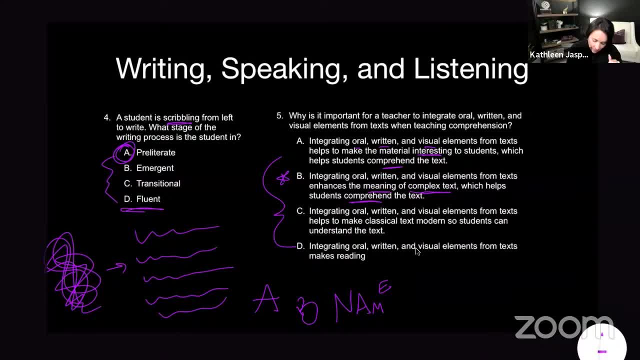 B is looking like it's my front runner so far. A is out. compared to B, B is the better one. C: integrating oral, written and visual elements from text helps to make classical text modern so students can understand it. No, that I mean classical text. 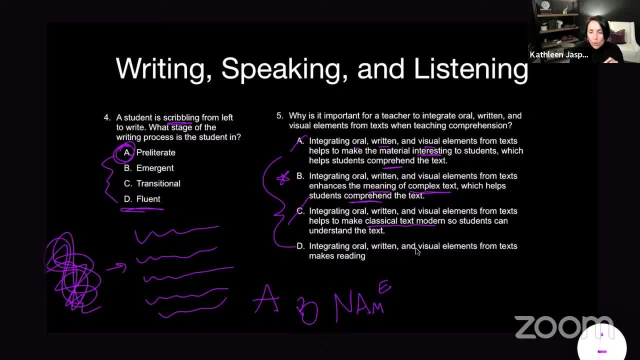 Yeah, I guess it would, but it doesn't beat out. B D: integrating oral, written and visual elements from text makes reading. Oh, it cut off. Sorry, that's supposed to be another bad answer. Sorry about that. We'll cross that off. 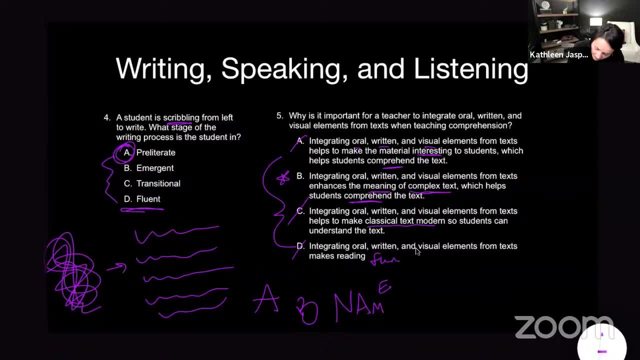 There. makes reading fun, We'll put. makes reading fun and enjoy. OK, do we want reading to be fun and enjoyable? Sure, but that's really not what we're focused on. We're focused on comprehension. That is the essence of reading. 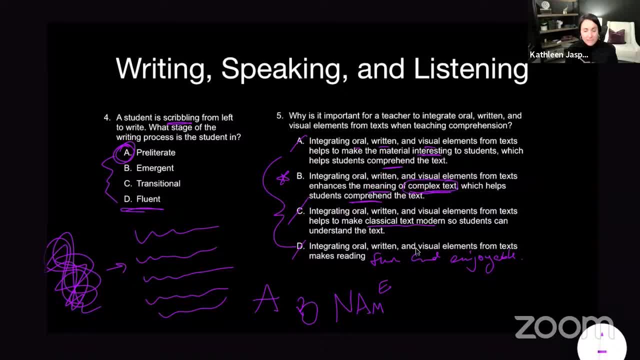 And we want students to be able to navigate complex text. Is reading always fun and enjoyable? No, you're going to have to read manuals. You're going to have to read stuff for your, for your job. Do we want it to be fun and enjoyable for kids as teachers? away from this test item. 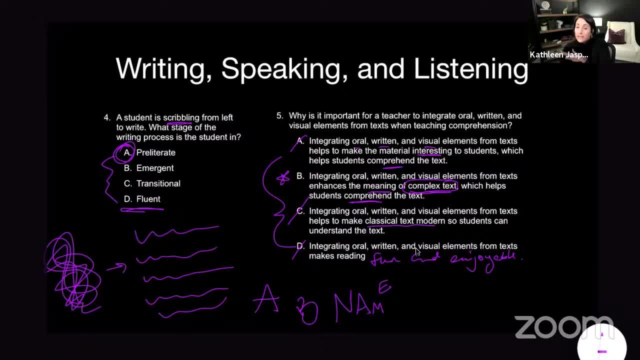 I would say to you: yes, please make it fun and enjoyable, Otherwise they're going to hate it, because they already hate it, because they're tested incessantly on it. So try your best to make it happy and fun. And so I like D as a teacher. 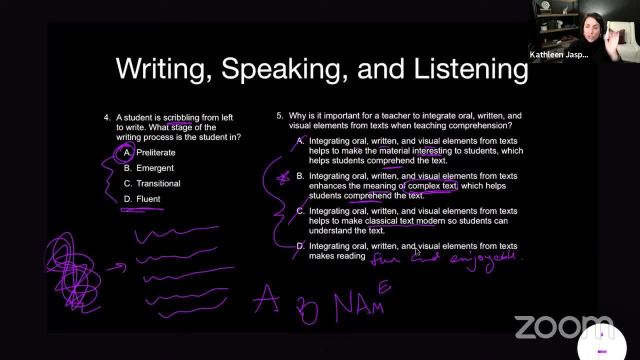 Right, But B is the best test question answer And I want to think like a test maker And the test makers are going with what the state wants you to know and the state wants you to prepare students for complex text on test day, So B is going to be the best answer. as a teacher, 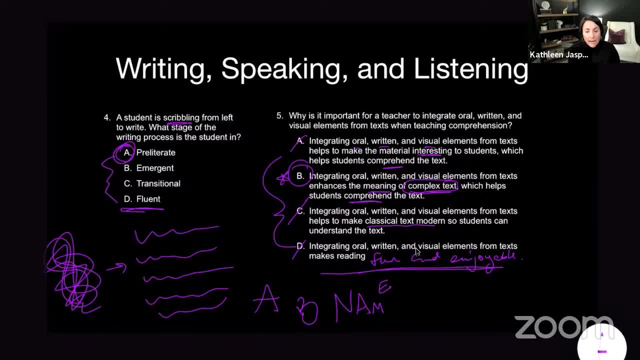 D might be your, your favorite answer, but you've got to think like a test maker and not just what you think about in your classroom. It's about the correct answer on the text. And then if we look at the, the question here, why is it important for a teacher? 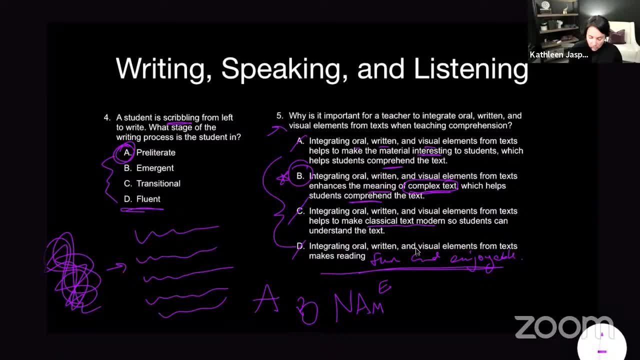 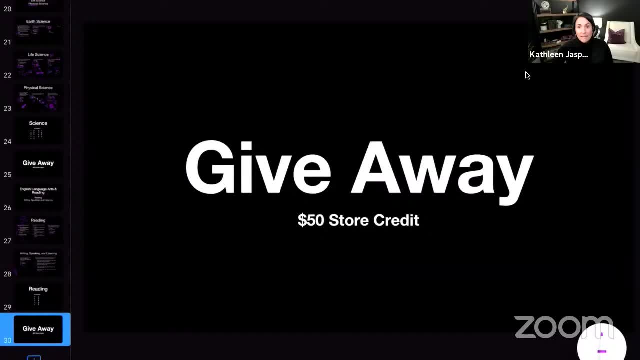 to integrate oral, written and visual elements. And then we go into the, the answer choices there. So B is the best answer there, All right, And then we have our answers. All right, We're towards the end, guys. We've got to give away. 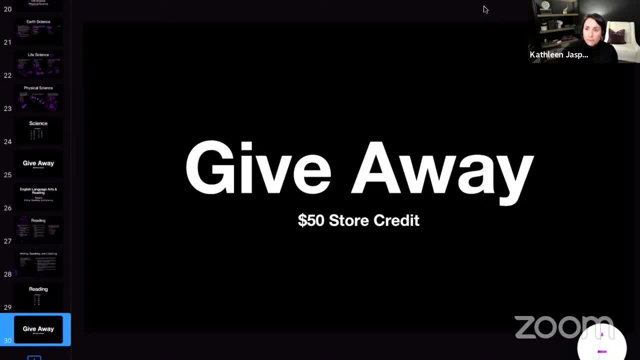 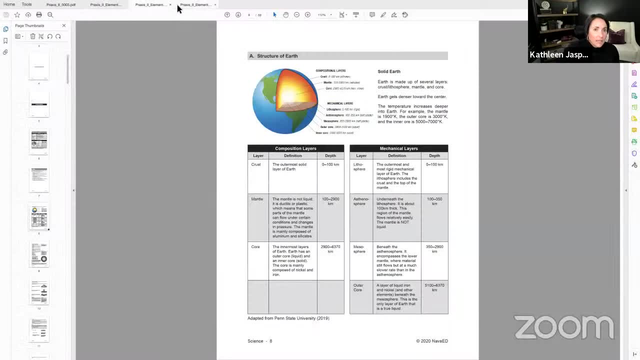 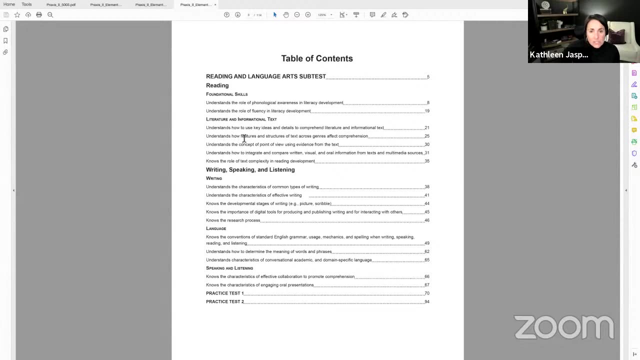 So I just want to share one more thing before we do the giveaway. We go to new share here. OK, so with the practice to English language arts, notice we have the foundational skills and then we have literature and informational text. You might have questions where you have to read. 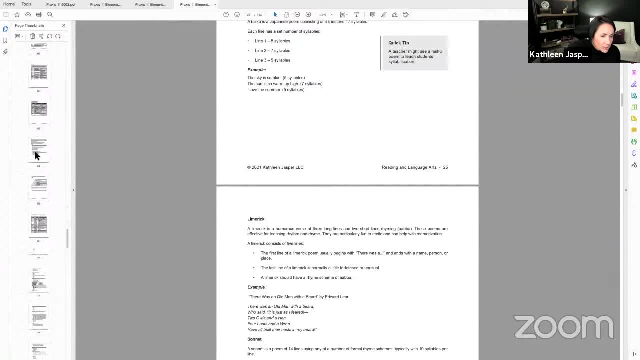 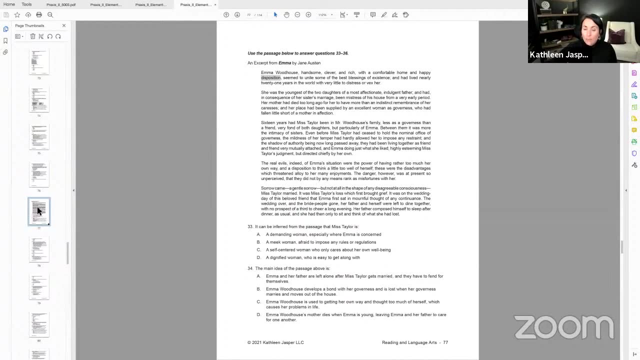 Let me go back here You might have to read. I just want to make sure you know this. OK, there are questions on the English language arts for five zero zero two where you have to read something like this and kind of answer some things about it in terms of an 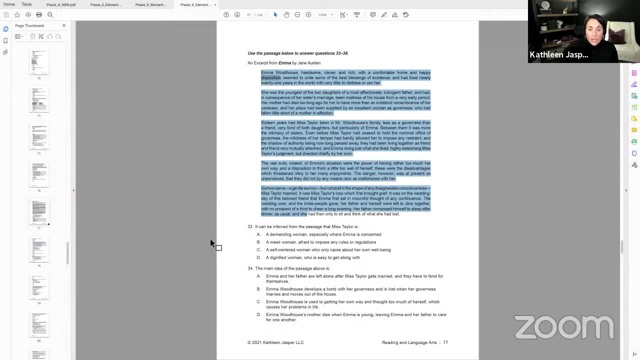 a language, arts and reading teacher. So you might say it's going to ask you things like the main idea. It's going to ask you things about personification, It's going to ask you about literary elements and things like that. So we have a few of those in here. 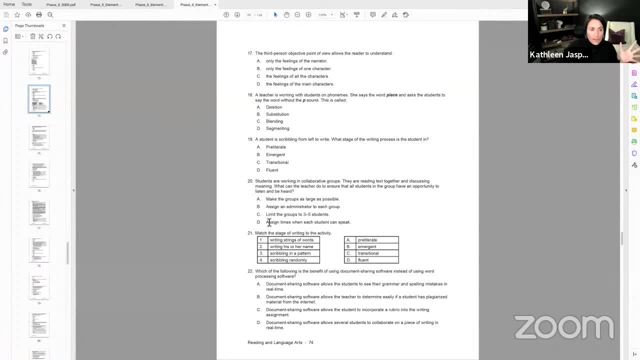 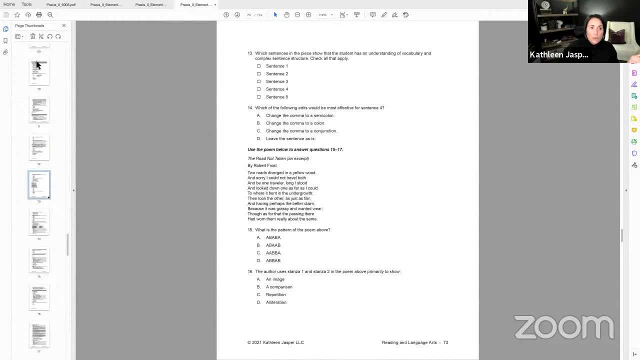 We also have, you know, the writing, writing portions and things like that, And so we have poetry in here. You're going to have a lot. The reading and language arts is a lot. We have the foundational skills and then we have it all the way down here. 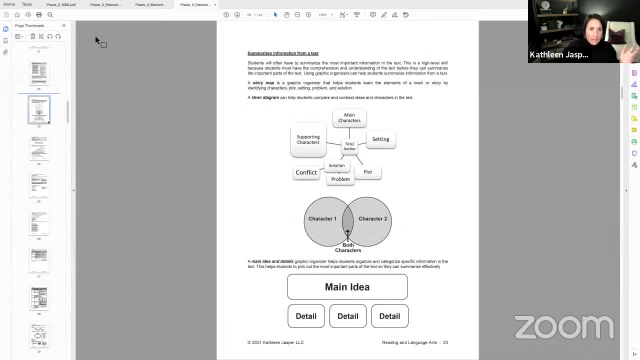 OK, so that's one of the sample tests. They're got tons of elements here for you. That's the book, And then let me just show you the online course is extremely comprehensive. for this There are the foundational skills. I go through it all. 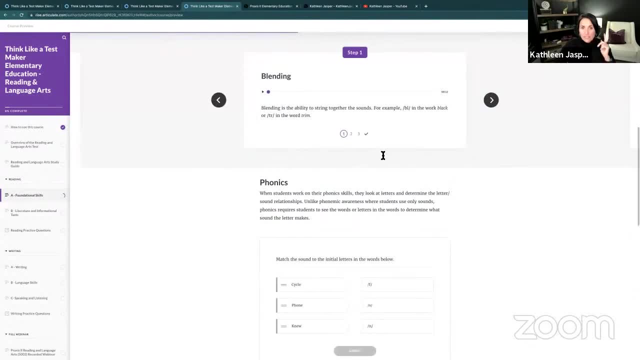 There's our umbrella. These are some oral activities because, notice, we're talking about phonemic awareness and that sounds only So. these are all listening things that I have you do here. There's some matching. There's always going to be really good videos there. 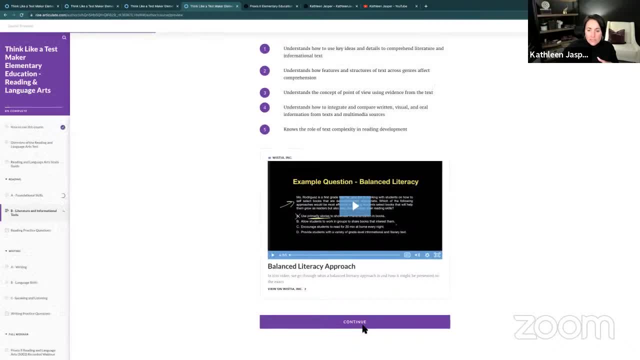 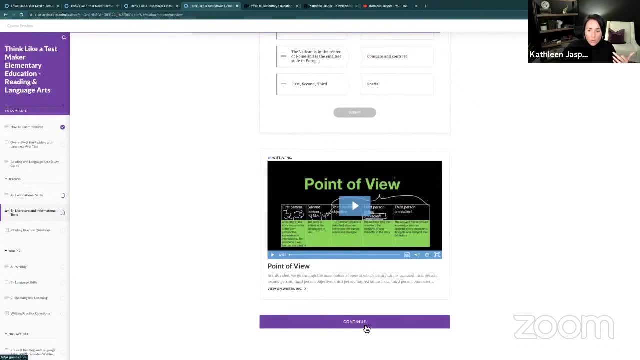 I go through all of this and you keep hitting. You keep hitting continue, continue. I mean, there's just whatever. There's a continue button, You keep hitting it and there's just more and more and more stuff here And so when? 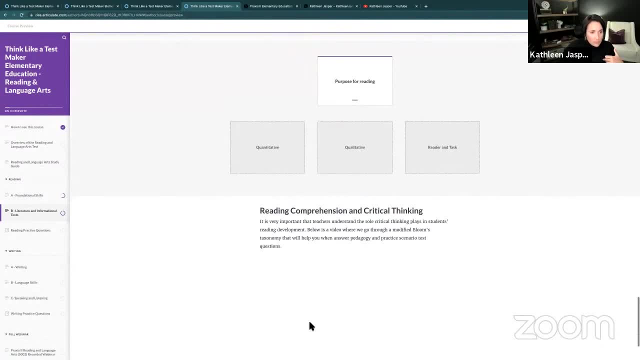 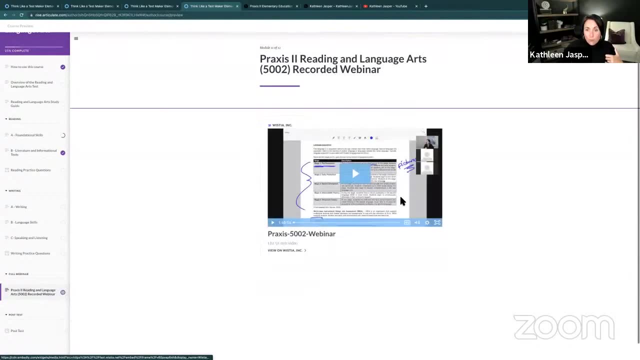 that little circle over here becomes all the way full and becomes a checkmark, which I believe it'll do now. yes, indeed, that means you're done again. We have a audio course here. It's a full webinar you can check out. 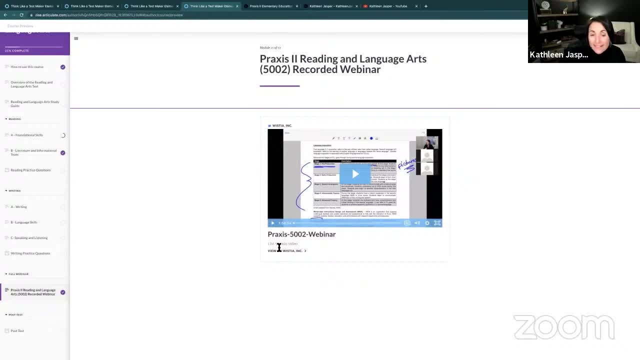 This is an older full course that I did. It's an hour and 50 minutes. Some of you like to put in your headphones. go for a walk. This is a really great way to do that, And then, of course, we have the post test. 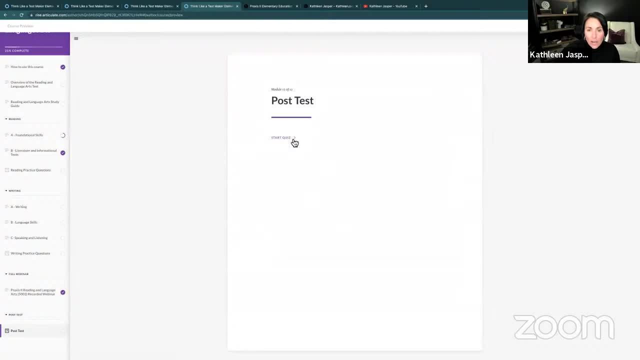 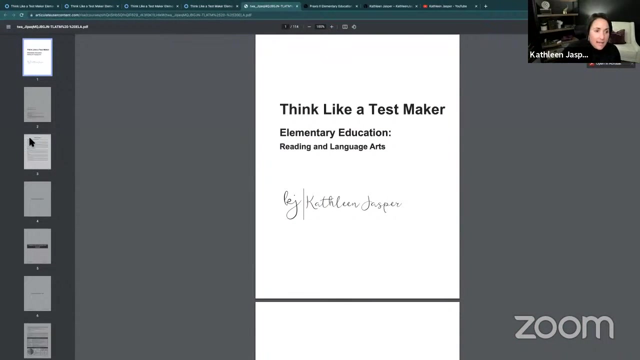 which is the second practice test for you to check out here, So you can take things online. So I would do that. You know how to use the, how to use the course And basically I tell you, go into the study guide first and then do the pretest. 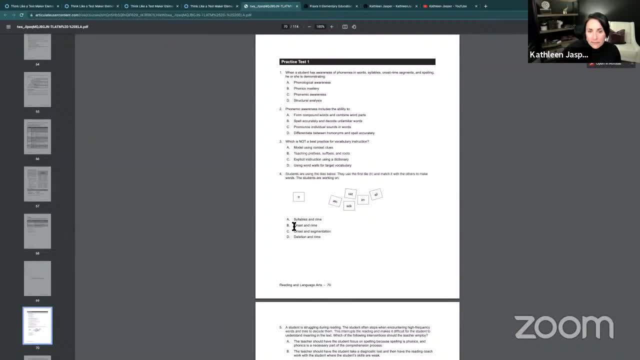 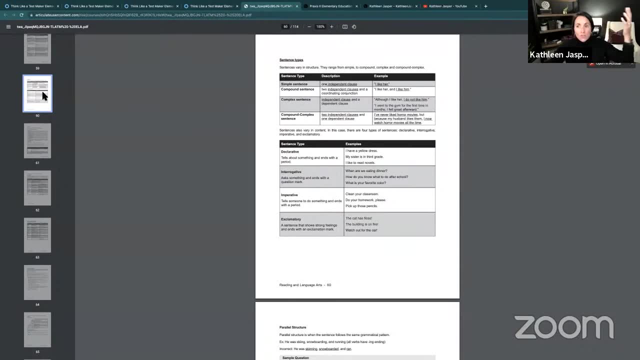 This is how I would do things. Do practice test. one is a pretest: Get a score. Do not look at the answer explanations. Just get a score and just be like: OK, this is my raw score. I got you know. 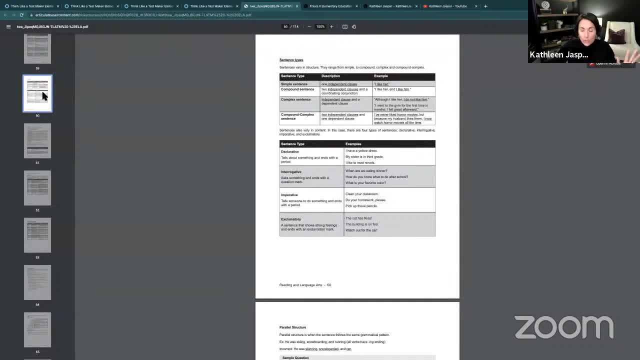 50 out of 80, which means you have work to do because you missed 30 questions, So you got it. You got to get back in there. Don't look at the answers. Just I am low in these areas and I'm going. 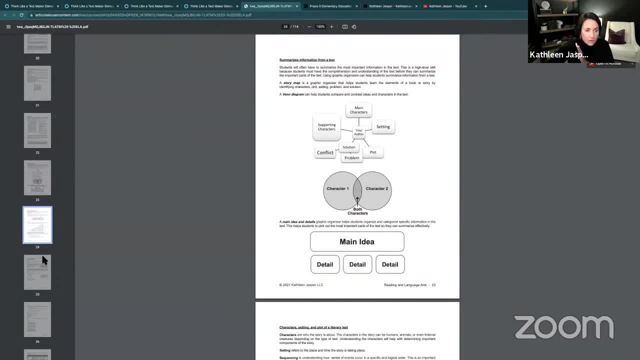 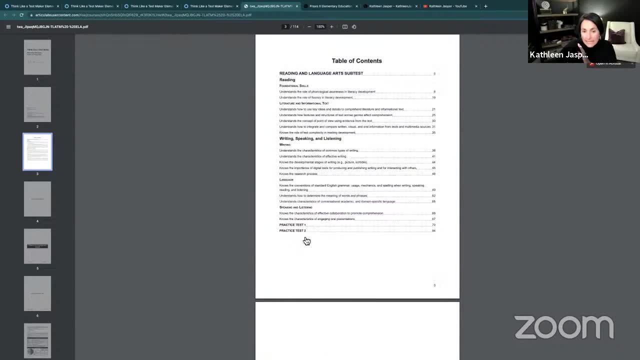 to now go in and work through all of this stuff here. OK, then what I would do is go back and take that same practice test again. Where are we Take that same practice test again? that now look at the answer explanations and see what you actually got wrong. 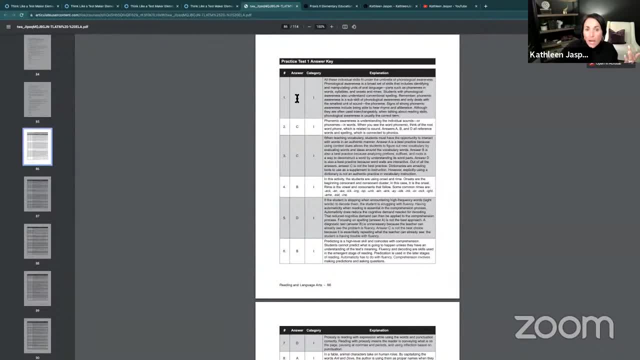 Do you see, by not looking at the answers as the pretest or not looking at the answer explanations as the pretest, you just mark it wrong and move on and don't don't kind of waste it. You can take it again and measure your skills. 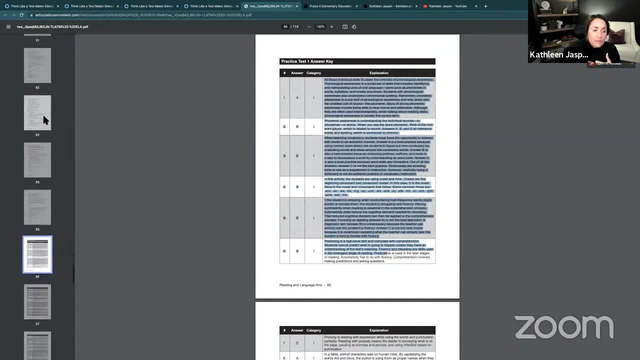 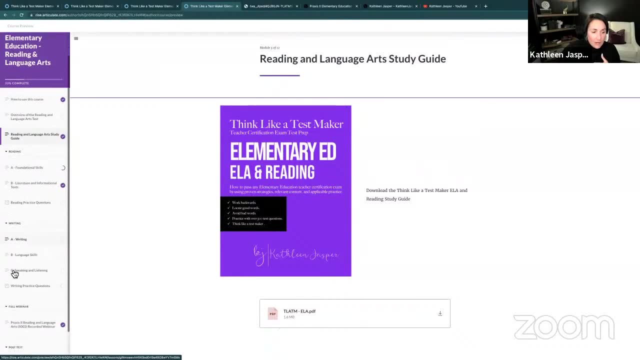 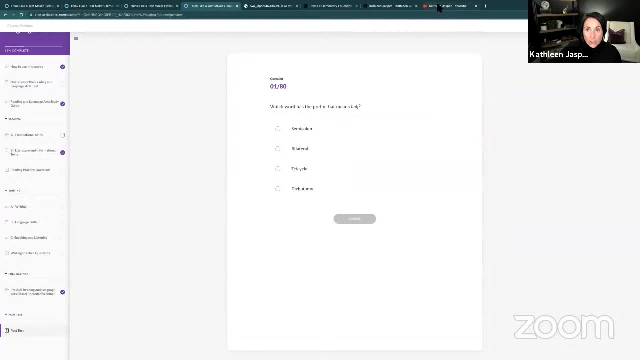 Then I would go back and see where you're still low And then I would use practice test two, which is right here, as the post test, And in our thing here we have that post test as an online module. All right Now. another thing I want to show you guys really quickly is on YouTube: 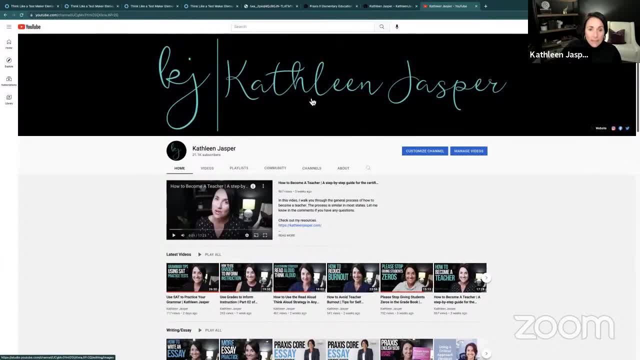 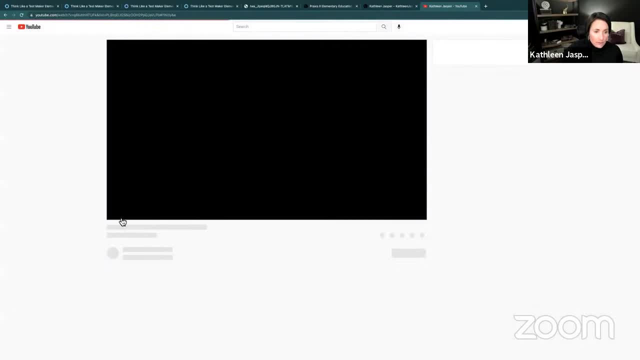 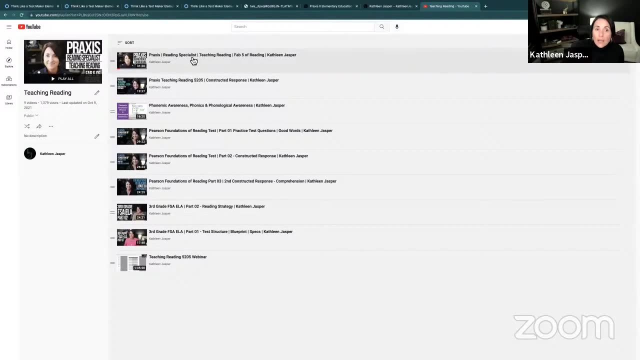 If you are someone who's like I don't have a lot of money, I need the free stuff. Well, guess what? This playlist right here: teaching reading playlist. You go here. Let me go here. OK, This has so many videos for teaching reading. 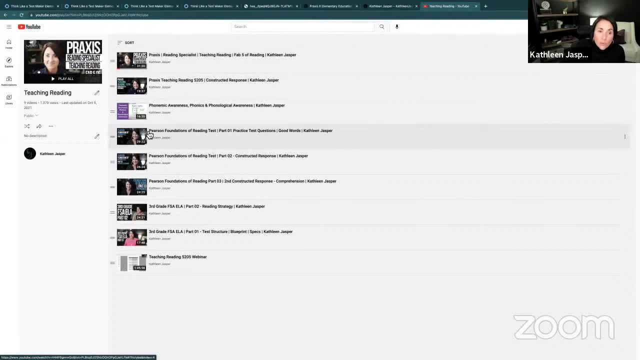 So if you want to go in and subscribe to the YouTube channel, do this. I've got teaching reading, foundations of reading. I have the constructed response. So if you're taking the teaching reading also, if you're a five nine zero one, 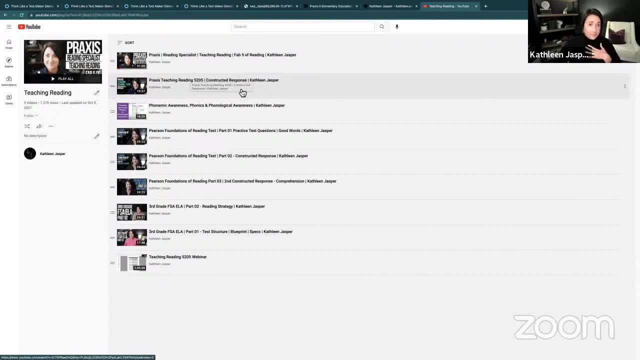 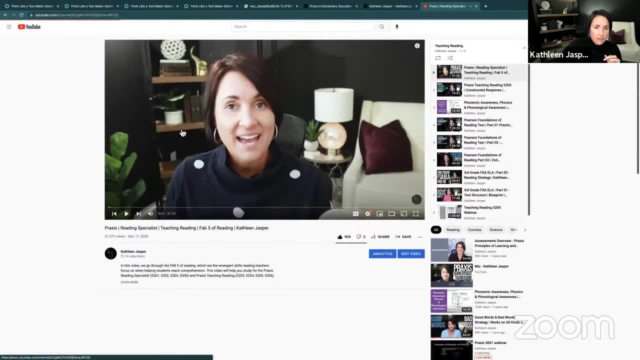 person and you have to take that teaching. reading this playlist is going to help you out tremendously. I also have OK, thank you very much. You are Kathleen Jasper, We see you. OK, you can. I mean, there's just so much here. 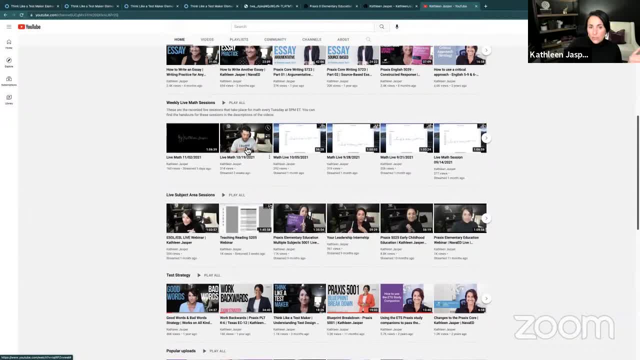 So I would definitely subscribe to our YouTube channel. And again, there's Jeremy. He goes live for math every Tuesday at five pm to six pm Eastern Time, And then- look at here, I have live subject area sessions. Here's my ESOL webinar- brand new ESOL webinar- teaching reading. 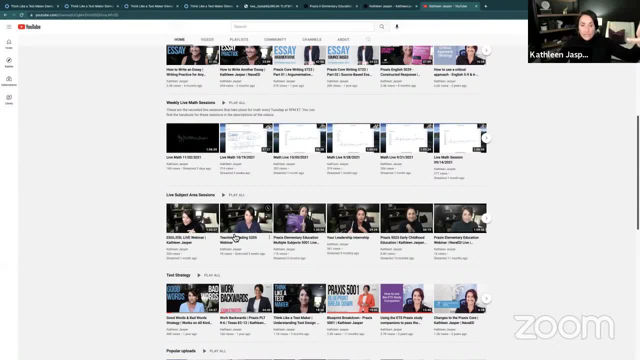 This is the same as this: You get a free study guide, You get the PowerPoints, you get everything. This is an old practice. elementary education I did nine months ago. This one's a little different, So if you want more, you could always do this. 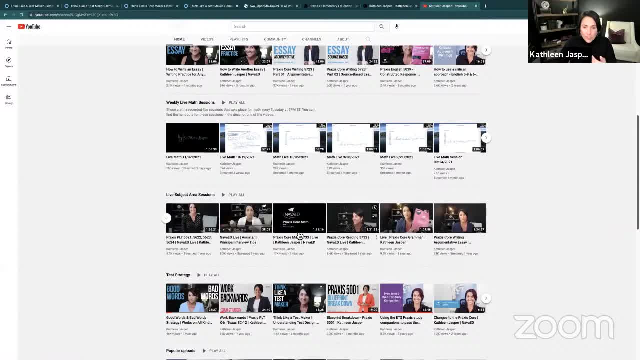 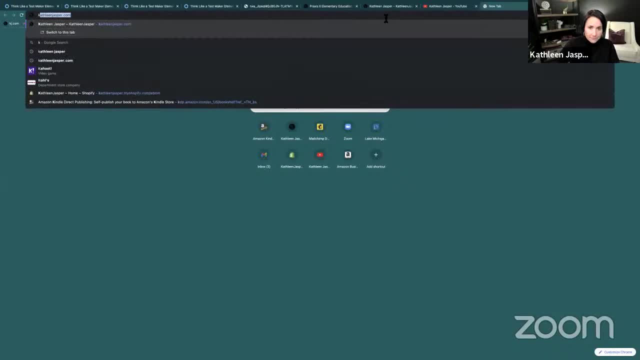 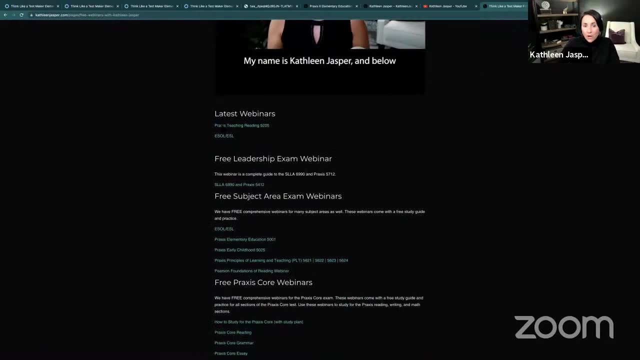 I got leadership early childhood, another elementary education, practice, core reading, math. I've got them all, So that really helps. You can also go to the website And here, if you go to free webinars, there's a video there that I'm talking to you, but they're all here. 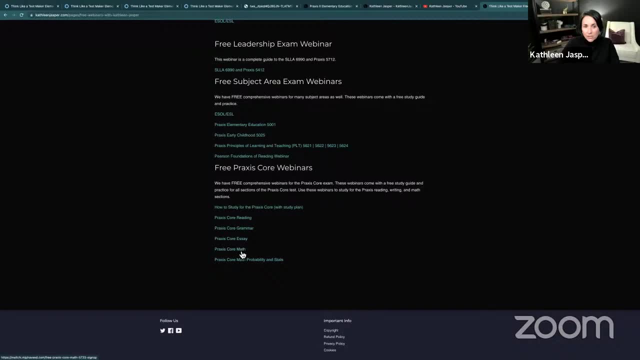 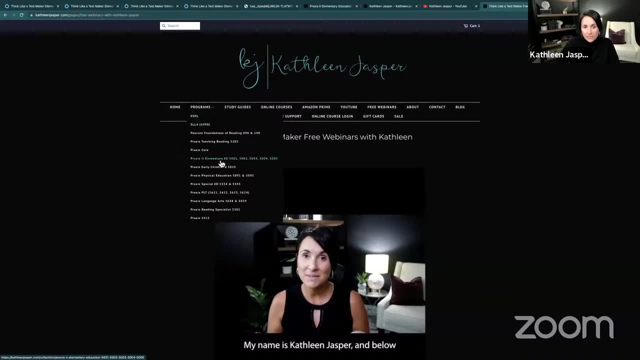 For you all of them in the practice core. I break up into all the sections. OK, but we got a new ESOL. We got so much here, And then under programs you can click what program. This is the program we're in right now. 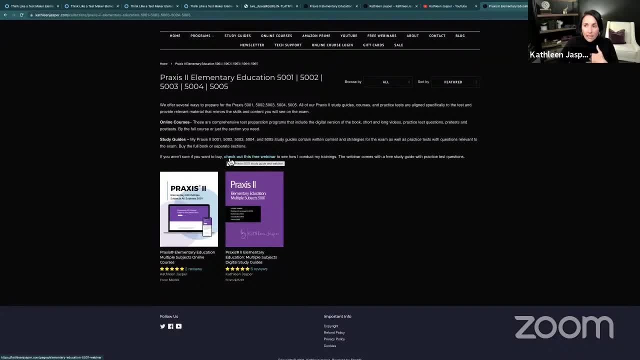 Five zero zero one, And when you get an email from me and a little bit with the replay, you're going to get an offer code that'll get you some money off. So if you won the store credit, don't use it yet until you get my email, because you'll also get. 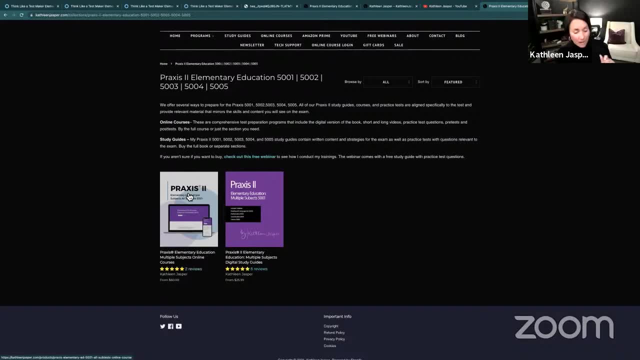 some money off So you can use a discount code and your store credit- John, Destiny and Cody- and I'm about to pick one more person, So that really helps you there. And then, finally, I just want to bring to your attention: 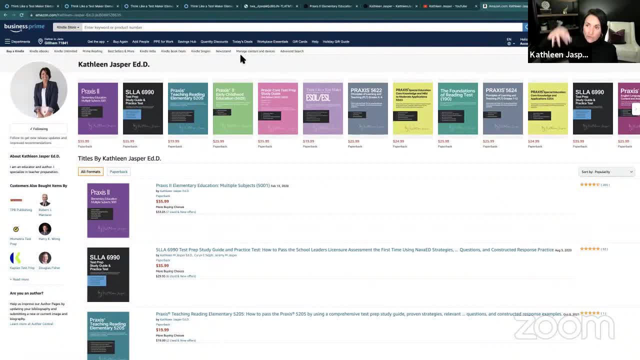 I want to share this with everybody. I don't sell physical books from my house anymore because I couldn't. It takes too long, Take six to eight days to get to all over the country. When I was just shipping in Florida it took two days. 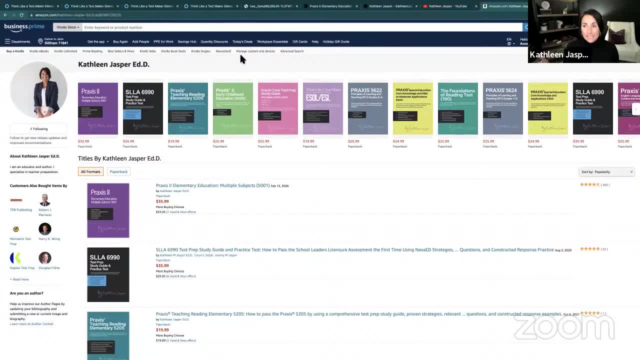 Then I became a national brand and it was taking like eight to ten days. Amazon Prime will get it to you in like twenty four to forty eight hours. I cannot do that. And they offer free shipping. I cannot do that as a business owner. 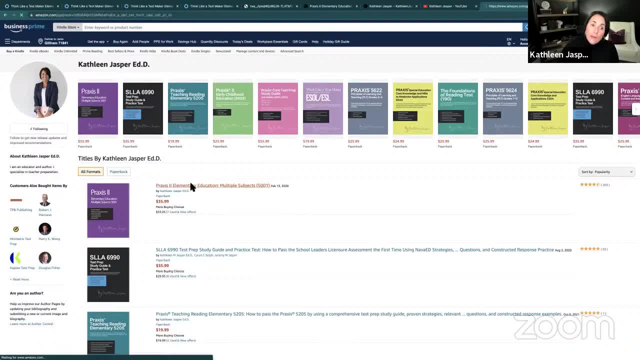 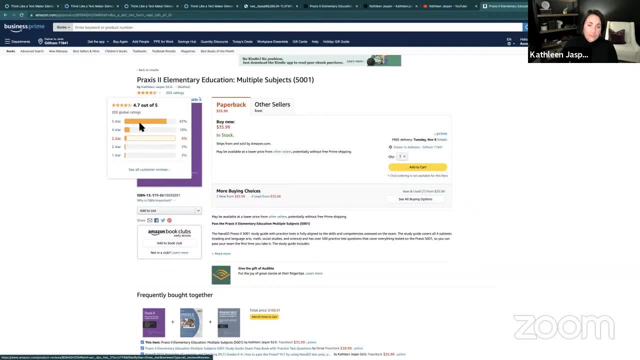 So all of the physical books are available here And I'm very proud of our elementary ed because we have two hundred and three five star ratings, are close to five star ratings. Of course we we always have some people who are not satisfied, but we do. 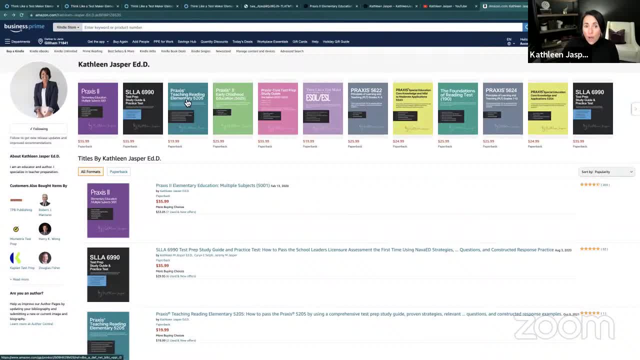 our best to make sure you're satisfied. and also all of my books are here. This is a new book: The Foundations of Reading. all five stars. This is all. book is brand new. This will help you with any ESOL exam, also available on our website. 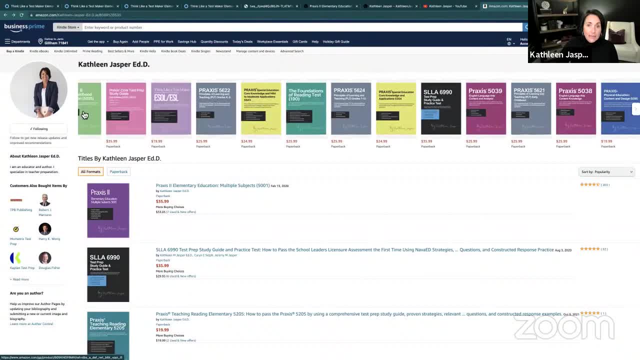 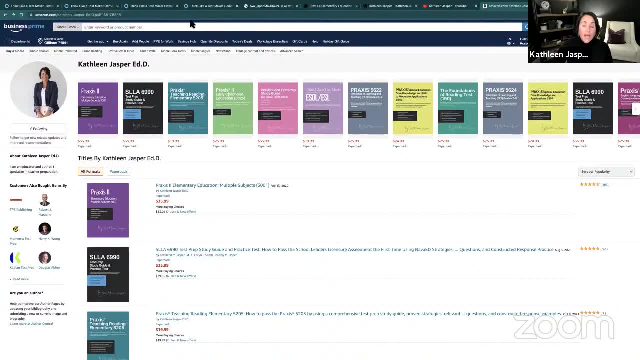 So we have lots of books for the practice exams and the Pearson exams And I'm working on Texas. Texas is my next state, you guys, So if you're from Texas and you're here, I swear I'm working on it. But it took me a long time to write all these books. 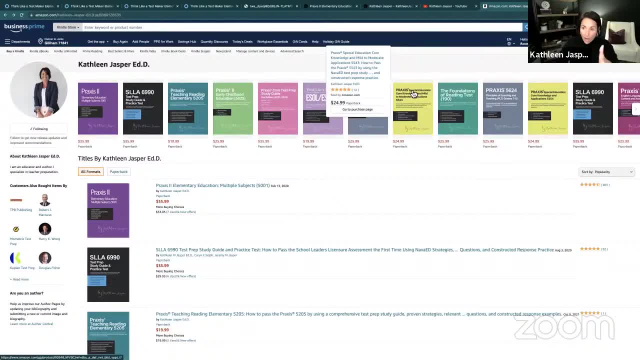 It's not as easy as it seems. So I want to make sure they're right and that I'm giving you the right material And you can see. you know we get a lot of five star reviews because they take a lot of time to make sure they have what you need, that they're aligned. 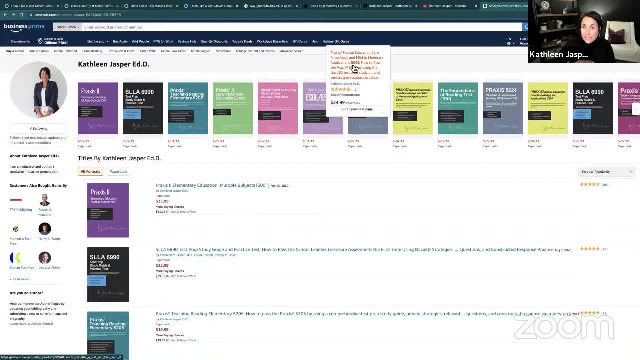 to the exam. Also, those of you taking this test. you might be taking your PLT as well, your five, six to two, or middle or high school or whatever. So that's something you may want to come back for And you can also see that we have it right here. 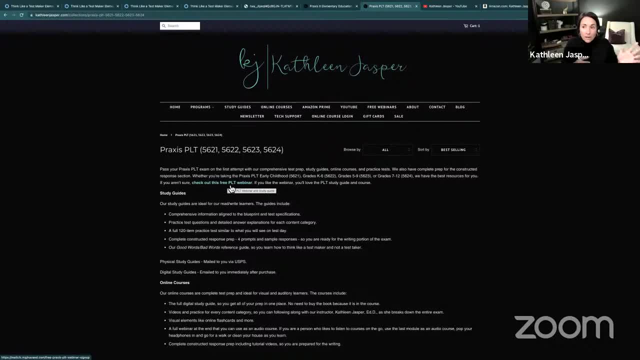 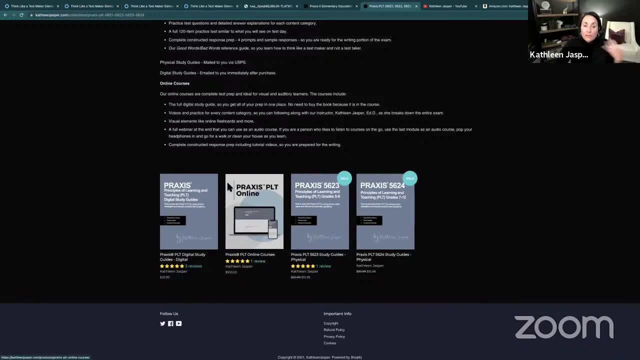 And I have a webinar for that. Check out this free webinar. So I always have a webinar to go with to show you what we do And it's to give you a little free so you see how I do things And if you like the way I do things, you'll love the course. 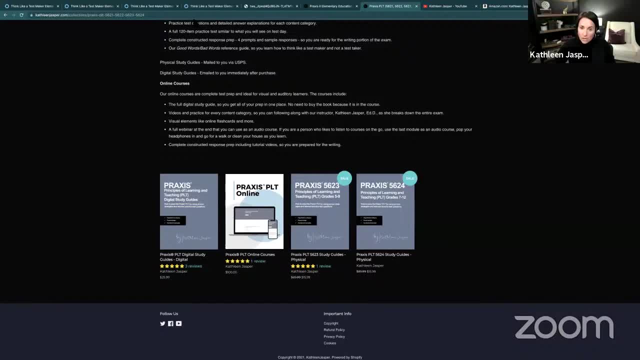 Also remember: all courses come with the book, So don't buy both. If you just want the book, then just buy the book. You do not get the course with the book, But if you buy the course, you get the book with it. 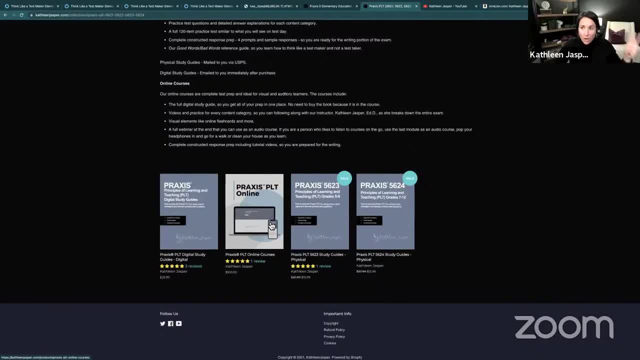 Okay, So remember that. don't buy both. Usually, if I see somebody who bought both, I go in and refund them immediately because it's an extra charge and you don't need it. Okay, And of course, you saw our course and you saw our books. 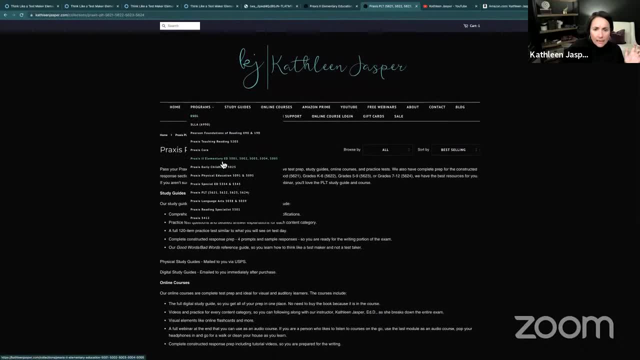 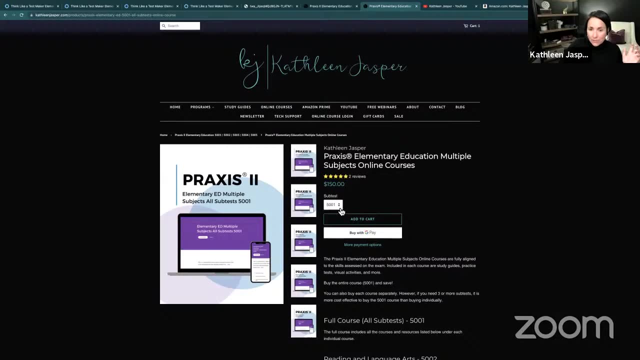 And again, one more thing I wanted to show you really quickly with the elementary ad. you can buy them separately. So let's say you don't need the entire course, you just need the math. Some people were here for just the math. 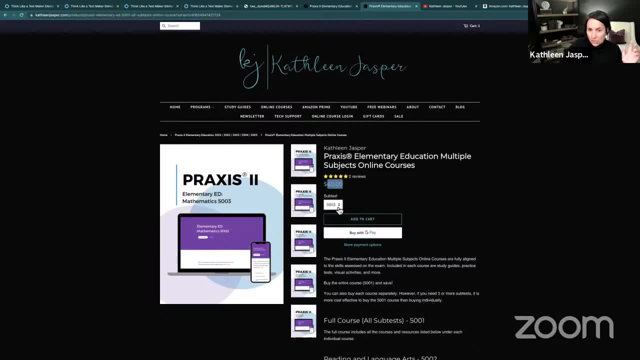 You can just buy the math and notice it goes down to $60 because it's just the math. Or maybe you just need social science. Just use this drop down to do that, And that will do that the same with the book. Let's go back here. 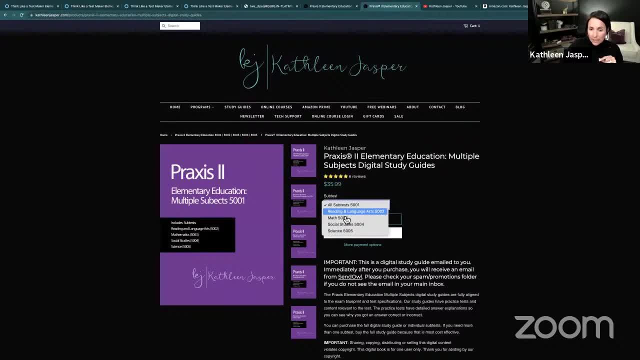 If you only need one section of the book, you can get that digitally. So let's say you just need the math, It goes down to 2599.. You just need the social studies or you need the full. Grab the full, All right. 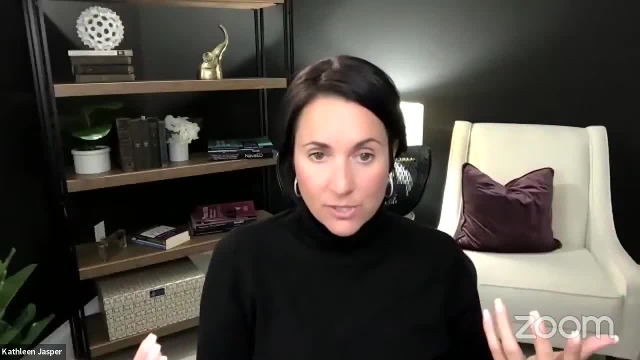 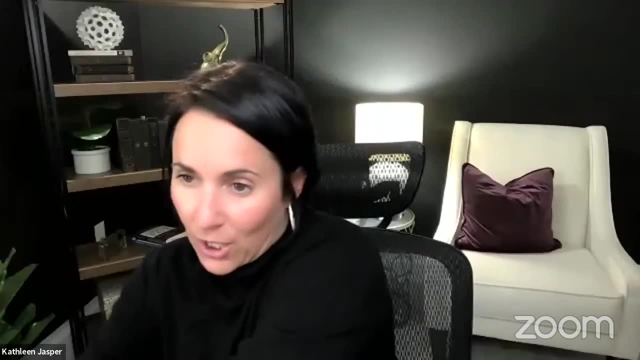 Once this is over, you're going to get an email from me with all the resources. If you're watching this in the future and not live, the link is in the description to get all the resources. Let's go to our final winner of the day. 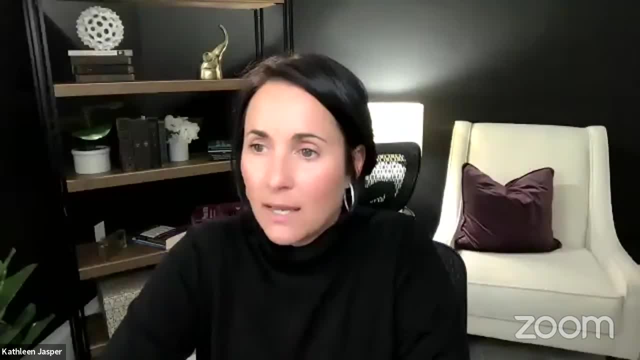 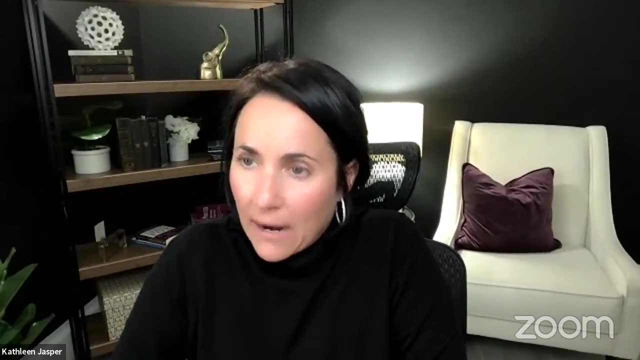 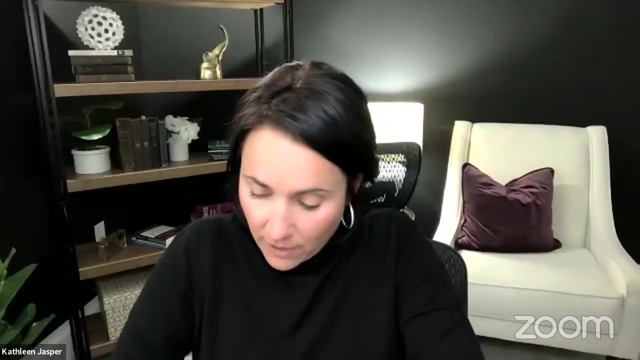 All right, My generator is going and I've got Luz Baron. Luz Baron, are you here? Let's just see here. All right, Luz, you are another winner of the $50 store credit. I'm going to get you an email as well, and you'll be able to use that. 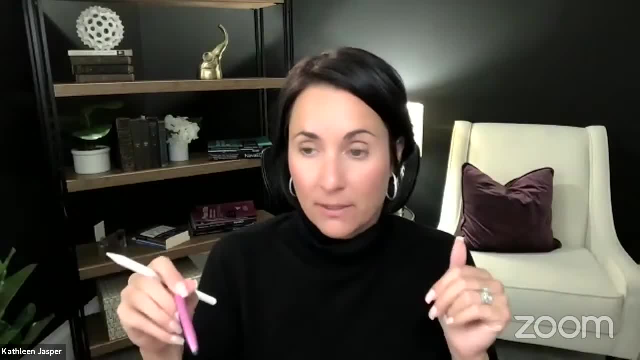 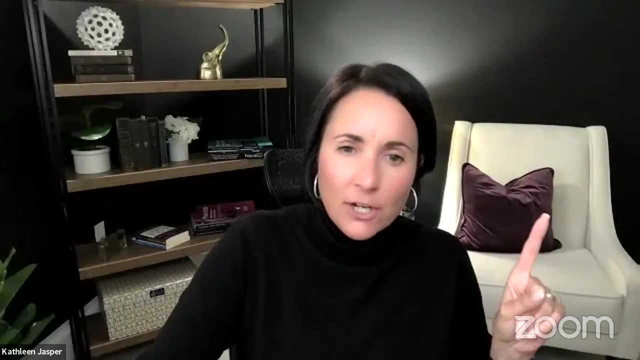 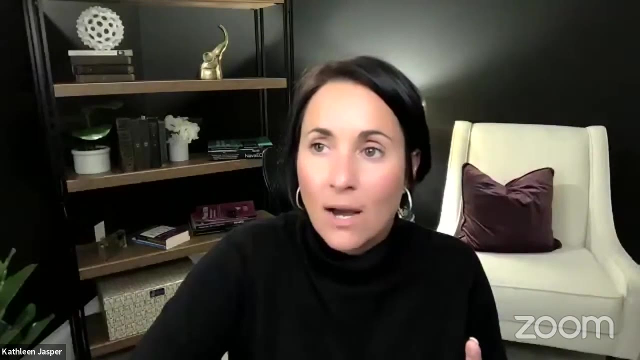 But again, wait to buy anything until you get both emails. So the store credit and the offer code. and I'm really excited, You guys. the offer code today is hang on, Let me, let me see. I added the offer code recently. 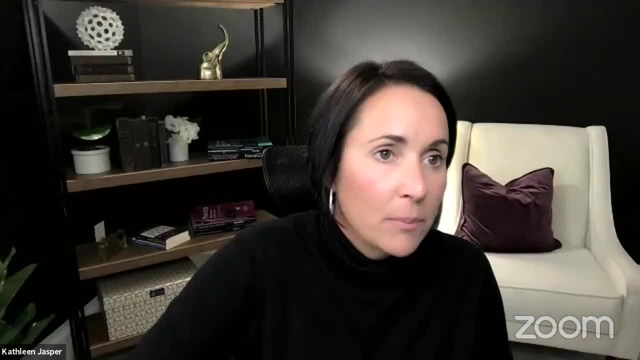 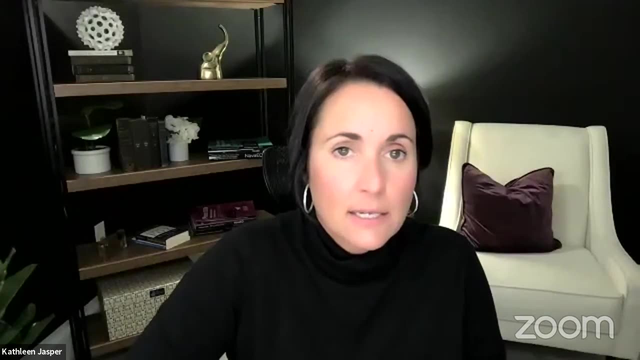 Let me just see what it is. If you want to go in now, If you want to buy it, I'll put it in the chat. Let me just grab my offer code here. OK, this is the offer code. I'm throwing it in the chat for you. 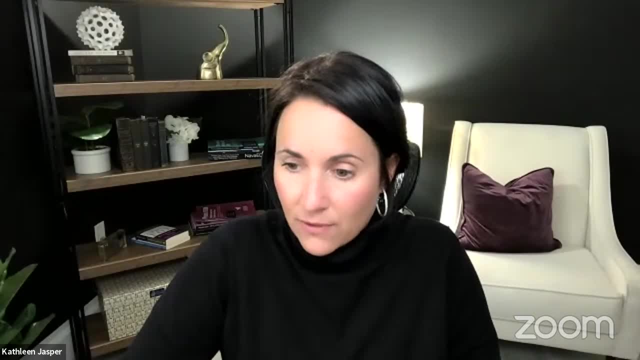 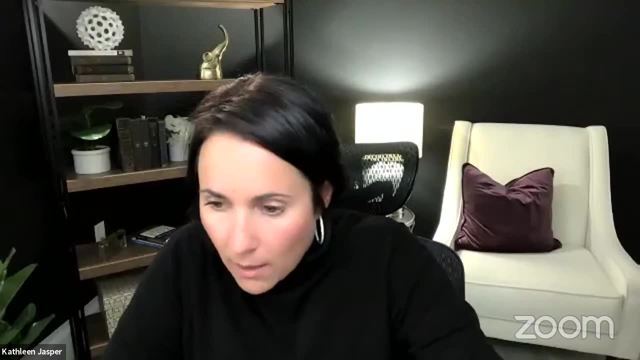 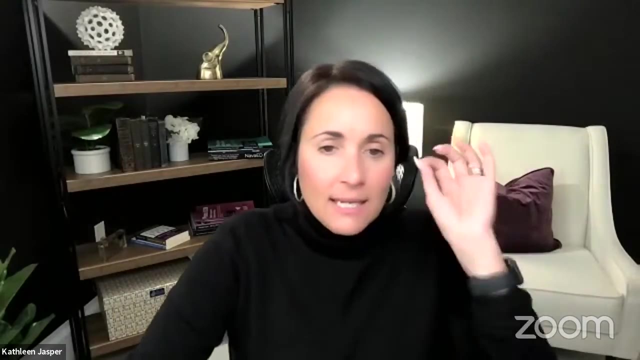 If you don't have time to wait for my email and you're like I want to get it now, That's fine, Let me go to everyone. This is the offer code, So it's EE Web 2021.. EE Web like elementary education web. 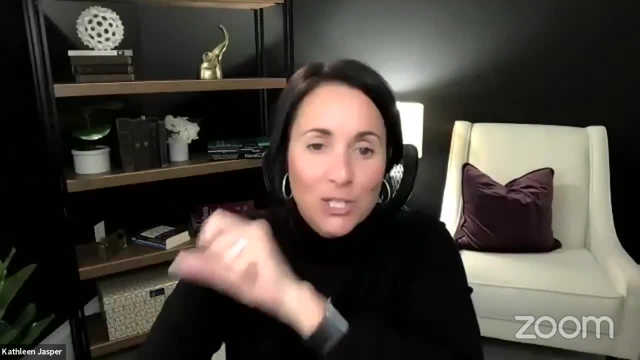 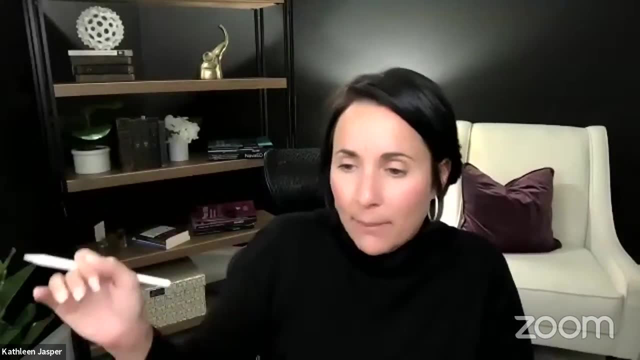 like Webinar 2021, EE Web 2021.. The reason why we have different offer codes for different things is we like to track to see if this was working, or whatever. So EE Web 2021.. But that will also come in an email for you, and the replay and all of that. 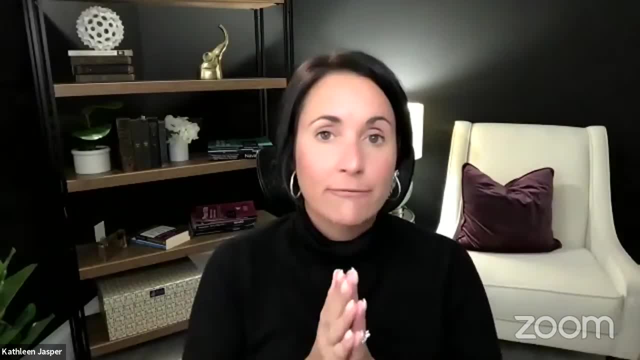 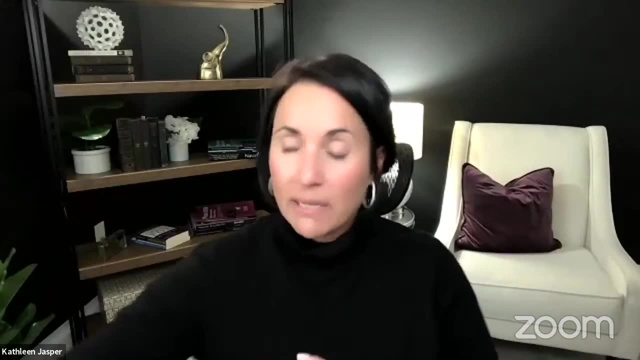 All right, OK, so that is the final. Now, if you are here for the Texas exams, you have one more section, which is the PE, the arts, and all of that. We didn't cover that today because I am working mainly for the Praxis 2, but I am. 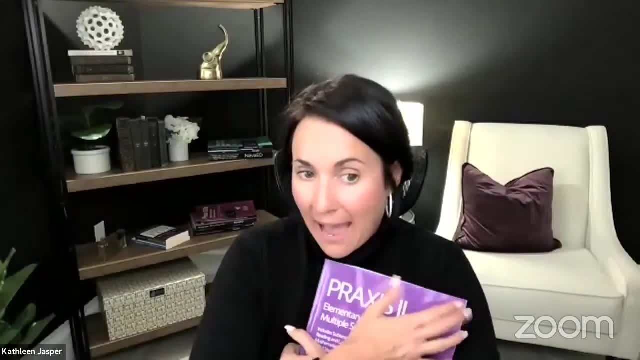 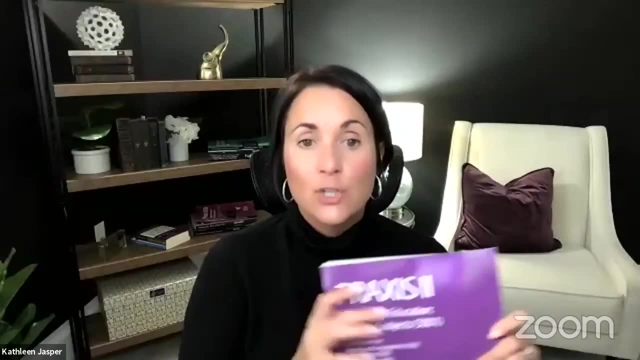 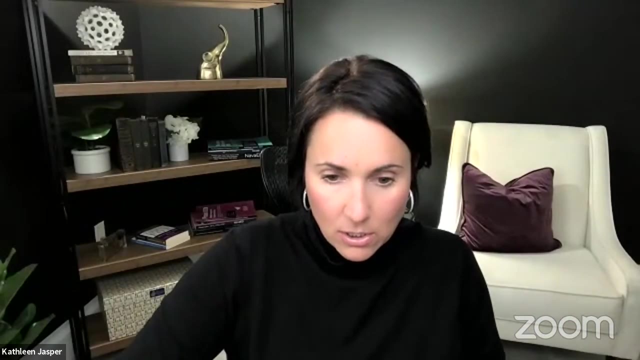 on the Texas exams, And so your book will have that extra section. So if I do have some resources for that. So if you want this book and you want the supplement, you can email me at info. Let me show you the contact page. 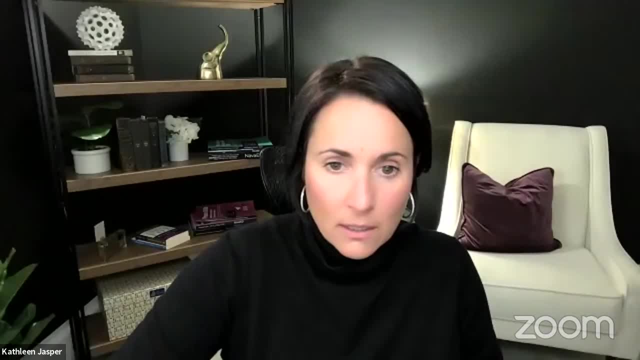 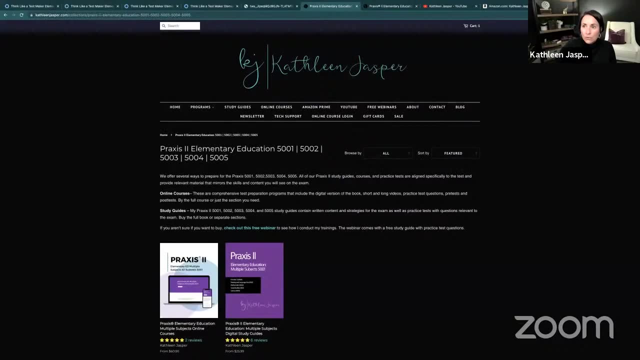 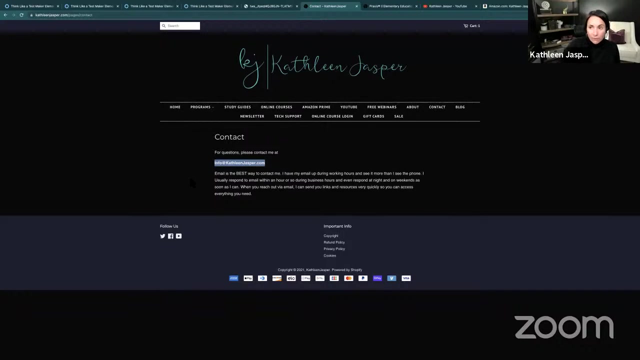 Let's go Hang on. We go here So you can go to This contact page every time if you want to email me. This is the best way to get in contact with me. I have my phone with me all the time. 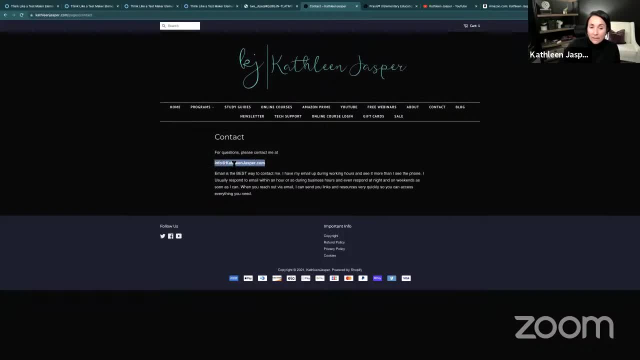 I have people watching my email so that I, if anybody has ever emailed me, you know that I get back to you pretty quickly. So if you have any questions, info at Kathleen Jasper dot com. But if you are a Texas person and you want to buy this program but you're like